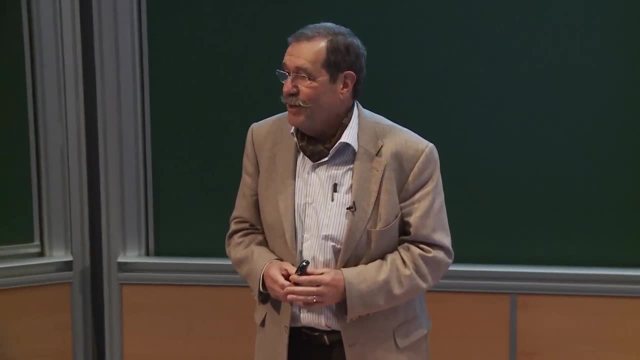 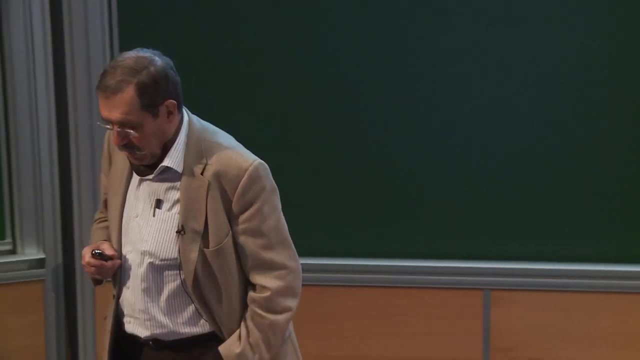 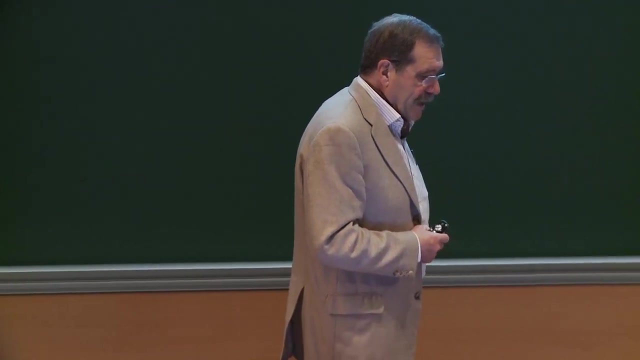 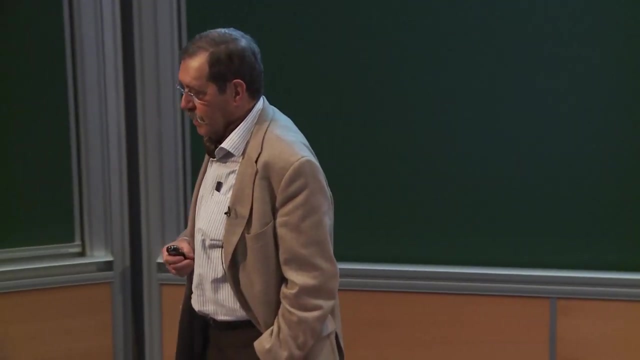 to interact more than I ever did in my life with a mathematician, And it's very interesting. Now, what is my talk about today? It's about the discoveries which established quantum optics starting in the 50s, 1950s, not 18.. 18 is more classical optics, But starting in the 1950s. 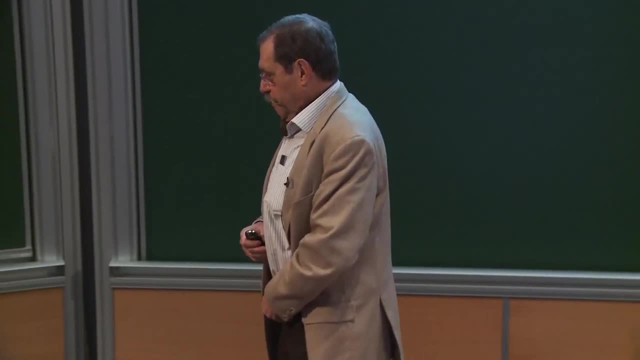 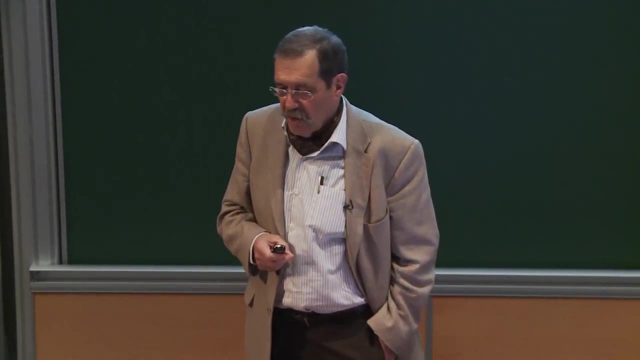 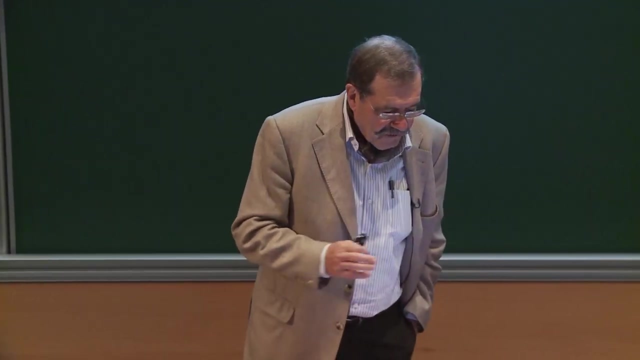 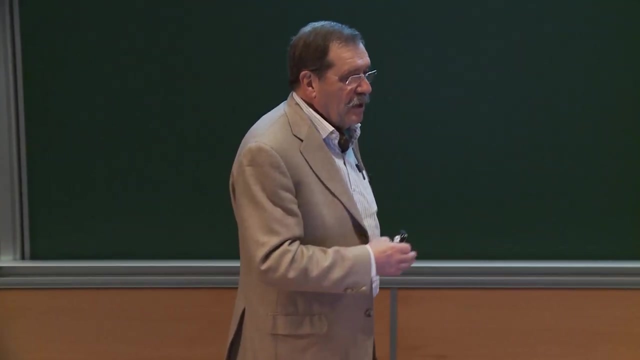 there were a famous paper called the or effect, discovered the Hambury-Brown-Twiss effect, which is considered the founding phenomenon which started quantum optics. Then there is something strongly related to entanglement: Hong-Wen-Mandel and, of course, Bell. And I have a pretext. 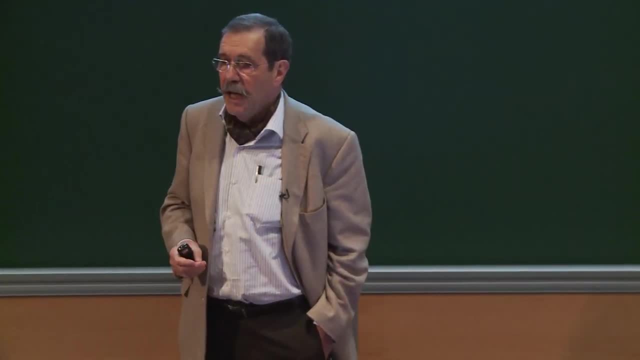 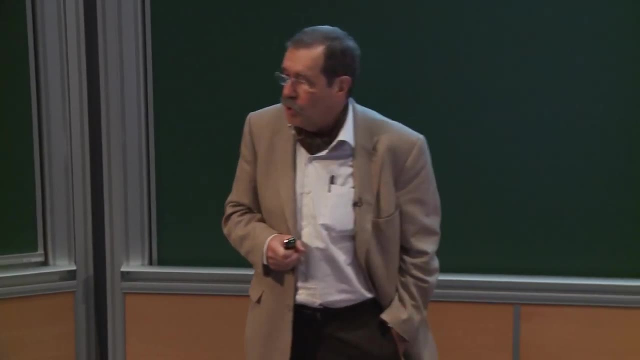 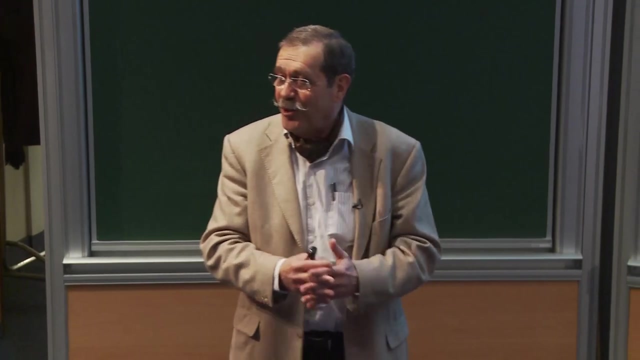 and I love explaining this story And it turns out- this is why I have this subtitle here- it turns out that quite often people come and say, oh, all my life I heard about HBT but I did not know what it was, So I'm so happy that you're explaining that And the pretext for explaining it. 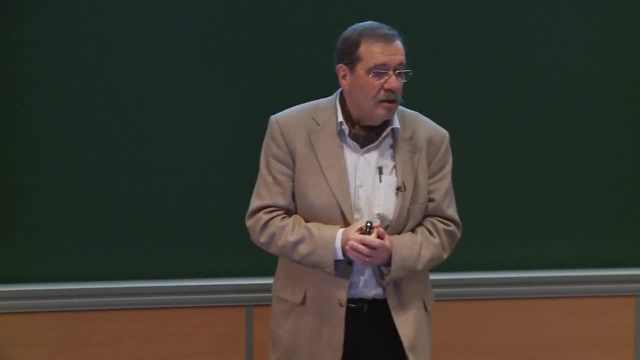 is that all these effects which have been in quantum optics, they are the effects of quantum optics And that's an effect that is very important. And the pretext for explaining it is that all these effects which have been discovered and studied with photon, we are revisiting them. 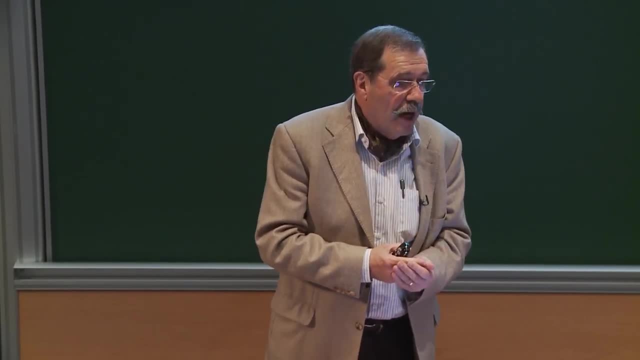 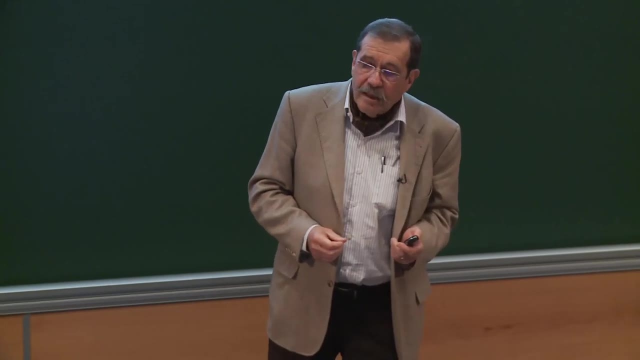 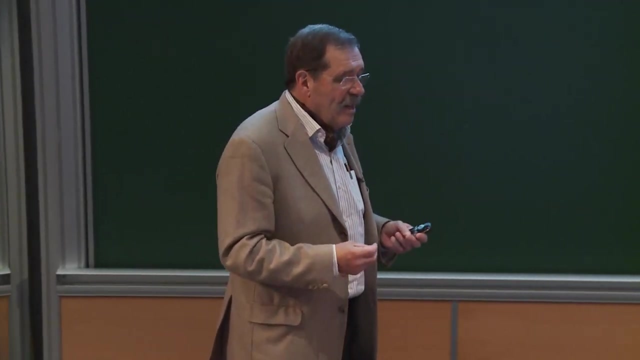 with atoms in place of photons. And so you will see in the talk, from a certain point of view, after all it's a quantum particle, But it's a special quantum particle. It's a particle which has a mass, okay, and a photon has no mass, And in some cases it makes a serious difference. 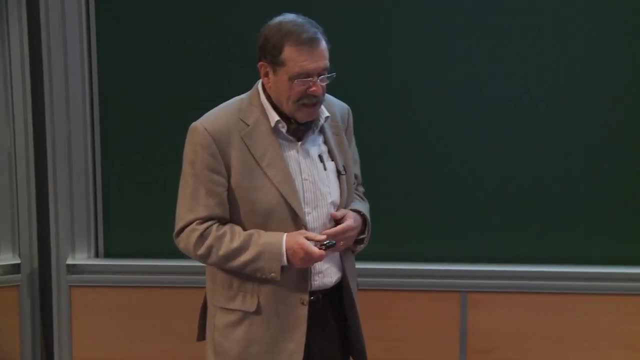 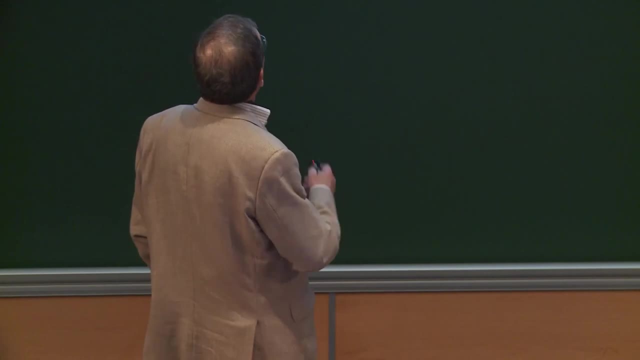 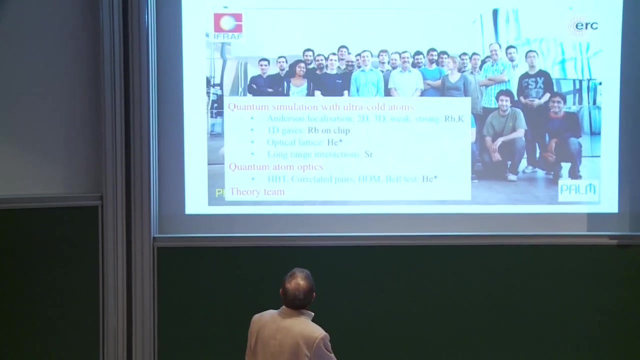 And there is another difference that I will emphasize during this talk: Dr Jean-Marie Sauter, Professor of Mathematics, University of Oxford, UCD. So let us start Well. this is to say that we have a group with plenty of people working on many different subjects. So we work on quantum simulation with 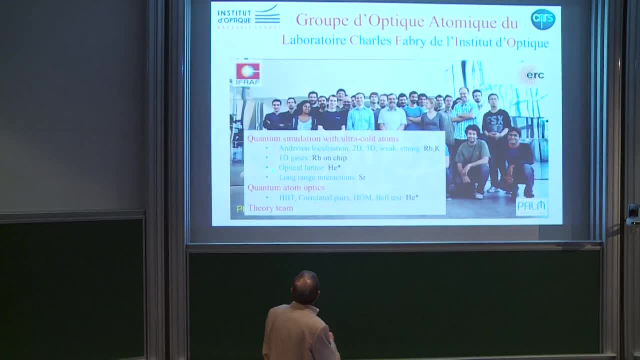 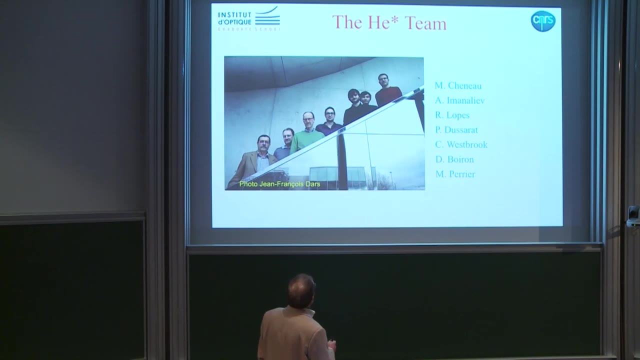 ultracold atoms, Anderson localization and other subjects, But the topic of today is quantum atom optics, That is to say, quantum optics not with photons, quantum optics with atoms. Okay, And these are the people who have performed the experiments on metastable helium that I will describe today. 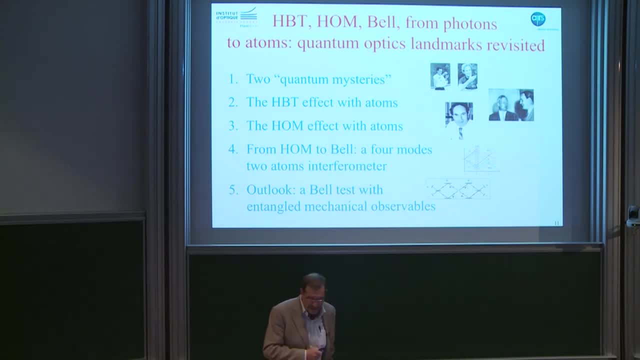 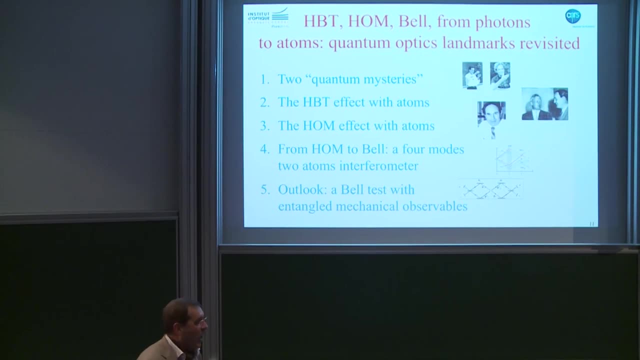 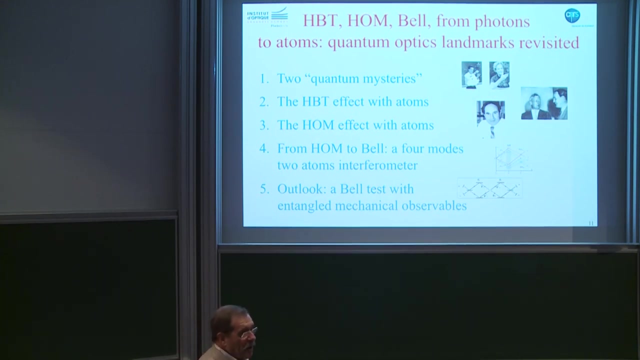 Okay, And I like to start with the result of my thinking about quantum physics. I really I'm still absolutely amazed by quantum physics. I think quantum physics is a big mystery, But I think, when thinking deeply about it, there are two different kinds of mysteries. 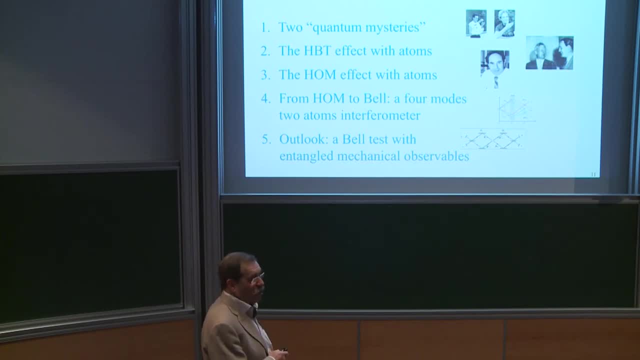 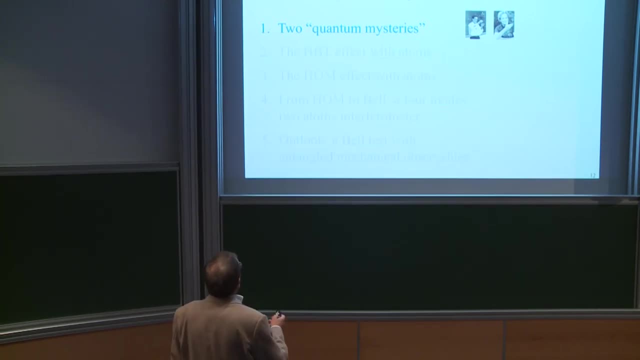 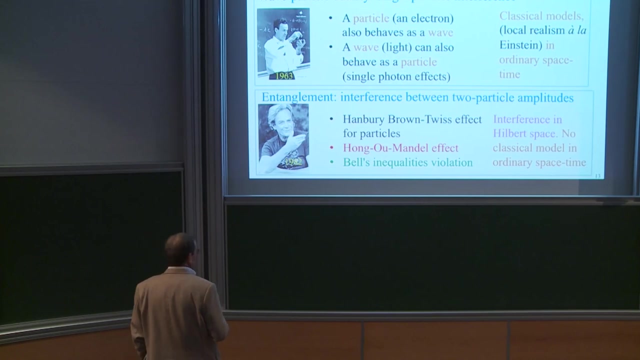 And because I would not dare to present it if I was alone, I have a strong support by a citation from Richard Feynman. So let us start with two quantum mysteries according to Feynman In his book, the famous book Lectures on Physics, published in the early 60s. Feynman- 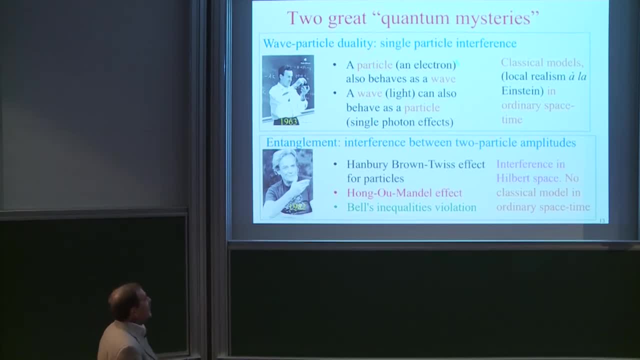 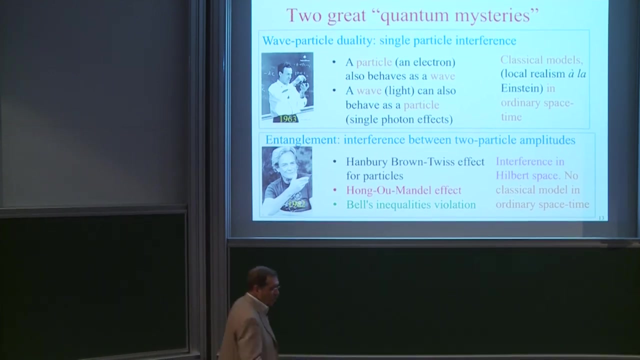 emphasizes wave-particle duality and says this is the only mystery of quantum mechanics. Okay, And wave-particle duality is about a single particle. If you have a single particle, a single electron, a single atom or a single photon, okay, but let's say a single. 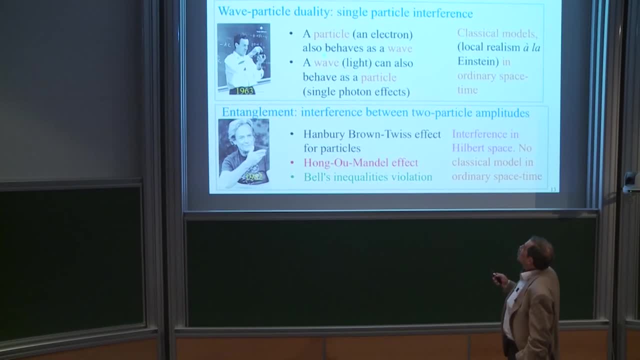 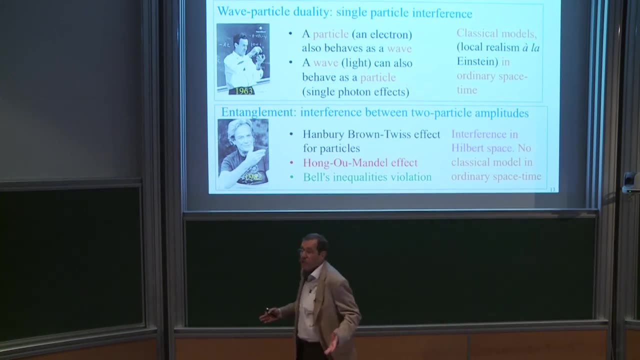 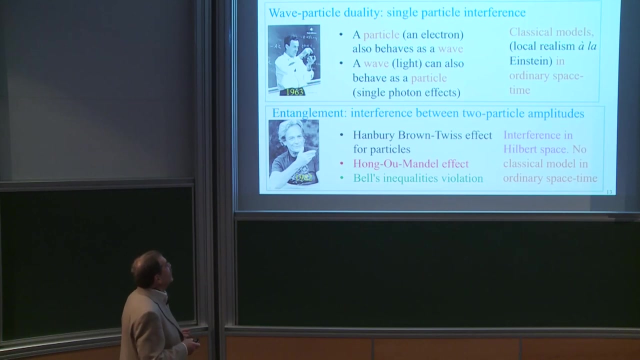 atom, a single electron. we know that it can also behave as a wave, And vice versa. something that we think is a wave that is light, for instance, can in some circumstances behave as a particle. okay, And this is wave-particle duality. 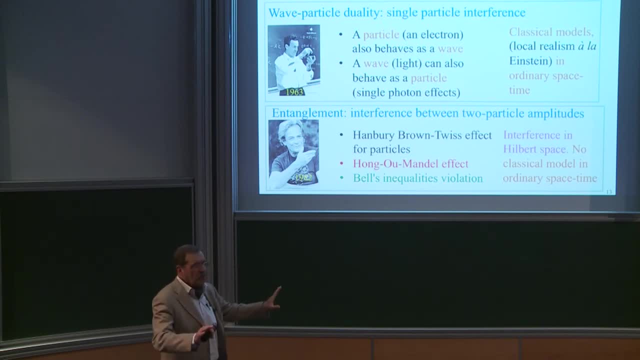 20 years later, after here claiming: all the mystery of quantum mechanics is here. Okay, After 20 years. in the early 80s, it was a time when I was completing my experiments on the test of Bell's inequality, and it's about that Feynman recognizes that there is something, a second 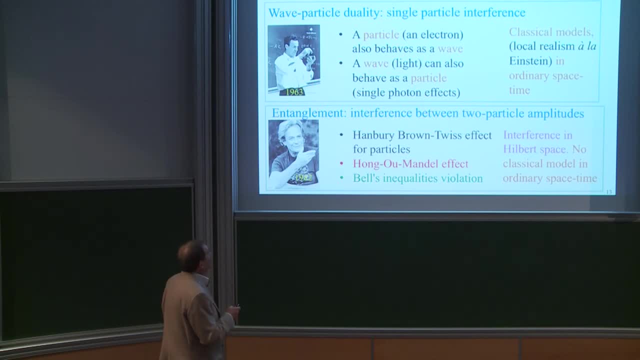 mystery. And the second mystery is around entanglement, And the first obvious difference between wave-particle duality and entanglement is that wave-particle duality is about a single particle, while entanglement is about two particles, And so there is a series of wonderful 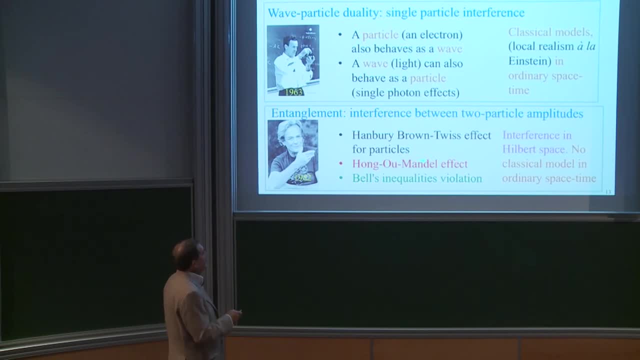 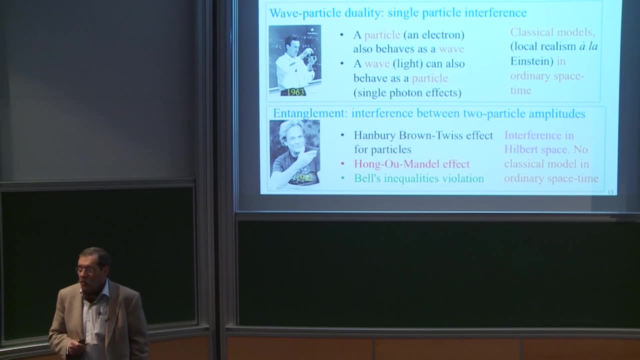 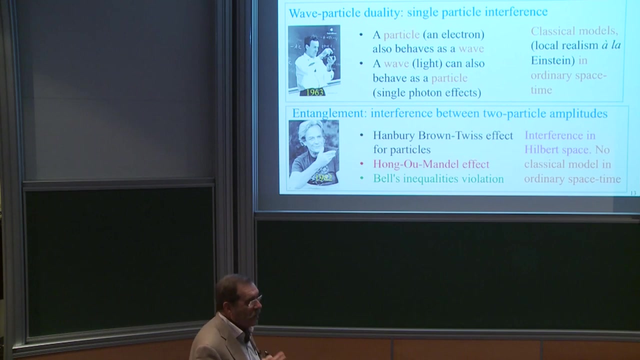 effects, Hambury-Brandt-Wies effect, Hongo-Mandel effect and test of Bell's inequality, Bell's inequality violation. And I really think that these two mysteries, or call it whatever you want, are different in nature for the following reason, And again, this is a result of thinking: 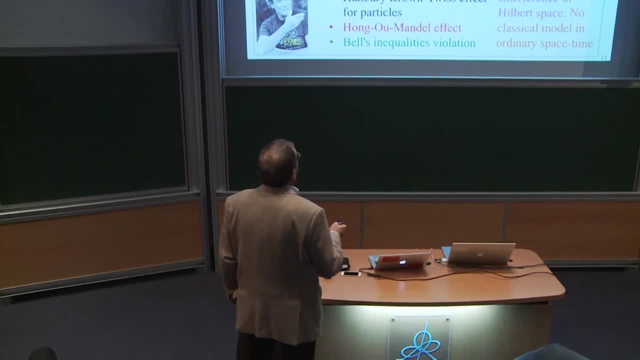 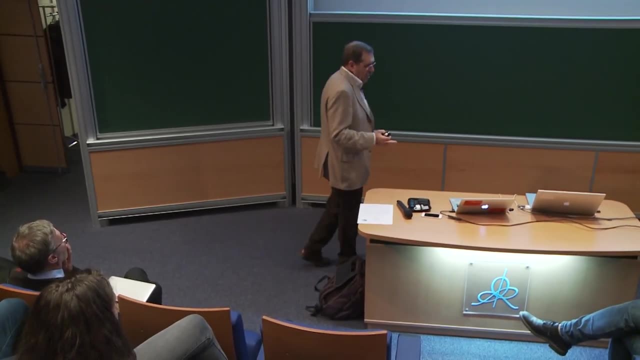 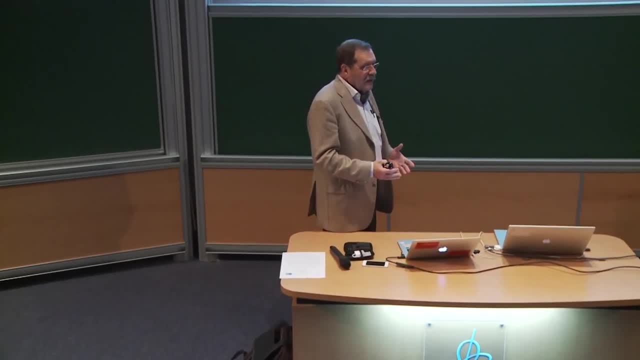 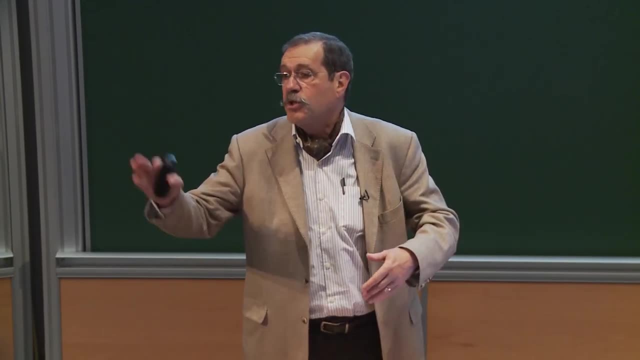 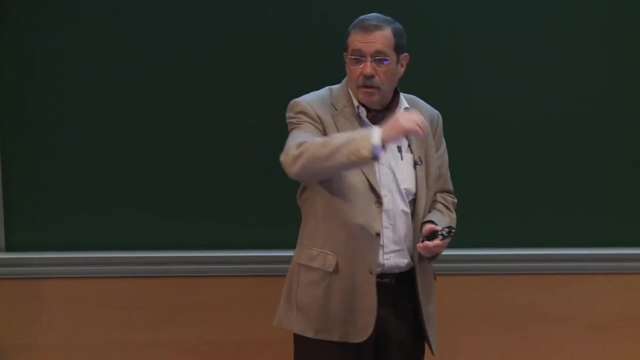 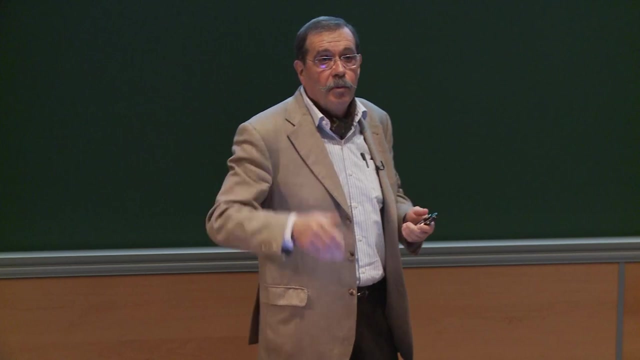 come with models describing things in our real, ordinary space, three-dimensional space where we live. okay plus time. okay, space plus time, Because when I have a particle, I know what is a trajectory of a particle And if I have a wave, I know exactly how to describe the propagation of a. 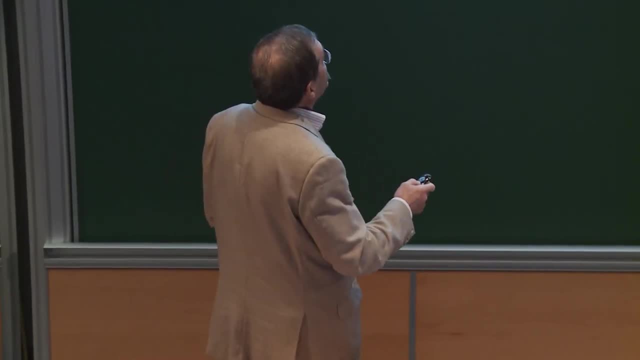 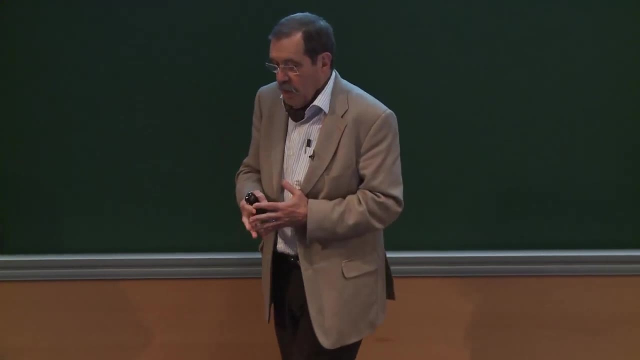 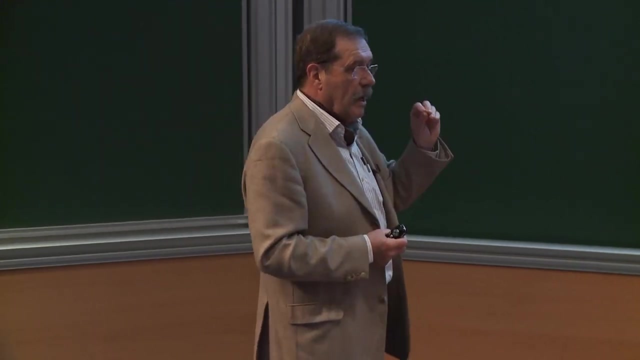 wave, So I can describe everything in our ordinary space-time. When it comes to entanglement, the good way of describing it is to describe in a Hilbert space, which is a tensor product of the space describing the first particle and the space describing the second particle, And in that 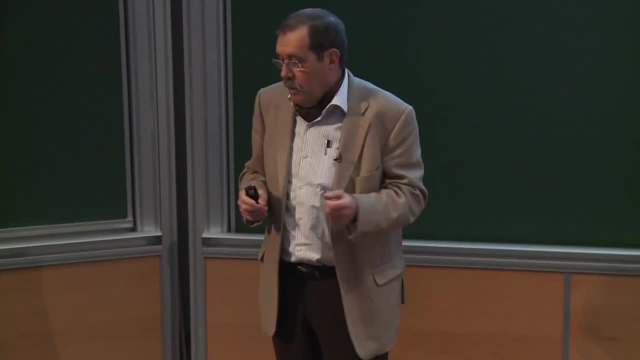 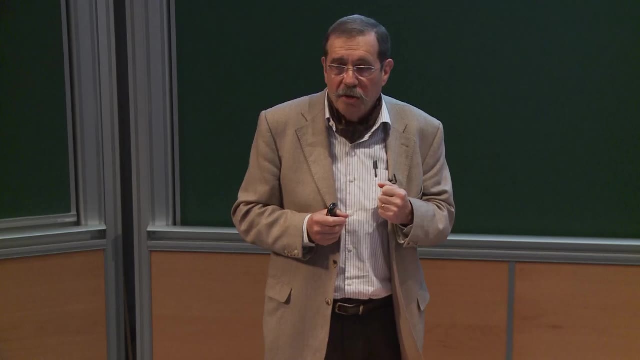 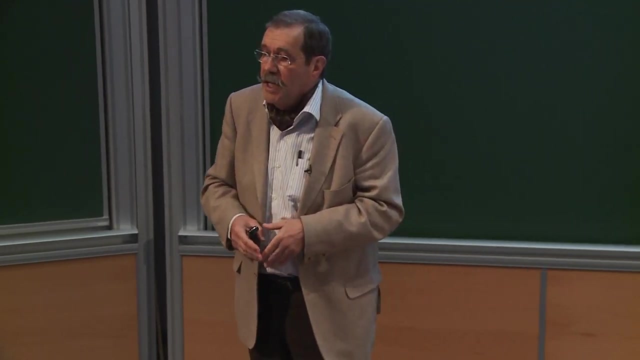 abstract space, there is no problem. But as a great theorist of quantum optics, H R Perez, once said, quantum phenomena do not happen in a Hilbert space, They happen in a true laboratory, in a real laboratory. In a real laboratory is our ordinary space, And as soon as you try to 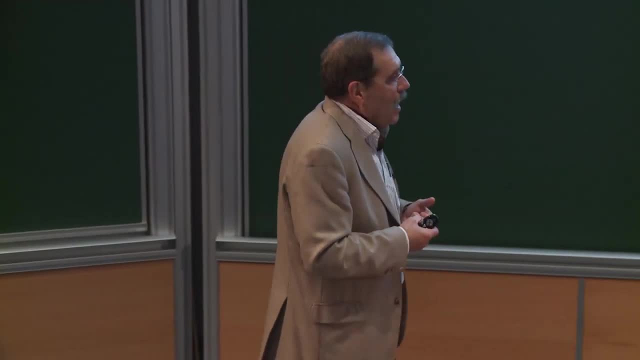 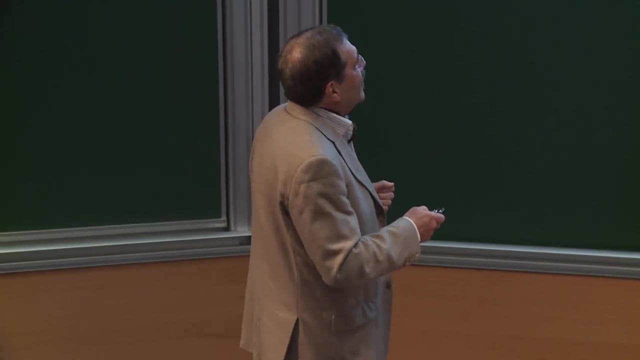 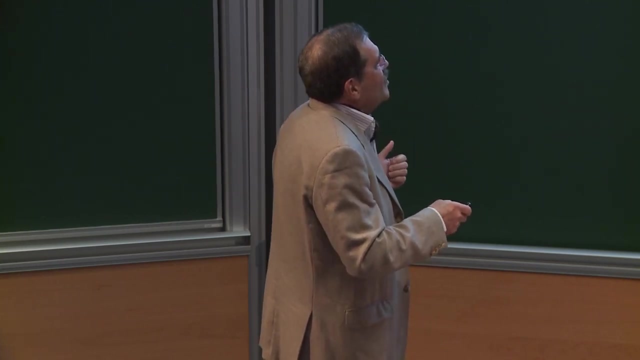 represent things in our ordinary space. then you have bizarre things like nonlocality, et cetera, et cetera. okay, The fact that the only good model for describing it is in a Hilbert space and the fact that there is no reasonable classical model in ordinary spacetime makes a major difference. 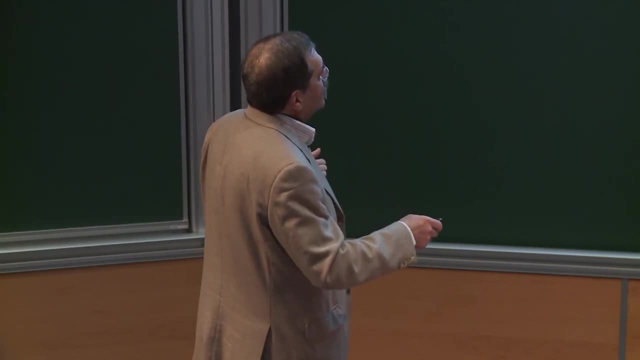 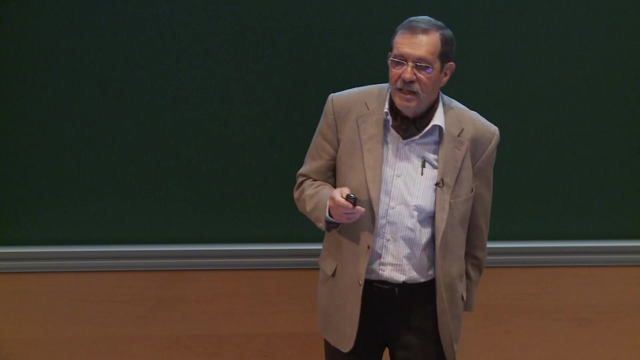 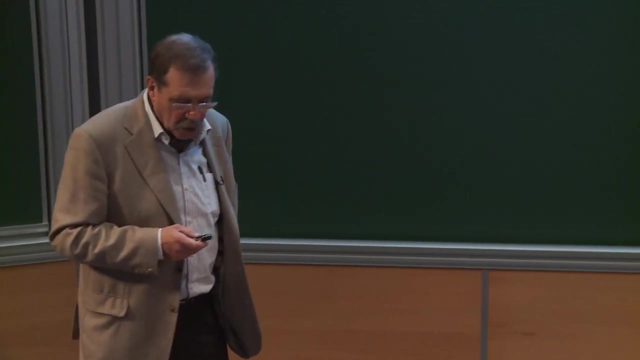 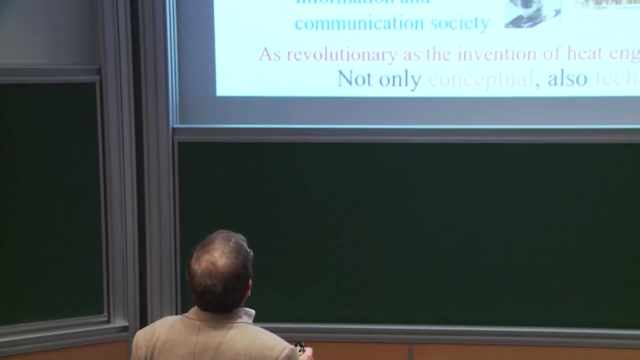 between these two. So today I will really concentrate on this, that is to say on the experiments which suggested that entanglement is really something important and fascinating. So, to finish with this global presentation, what we call the quantum revolution. but let 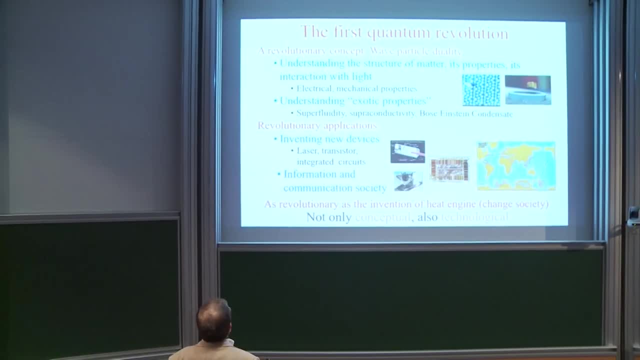 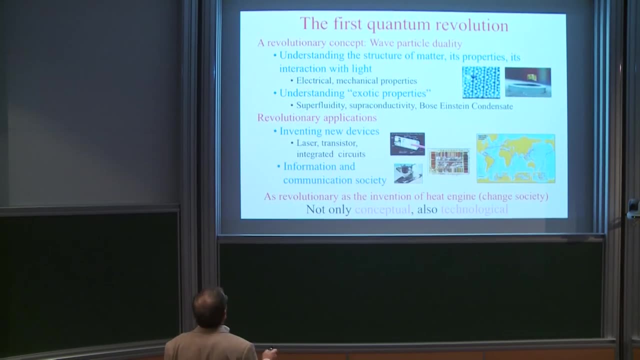 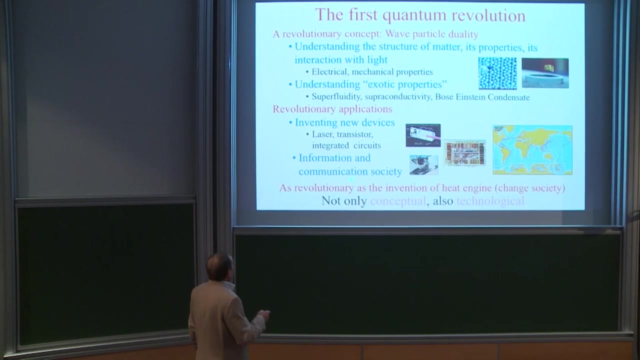 us call it. the first quantum revolution was first a revolutionary concept about wave-particle duality, And it allowed to understand the structure of matter, its properties, its interaction with light, and then transistor, etc. etc. It has given us the environment. 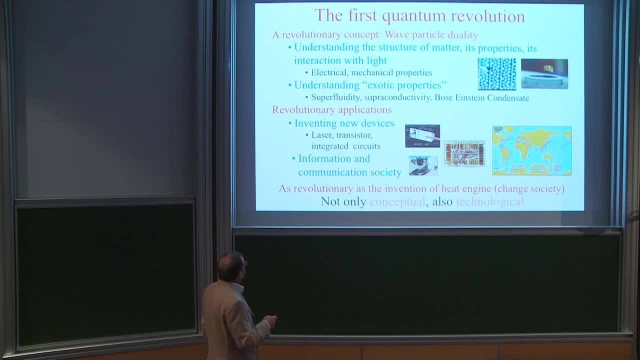 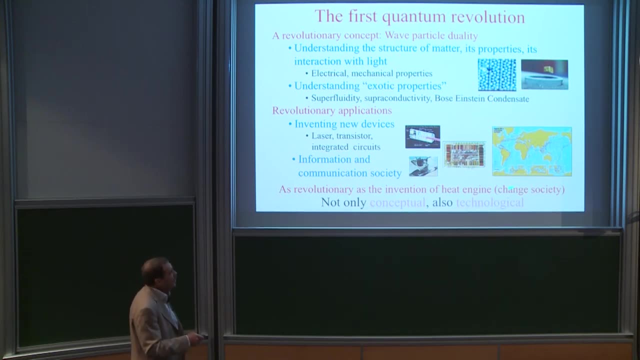 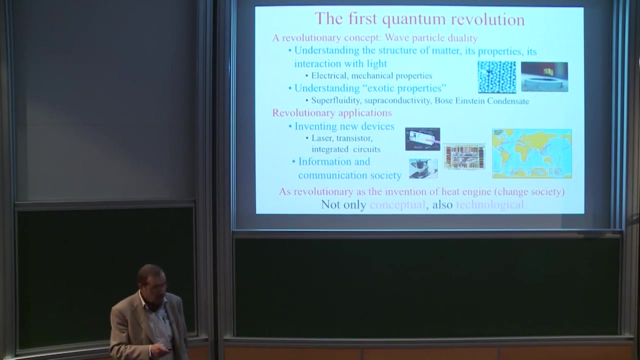 Information and communication society. and, of course, no need to emphasize that it is as revolutionary, for instance, as the invention of the heat engine. it has totally changed the society. So it was first conceptual and then technological, and it changed the society. 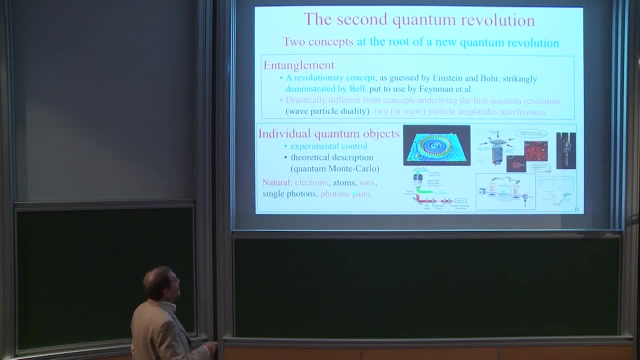 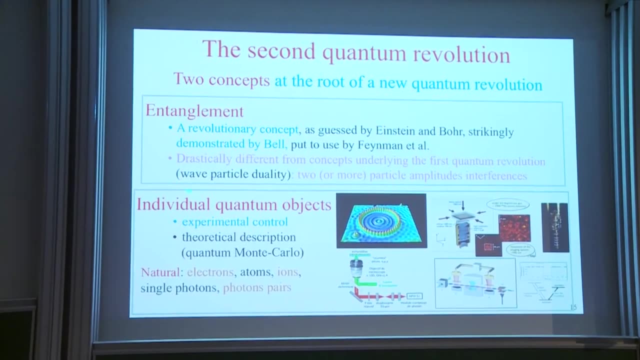 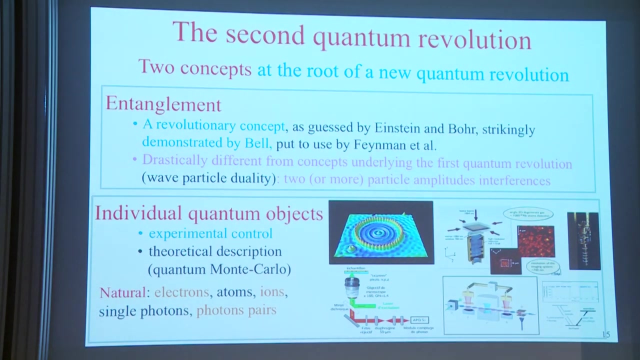 And the second quantum revolution. I will focus on that today. I will focus on the fact that there is entanglement. Entanglement, which is really a very strange property. And there is another thing, which will be implicit, but I like to emphasize it. 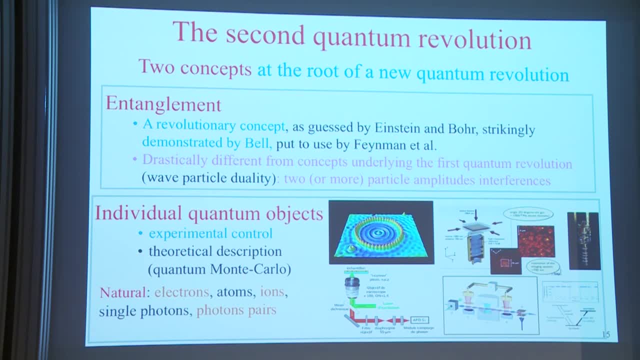 A major ingredient of the second quantum revolution is the fact that, starting in the 1970s, physicists, experimentalists, have learned to control, observe, manipulate, single microscopic, single quantum objects. You have to know that in the 50s, people as smart as Schrödinger wrote strong sentences. 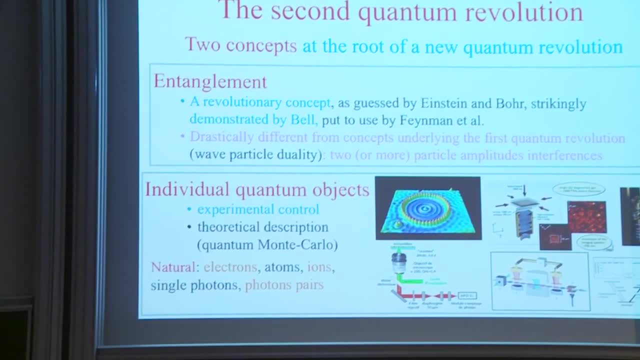 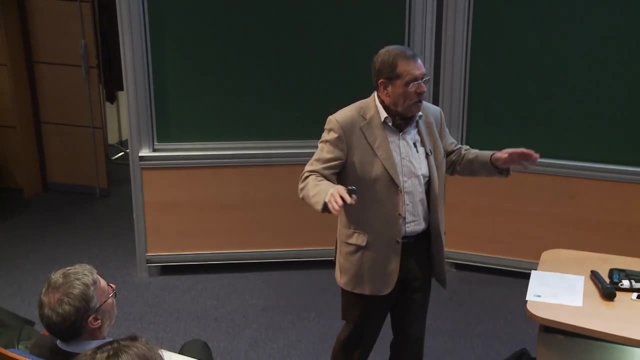 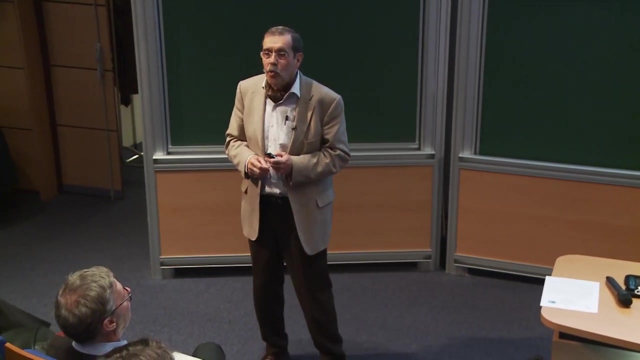 saying: 1. It is clear that quantum mechanics is only to describe large ensembles of microscopic objects. Schrödinger continues: 2. As soon as we pretend to describe a single quantum object, we are led to ridiculous consequences. 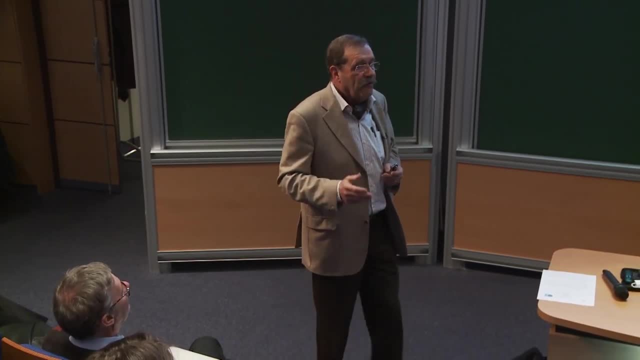 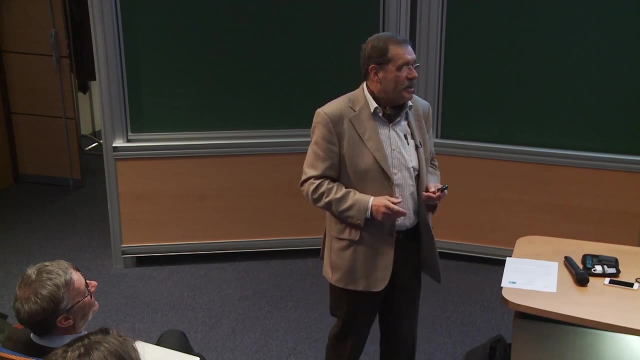 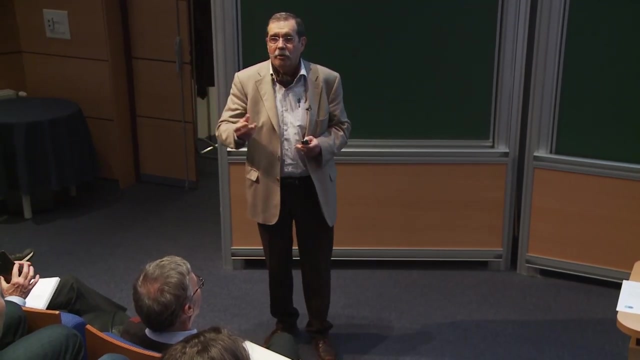 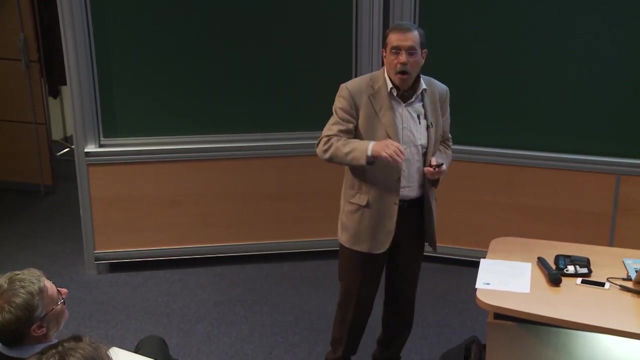 And claiming that is just as fantastic as if our colleague, a paleontologist, would tell us that he has an alive dinosaur in his lab. So there the feeling that quantum mechanics is only for large ensembles of microscopic objects, And then we can understand why, in contrast to Einstein, why most of the people were not. 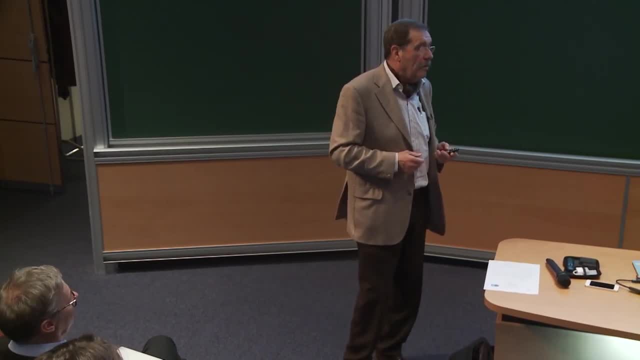 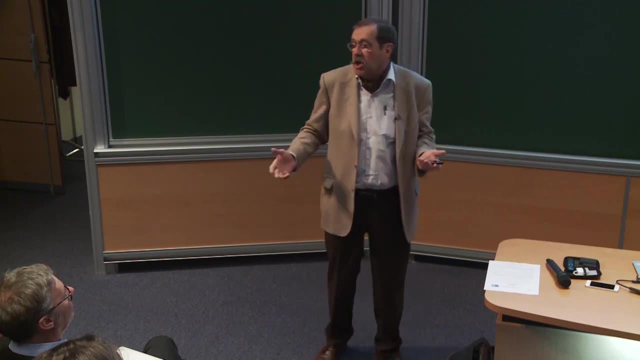 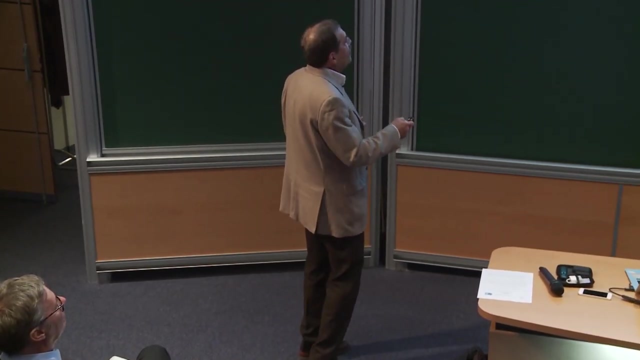 annoyed by the fact that quantum mechanics was making probabilistic prediction, Because if you have a large ensemble of objects, the theory makes probabilistic prediction, Of course there is no problem to accept it. So the fact that, starting in the 1970s, the physicists showed in the laboratory that they 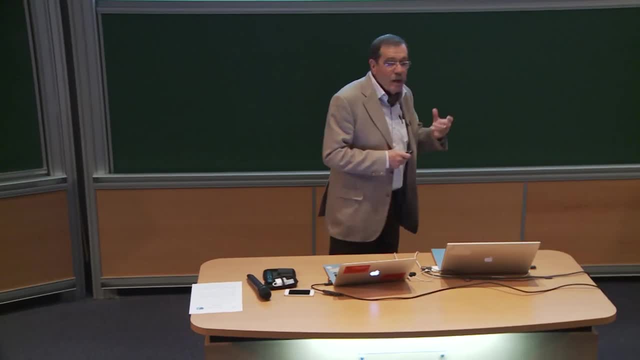 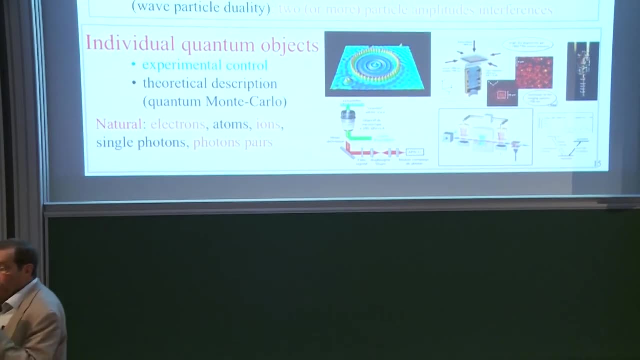 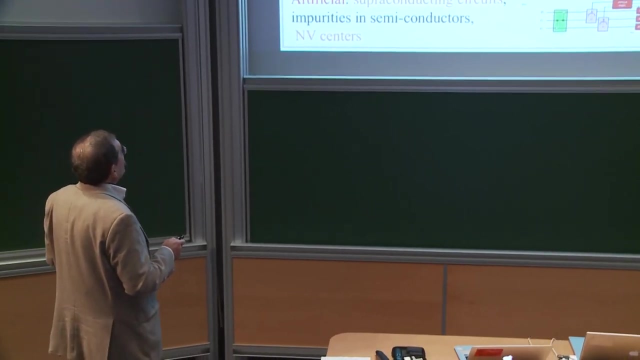 can observe and manipulate single quantum objects really totally changed the situation, in particular because there is an equation of observing entanglement: if you cannot isolate single pairs of entangled objects, Okay, So yes. Well, the point that I want to make here is that 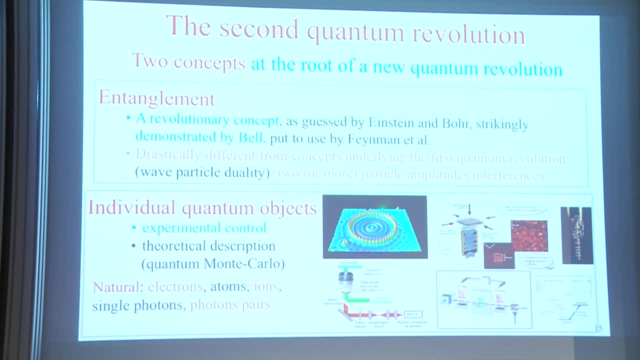 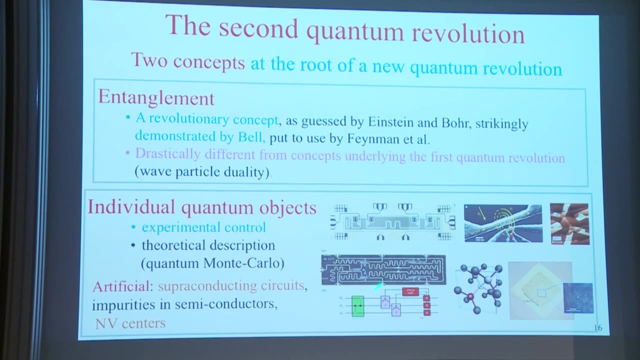 Let's say, for example, a single quantum object is the basis of a tree, which is the basis of a tree's natural existence, the basis of an object. So a single quantum object in a tree is the basis of an object and which there is. 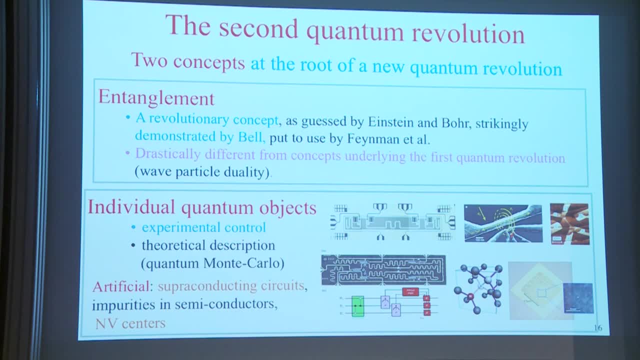 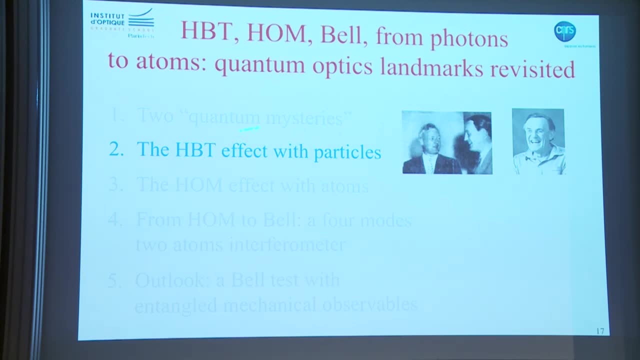 nothing in the tree. A single quantum object is in fact a natural object. So the nature of the tree is not a tree, it is a thing. The idea is the nature of this tree, The evenness of the tree, The whole tree. 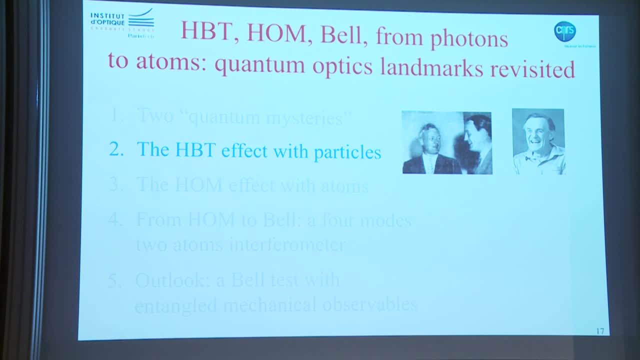 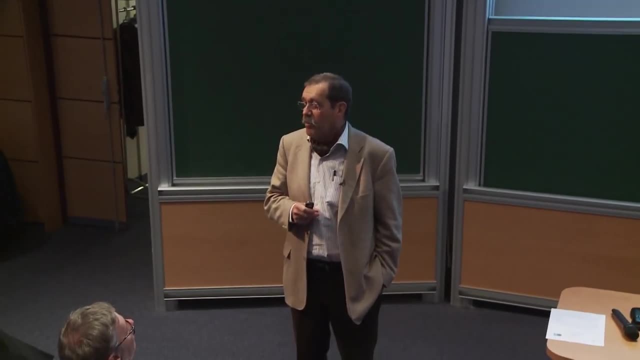 Brown. if you look on the Google image, you have dozens of images of Hanbury Brown. If you look for Mr Twist, you will find no image because in fact he became a member of the intelligence service or some secret service, and people in secret service do not. 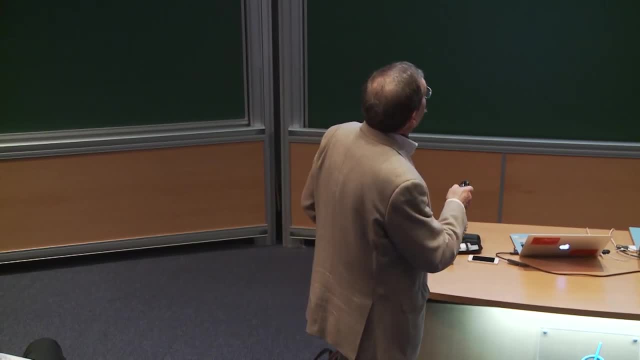 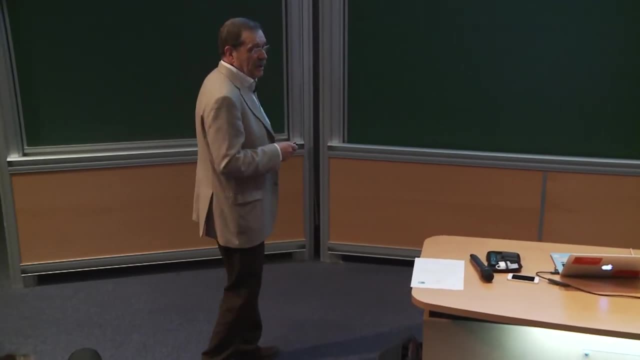 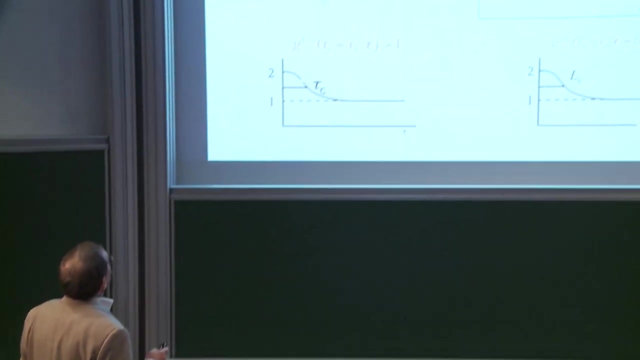 publish their photo. But somebody privately gave me this photo of Hanbury Brown and Twist, So it's a personal photo. it's not on the web, unless if people copy my transparencies and put it on the web. So this is the famous Hanbury Brown and Twist effect that it was published in 1956. 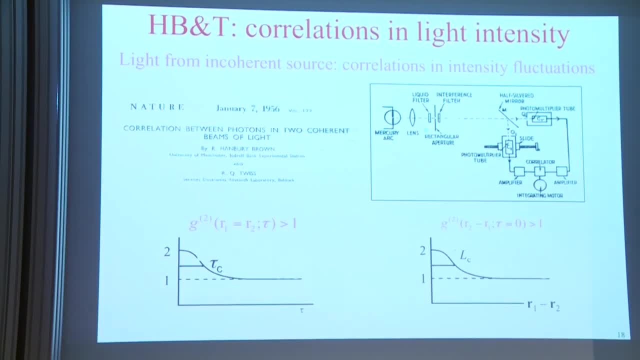 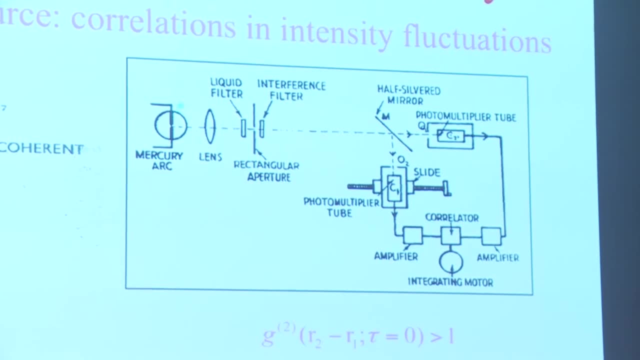 The experiment is the following: You have a lamp, a classical lamp. Laser was invented in 1960 only, so it's a classical lamp. there is no doubt. There is a filter to select more or less monochromatic light. a single line in a mercury lamp. 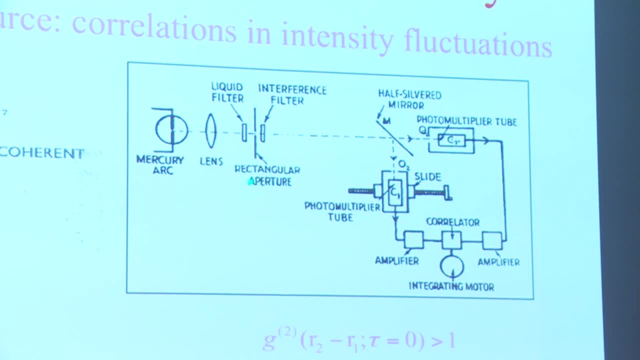 And you put it on a small object, There is a hole or rectangular aperture, so filters to isolate a single line. And then this light beam is analyzed with two photomultipliers. It's after World War II and during World War II they have developed this technology. 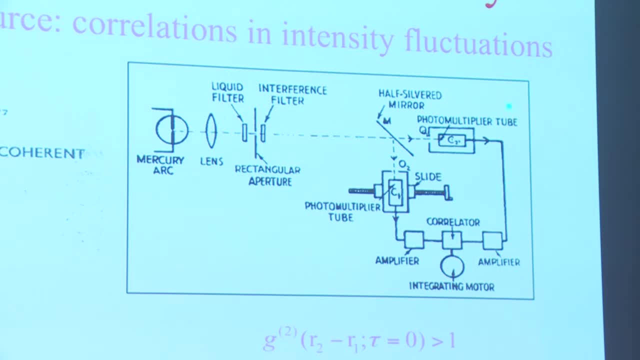 like photomultipliers, et cetera. So you have two photomultipliers, which are very sensitive photodetectors, And there is a beam splitter here. And you know what is a beam splitter? okay, It splits a beam in two. 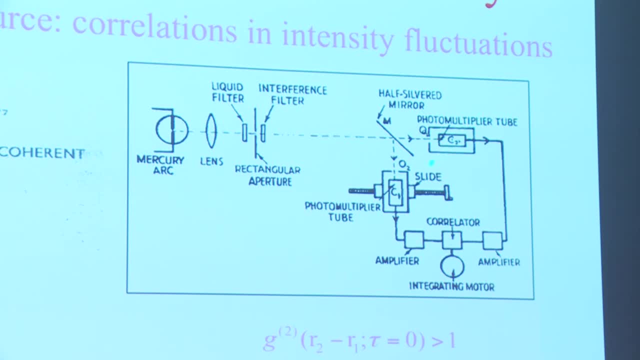 And they look at the correlation between the photocurrents. And nowadays, well, people laugh when you see that because nowadays you have electronic circuits and you just look at the correlation At that time. to make the correlation you need to have a multiplying system. okay. 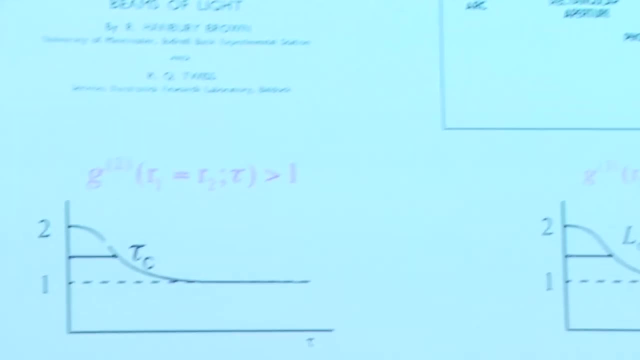 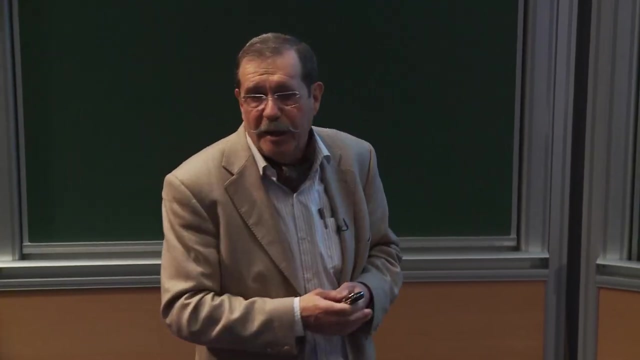 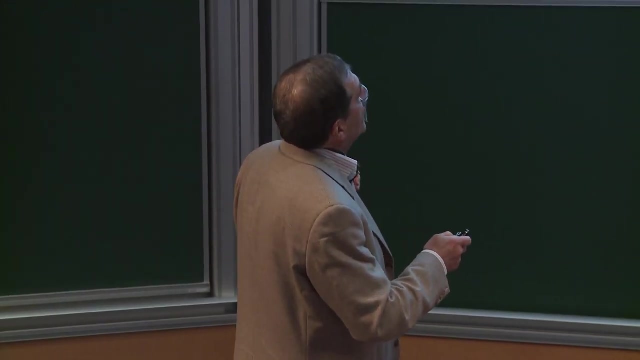 And it's just mechanical with a motor. okay, You have a current coming on one side, a current coming on the other side and the rotation of the motor is proportional to the integral. It's really amusing. And the correlation of course. what is it? 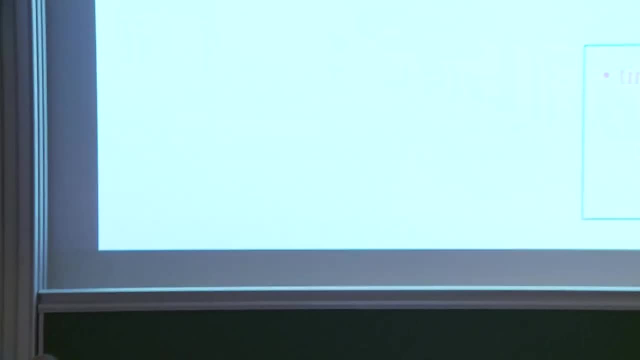 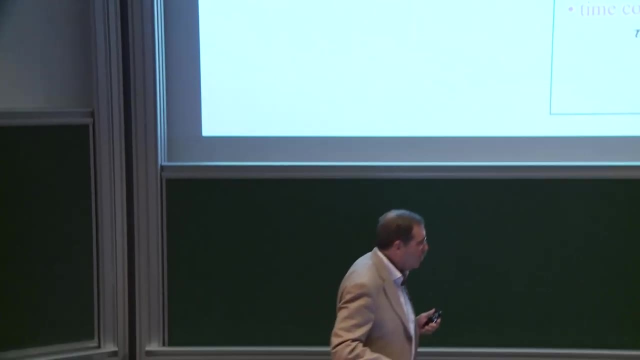 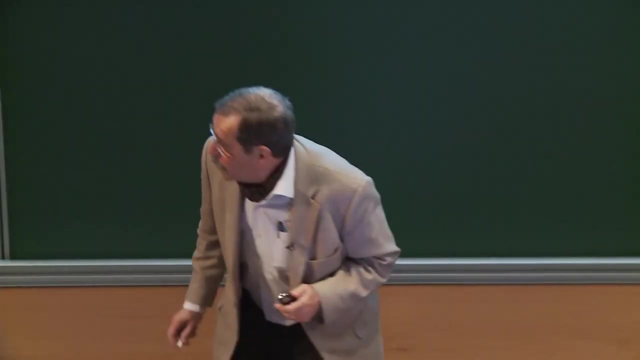 The correlation should be written somewhere. It's not written, Okay, So I will write. I will do like a mathematician, I will write what is a correlation, piece of chalk somewhere, Voila Merci. So the correlation, the current correlation, is nothing else that. 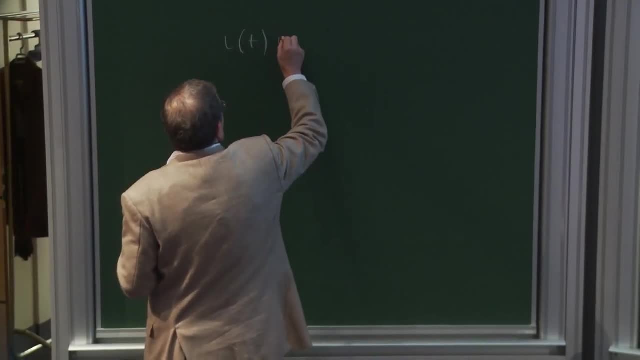 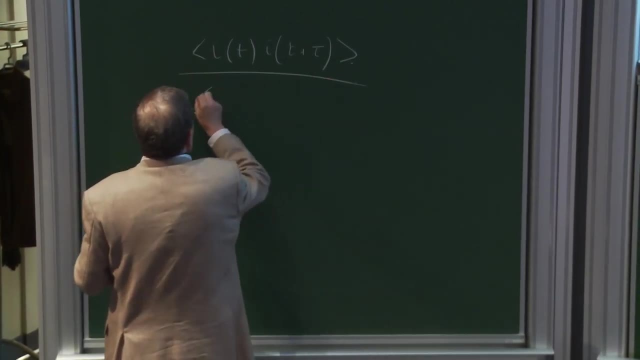 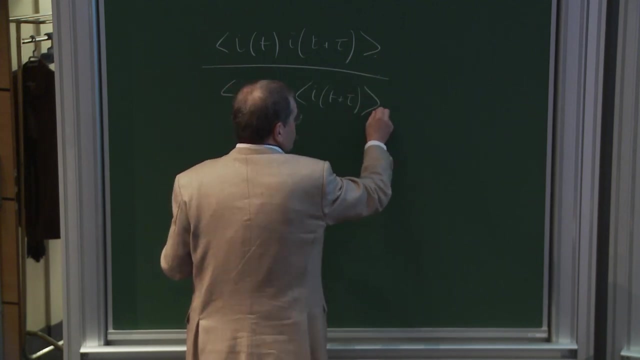 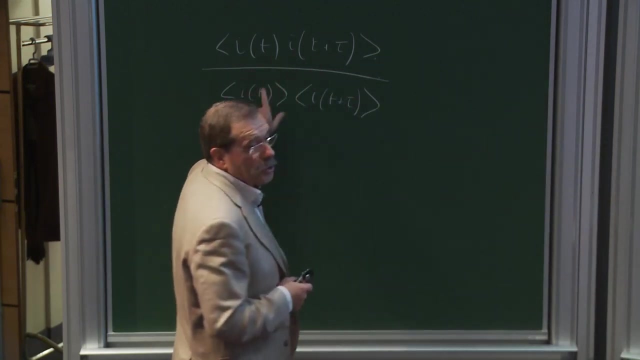 Okay, Okay, So the average of the product of the photocurrents with a certain delay divided by the product of the averages. okay, So this is a correlation function. It means that if there is no correlation, the average of the product is equal to the. 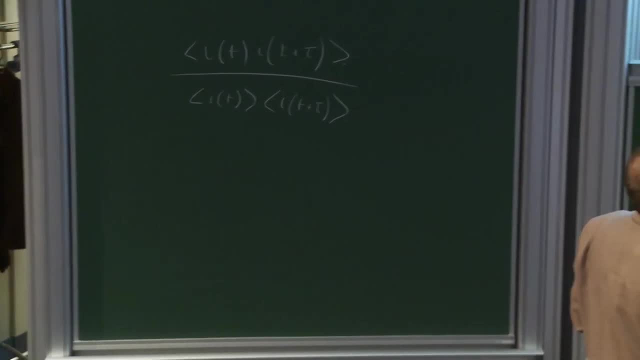 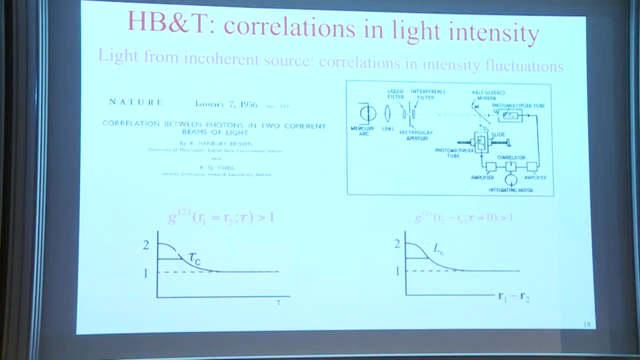 product average and g is equal to 1.. And when they measure it, okay, What happens? What they find is that. oh well, what I should say. I am too fast. Is it I1 and I2, or it's I and I? 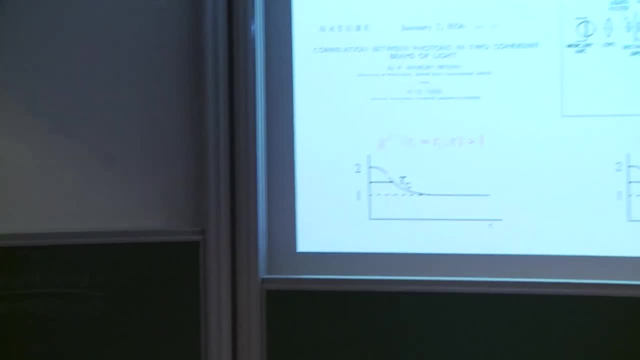 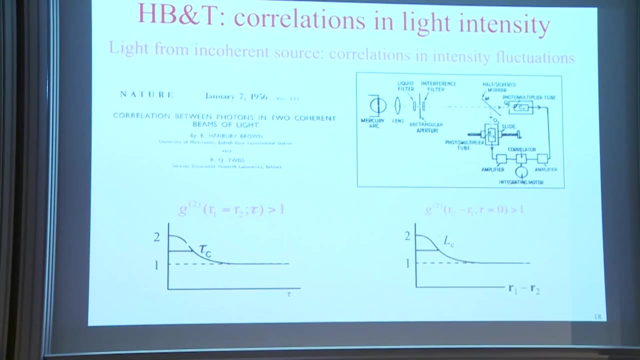 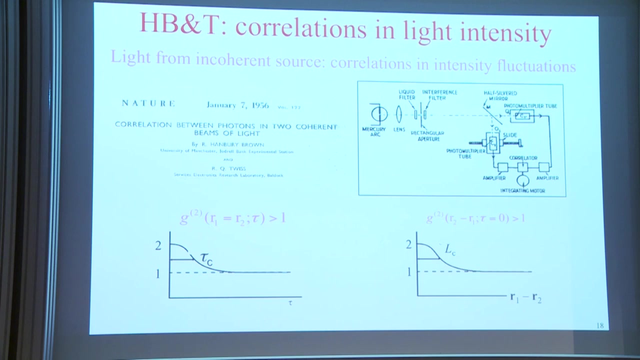 Excellent question, Both It's and that I missed. that's it. It's I1 and I2, but you can replace the problem. You can think that what you are doing is going in the image space. so you can think that. 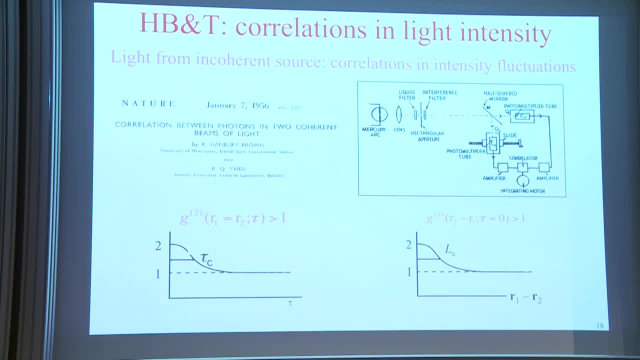 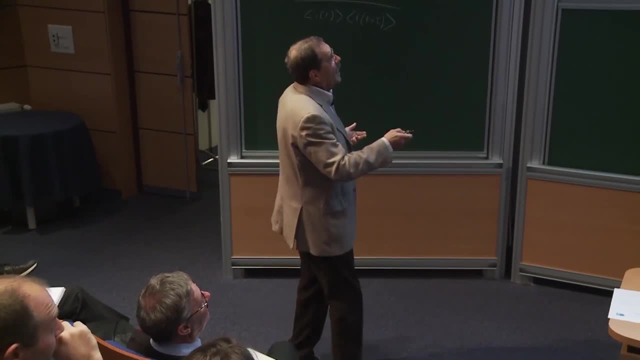 you have put this photomultiplier on the other side, Okay, And so you are in the same space. So it's a good question and the answer is both: Technically it's this and that, but when you are on the other side, okay, it's I of R1. 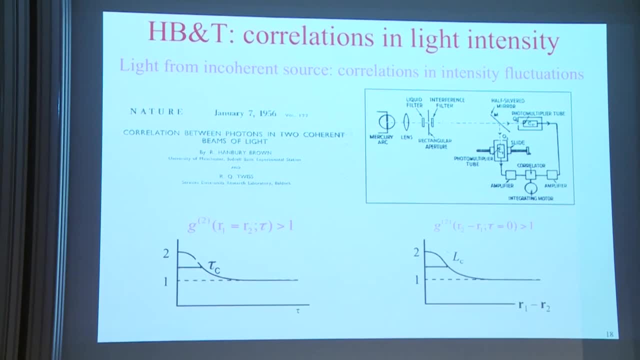 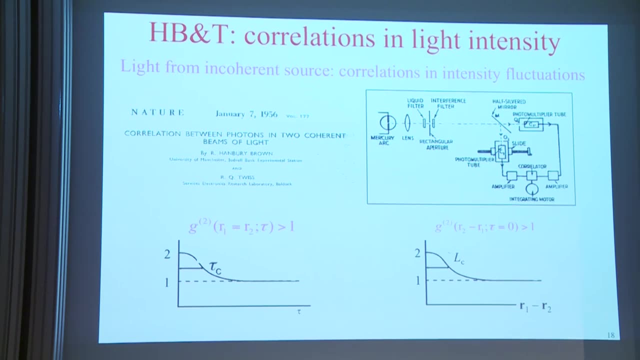 and I of R2, okay, which are in the same space, Okay, And so conceptually you can think that you put these there. So what you find first. Let me- Okay, I am here. What you find first. 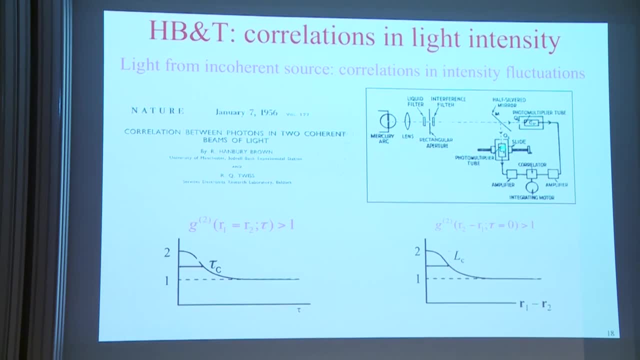 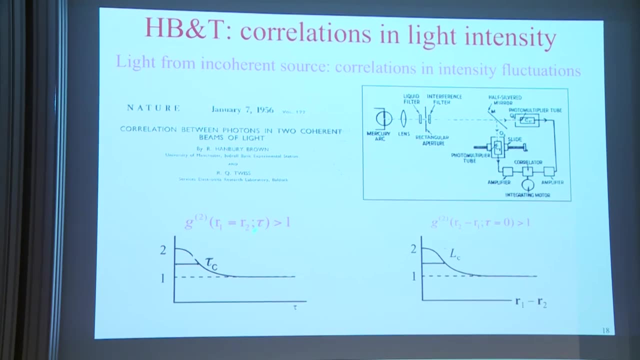 Okay, If you put the first photomultiplier exactly on top of the other one, exactly image of the other one, so R1 equal R2, and you look at the correlation versus the delay. When the delay is null, the correlation is two, which means that the two photocurrents 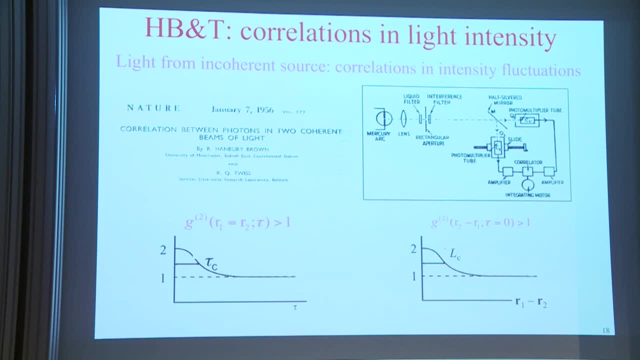 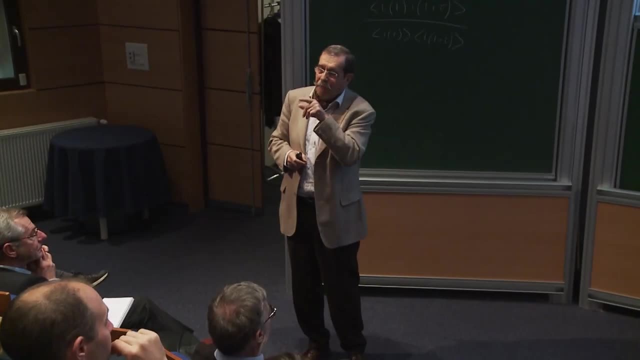 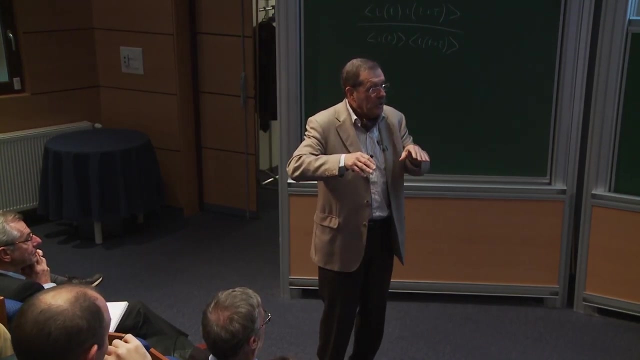 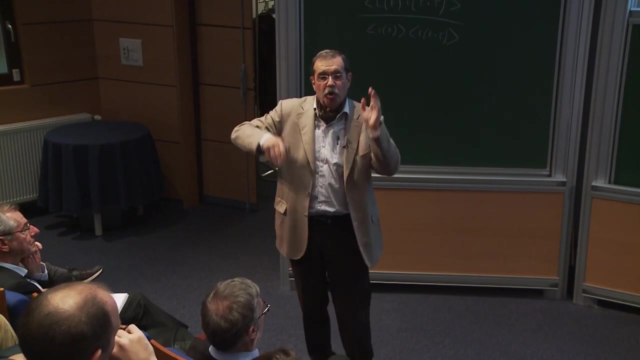 are. There is a correlation. Are correlated- Okay, The fluctuations are correlated. This is not obvious. Okay, Because if the fluctuations were due to each detector individually, there would be no correlation. It means that what they measure is correlation in light at the end of the day, and not correlation. 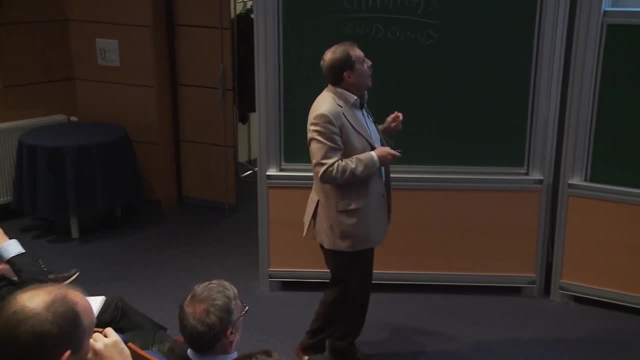 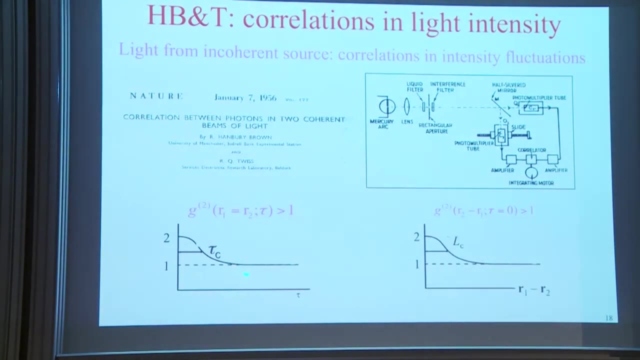 due to noise in the photomultiplier. Okay, But And when they separate the two images of the two photomultiplier, then it drops to one. Here there is no correlation. No, sorry, When they change the delay. 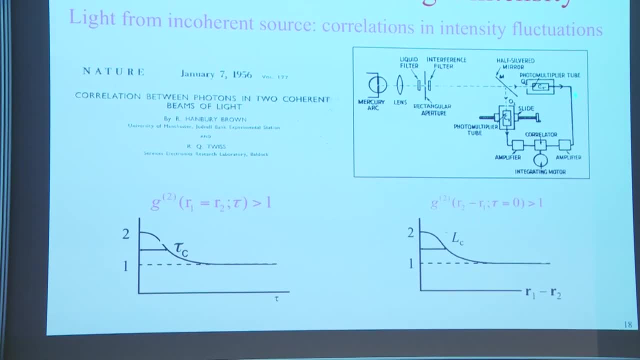 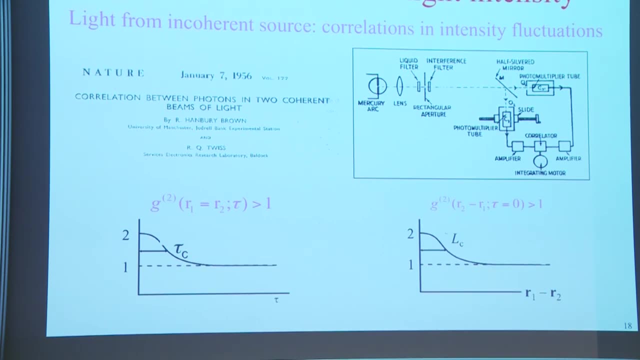 Okay When they change the delay. and to change the delay you just add meters and meters of cable. One meter of cable is five nanosecond. One meter of cable is five nanosecond, So you can change the delay by adding meters and meters of cable. 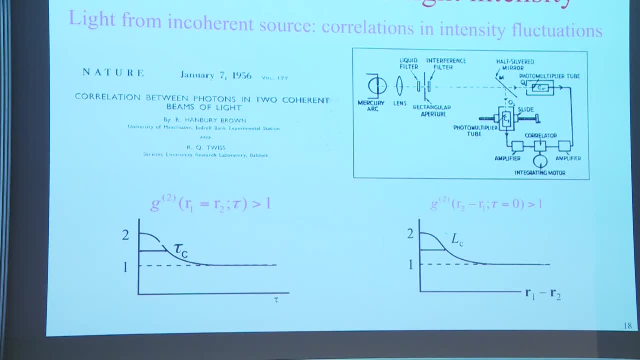 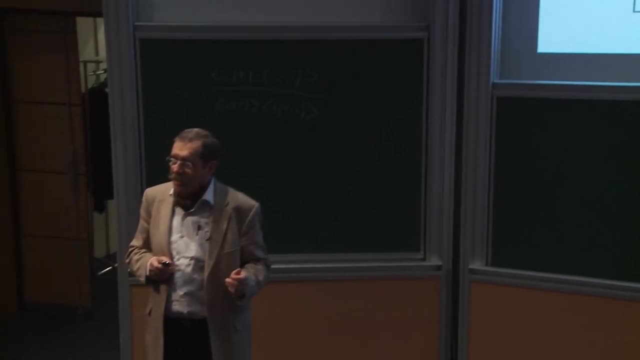 I was doing that during my thesis And if we were writing the formula, I would be quadratic in the photon operator in A. Yes, exactly So it's square, Square times square. It's a quasi-correlation. Yes, We'll see that in a while. 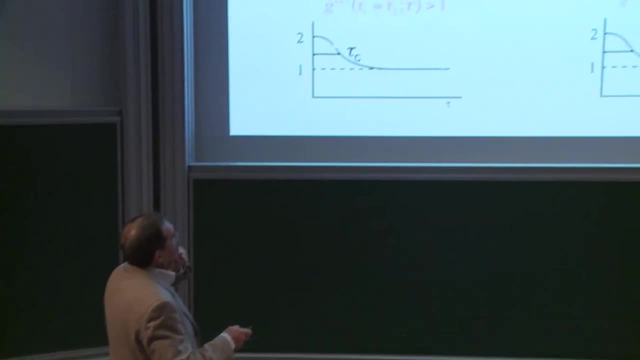 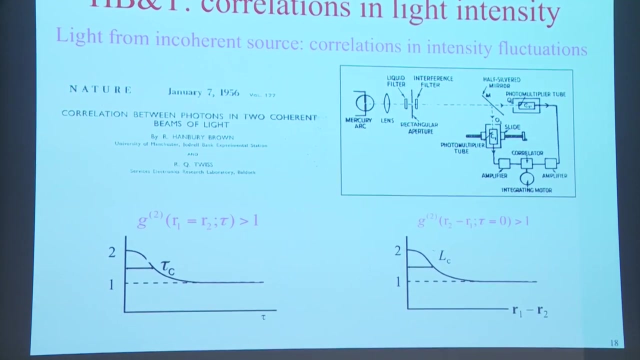 Now if, rather than changing the time, they work at delay, which is null, and so, of course, when this is the same as this one, now they separate the two photomultiplier and it drops from two to one, and there is a characteristic distance here, just like there is a characteristic. 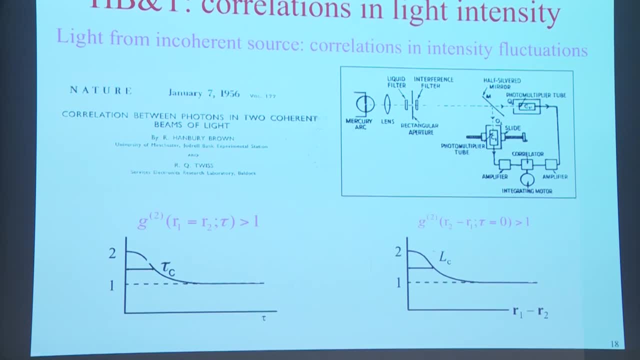 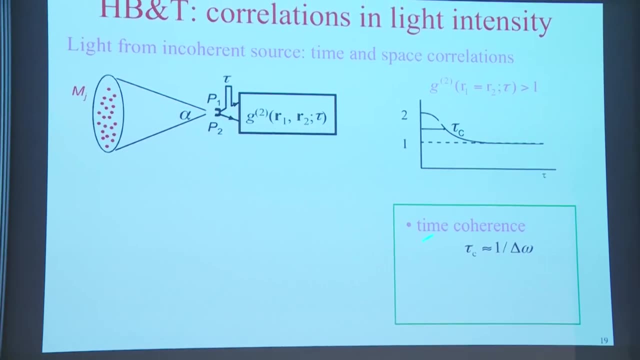 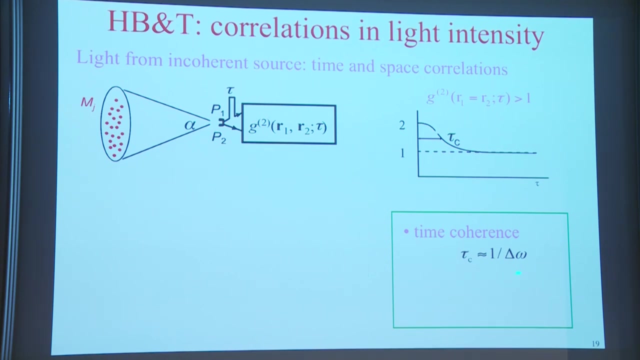 time here. We call it the correlation time and we call it the coherence length or the correlation length. Okay, Good, What they find is that this time, this correlation time is nothing. that's what we call, in optics, the time coherence, which is just the reciprocal of the bandwidth of the line. 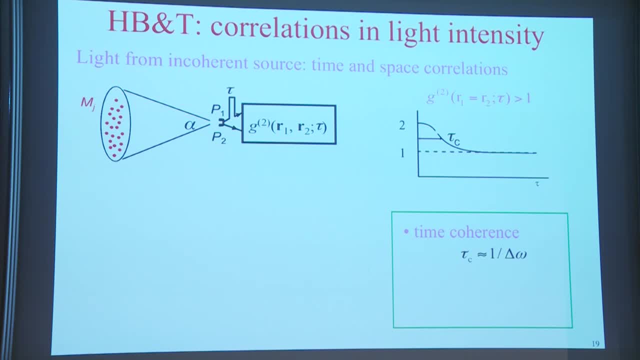 Okay, So a typical line will be one gigahertz, so it is one nanosecond, something like that. Okay, And then here, and this is an important thing for them, the coherence length is what is called the spatial coherence, and the spatial coherence is nothing else than the wavelength. 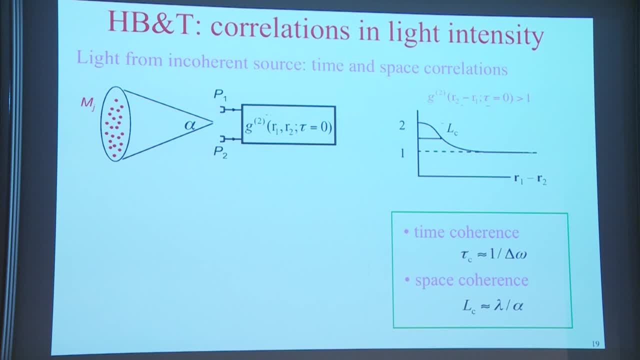 divided by the angular diameter that you have here. And this is the reason why they were doing the experiment, because by measuring this coherence length, they could determine the angular diameter, Okay, The angular diameter of stars. This was the goal of their experiment. 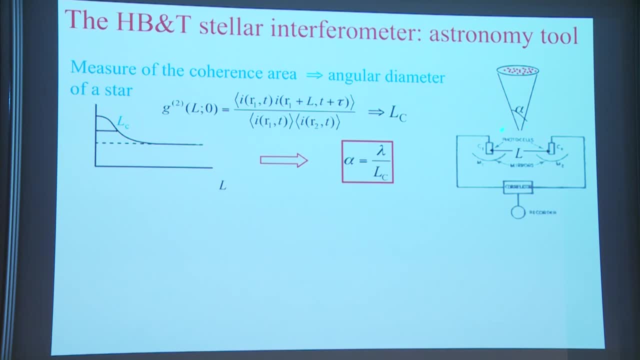 I will show you that. Okay, So the idea was the following: Okay, You have two detectors. When the detectors are close, you watch a star. When the detectors are close to each other, there is a factor of two and at a certain 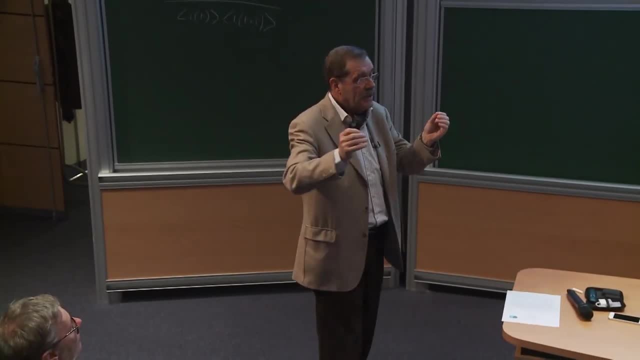 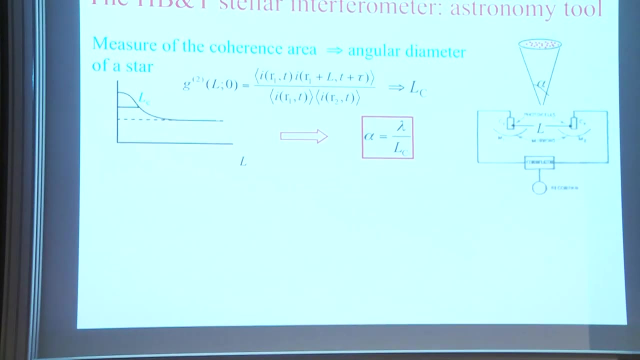 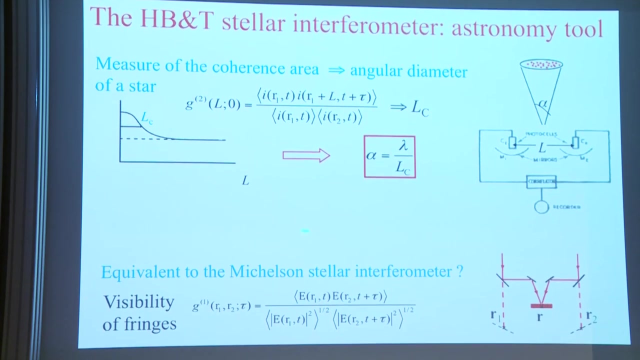 distance it drops to one. This gives you the coherence length, LC, and from LC you can determine the angular diameter of a star. And you know that measuring the angular diameter of a star is very difficult. It's very difficult for the following reason: 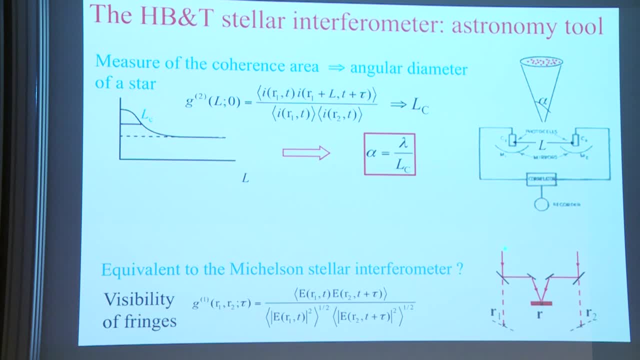 There was a system used by Mr Michelson which is an interferometer in which you just look at ordinary interference between the light coming from the same star on two points And what you observe here is fringes And the calculation which is well known. 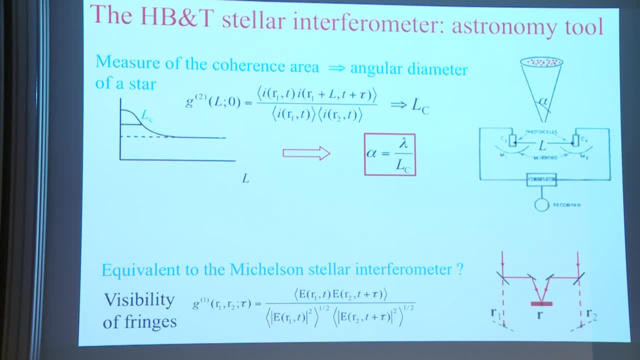 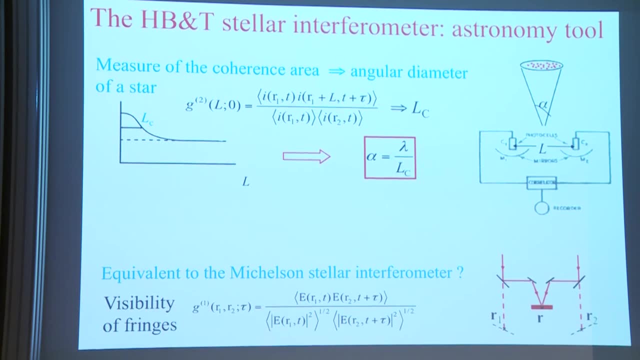 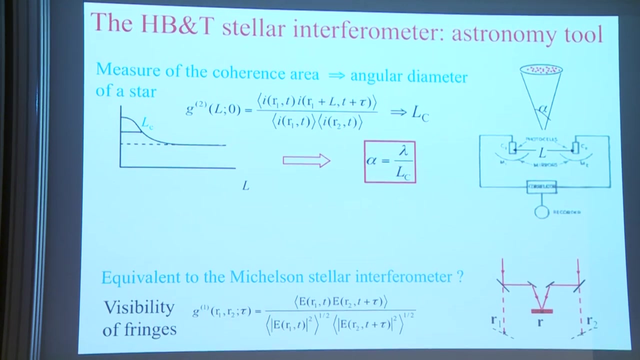 In optics tells you that again. what happens is that when you increase the distance, the visibility, the contrast of the fringes will decay And the typical size will be again LC, the length of coherence. Okay, And so just by observing how the visibility of the fringes decay, you can measure the 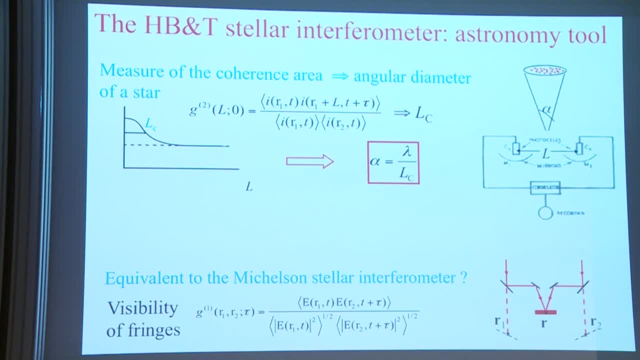 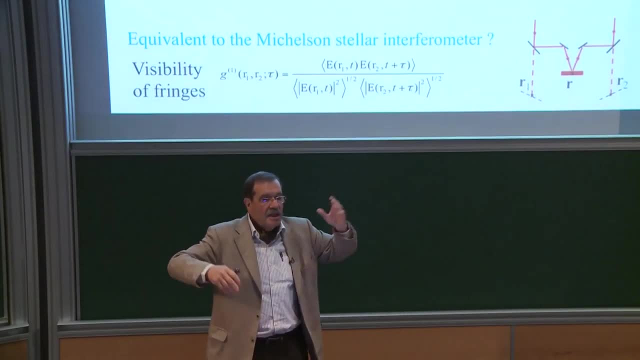 angular diameter of a star. But there is a problem, and you have all heard of this problem: It is the fluctuation, Okay, The fluctuation of the atmosphere, And because of this fluctuation of the atmosphere, there is a difference in the path here and 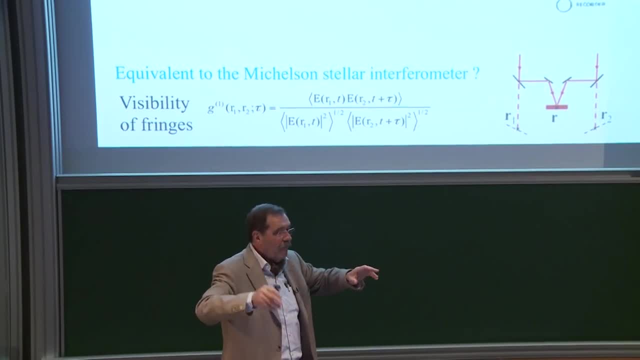 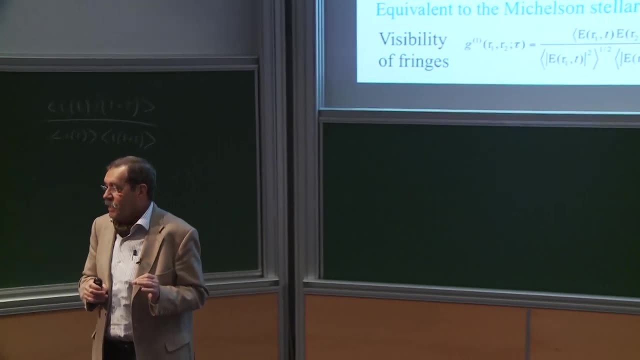 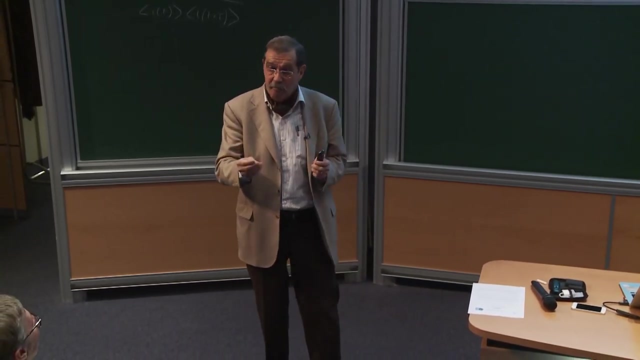 a path there And there is fluctuation in the relative phase, which means that the fringes move like crazy. Michelson was a fantastic experimentalist. This is a true story. He was able to observe the fringes and although they move very fast, he can say, hmm, good. 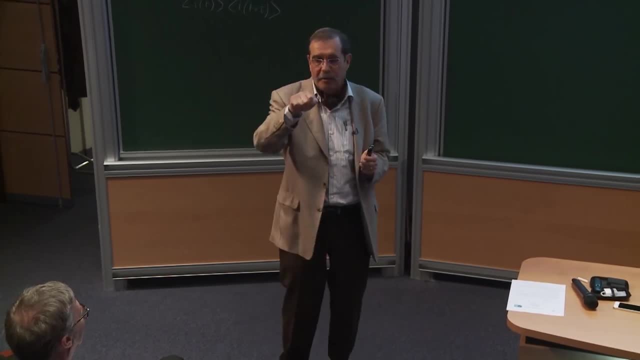 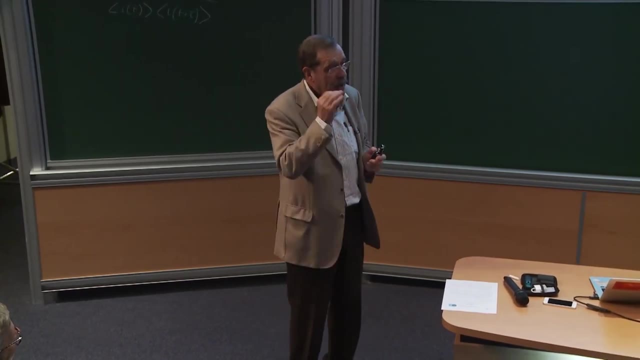 visibility. Let us decide it's 90%. They would put a point 90%, Then he would increase the distance between the two detectors and he'd say, hmm, 50%. And he really made measurements of angular diameter of stars with that. 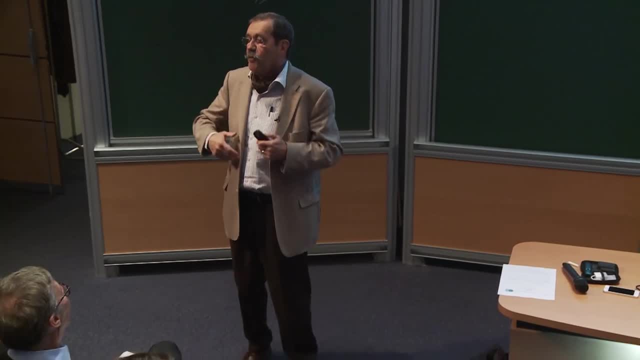 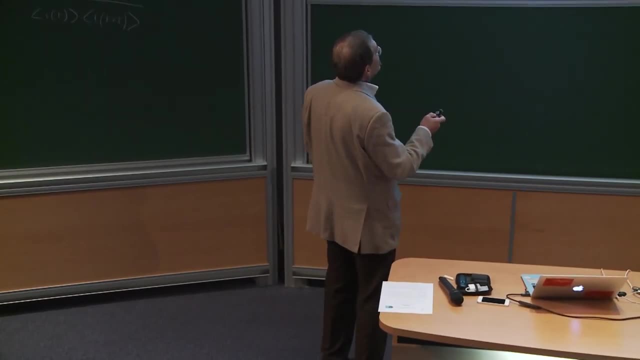 But honestly, it was not very convenient And, of course, in modern time, we want to have objective measurements. Okay, And this is why Ambrey Brown and Twist and then did this method, which is different, because this method is insensitive. 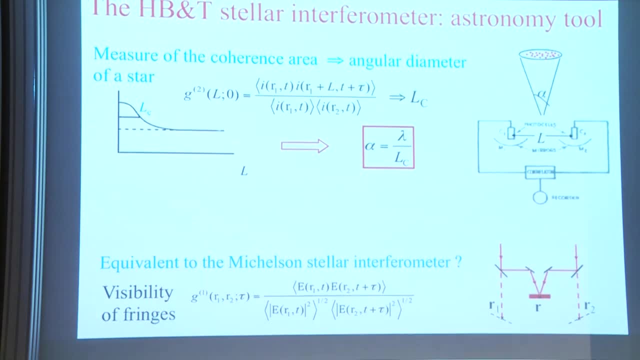 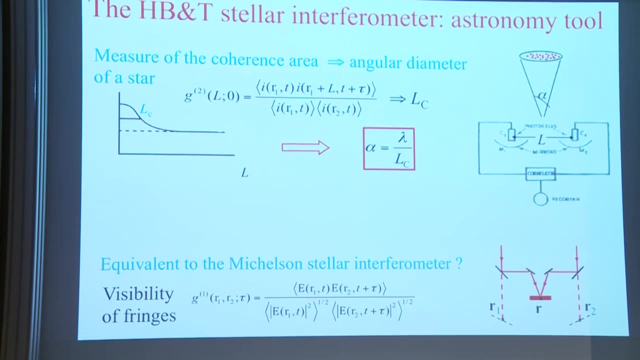 Okay, Insensitive to the atmospheric fluctuation. I have not planned to explain it, but if you ask me the question, but after I finish my explanations, if you ask me the question, I will tell you why it is insensitive to atmospheric fluctuation. 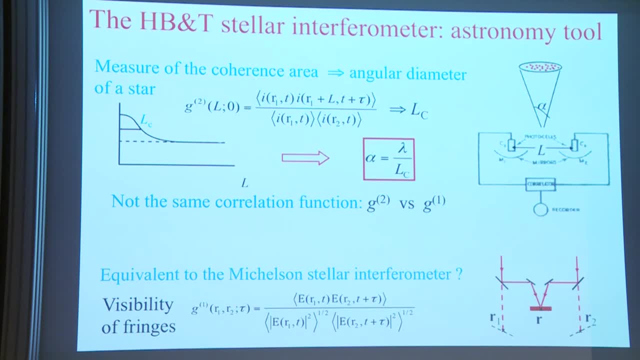 But this was the goal. Michelson is the same as a- Absolutely That's a great Michelson, American physicist of the end of the 19th century. Okay, And we can note that He's not the same thing which is measured. 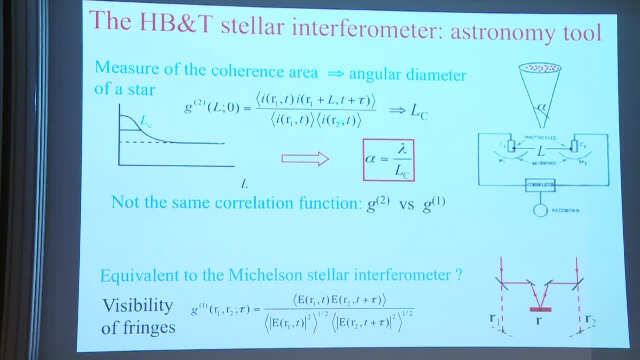 Now, Thibault, you are going to be happy. In fact, what we are measuring here is what is called G2, which is second order in intensity, And intensity is a square of the electric field. Okay, And so here we measure a fourth order correlation function for the field, while here, with Michelson, 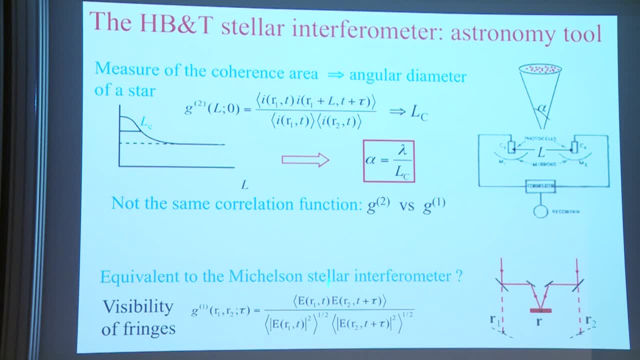 we measure a second order correlation for the field. So obviously it's not the same. It's not the same correlation function which is measured, But- and so I'm very blind to this- This is insensitive to atmospheric fluctuation. 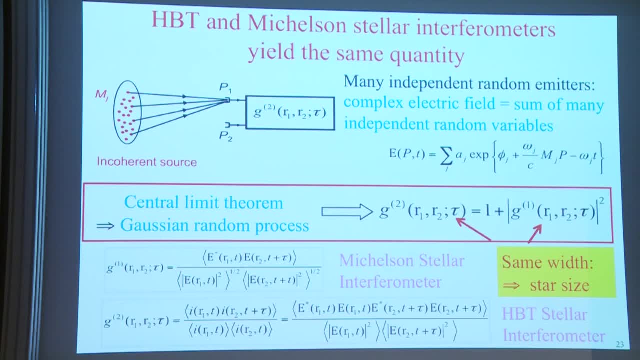 But although it's different function, in fact they are strongly related for a reason which is a mathematical reason. Well, mathematical from my point of view, probably for you is not. The idea is the following. Let us describe the light arriving here. 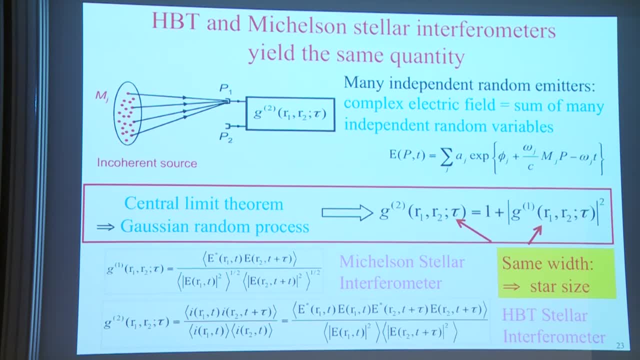 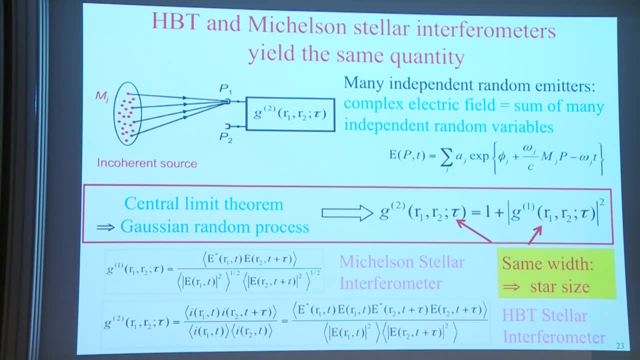 So I can only think of classical waves. In fact, I have an incoherent source, which means many independent emitters, So the wave that I receive here is a sum of many contribution, which is a sum of waves with phases that I take as uncorrelated, random variables. 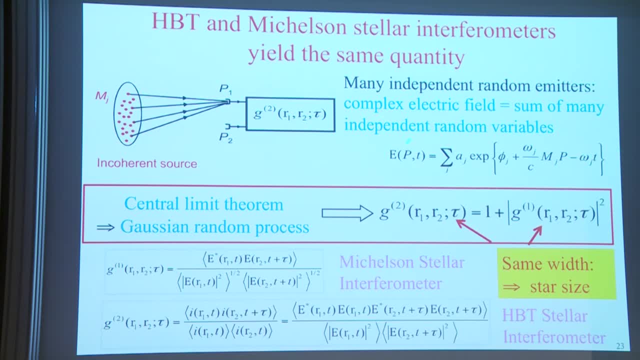 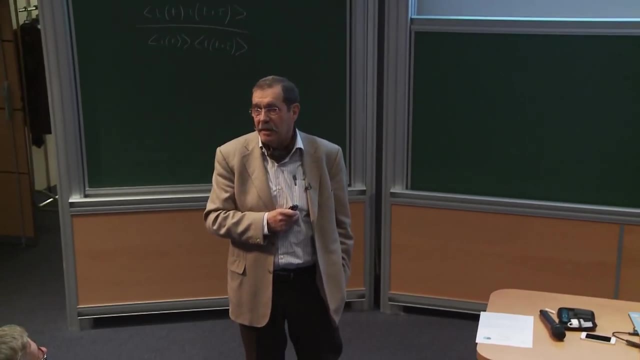 a given time and a given point, is a sum of independent random variables with the same statistical properties, and we know that. then we can apply the central limit theorem, which tells us that we have a Gaussian statistics. and when we have a Gaussian statistics, we have the Vick theorem, which allows us to express a. 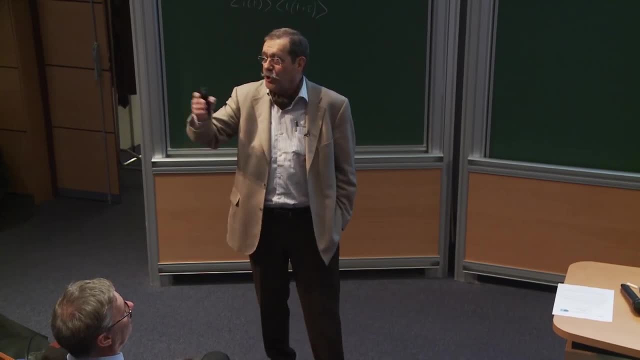 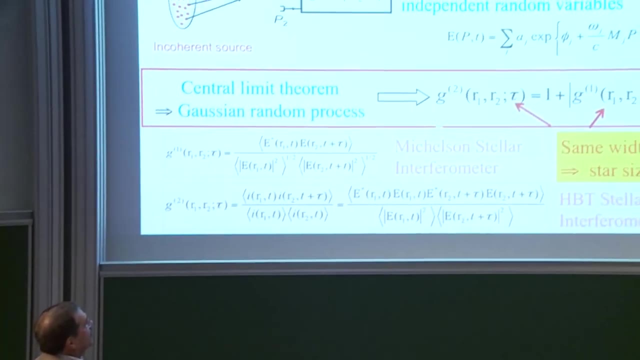 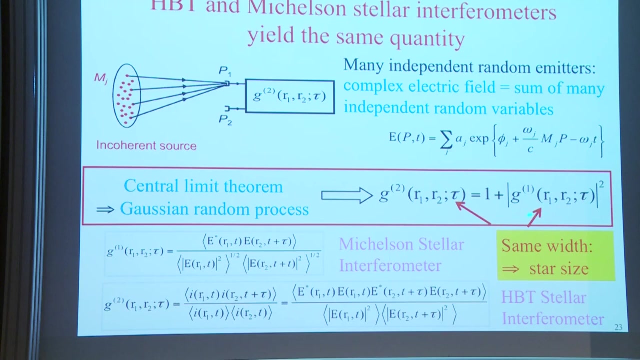 fourth order, correlation function as a function of a second order and at the end of the day we have this formula: the correlation function measured by Ambrose Browne twist is equal to 1 plus the square of the correlation function measured by Michelson. so within a factor root 2 or something like that, the 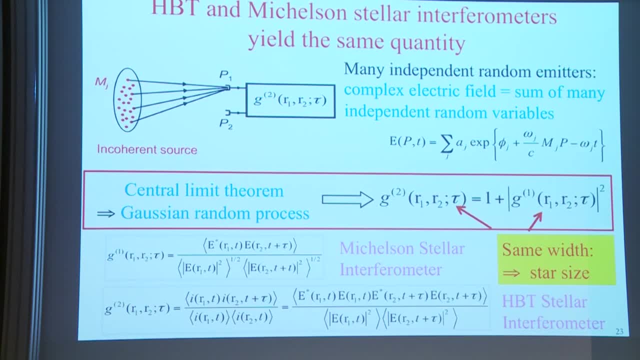 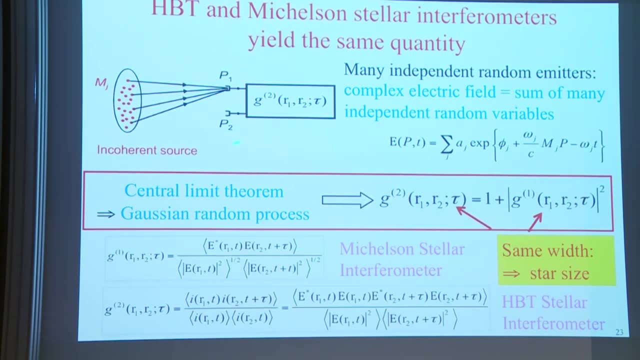 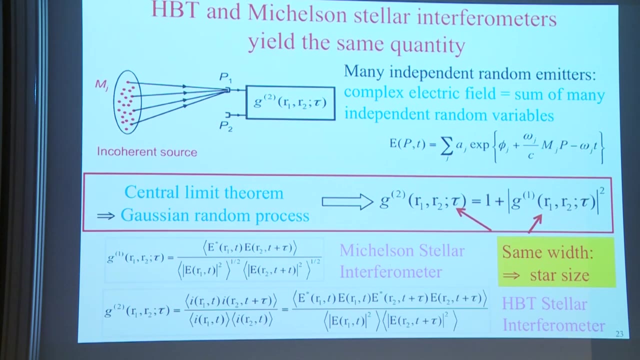 widths of this function is the same as the width of this function. maybe there is a factor of root 2, we don't care- and so this is a good understanding of our data, of what happens here, at least an understanding from a mathematical point of view. 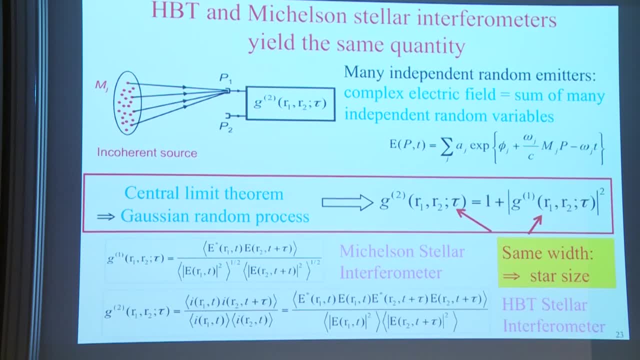 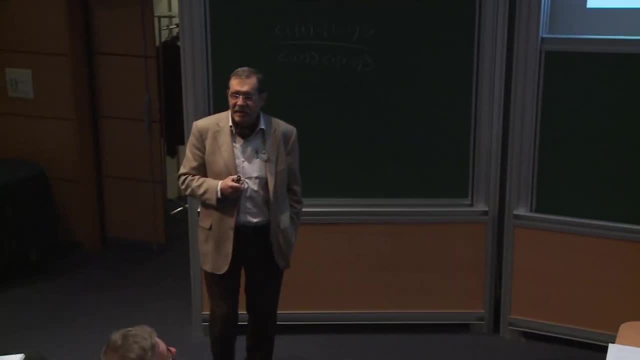 Where is the transferic noise in your formulas? Because you say it's both things in the same formula. Well, it's not in my formalism, but a hand-waving explanation. I could do a full calculation, but a hand-waving explanation. 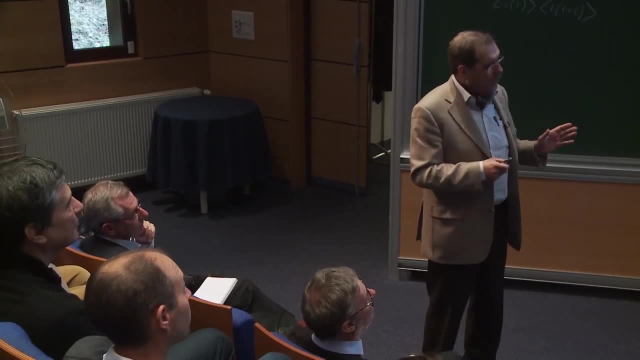 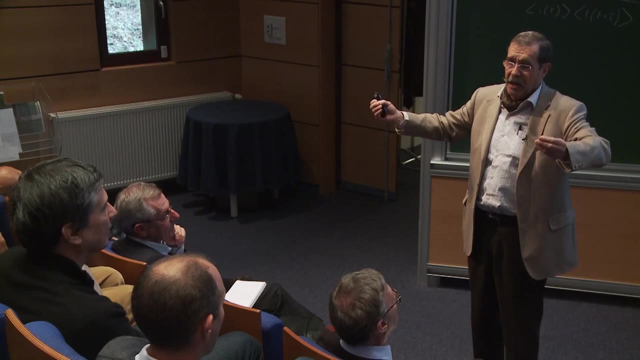 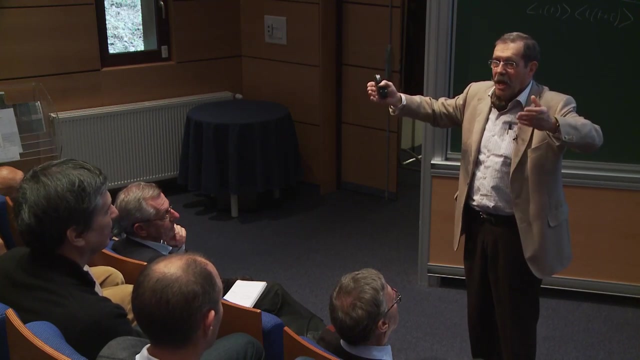 is the following: In the Michelson experiment, you look at an interference between something passing here and something passing there. I get extra, And so what is important is: what is the difference between the paths? And the fluctuation is of the order of a few micrometers. 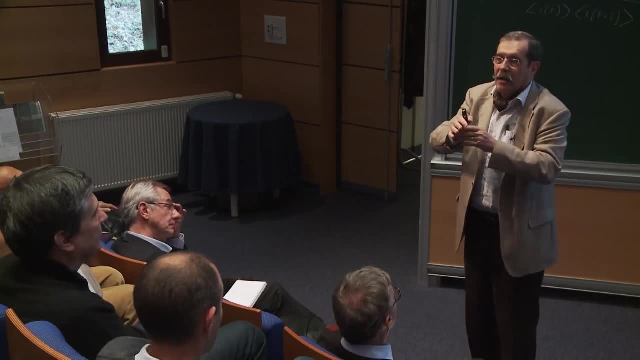 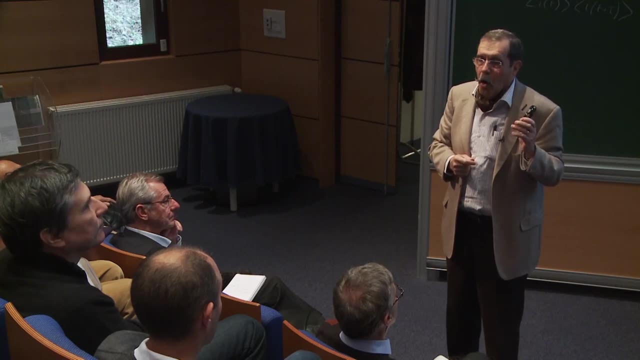 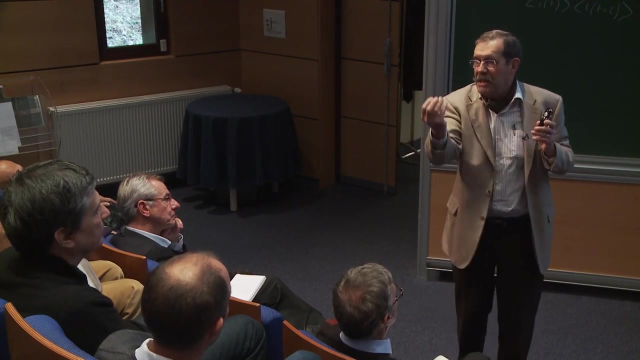 which is several wavelengths. This is why the fringes move. Now. the Ambry-Brown and Twizy effect at the end of the day amounts to looking at a bit note Here and a bit note there And compare the two bit notes. 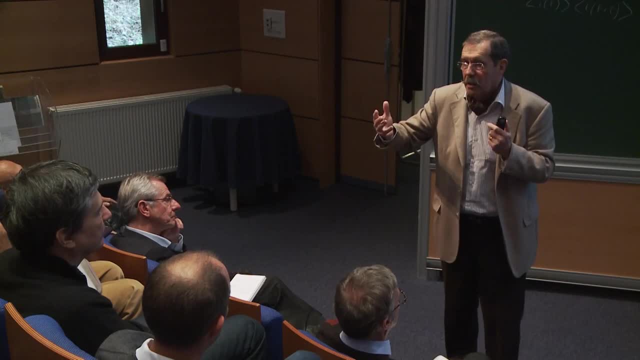 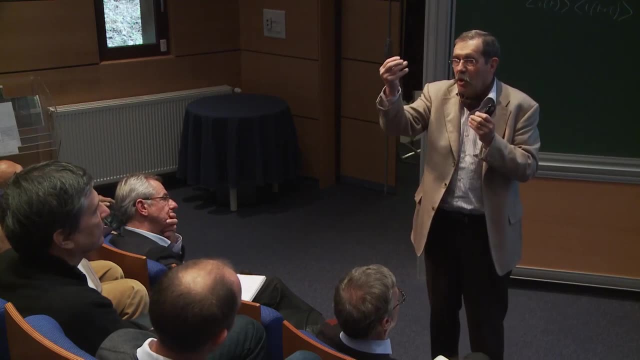 But the bit note will be in the gigahertz Because when you look at this fluctuation, it is in the gigahertz range. So in fact, you look at bit notes. The bit notes are in the gigahertz range. And in the gigahertz range the wavelength is of the order of several centimeters And the fluctuation of the atmosphere is very small compared to that scale. I can show you full calculation, But the real idea is what I explain to you. 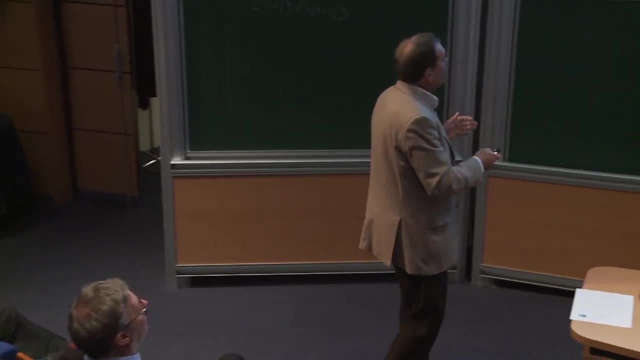 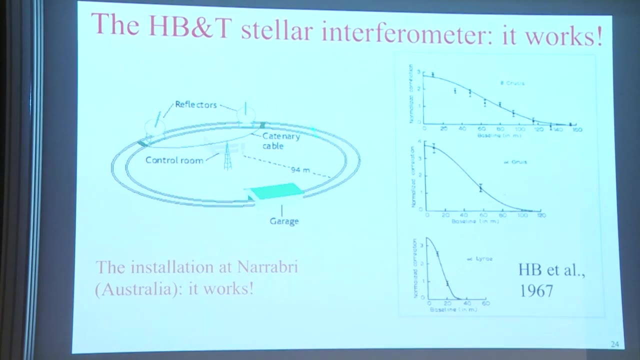 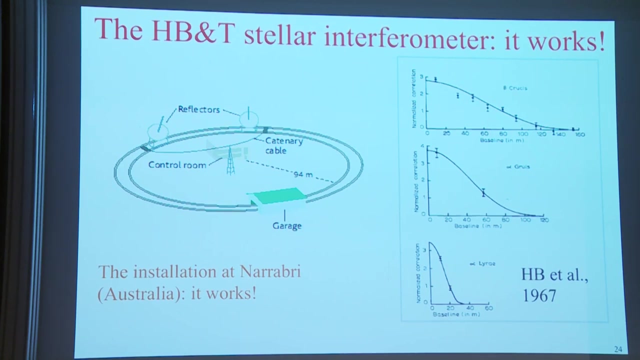 Okay, So let us continue, Because we have not yet entanglement and things like that. They moved to Australia- And I will tell you in a while why they moved to Australia- And they built an observatory. So you see, you have like a railway here. 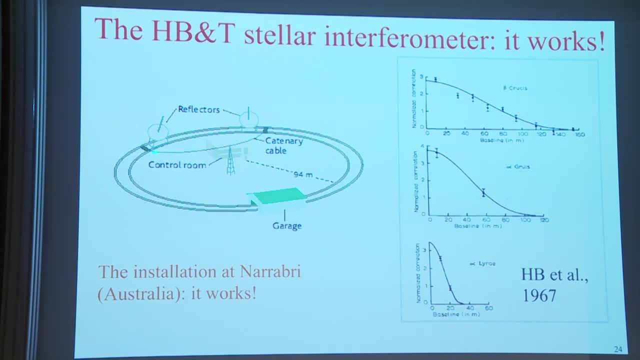 Diameter is 200 meters. So you have here one detector, another detector, And they look as a function of the distance And for instance, for this star of the Southern Cross, beta of the Southern Cross, they observe G2 decaying after 60 meters. And from this they get the angular diameter of the star. So it works Okay, So fine. Why annoy you with that? Because, after all, Hamburger and Bryant-Witt's correlations were predicted, observed and used to measure star angular diameter. 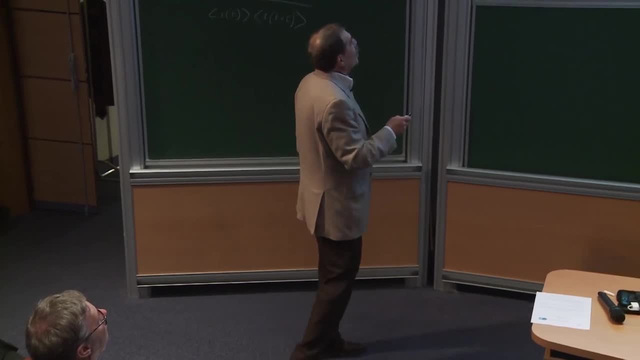 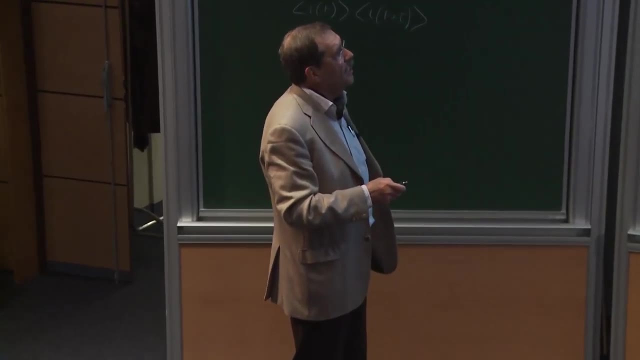 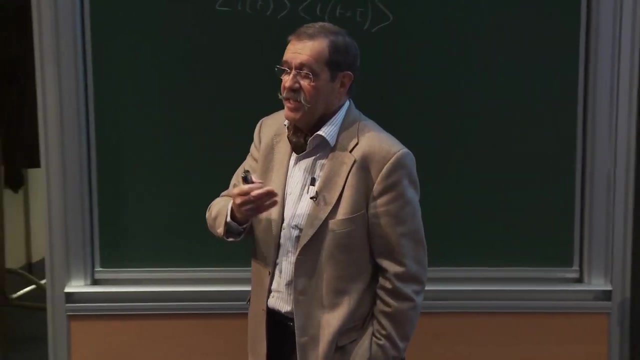 more than 50 years ago. Why bother? Because the equation of their interpretation provoked a debate that prompted the emergence of modern quantum optics, And the question was: can we describe it in a classical way? I have shown you that Yes, it's easy. 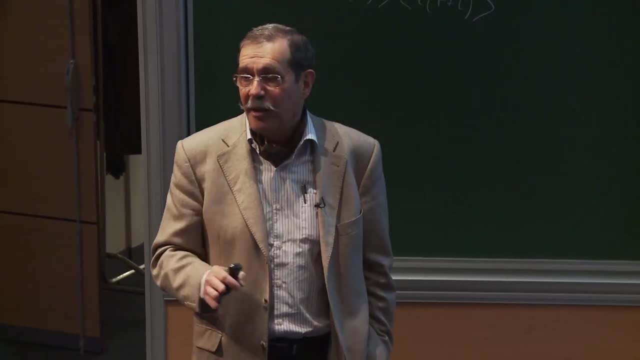 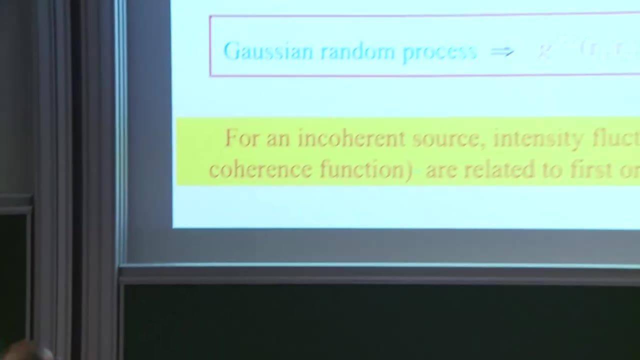 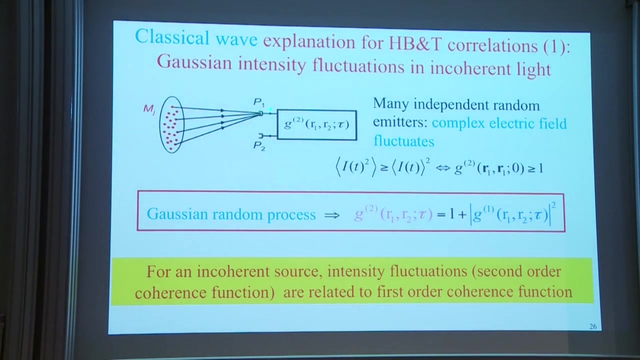 Can we describe it in a quantum way? And then it turns out to be very subtle. So let us come again to the classical interpretation. The classical interpretation amounts in a sense- if you look at the fluctuation here- it amounts to saying that the average of the square 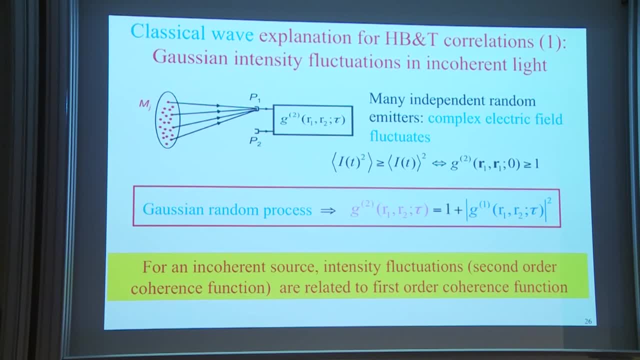 is bigger than the square of the average, And if we have a Gaussian process, there is exactly a factor of two in the ratio. This is characteristic of a Gaussian process. So this is what we have seen. OK, There is another image that I love. 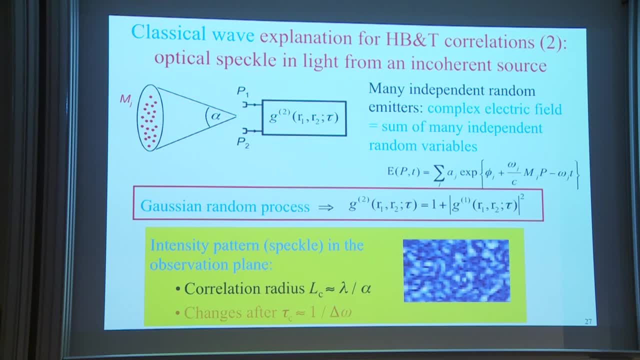 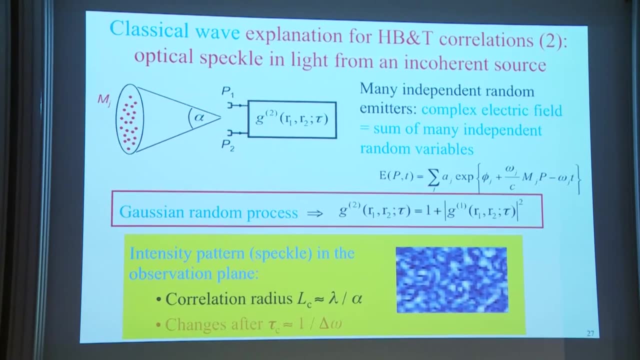 and I would like to show it to you. I forgot. You all know what is a laser speckle. No, Yes, No, you don't know. Ask anybody: a small piece of plastic, of anything through which I can pass my laser beam. 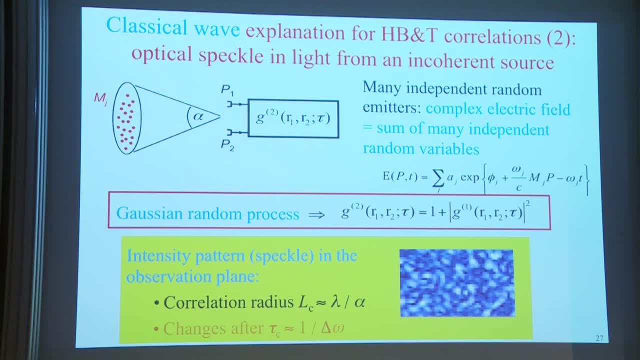 A piece, un petit morceau de plastique n'importe quoi. Oui, à peu près transparent, Même s'il est un peu diffusant, c'est pas grave. Oui, oui, quelque chose Parfait ça. merci. 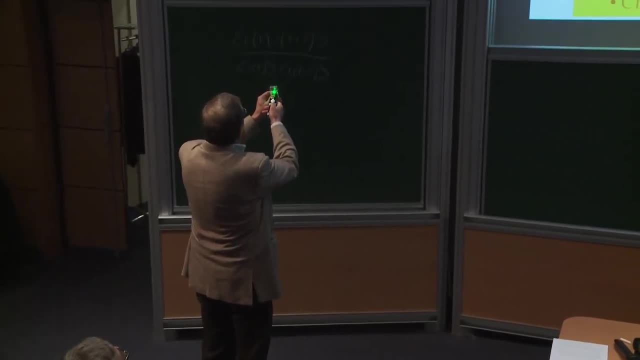 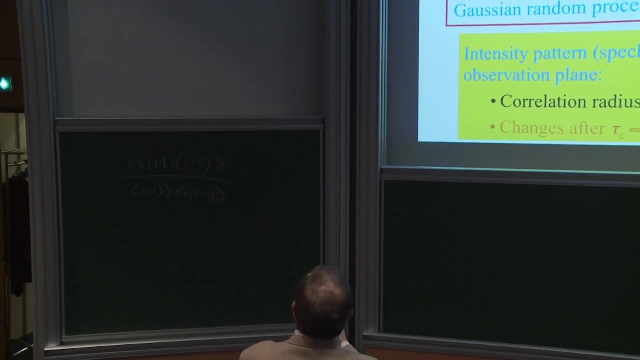 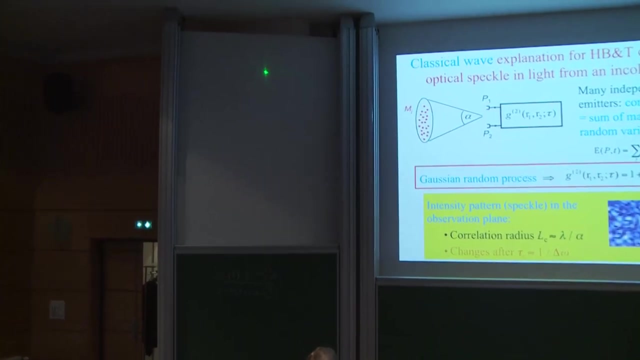 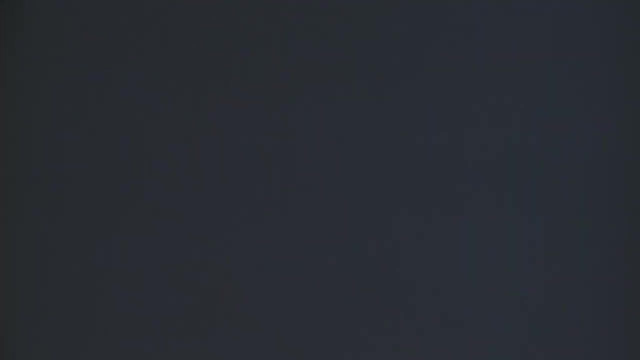 Puis, je t'en prendrai une après. If I go further, Apart from the cross, you see that you have black and dark, dark and white spots. Do you see them? A granularity? OK, It's a random granularity. This is a laser speckle. 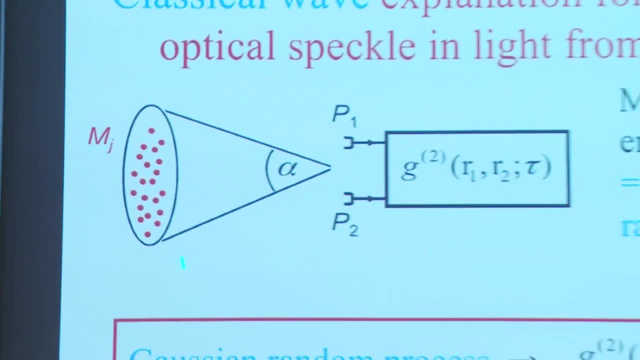 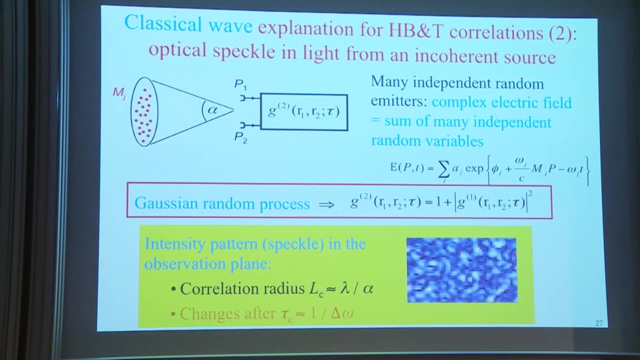 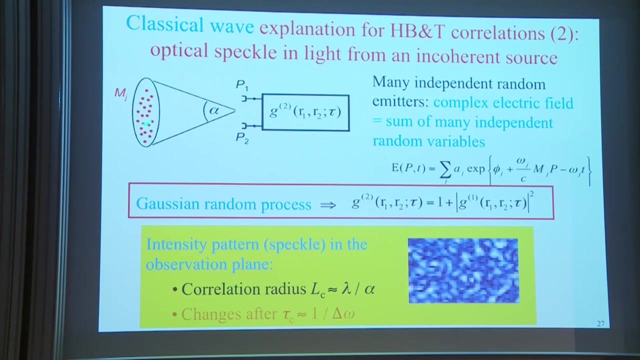 OK, The idea is the following: Let's suppose that I freeze what I get here at the scale of 10 to the minus 15 seconds. OK, So nothing evolves. What I get is this interference between these many independent, random variables. This is exactly what I get here. 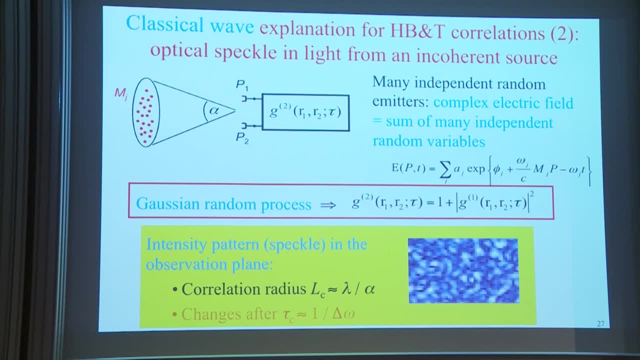 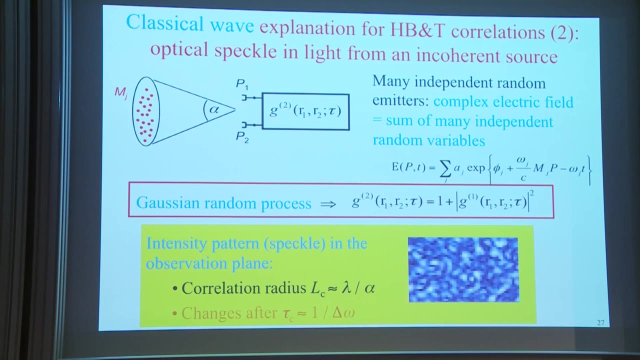 That's the speckle. Now, if I let time go on, what will happen is that this speckle will change OK, All the time. If now I put two detectors separated by a large distance, it's totally incoherent. 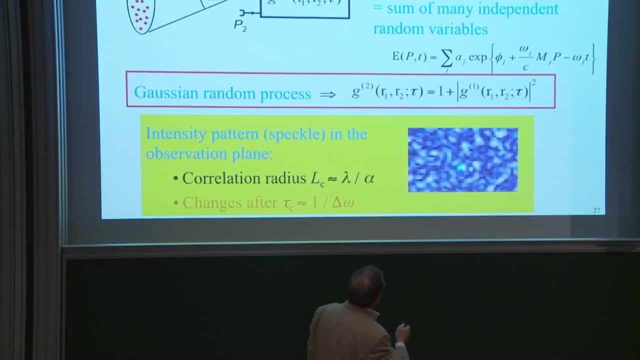 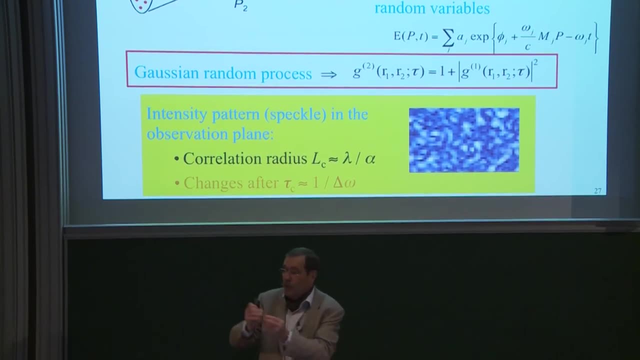 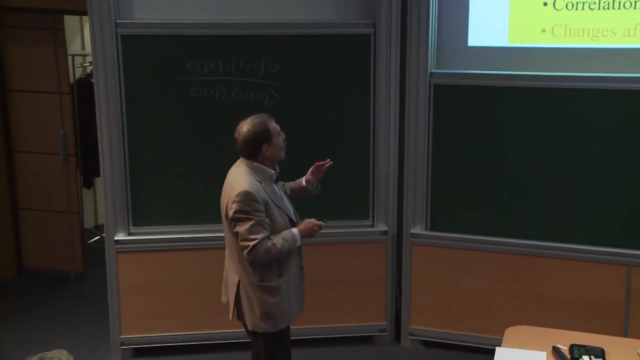 But if I put two detectors at a distance which is less than a typical size, that is to say less than the correlation length, here the fluctuation will be correlated. This is a very nice classical representation of the calculation I have shown, So we understand perfectly well. 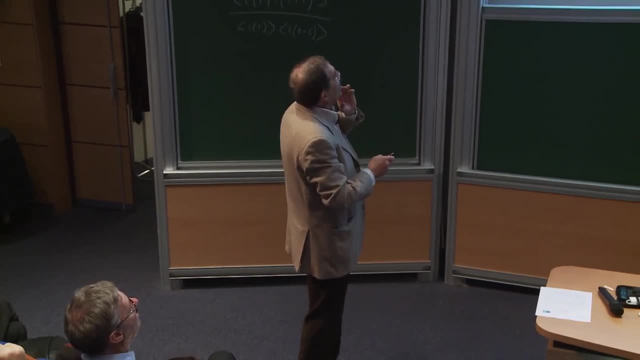 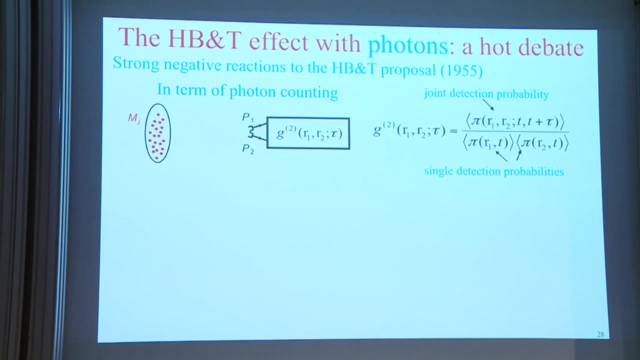 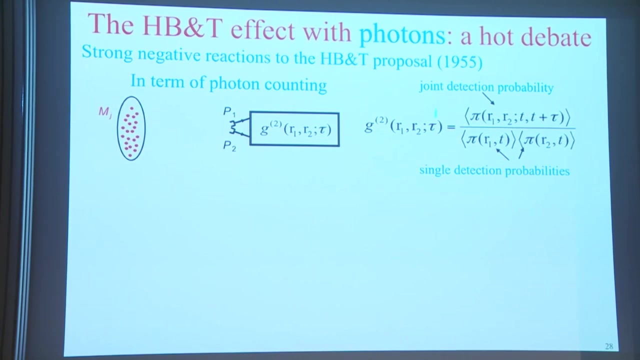 from a classical point of view. Now, when people try to understand the Ambry-Brown and Twisse effect, taking into account the quantum nature of light and thinking of photons, this is the description that you give. The G2 correlation function is the ratio between the probability. 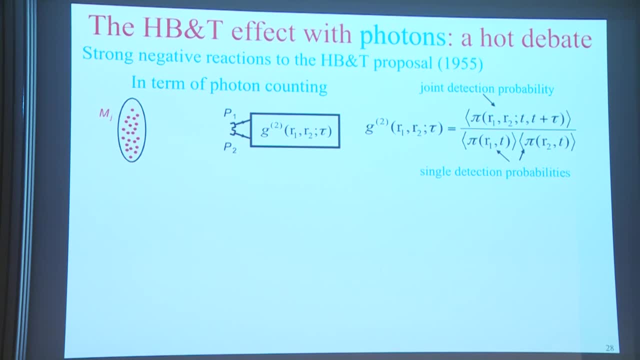 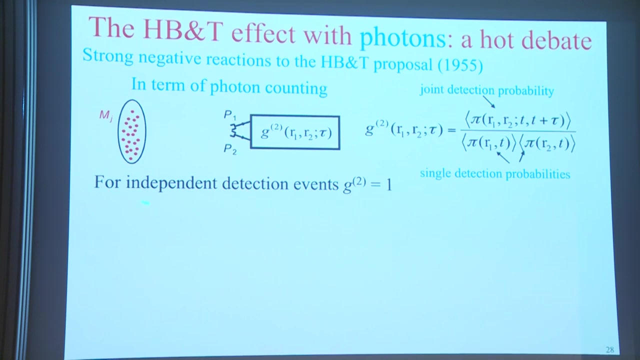 of joint detection of two photons divided by the product of the probability of single detection, And then if you find a factor of two, there is a problem because if you have independent detection event, the probability of joint detection is just equal to the product. 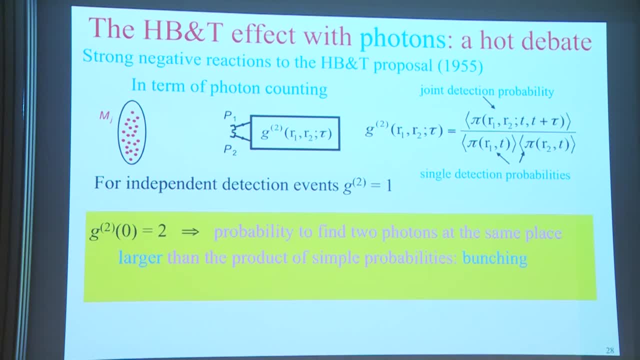 of probability of single detection. So if you find G2 different from one, it means that the photons tend to come by pairs, tend to come together. The factor of two say we detect the photon by pair close to each other. But how can it be? 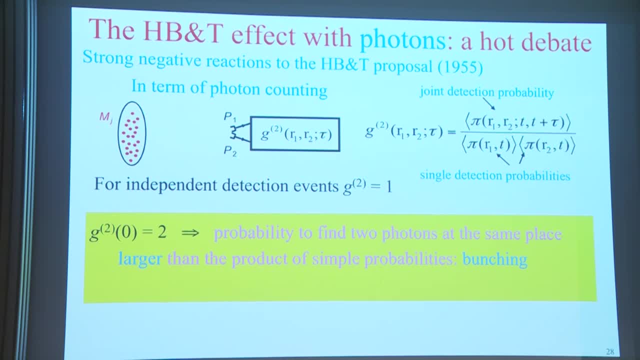 You have a star. The photons are emitted by different points of the star, maybe separated by thousands of kilometers. Obviously, they are independent particles. So how can it be? So you know what happened to Ambry-Brown and Twisse: They applied for grants. 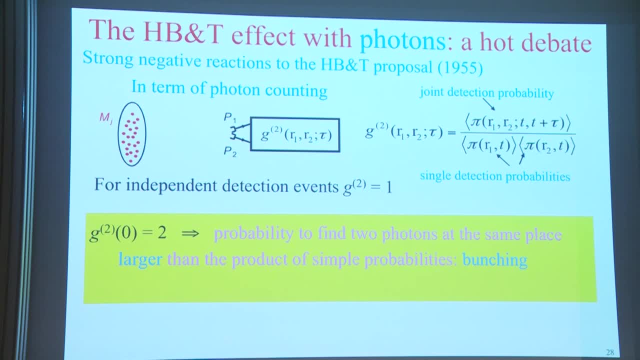 They were in UK. OK, in England They applied for a grant to build an observatory and they did not get their money because the referee said: hey, it's stupid, because of course photons are independent. They are not going to have this bunching factor. 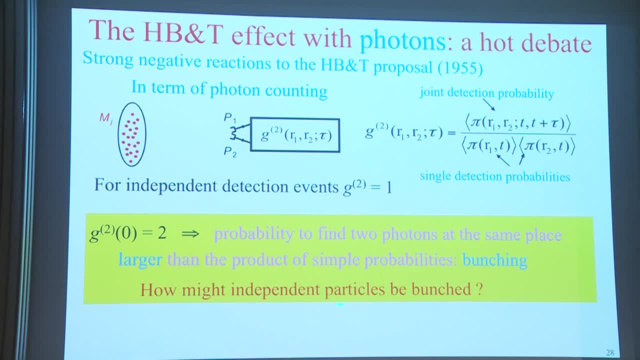 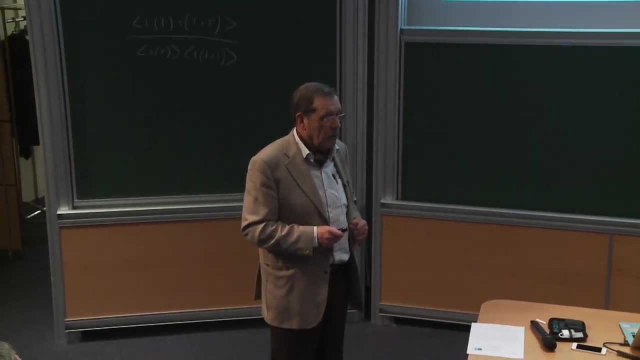 And so the question: how might independent particles be bunched? No, they are not. The referee said: OK, we don't fund you. This is why they immigrated to Australia, And there are two interpretations to the fact that they were funded in Australia. 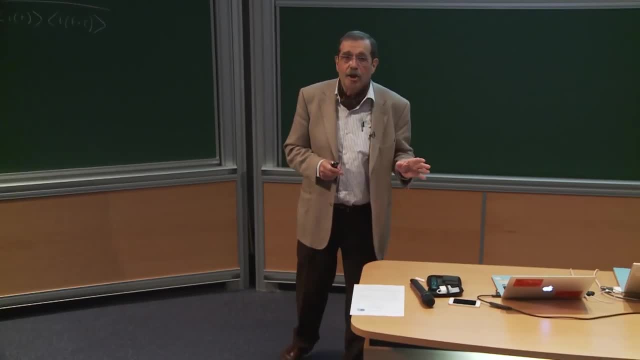 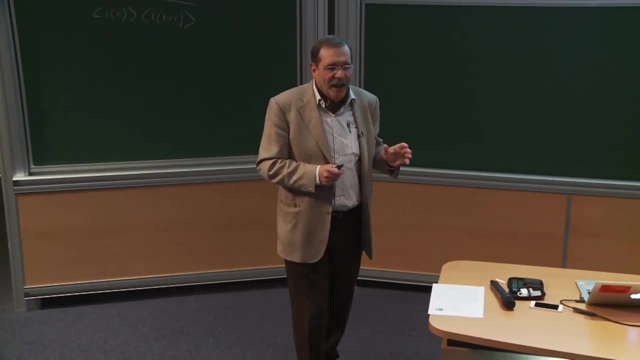 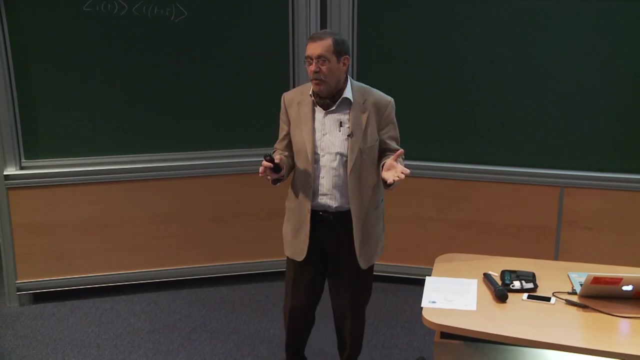 Are there Australian people in the room? No, There are two interpretations. The first one. The first interpretation is that quantum mechanics was not yet arrived in Australia, So they did not know about photons, And the second interpretation is that they were very smart. 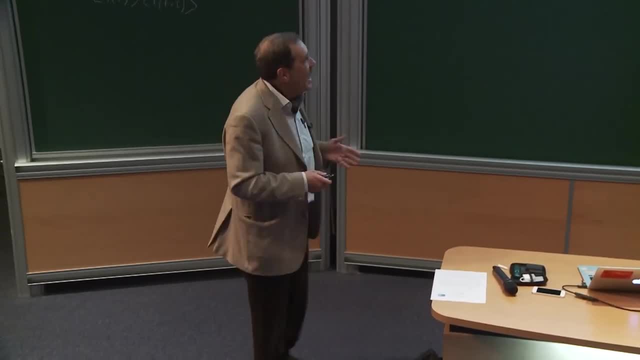 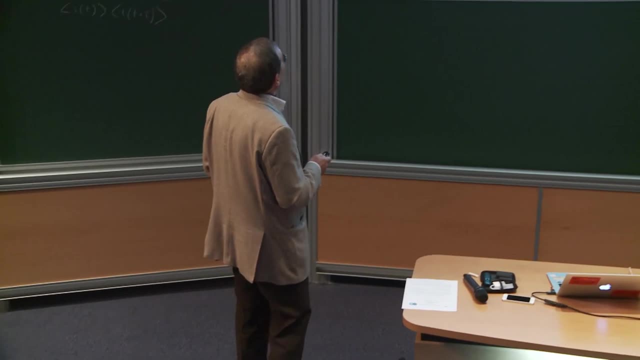 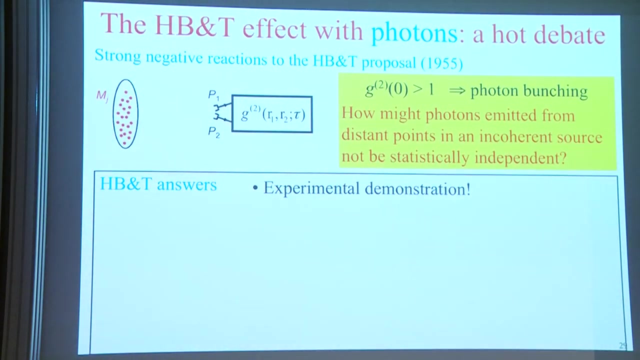 So you choose. Anyway, the Australians funded them and they built the observatory and they found that they use it. OK. Of course, before immigrating to Australia, they tried to argue with the referee, as we all do, OK. 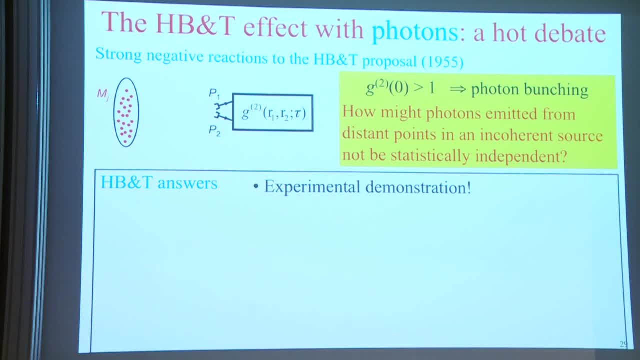 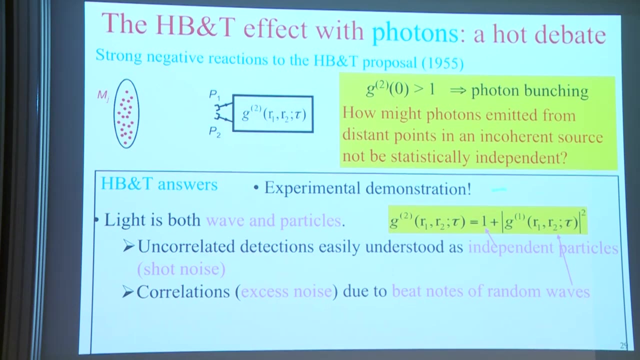 when referees are not fair to us, we try to argue. So the first thing they did was a small tabletop experiment I have described. They say, hey look, there is OK. And then they made basically the reasoning that I have made here. 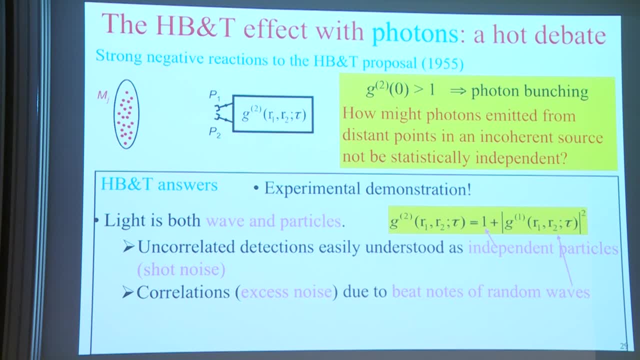 But they added the fact, you know, light is both a wave and a particle, so in a sense, et cetera, et cetera, And uncorrelated detection can be. well, they gave a very nice interpretation of this formula. 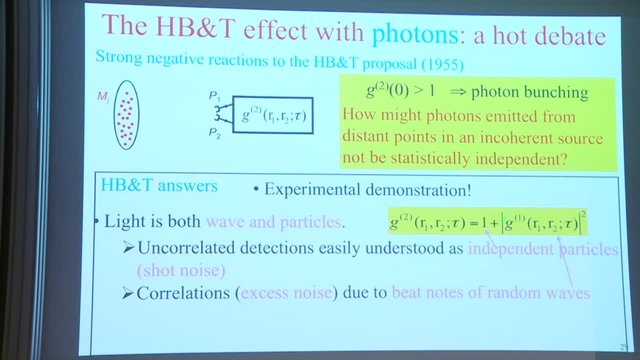 which is the following. They said: the first factor here is the one that you would get if you had really independent particles. OK, This is what we call the shot noise. The shot noise is what you have when you have many independent particles. And they say: the second term: 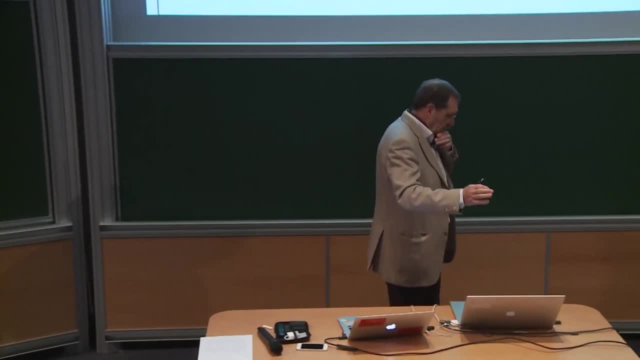 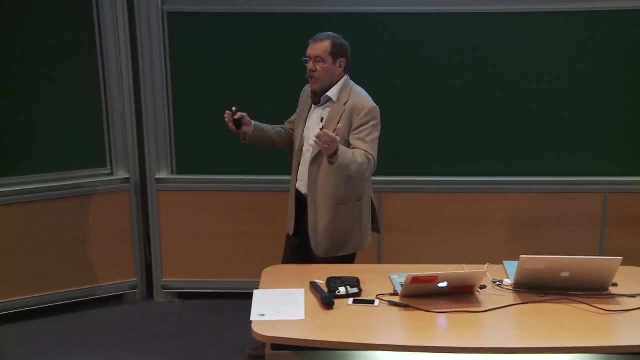 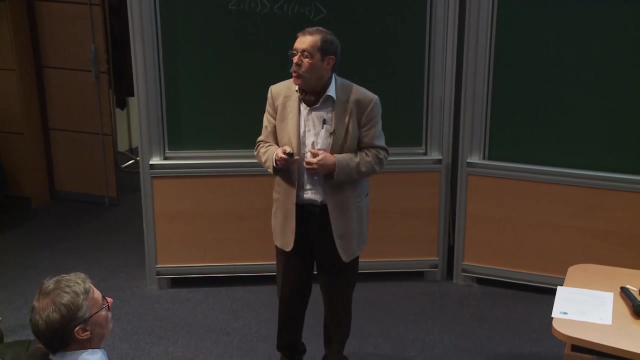 is the fluctuation that you can represent by the following model. Let's suppose that you have many independent waves. Each pair of waves give a big knot, And so you have an addition of many uncorrelated big knots, And when you do the correct calculation, 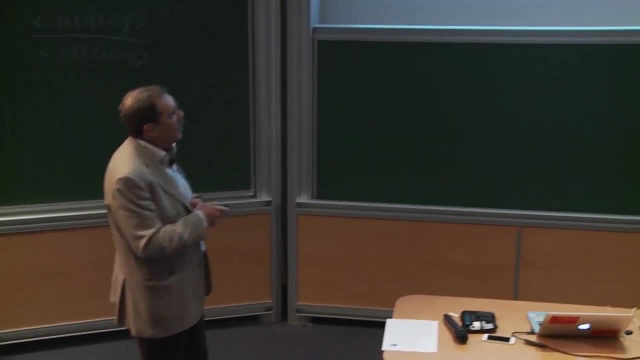 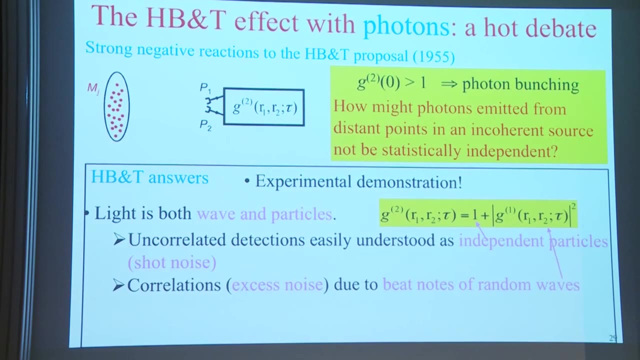 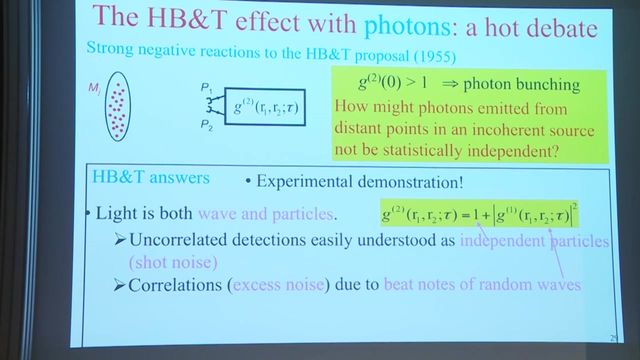 you find it did this second term OK, Big knots of random waves. And the reason why I like to cite this formula is because my hero, which is your hero, also wrote this formula in 1909 in the famous Salzburg Conference. 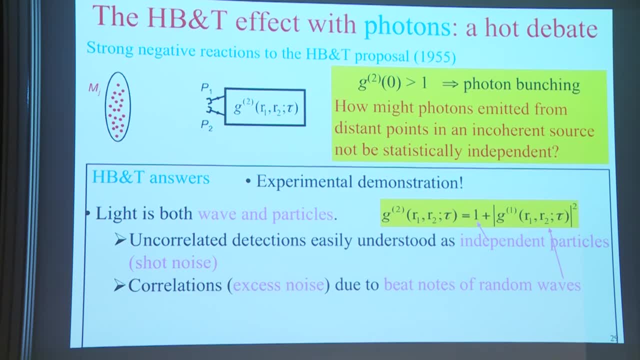 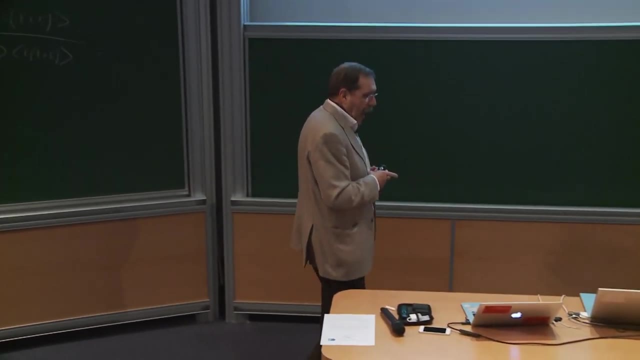 1909, OK, Einstein was a young physicist. It was his first appearance in a real conference, serious conference. OK, He was probably still an employee of the patent bureau in Berlin. And in 1909, Einstein, who had invented, 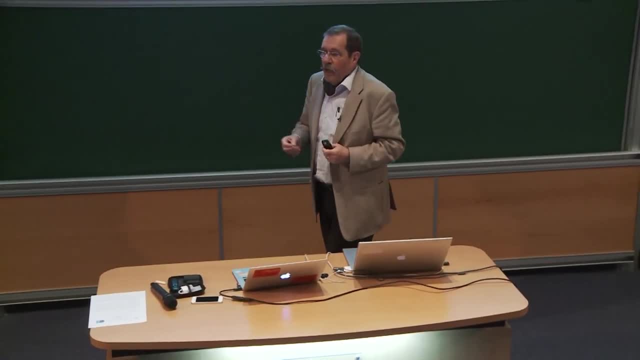 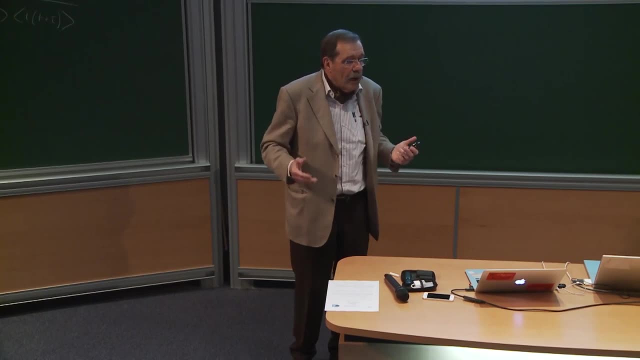 the concept of photon in 1905, was obviously obsessed by this equation. OK, We have photons, but we also have interference. OK, He could not dismiss Jung Fresnel and all these people, And he was obsessed by that. 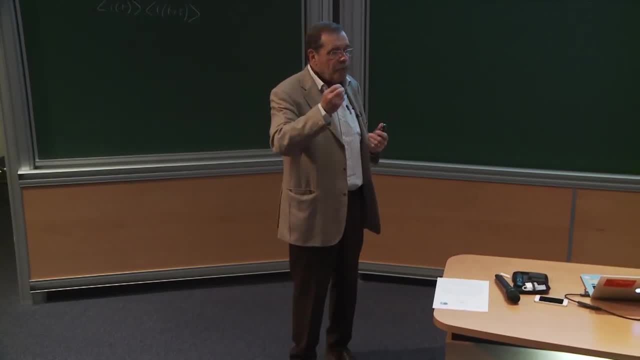 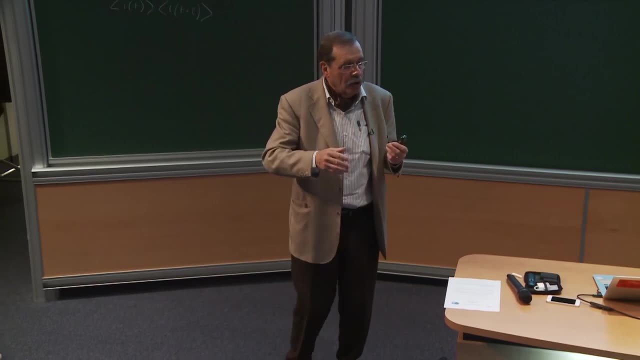 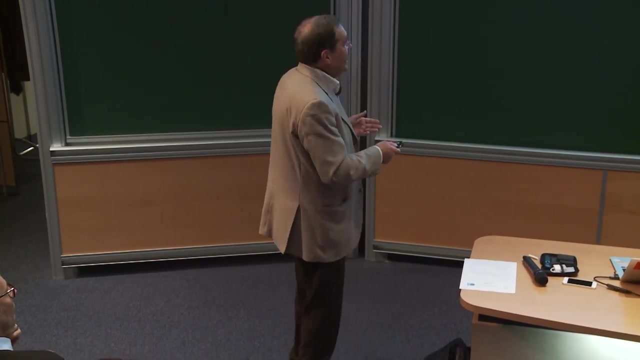 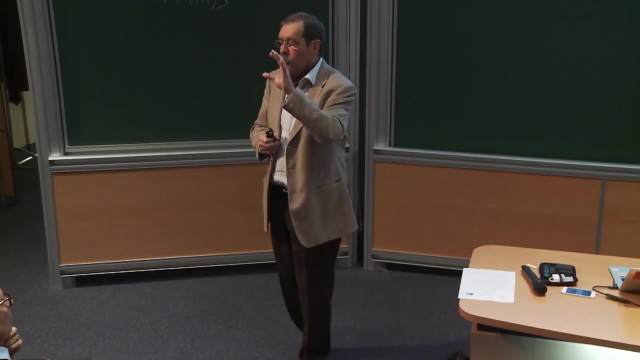 And he came to this conference in Salzburg and presented several reasoning saying that light is both a wave and a particle. So he really invented the concept of wave-particle duality in 1909.. And he explicitly wrote this formula for fluctuations in the blackbody radiation: 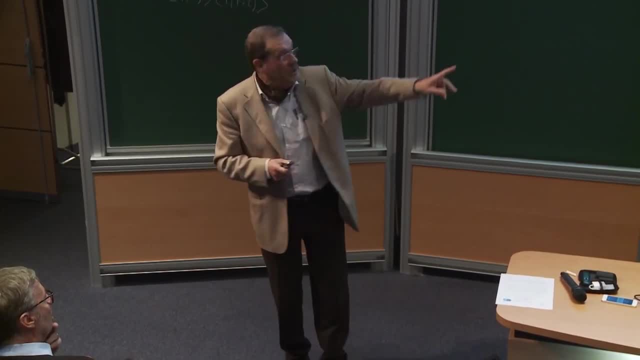 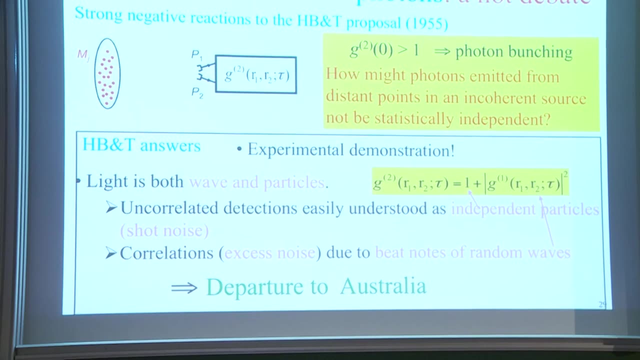 in the thermal radiation. OK Planck formula, et cetera. But he could write this And he correctly interpreted this formula In fact: Whoops. OK, I should depart to Australia, but I wanted to say No. 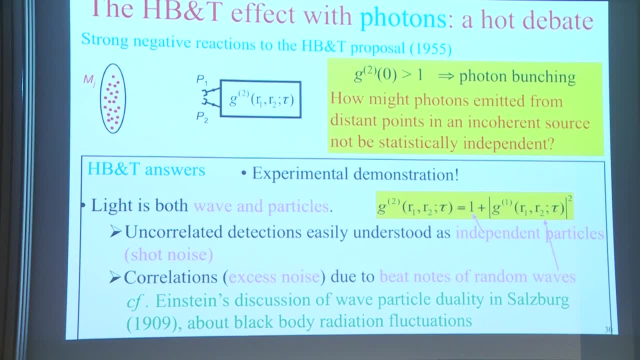 Voilà, No, no, Einstein, What he did? What he did was calculating the fluctuation of the pressure on a wall due to blackbody radiation. OK, And he found the formula which is his formula, And he correctly interpreted the result in saying: 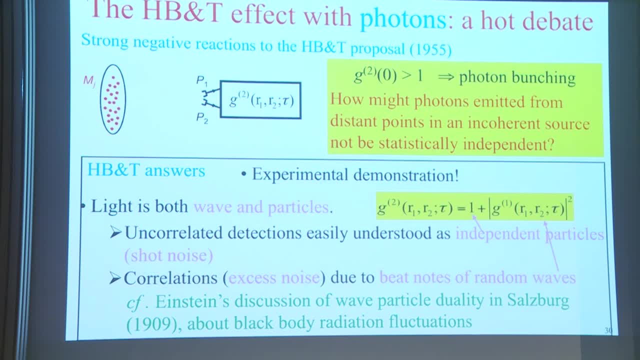 the one is a fluctuation that you have if you have many particles arriving on that. So you have a randomness, OK, a Poisson process, et cetera, and you have some randomness And the other term is a term that you have. 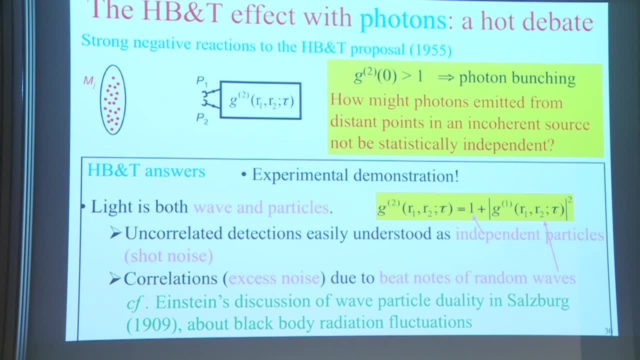 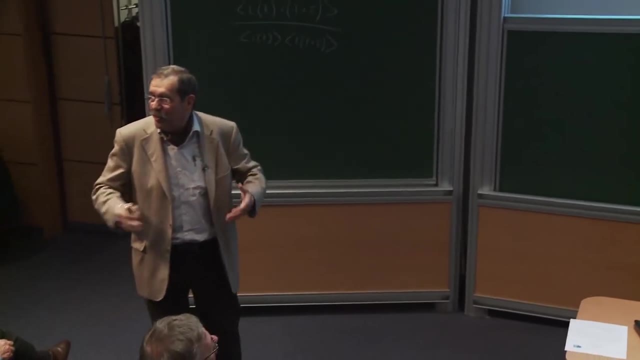 if you consider as many waves with relative phase, which are random variables, big nodes, et cetera, et cetera, This is absolutely fantastic. I mean, we never recognize enough the genius of Einstein. We always discover new things in all the papers of Einstein. 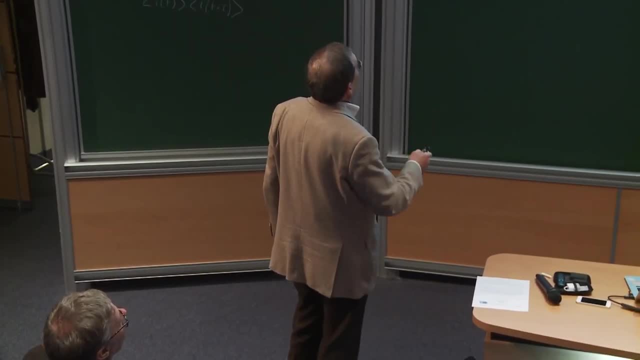 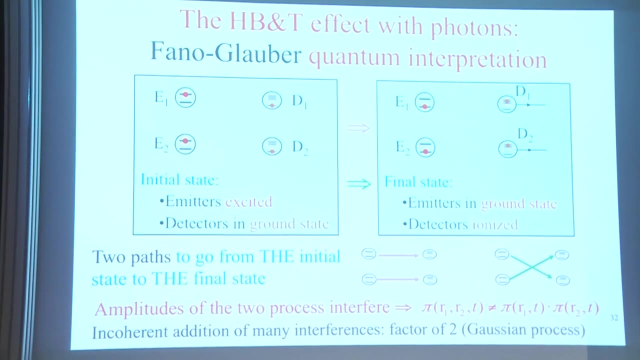 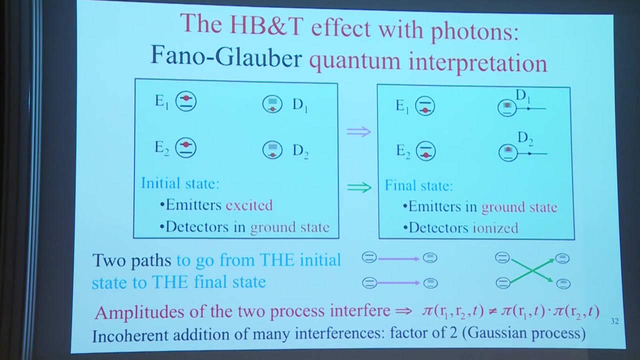 OK, So I recommend this, And there is a book which explains that very well. OK, Now, good as it was, the defense of Ambly-Brown and Twist was not fully convincing from a fully quantum point of view, And the first really convincing description. 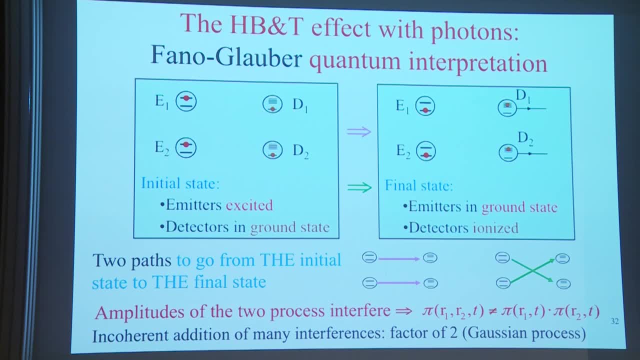 of the phenomenon in terms of full quantum mechanisms and full quantum optics is due to Glauber. Well, Fanon had the preliminary of that, but the clear explanation is due to Glauber, And Glauber presented a toy model. You all know what is a toy model. OK. 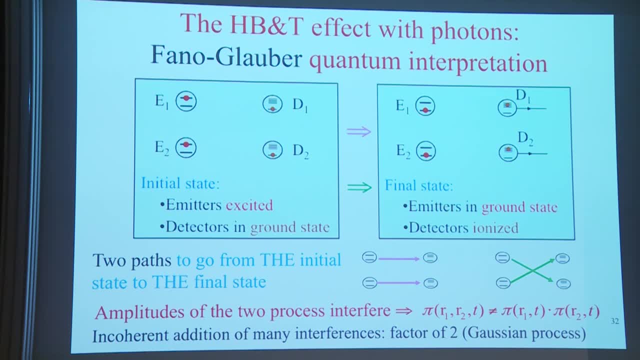 It's a small model which certainly does not describe reality in all its details, but the basic idea is in it. So Glauber came with a toy model which is the following: We have two emitters which are excited, ready to deliver a photon. 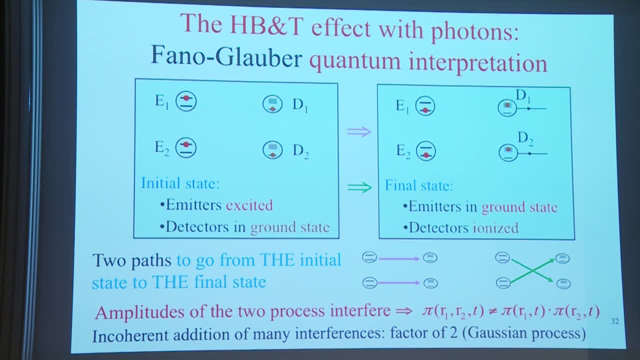 And we have two detectors which are in the ground state, ready to detect the photon, And then the two photons are emitted and they are detected. And so, at the end, what do you have? You have the two emitters which are in the ground state. 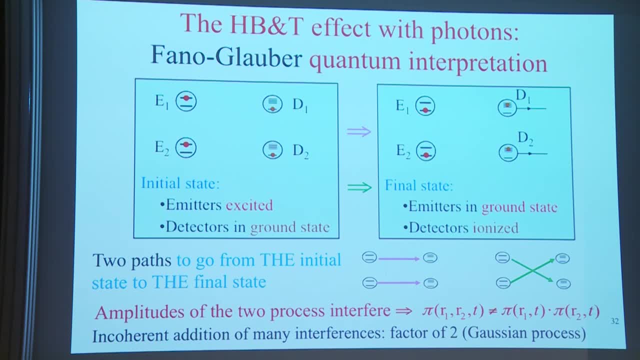 and the two detectors are excited. And when they are excited the electron is free, and then you can amplify it with an electron multiplier And you observe a pulse. OK, And Glauber says, OK, we all know from the basic principle. 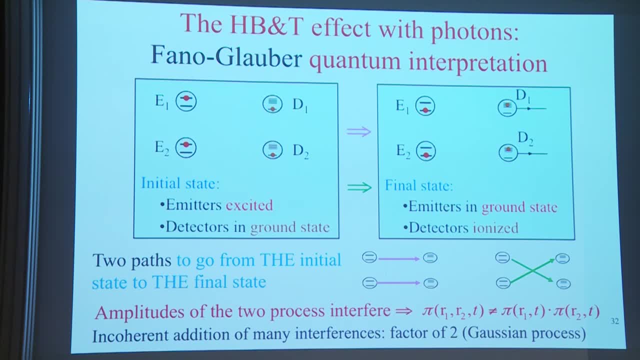 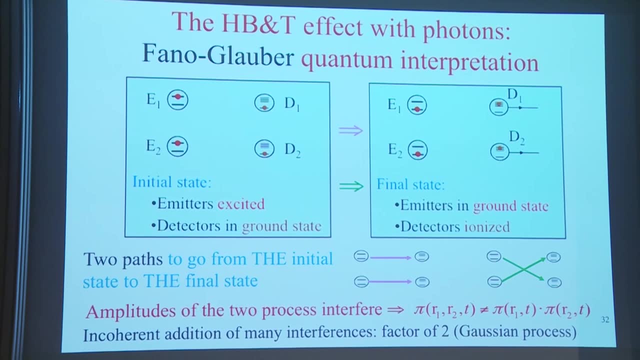 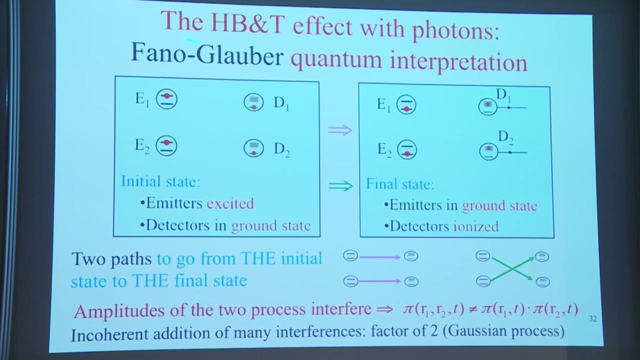 of quantum mechanics that in order to calculate the probability to go from an initial state to a final state, we must consider all the possible paths and add the amplitudes associated to this path. And in fact he says there are two possibilities to go from here to there. 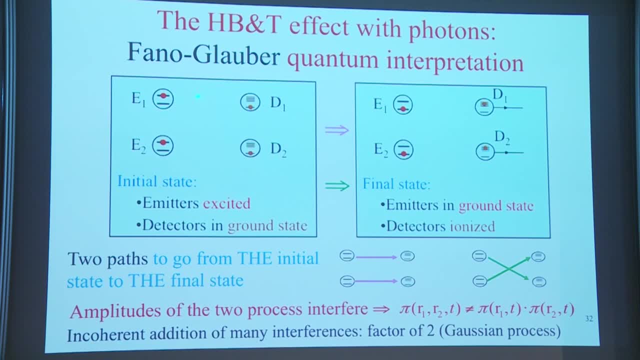 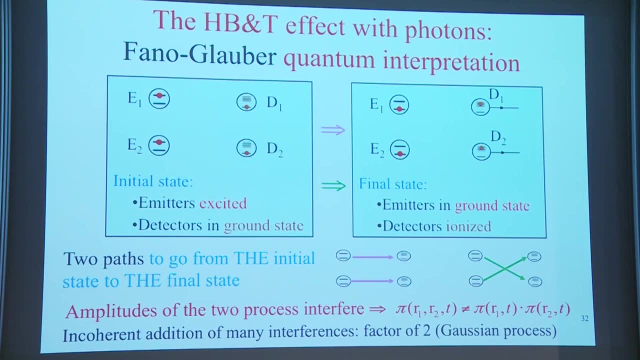 The first possibility is that the photon emitting here is detected there and the photon emitted here is detected there. So it's represented by this diagram. But there is another diagram where the photon emitted here will be detected there, and this one will be detected there. 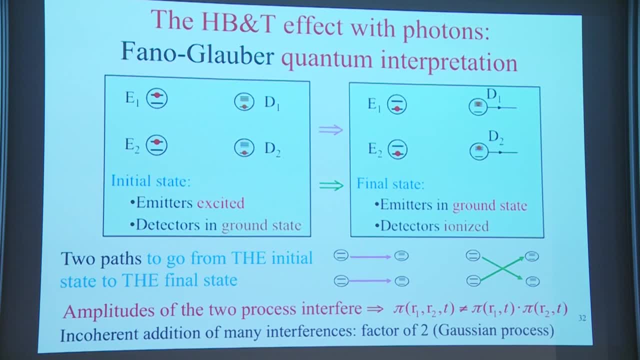 It's a second diagram, And what you must do to calculate the probability is first add the two diagrams, OK, and then take the square of the modulus of the complex amplitudes, OK, And so you have an interference between these two diagrams. 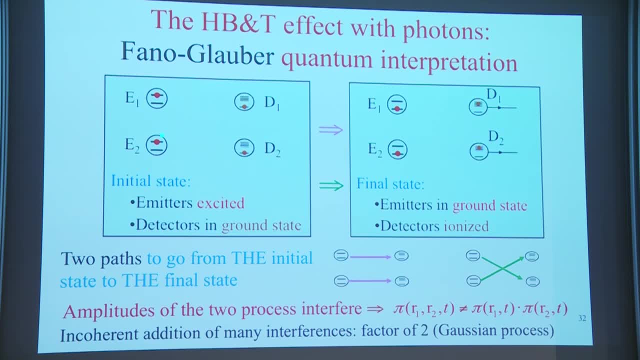 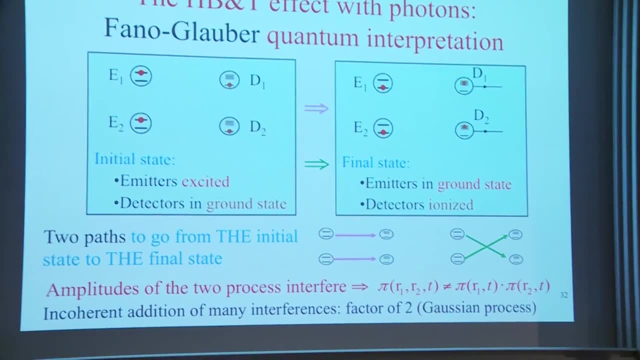 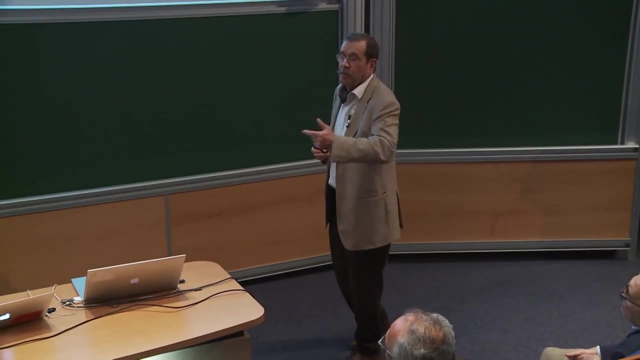 because there is a phase which depends on the distance of the emitter. So when I am going to have many pairs here, these various interferences will produce a fluctuation and it's not very difficult to find that this fluctuation is a Gaussian fluctuation and you get the factor of 2.. 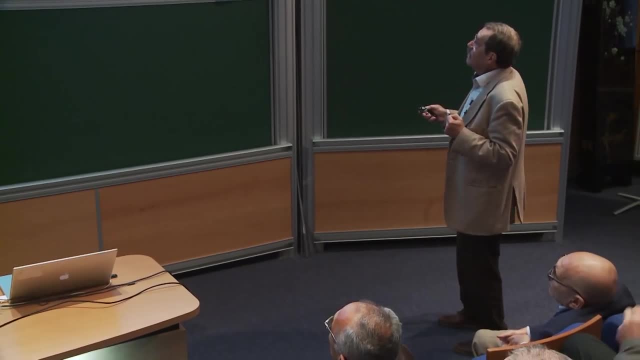 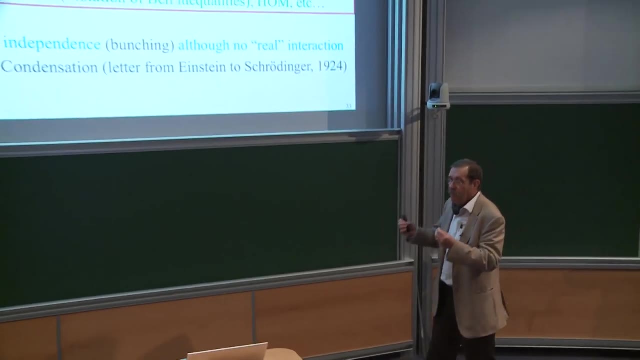 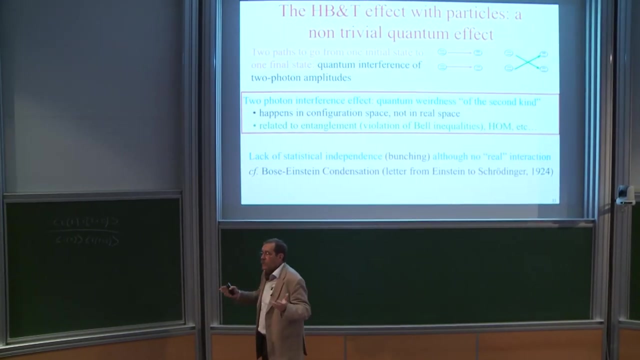 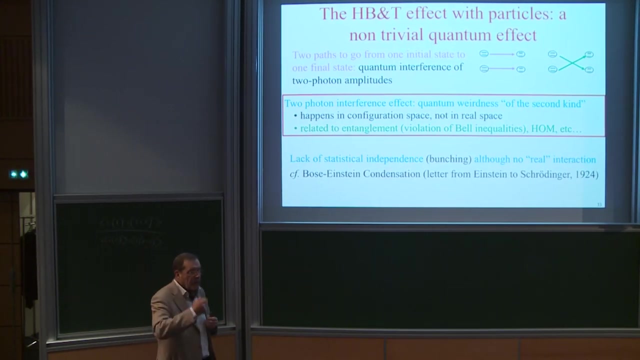 Why is it important? It's important because, to my knowledge, it is probably the first time when somebody explicitly invokes interference of two photons. I don't know example in the literature of somebody explaining an effect by saying: what I have is an interference between amplitudes associated to two photons. 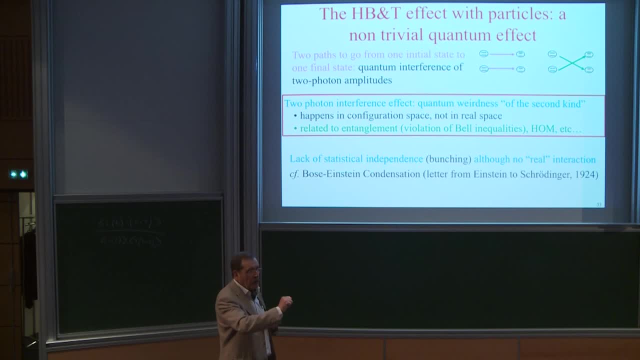 It's one two-photon amplitude, another two-photon amplitude. They are complex numbers. I add these complex numbers And then I take the square modulus. OK, So this is what we call these two-photon interference effects. quantum weirdness of the second kind. 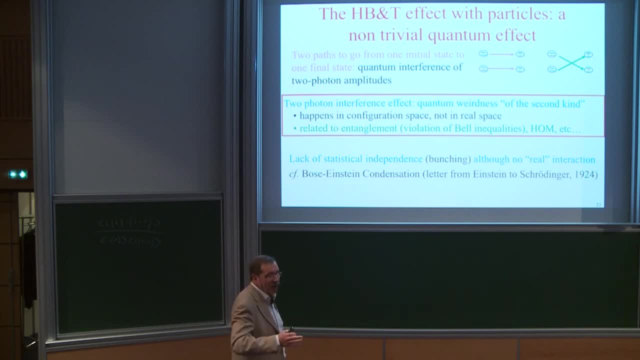 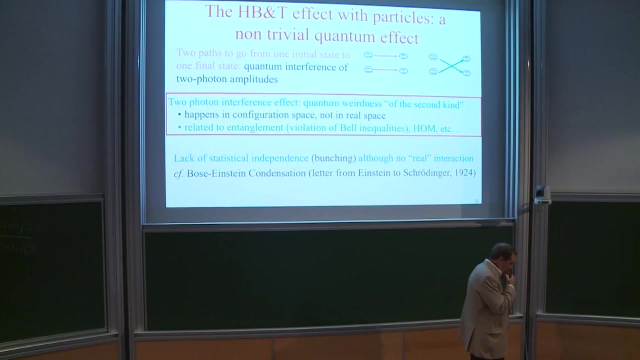 that is to say the one that Feynman discovered, well, discovered, realized that it is important in the 1980s, OK, and is related to entanglement. Now, again, I will cite Einstein. We have to understand. 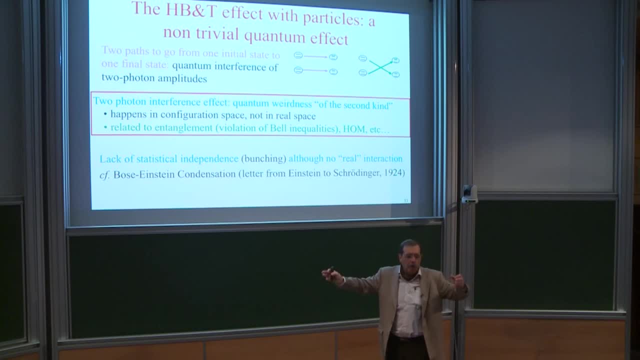 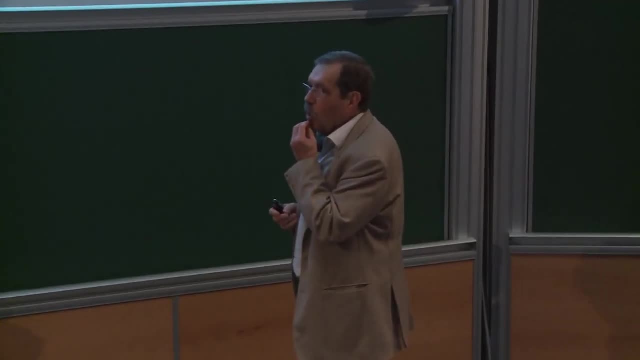 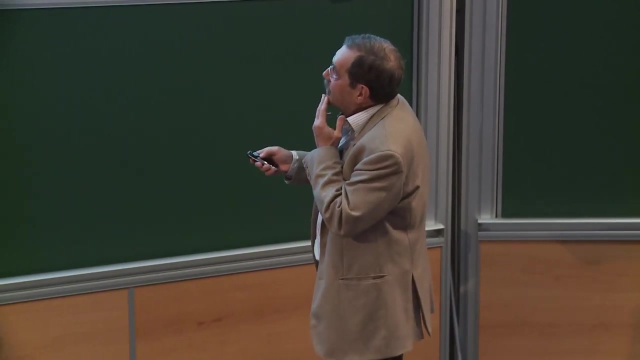 Because this is referee who say: look, we have independent photons, et cetera. They were right, The photons are independent. So we have to understand that these effects, which is called the bunching effect, it's not, it's a lack of statistical independence. but there is no real interaction. We should not think of it as the two photons having some kind of attractive interaction between each other. It's just like Bose-Einstein condensation. This is why I cite the letter from Einstein to Schrödinger. 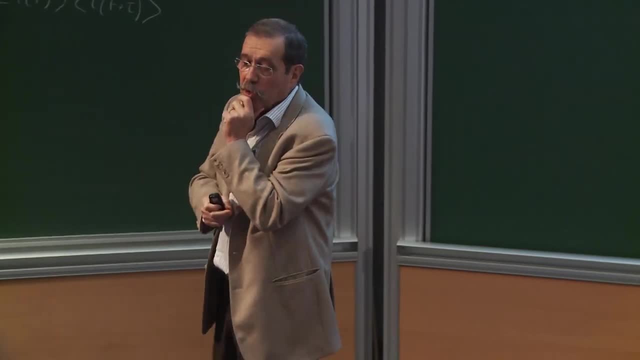 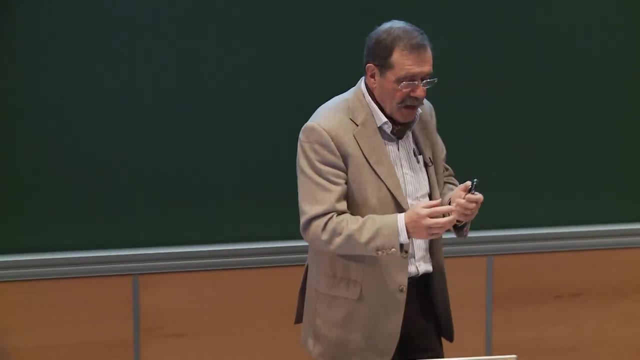 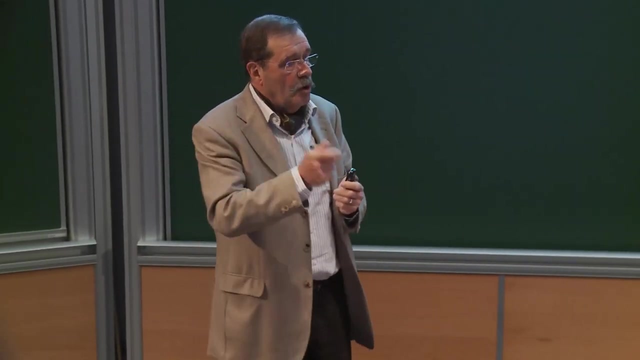 about what is called Bose-Einstein condensation. Bose-Einstein condensation is the fact that when you have bosons who like to be in the same quantum state, the statistics is different. And when Einstein published his paper in 1924, Schrödinger sent him a message in saying: 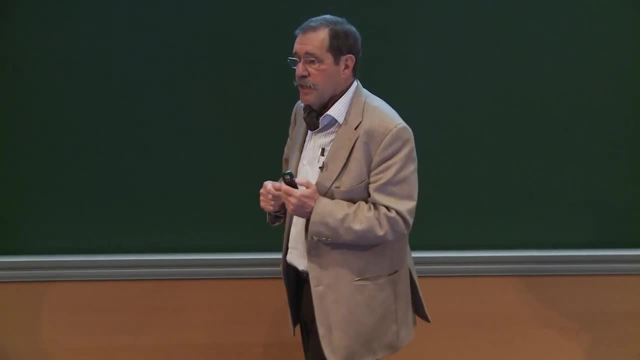 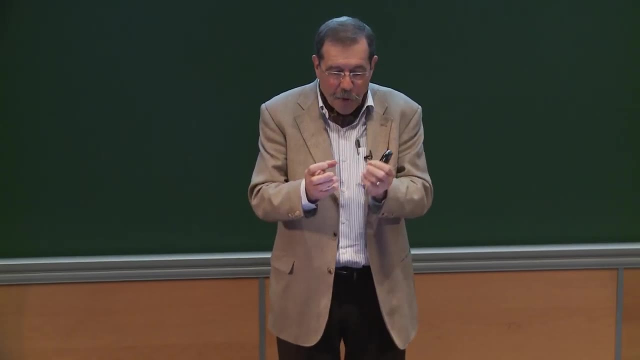 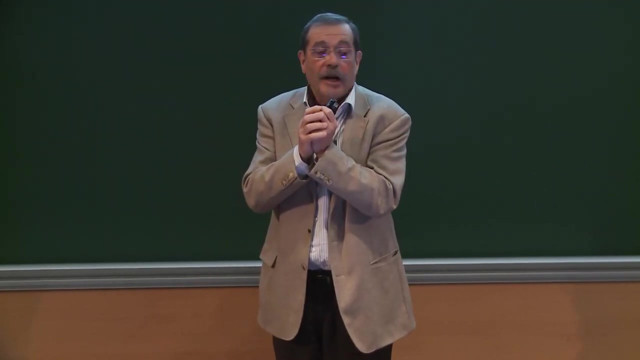 you have made a mistake in your calculation. And Einstein said: no, no, no, no, I don't have made a mistake. It is true that everything happens as if the boson would like to be on top of each other, But don't think of it as a real interaction attracting them. 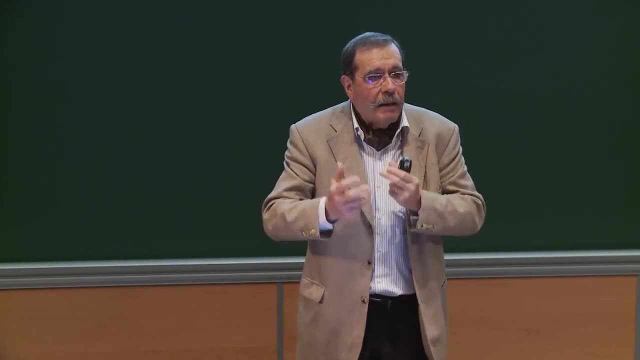 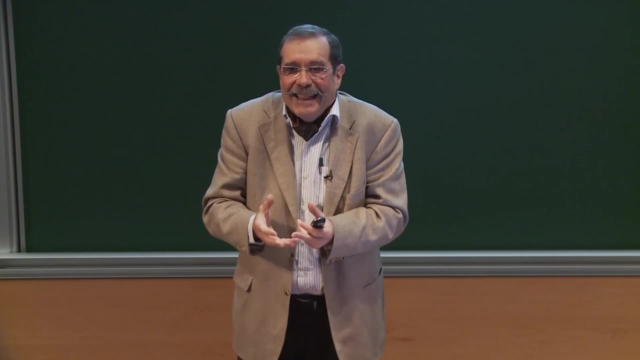 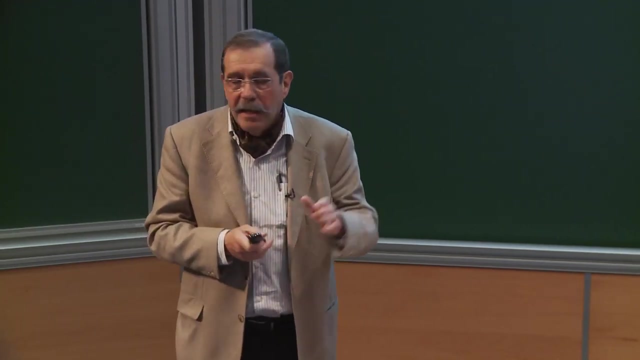 It's the way we describe the problem with the different statistics, or here, with complex amplitudes, which at the end makes it look like if they were attracted towards each other. It's extraordinarily subtle and it was understood again here. So it's the first time. 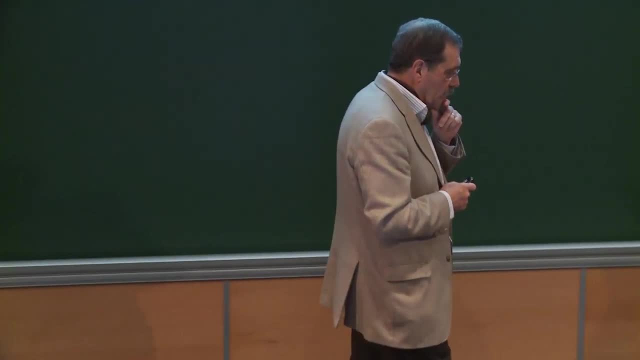 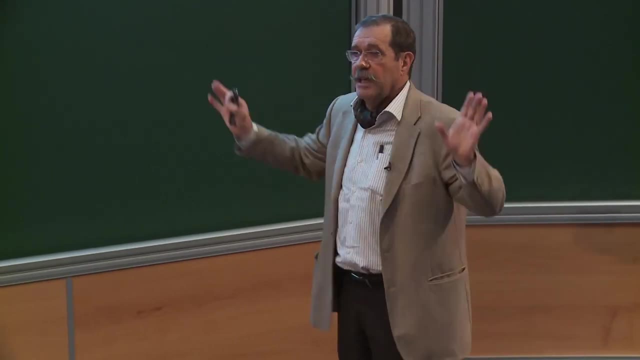 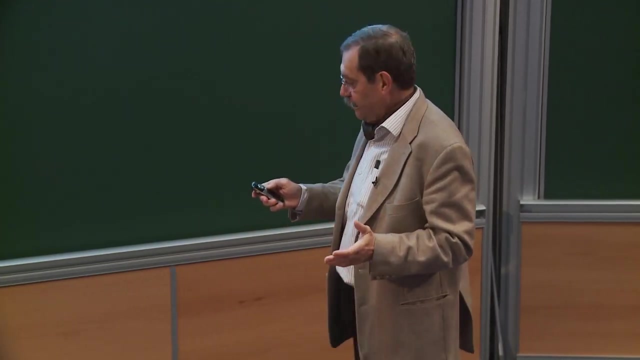 the Amber-Ivan-Lentwee effect, when somebody invokes interference between two photons And more than that, Glauber develops a full formalism of quantum optics which will be available for future discoveries. So it's kind of ironical. 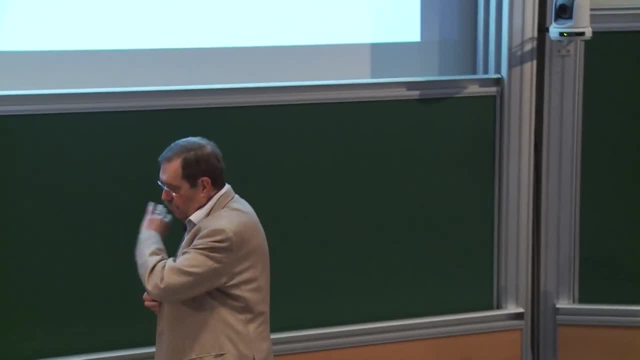 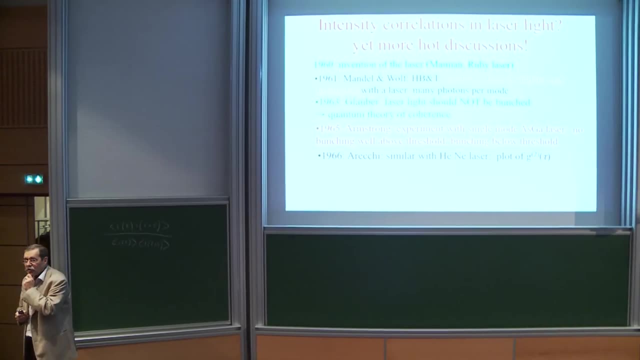 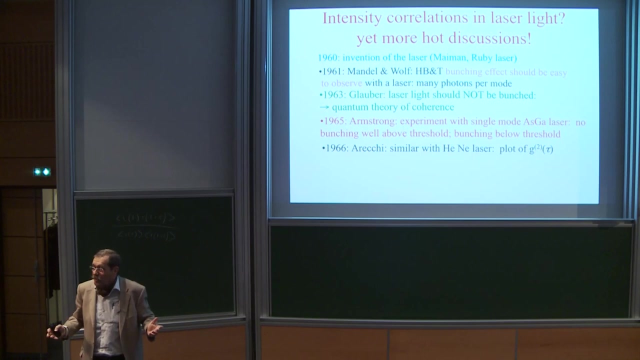 So there was terrible and hot discussion. Claude Quintanilli was a young researcher and he went to conference and told me Glauber would shout and then Mandel and Wolf would shout. There were terrible fights in conferences about that, So it was a really hot discussion. 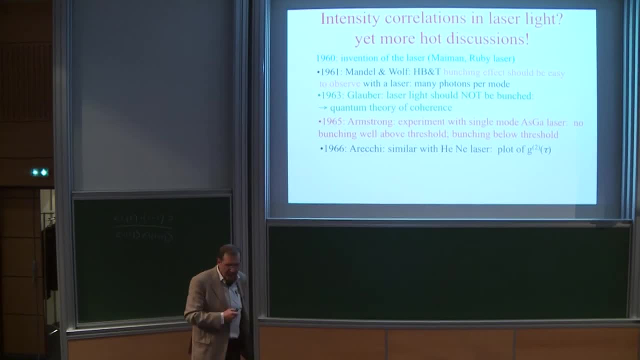 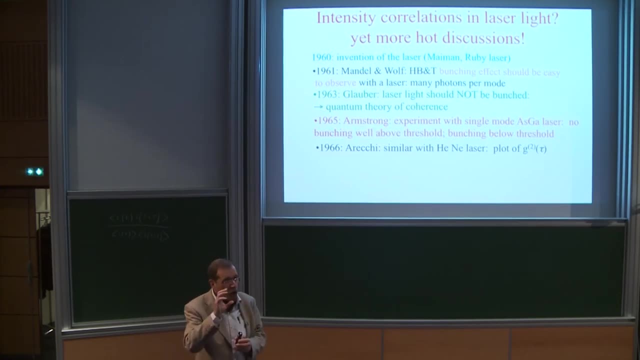 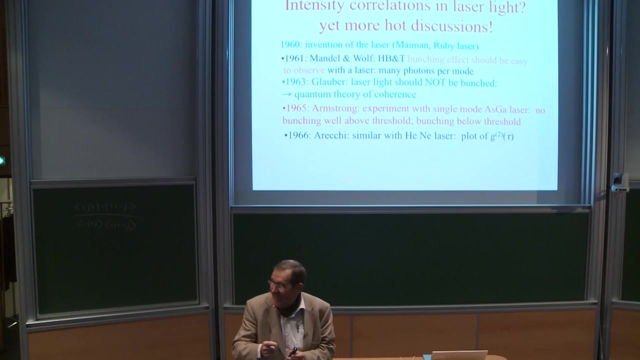 And when laser was invented, there was a terrible discussion of which you can find the trace in physical letters. I mean, when you look at the introduction of the physical review letters about these subjects, they literally insult each other Literally. You read the introduction and say: 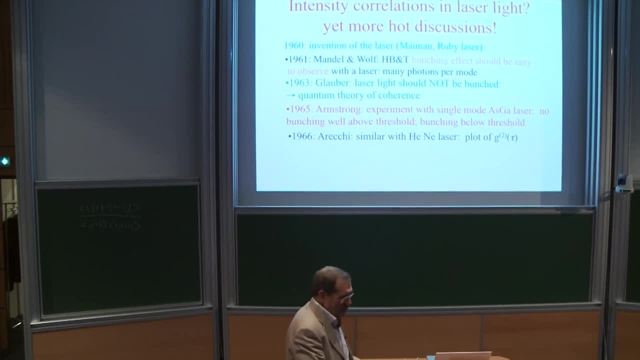 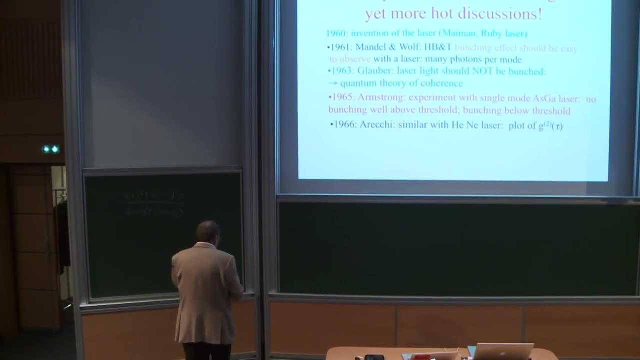 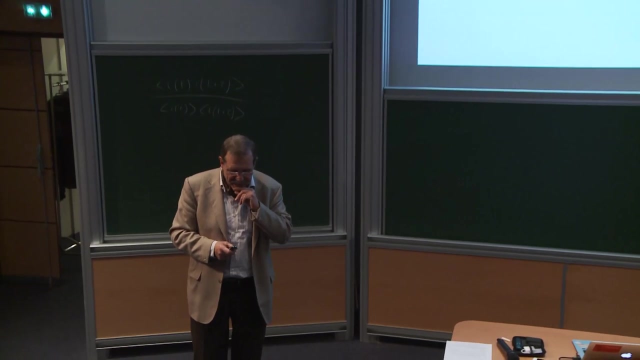 they have not understood anything. Okay, this is a real explanation. So what was the debate? Some people thought that the laser was invented in 1960, and so people thought that with the laser, it will be easy to observe the Ambery-Brant twist effect. 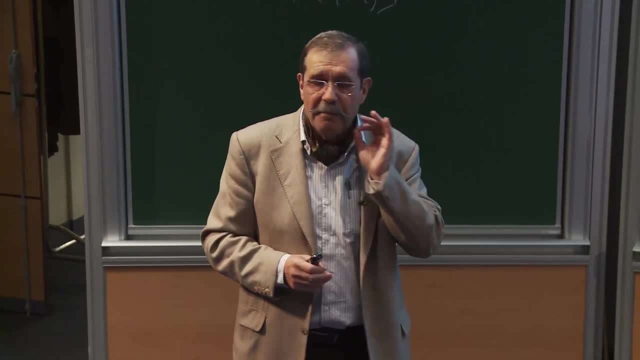 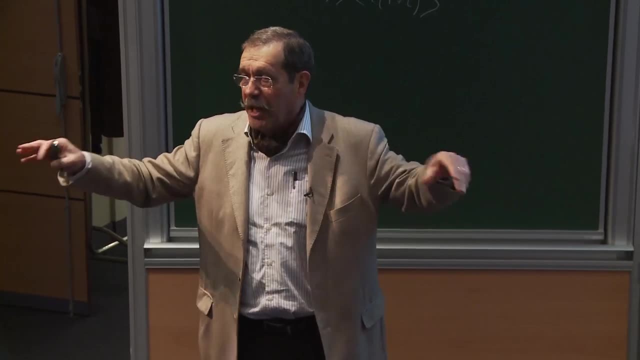 And Glauber, who had made the correct theory of the whole effect, immediately realized that it was not the case and that with a laser you would not have any Ambery-Brant twist effect, That is to say in a laser beam. 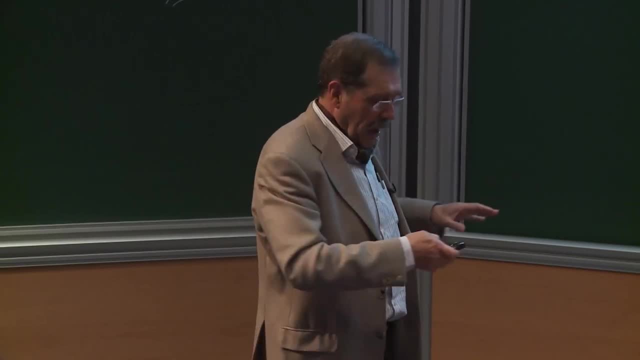 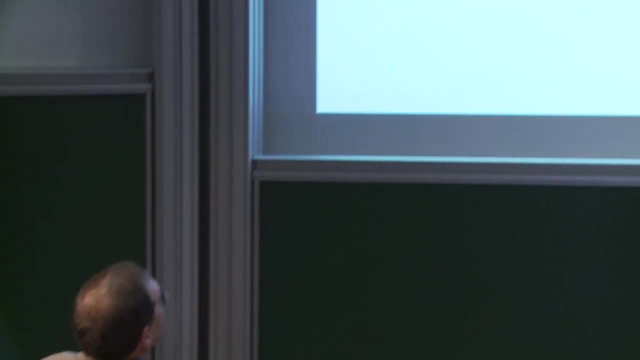 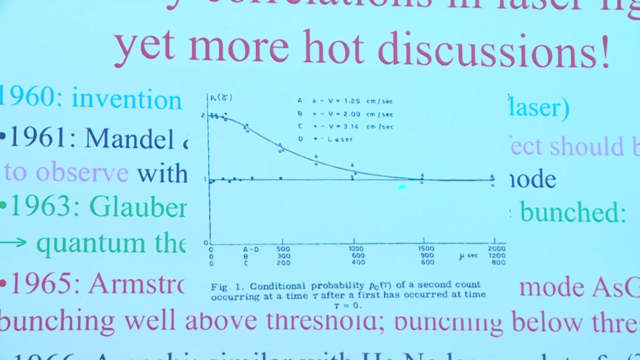 the photon are really independent of each other And the calculus. so there was an experiment which shows this. this is a single-mode laser, this is a chaotic light and you see the difference: Single-mode laser, the G2 function is one all the time. 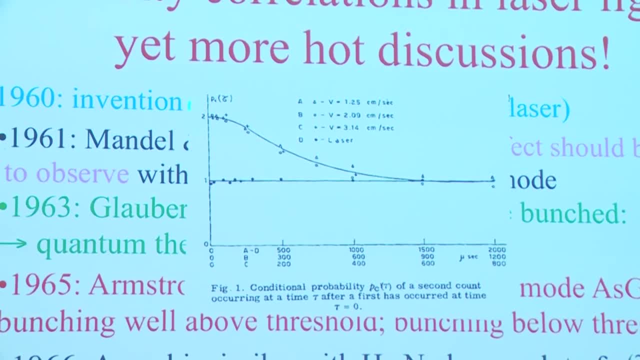 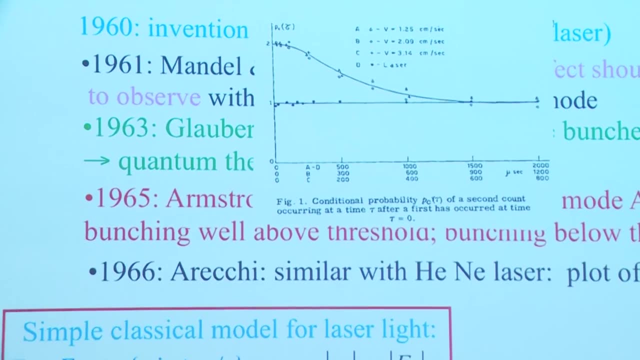 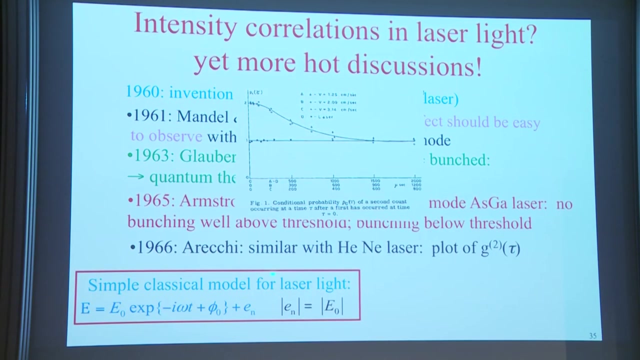 while with the other with chaotic light, then you have a factor of two And again this is extremely easy to understand in a classical vision, And in the classical vision the idea is the following: Laser light is a light of which the amplitude is extremely stable. 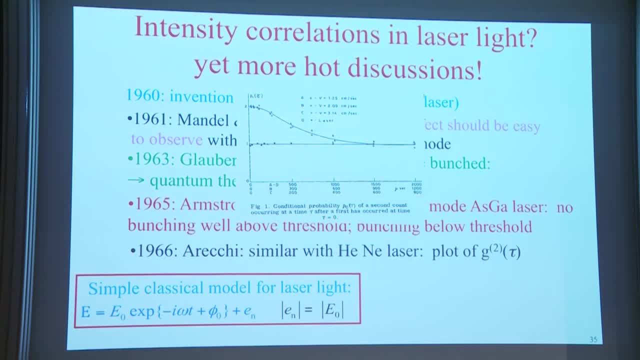 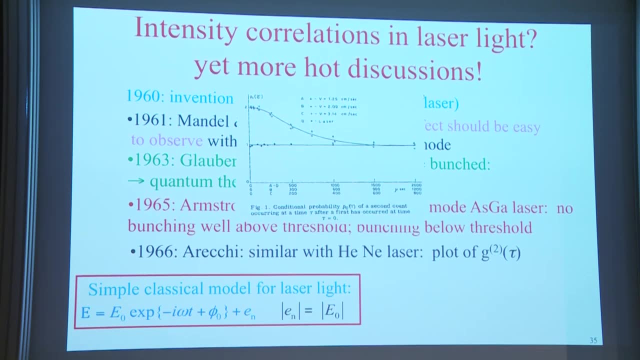 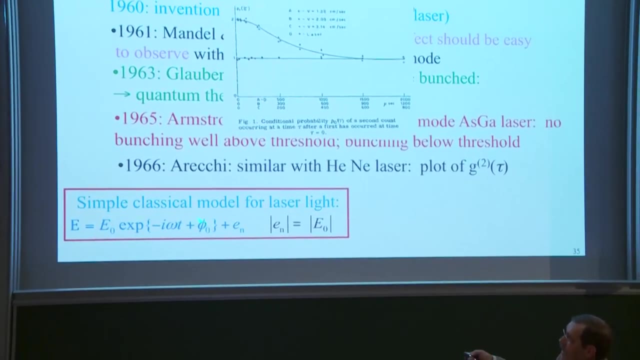 There is an extremely tiny fluctuation which is very small. The only significant fluctuation in an ideal single-mode laser is a fluctuation of the phase And of course this fluctuation of the phase is enough to provoke a line width because if the phase changes, 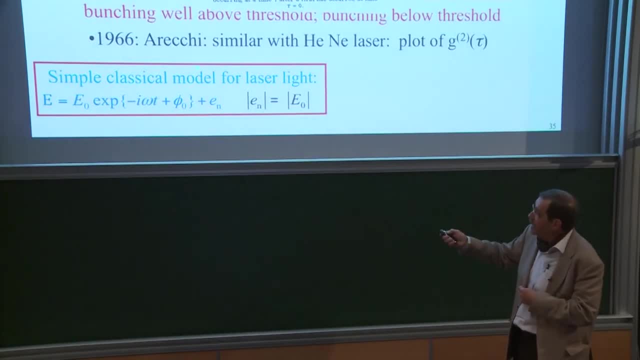 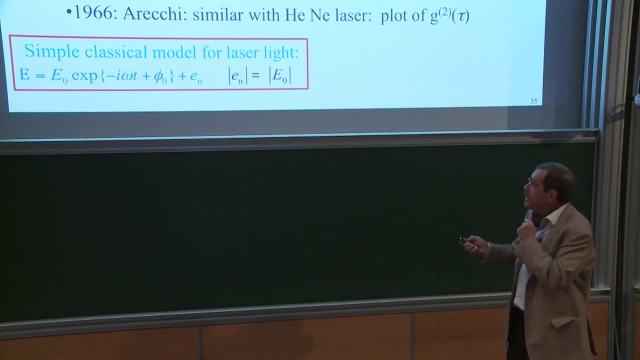 the instantaneous frequency, which is a time derivative of this whole factor, changes. So you have a laser line width, but this laser line width is due to phase fluctuation and not to any amplitude fluctuation. This is negligible, Well negligible. 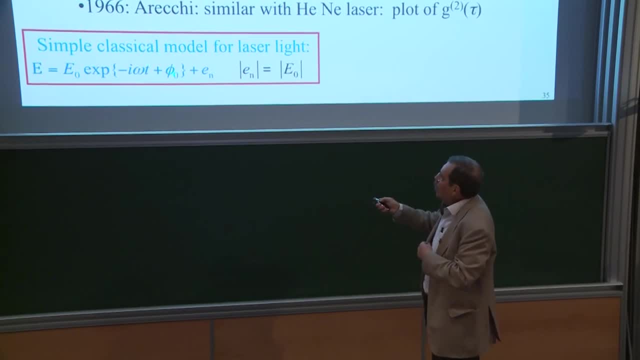 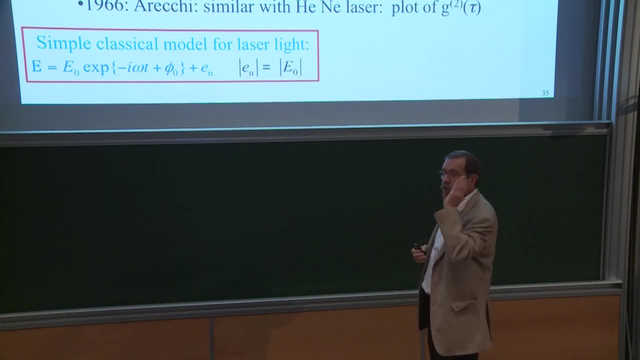 well, don't look at that, This is technical. So if really you can neglect this term, then when you take the square modulus of that, you have a constant intensity. Although the phases fluctuate, the intensity is constant. There is no big note. 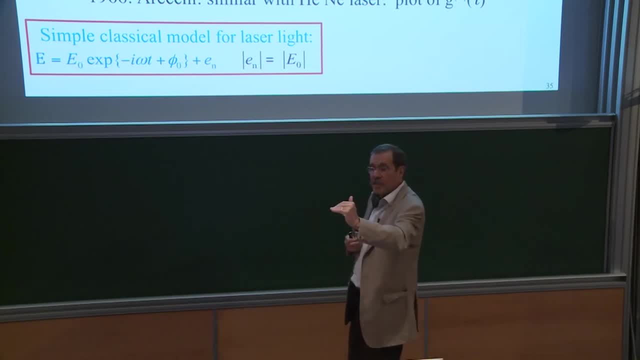 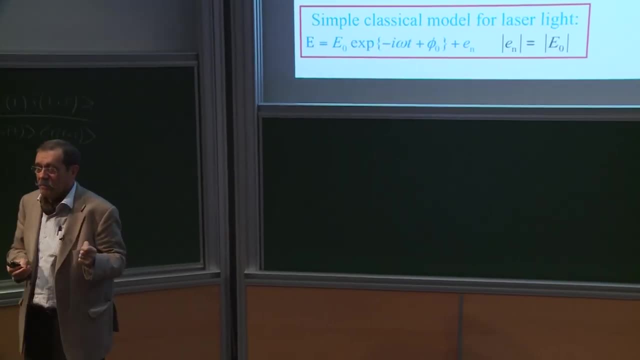 because there is only one wave And if the intensity is constant, the probability of photodetection is constant. If the probability of photodetection is constant, G2 equals 1.. And we say the photons in a laser beam are really independent. 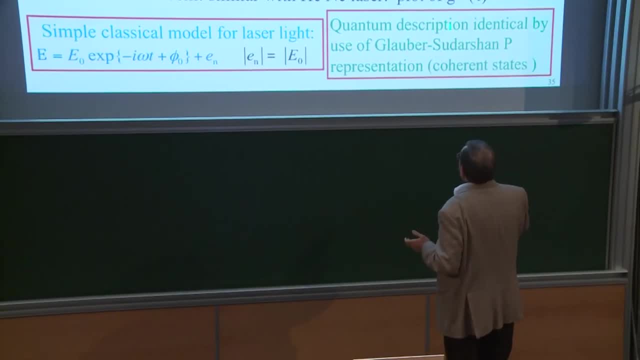 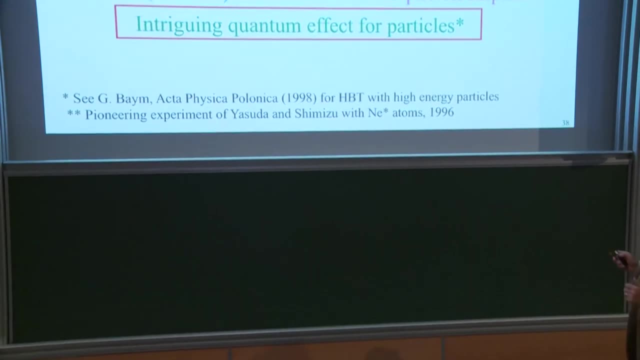 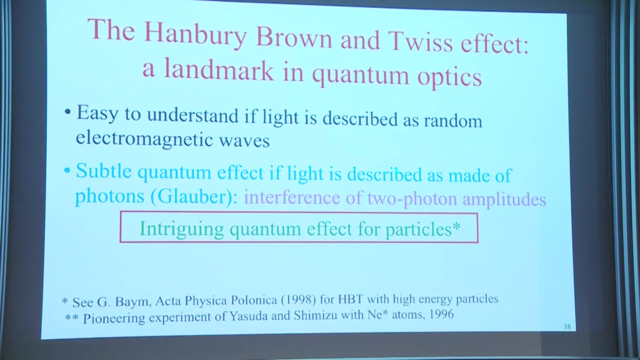 The quantum description, basically, is a technical way of rephrasing this classical explanation. Okay, So what is the conclusion? The Amber-Hilbryan twist effect is a landmark in quantum optics because, although it is easy to understand if light is described by random electromagnetic waves, 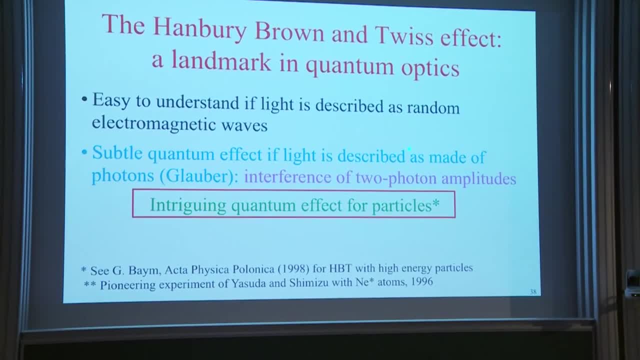 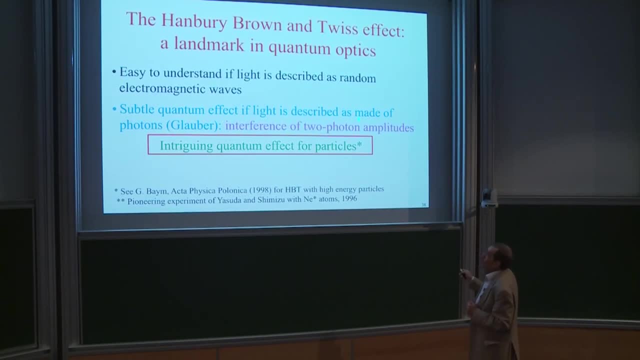 it becomes a subtle quantum effect. if light is described as made of photons, It's interference of two photon amplitudes And Glauber had to develop the full formalism to describe it. I would not say he started from a standard formalism. 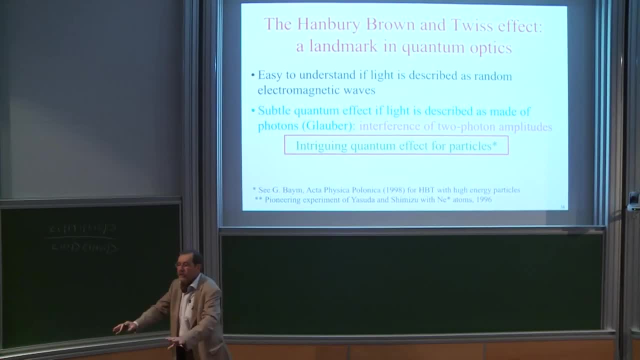 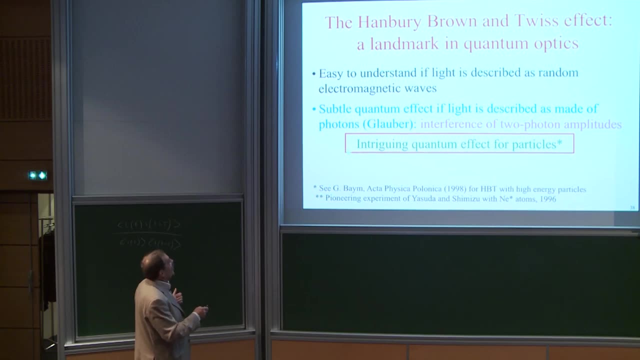 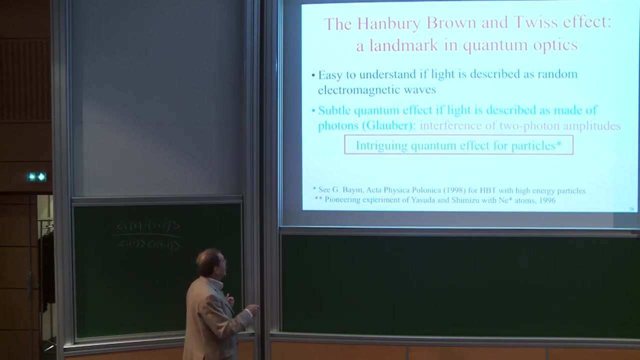 of quantum physics, but he really adapted it specifically to the case of light, these quantum optics, And of course from this we understand that it is an intriguing quantum effect for particles. Okay, And there is a first example of that which is described by Gordon Bain. 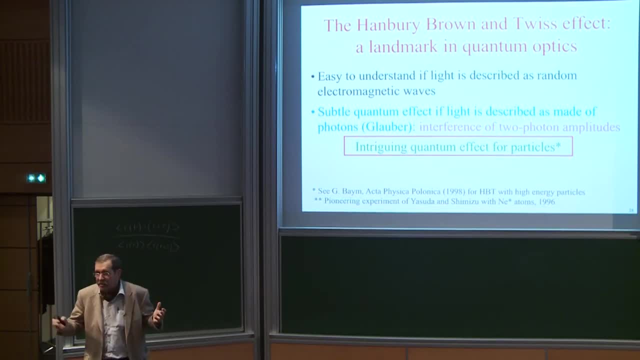 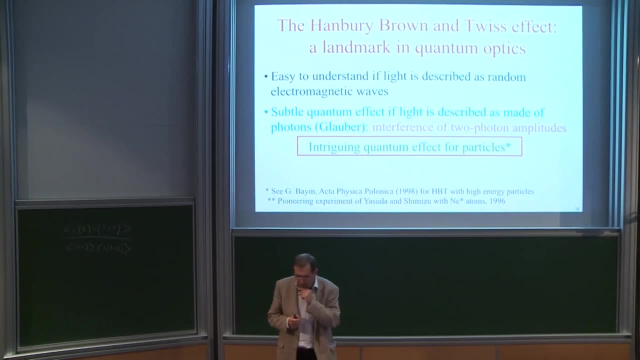 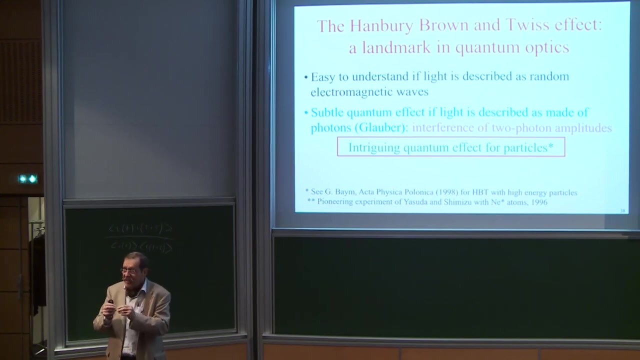 You may know he's a famous theorist. You may know him or may not. It depends on the communities Where he explains that you can use Amber-Hilbryan twist effect for knowing the size of the cross-section of collision between nuclear particles. 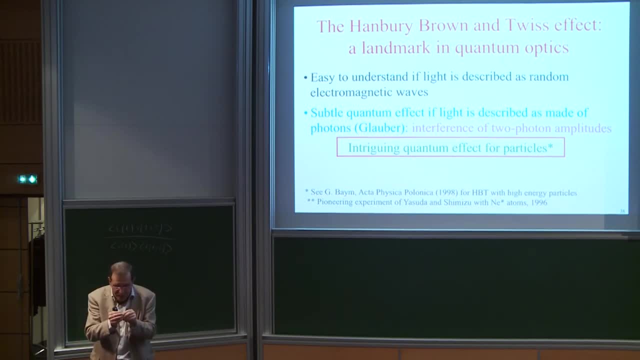 Rather than looking at the size of a star, you look at the size of the cross-section of collision of particles. It works, But anyway. And in our lab- who has a question? can we observe the Amber-Hilbryan twist effect? 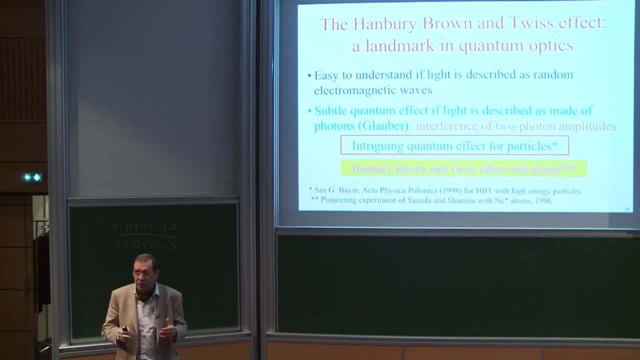 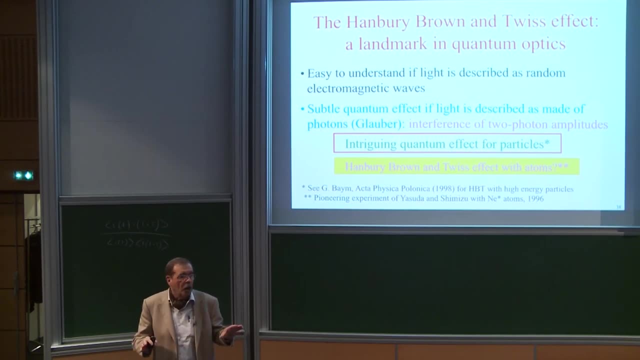 with atoms, Because with particles it's a really interesting effect. So of course I will not talk about all I have planned, but I prefer to go slowly, unless you tell me that I am too slow. but I prefer to explain slowly one thing. 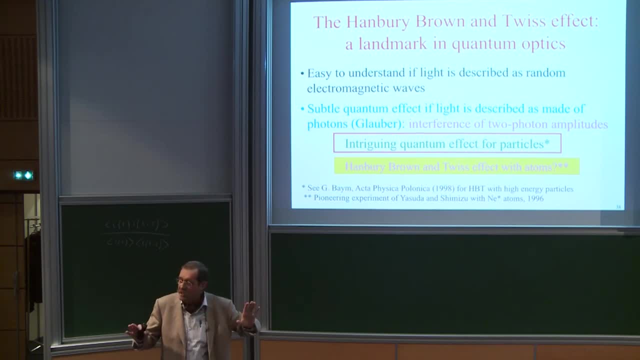 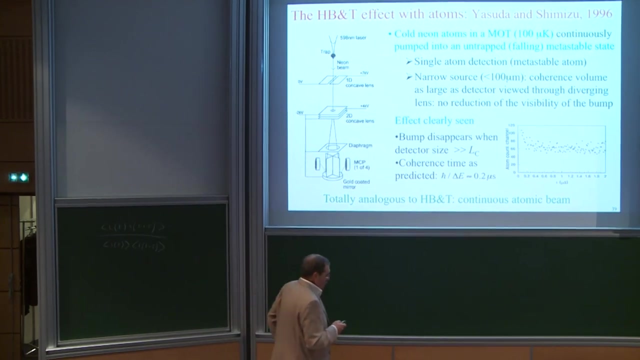 that not explain well many things, Okay. So, if you agree, I continue with this speed, which is not very fast, but I'm using ultra-cold atoms, Which are very slow, So I'm contaminated. Okay, Let us skip that. 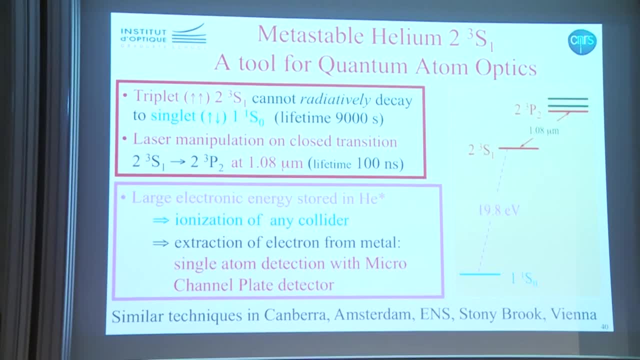 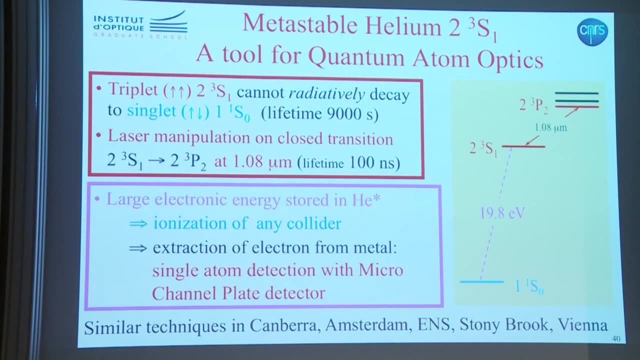 This is technical. So how are we working with atoms and doing quantum optics experiments with atoms? The key ingredient is metastable helium, And I will explain you why. Let us come back to quantum optics. The development of quantum optics is totally linked to the invention. 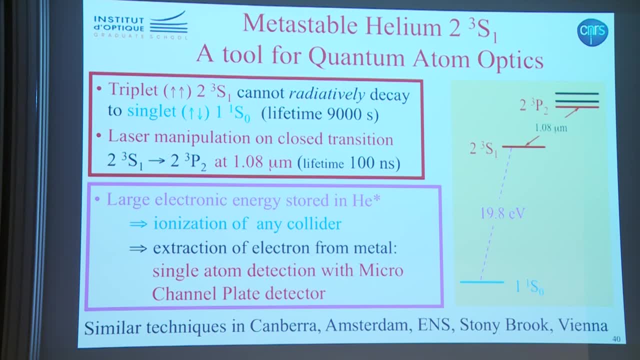 of single photon detection, the photon multiplier, The fact that you can detect one photon, then the next, then the next and look where and when was this photon detected, And then you look at the correlation between two detection events, et cetera, et cetera. 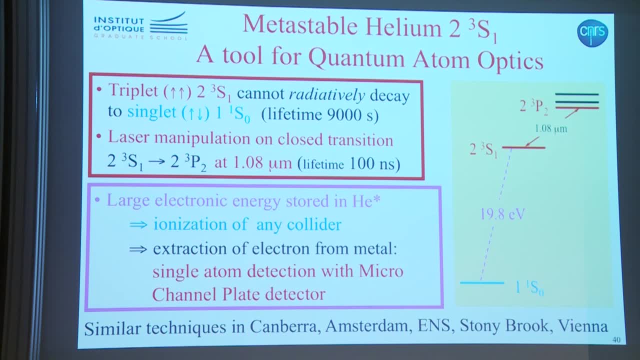 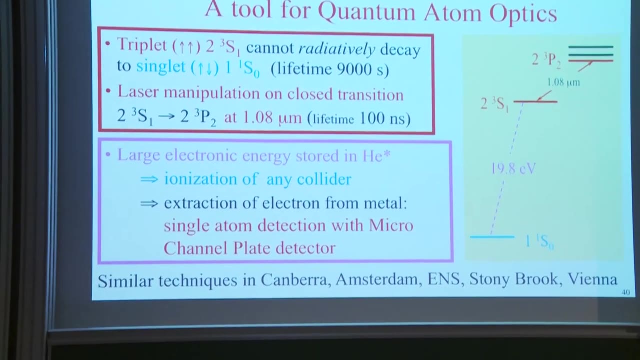 What we have here is metastable helium. It's an atom that we can detect individually for the following reason: Helium is an atom with two electrons, And I'm pretty sure you know that the electron has a spin, So you have states where the two spins are parallel. and states where the two spins are anti-parallel. These states are called triplet states because the spin is equal to one and then you have two possible projections: one zero minus one, While when the two spins are anti-parallel there is only one state. 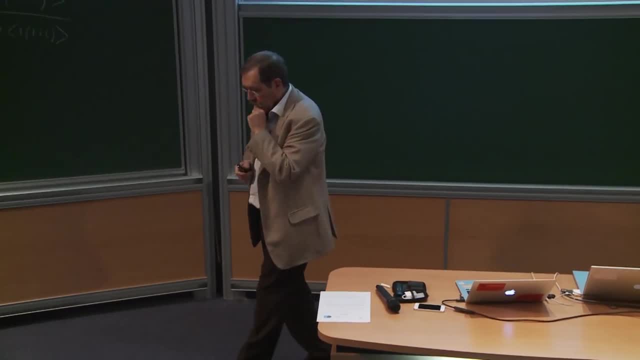 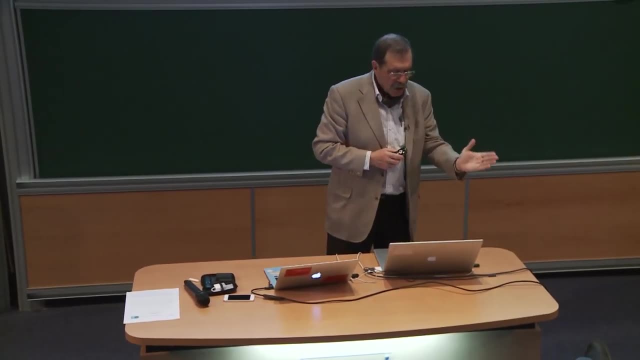 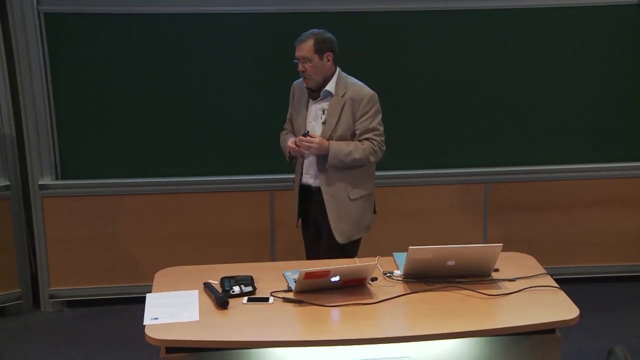 so it's called singlet. Now the important thing is the following: You cannot go from a singlet state to a triplet state by absorbing or emitting a photon. It's called the selection rule, And the reason is that the strong transition with light. are due to electric dipole interaction, And when you flip a spin, which is a magnetic moment, the electric dipole plays no role. So the probability to go from a singlet to a triplet state by either absorbing or emitting a photon is extremely weak. 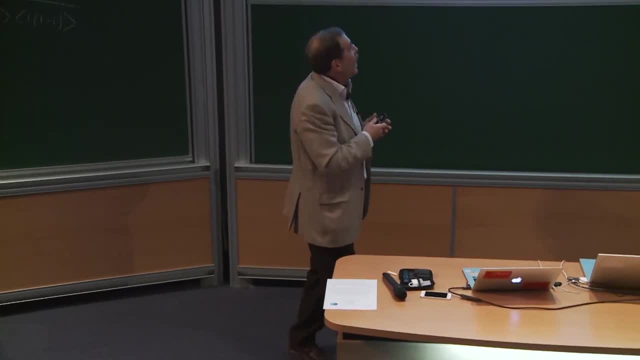 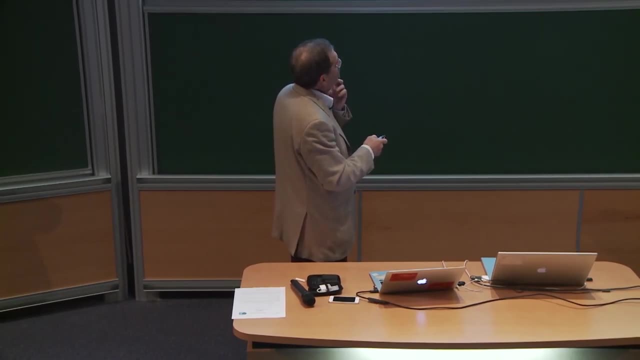 It's not exactly zero, but it's extremely weak, Which means that, in fact, you have two series of levels for helium. You have the levels which are singlet, which are called like that, and there is a full series of levels that I have not represented here. 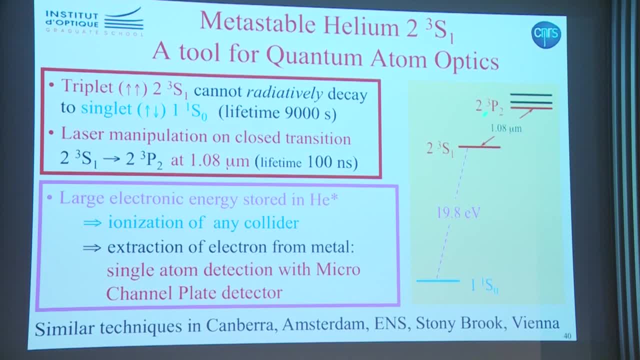 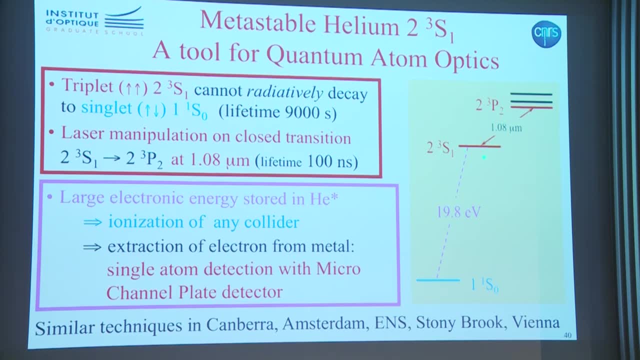 And then you have a full series of levels which are triplet and they don't talk to each other, And it turns out that the lowest level which is a triplet is 20 electron volts above the real ground state. So now there is a story. 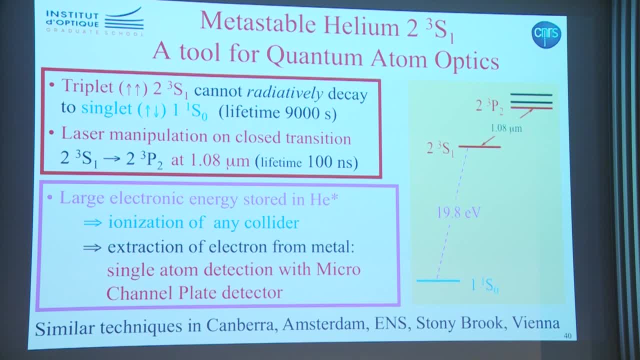 If I start with an atom in any of these triplet levels, by spontaneous emission it will arrive here, and then I can excite it with a laser et cetera, And for all practical purposes this atom is just like an atom. 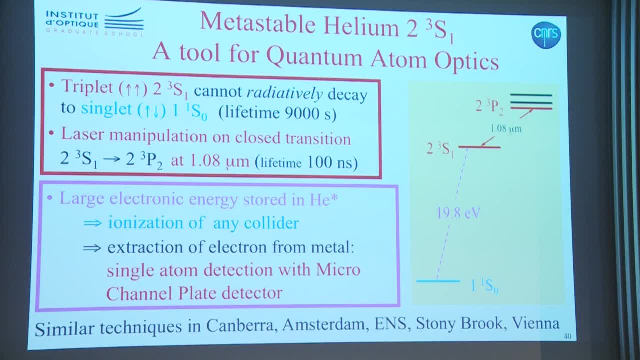 with a ground state here And I can use all the technique of manipulating the atom with laser to decelerate the atom, stop it, trap it, et cetera, playing onto this series of levels. So this is called a metastable level. 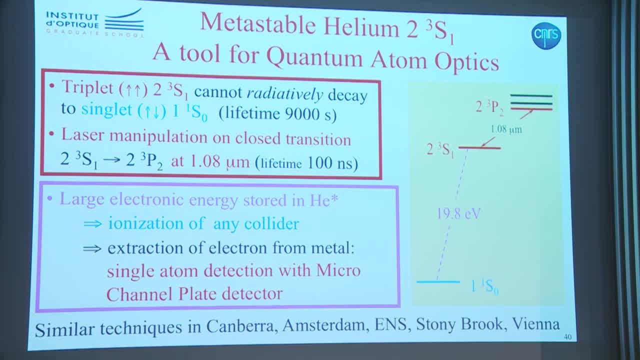 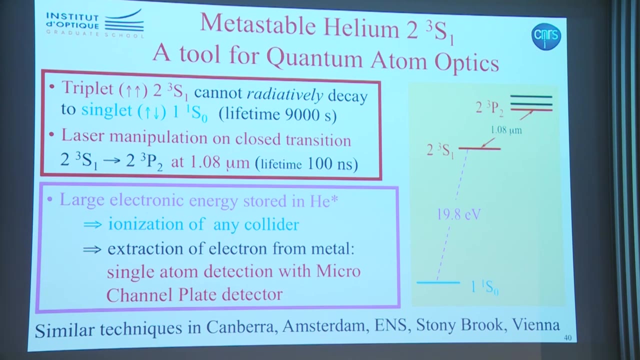 It's metastable because it's almost stable, but the lifetime is, I don't know, hours, But the real ground state is here. Now let's suppose that this atom comes close to a piece of matter. What happens When you are close to a piece of matter? 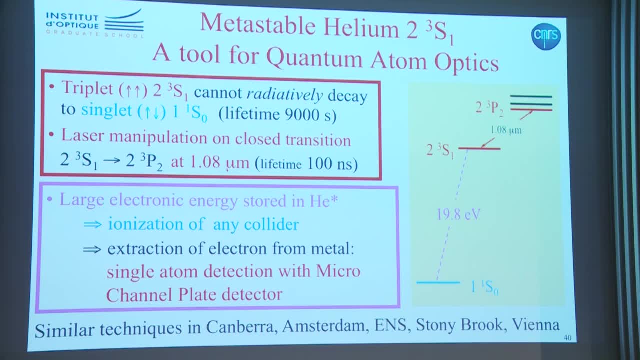 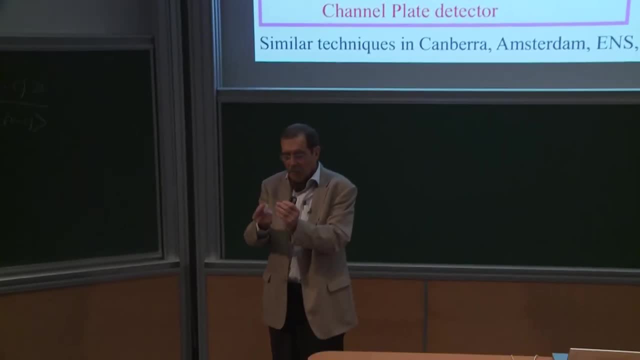 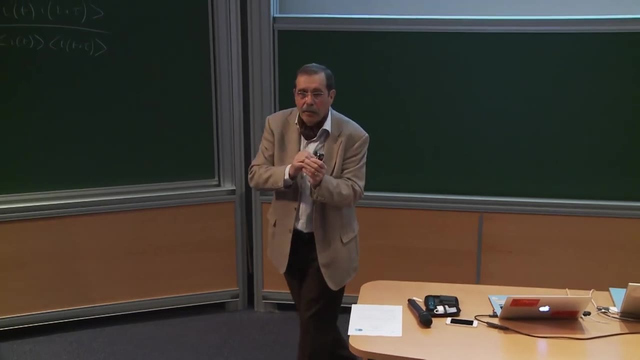 you have an electric field which is responsible for the Van der Waals force. You have some kind of electric field And the electron is moving rapidly In this electric field. And when a charge, an electric charge, moves rapidly in an electric field, 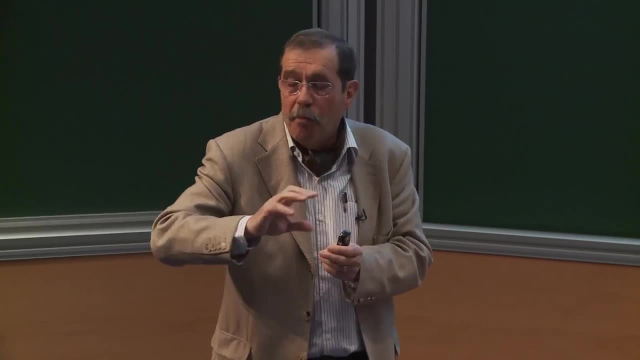 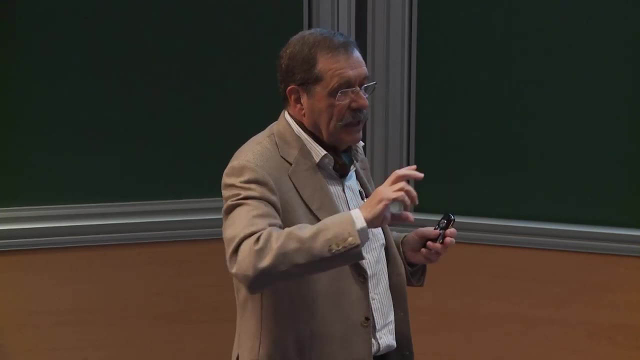 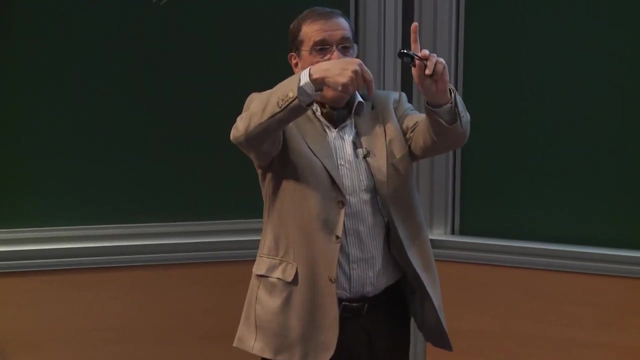 in the frame of reference of the charge, there is a motional magnetic field, And so, because of this motion, there is an effective magnetic field which can flip one of the spins, And if you flip one of the spins then you get in a singlet state. 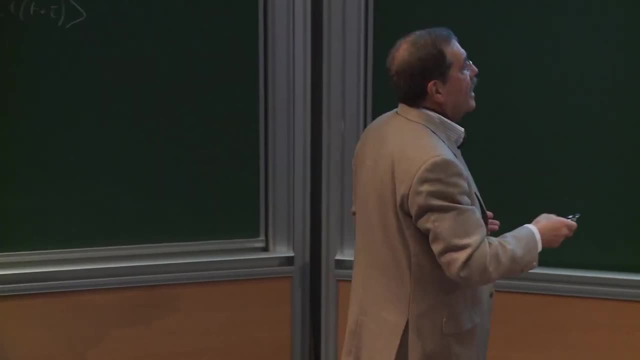 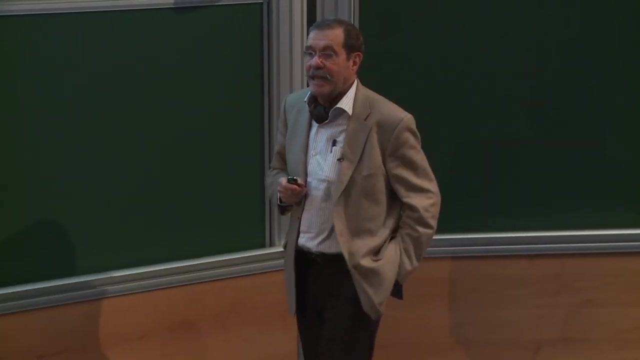 And now there is 20 electron volumes, 20 electron volts available And 20, well, 19.8, almost 20.. 20 electron volts is much more than enough to ionize anything, To extract an electron from a piece of metal. you need 5 electron volts To ionize an atom, a few electron volts To ionize a molecule: a few electron volts. So as soon as an atom in a triplet state comes close to a piece of matter, there is an electron ejected. 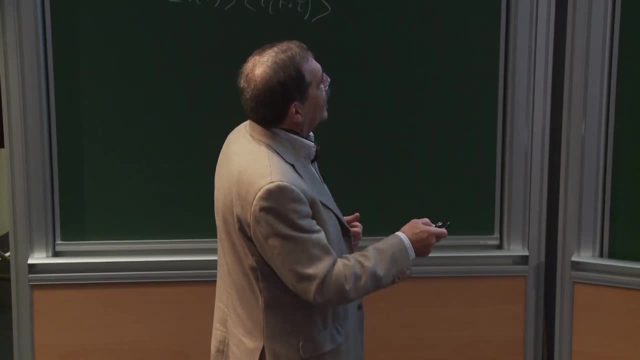 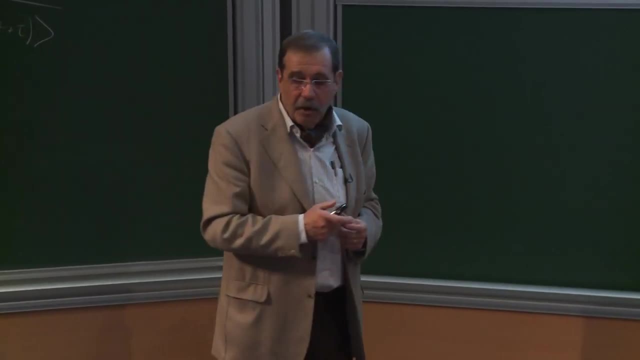 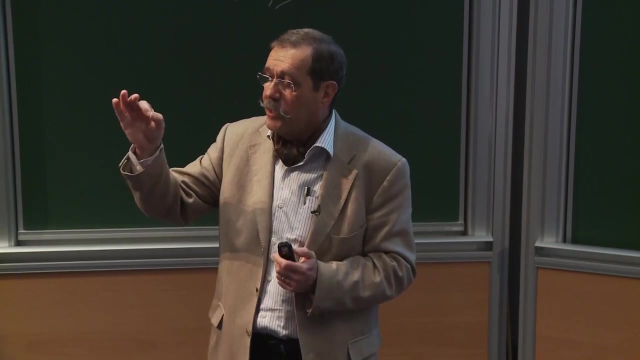 So we can extract an electron from matter, which will allow us to make single atom detection. Because remember what is a photoelectric effect? It's the fact that when a photon arrives on a plate of metal, one electron is ejected. 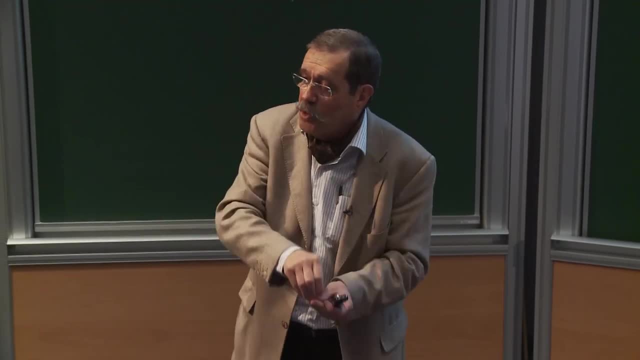 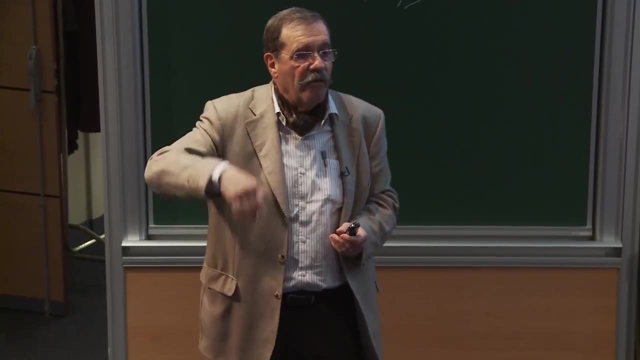 We have exactly the same process, So we can use the same trick, that is to say accelerating this electron, bumping it on a die knot and having a multiplication, And at the end we have a pulse of 10 to the 10th electron. 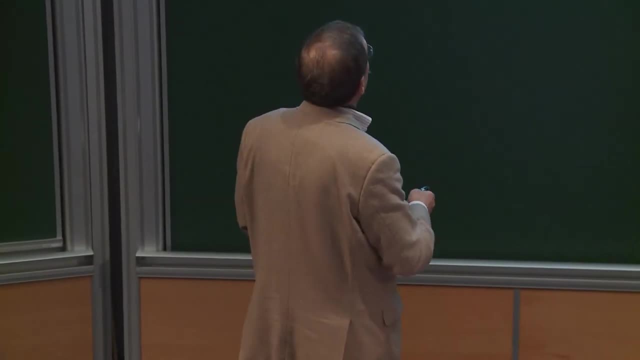 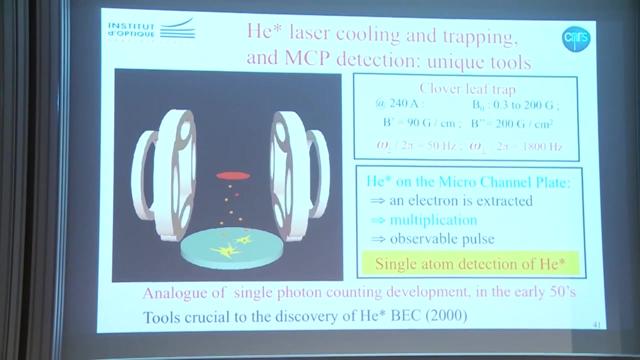 And this we can observe. So this is how it works. This is an artist's view. We have our metastable helium atoms which are trapped here with coils And they drop, And each time they arrive on a piece of metal here. 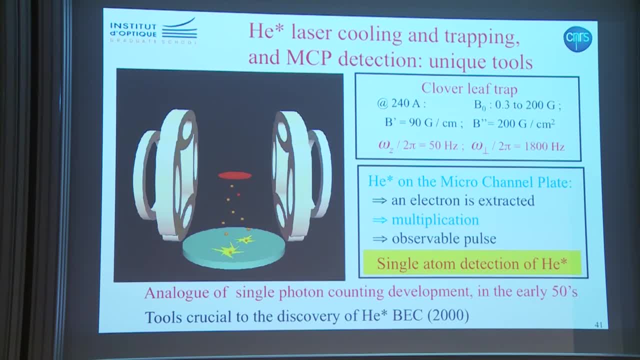 boom, there is an electron which is ejected. In fact, this is not a piece of metal. This is what we call a microchannel plate. It's millions of very, of very small tube which pass through the plate. Each of these tube is an electron multiplier. 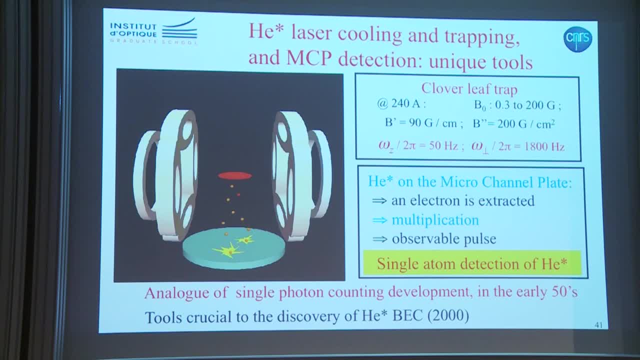 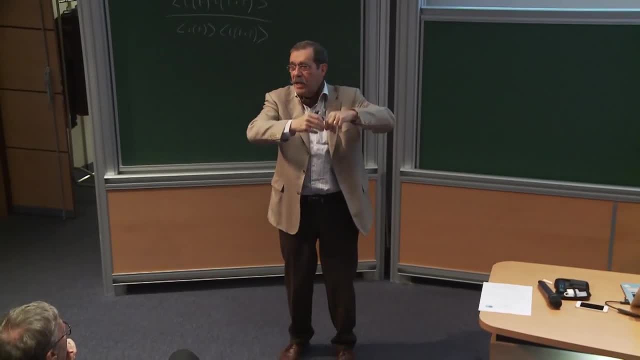 You have two kilovolt voltage difference between the upper part and the lower part And when an electron is emitted here it bounces on the walls and there is a multiplication factor each time it bounces on the wall. So if you have a factor of three, 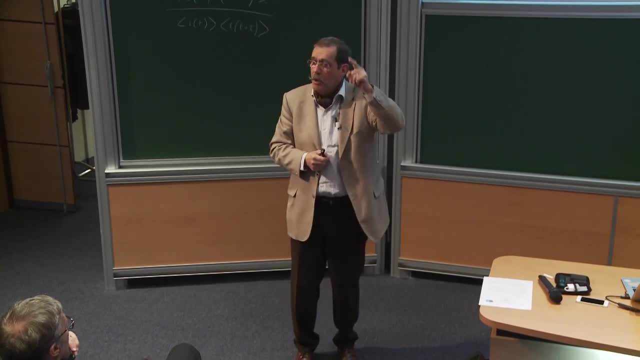 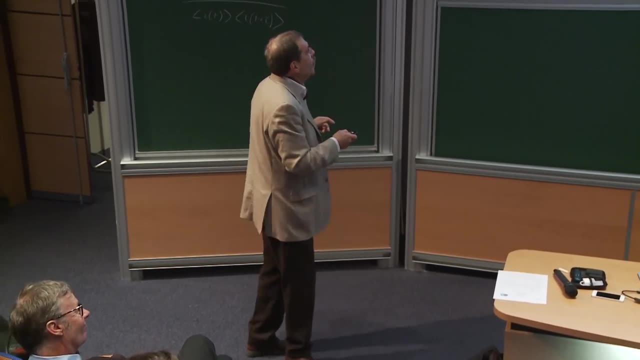 if you bounce 10 times, you have three to the power of 10, which is a lot. Okay. It's probably like two to the fifth or something like that. Okay, So now what we have on the other side? we have a macroscopic pulse. 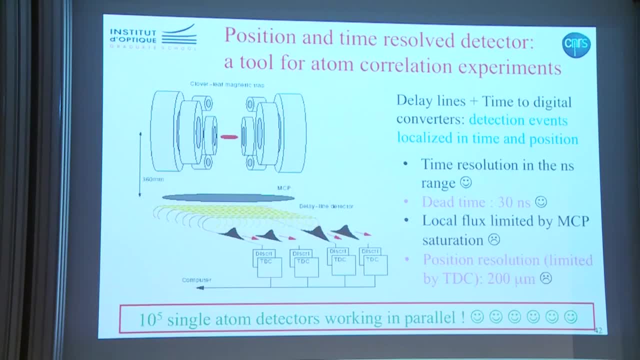 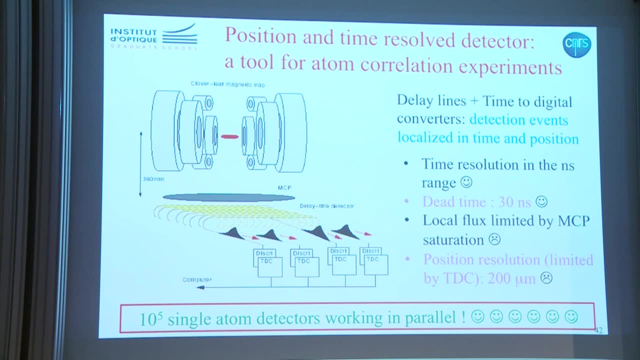 each time an atom arrives. here We have done yet better, And this is even better than photomultipliers, Because what we have done is, rather than just registering the fact that we have detected one atom, we can tell where the atom arrives. 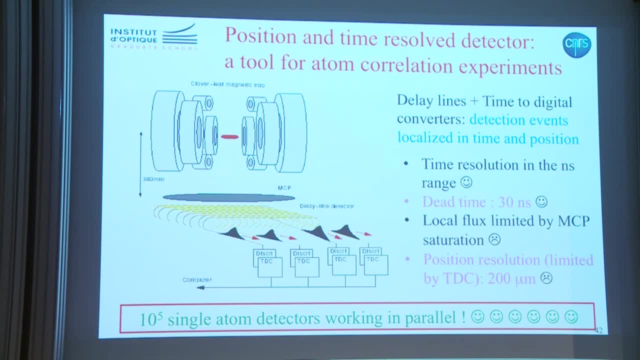 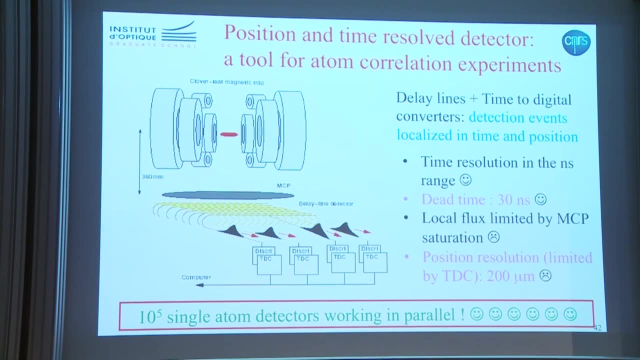 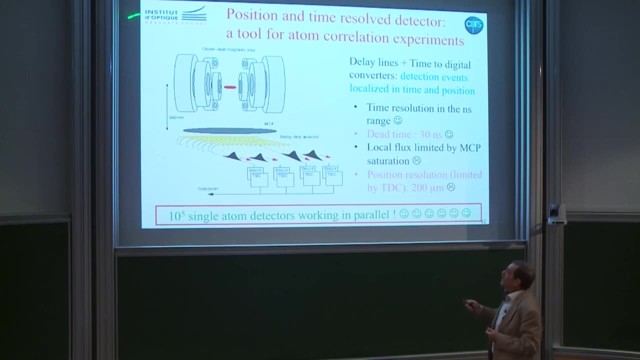 Because here we have delay lines and when the charge arrives here it's split along delay lines And by looking at the delay at the end of the lines we can tell where the atom was detected. So now we have a detector which is allowed to tell us where and when. 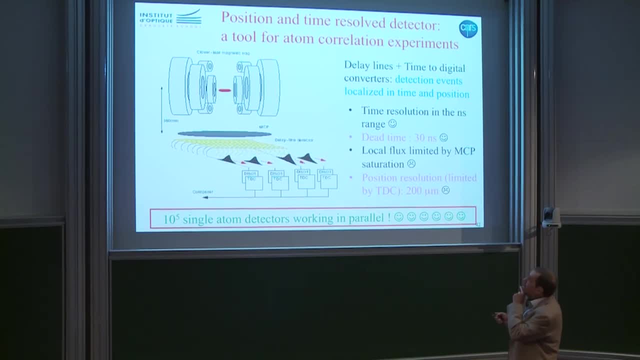 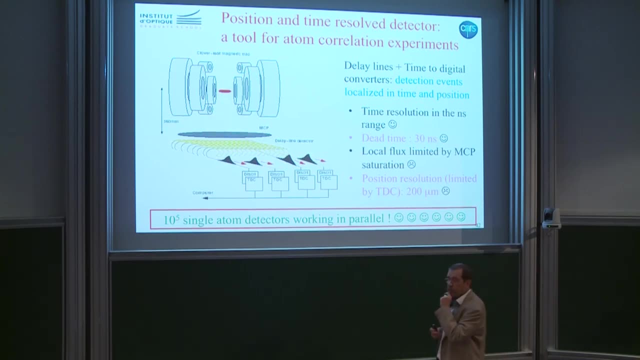 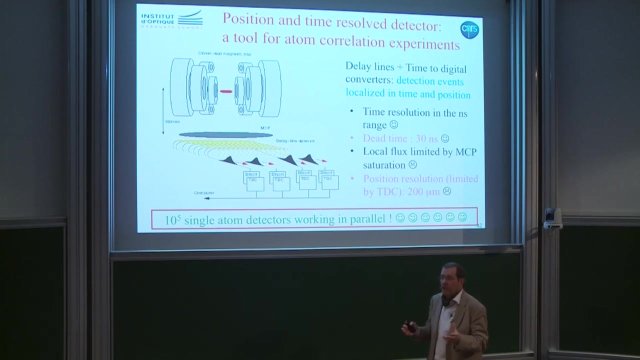 the atom was detected. And if you think of it, in fact, you discover that our two-dimensional detector is in fact, in our experiment, a three-dimensional detector. Why? Because we have cold atoms here with very small initial velocity. You drop them. 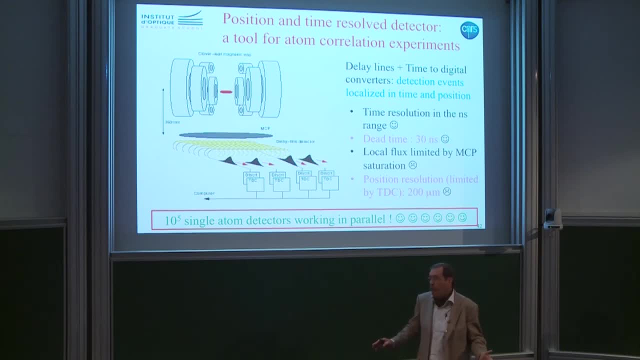 When they arrive on the detector, all of them have about the same velocity. So by looking at the time of arrival you can reconstruct the third dimension. So in fact this allows us to describe the full distribution, volumetric distribution, three-day distribution of the atom. 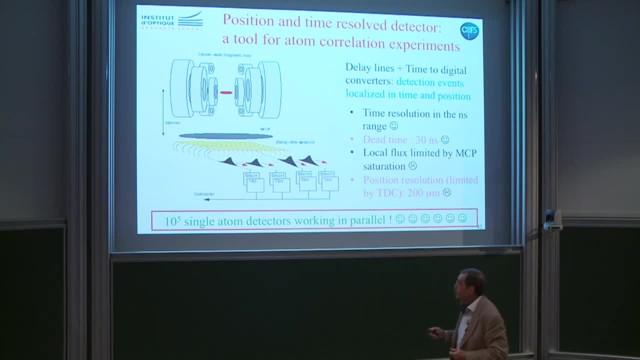 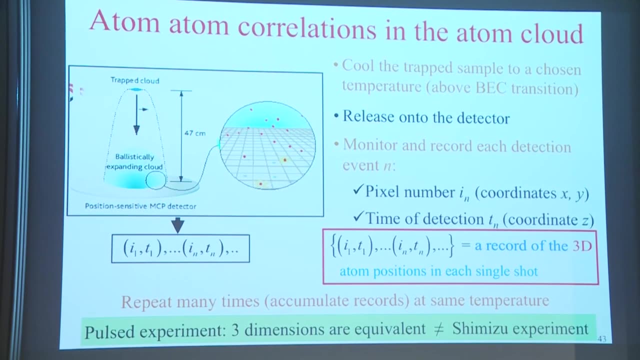 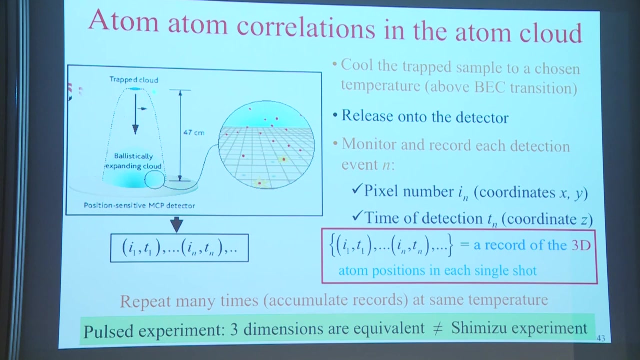 just before they fall on the detector here. So we have repeated the experiment, which is not exactly the Amber-Iberian twist, but very similar to the Amber-Iberian twist in the following way: We have a trapped cloud of cold atoms. 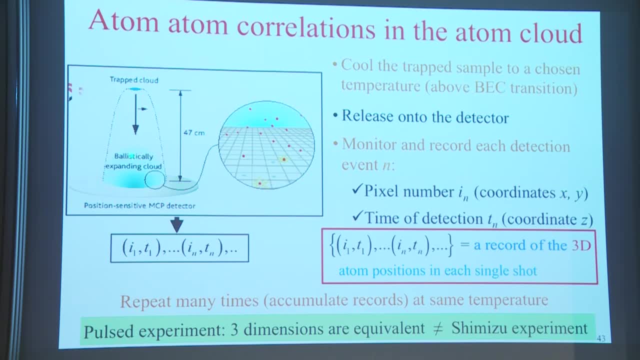 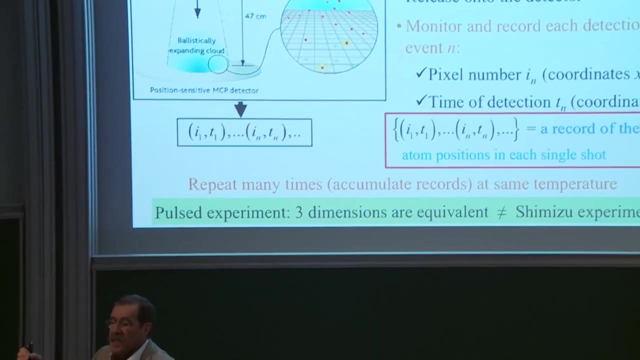 We drop them And when they arrive we detect all the arrival position and time. And so we have a set of points here, And with this set of points we build the correlation function, That is to say the histogram. what is the number of pairs? 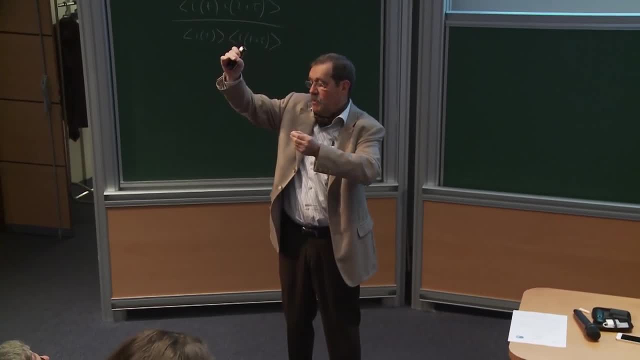 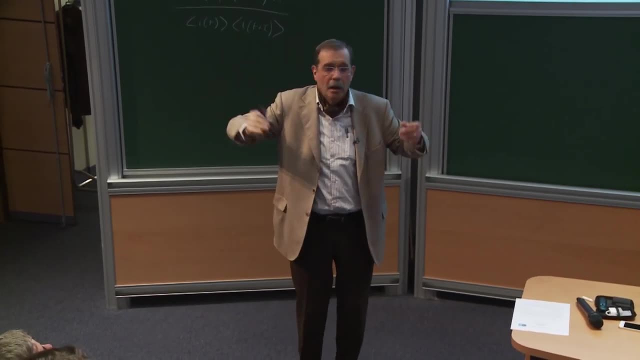 which are separated by this vector in the three-dimensional space, And the result is only noise. Most of the time is zero, From time to time is one. So we repeat the experiment and we build the histogram again. We repeat this experiment. 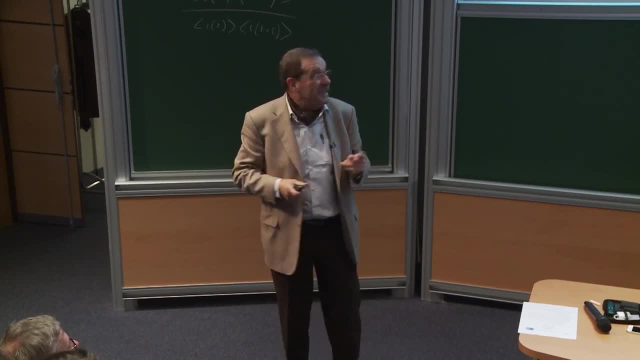 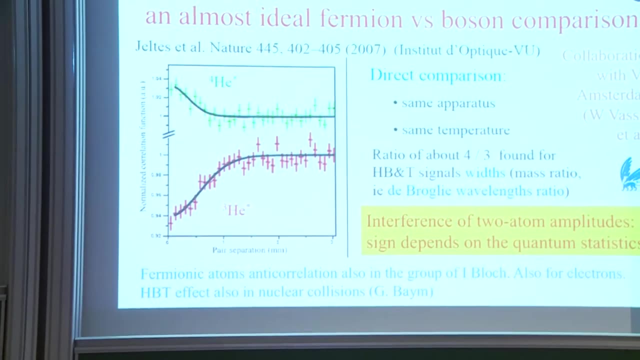 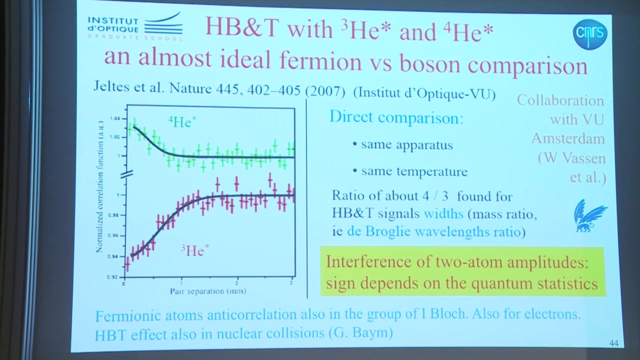 we build the histogram again And at the end we make the average of the histograms. And when we make the average of the histograms, this is what we get. And again, I repeat, we don't average single events On each pattern. 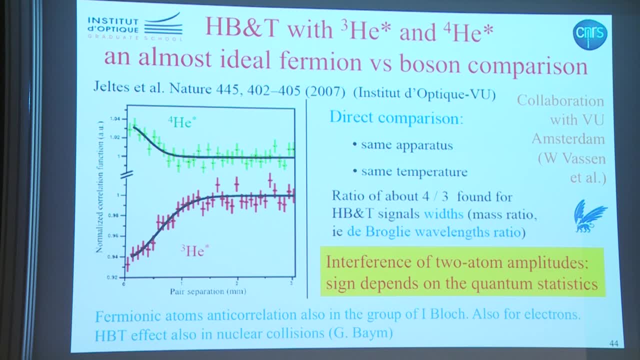 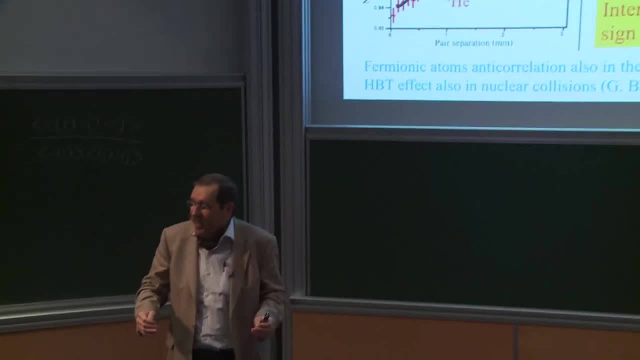 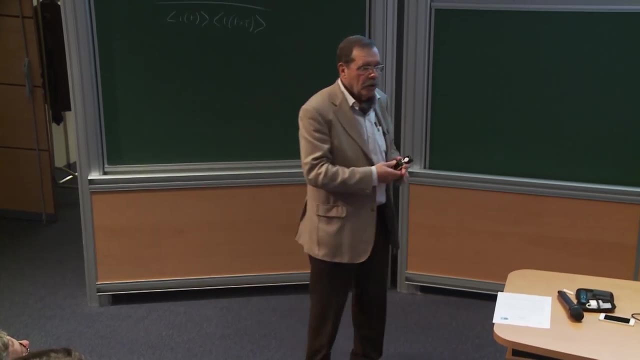 these are fantastic experimental techniques. You have noise. You look for a correlation in that noise. It's still noise, But if you average the correlation, then you get a signal. If you average independently it doesn't work. Okay, when you think of it. 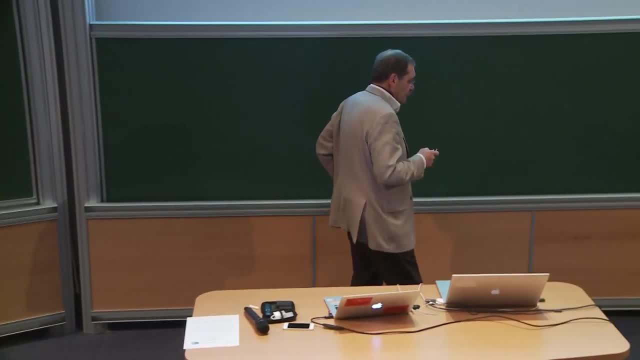 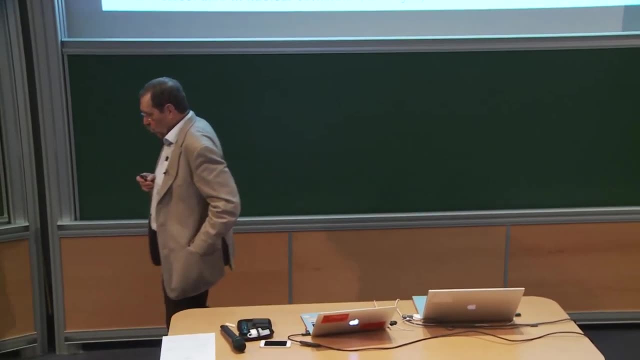 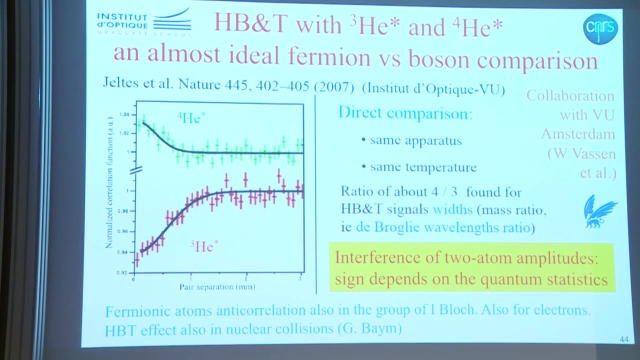 it's trivial, but it's beautiful. Now you see a second curve, And the second curve allows me to say why atoms are even more. Sorry for that. The other important difference between photons and atoms is that all photons are bosons. all photons are bosons. 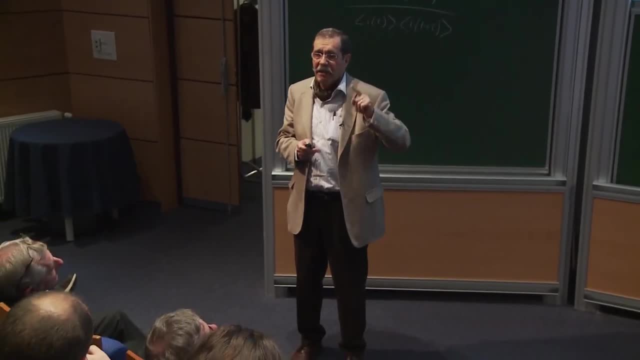 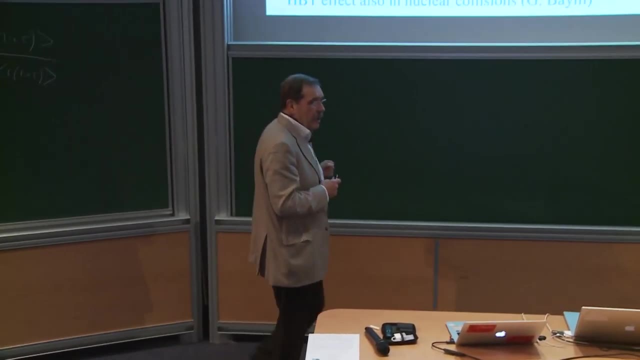 while four atoms are bosons and are fermions. For instance, in the case of helium, helium-4 is a boson, but helium-3 is an atom. So helium-3 is a fermion And, if I repeat the reasoning, 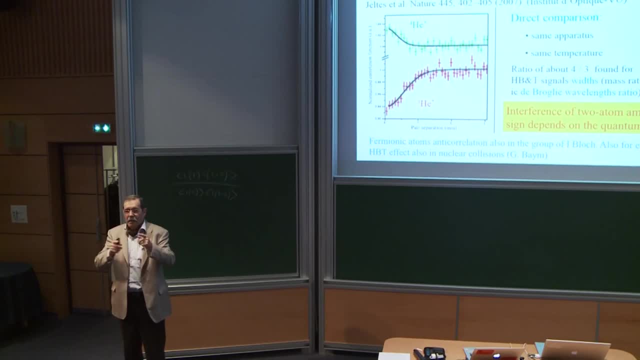 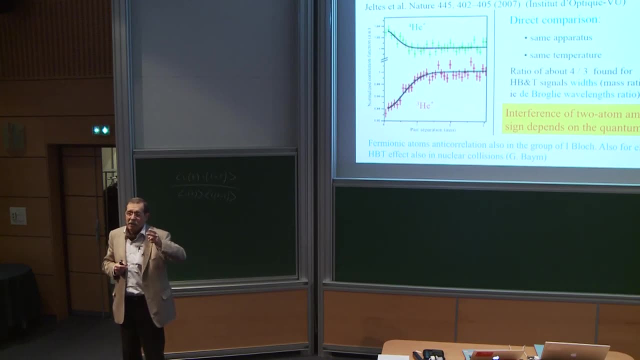 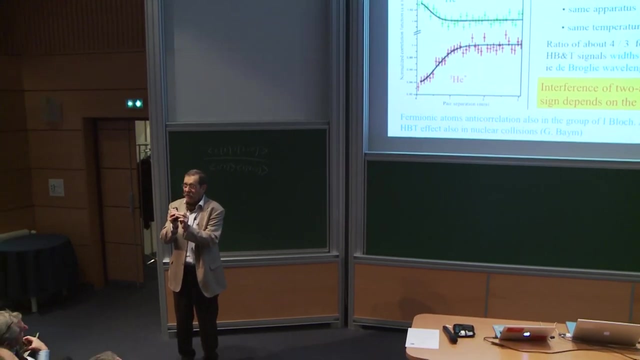 of Ambery-Brine twist with fermions. when I add the diagrams, I must add them with a minus sign, which means that the interference, rather than being positive, will be negative, which means that the probability of two fermions to be on top of each other. 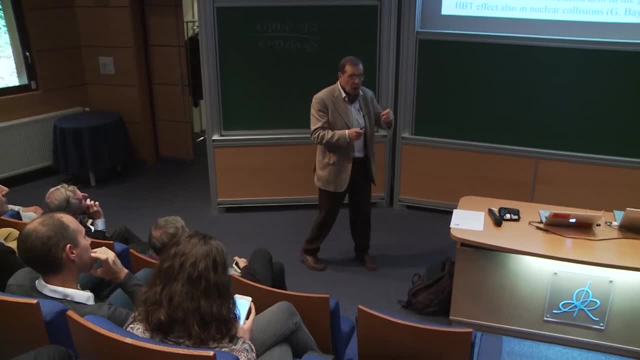 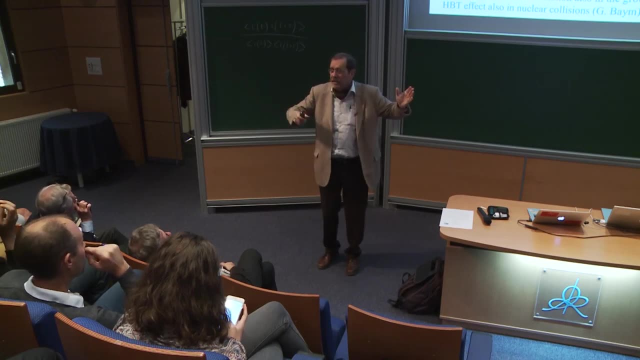 is small, is null, but nothing is perfect. This is well known, It's called the Pauli principle, But you have it directly as a consequence of the same reasoning that I did, And we have done a fantastic experiment in which we have a sample. 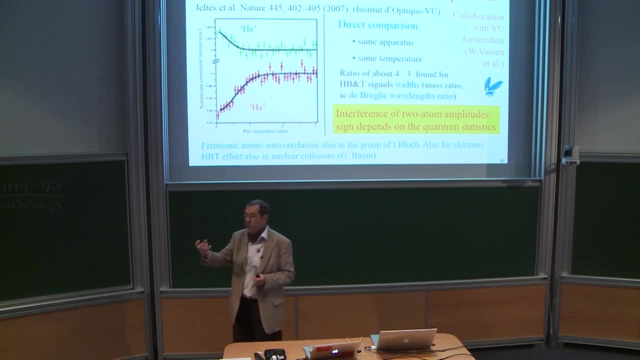 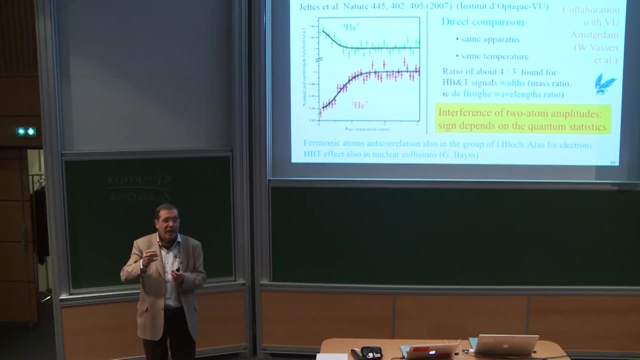 in which we have helium-3 and helium-4.. They are the same temperature, nanokelvin temperature, et cetera, same size of sample and we can at will decide to drop either helium-4 or helium-3.. 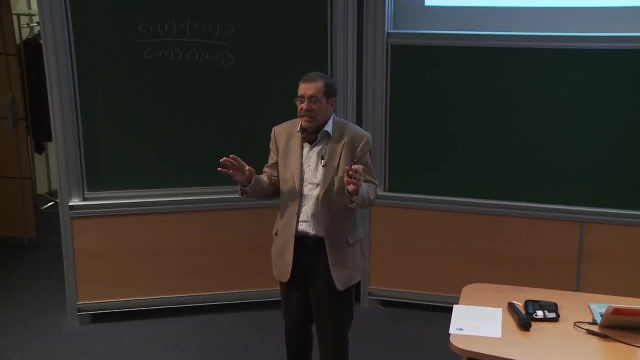 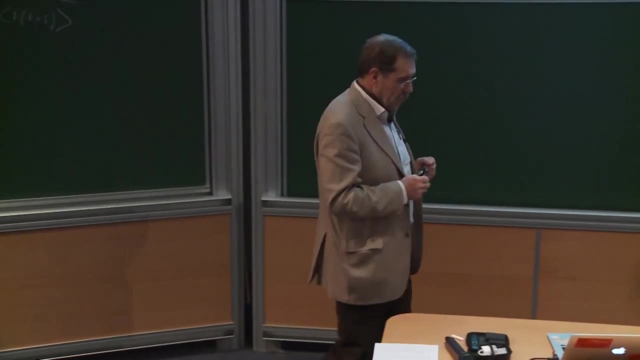 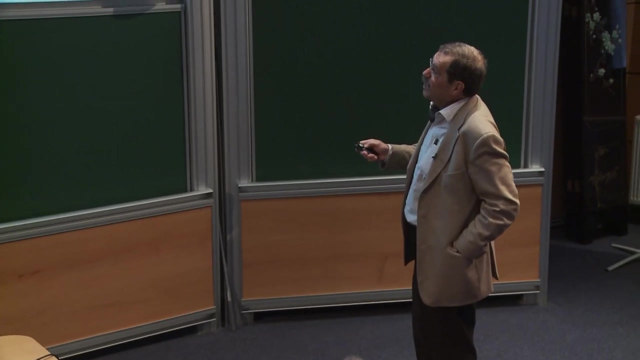 And so we can compare only the statistics. All the other parameters are the same and we see the difference. Now I have a joke I like to make, So I'll tell you. It will be a joke Here. the size of the hole is different from. 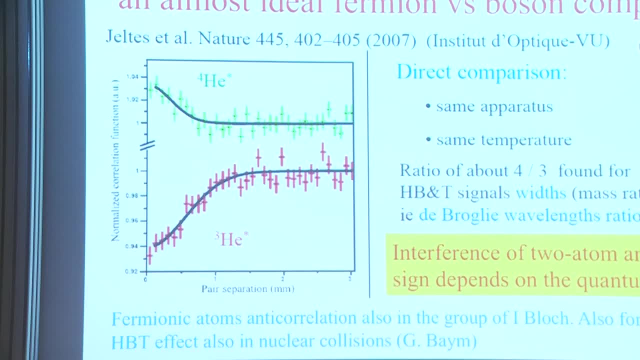 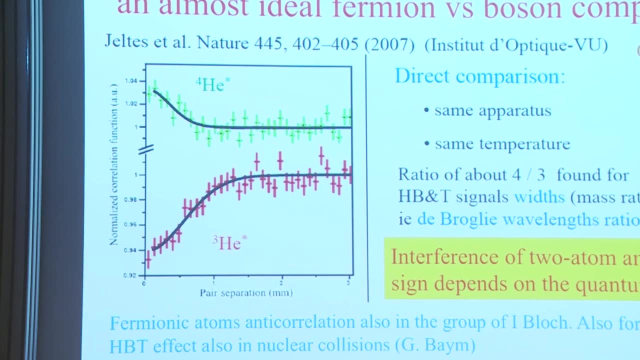 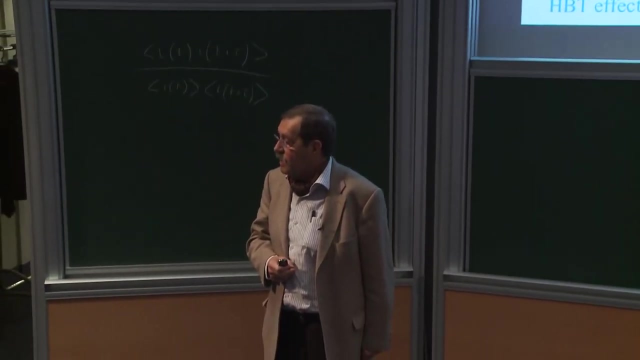 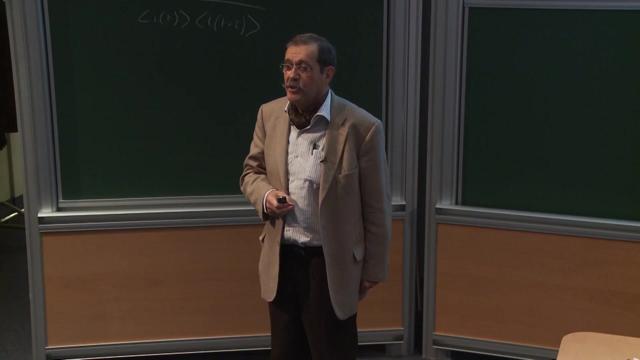 or the size of the bump is different from the size of the hole which is here. Why is it so? Because helium-3 and helium-4 do not fall the same way. Yes, Now objection, objection. Galileo told us: everything falls the same. 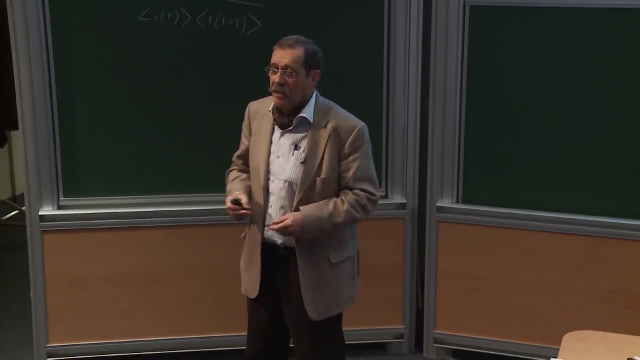 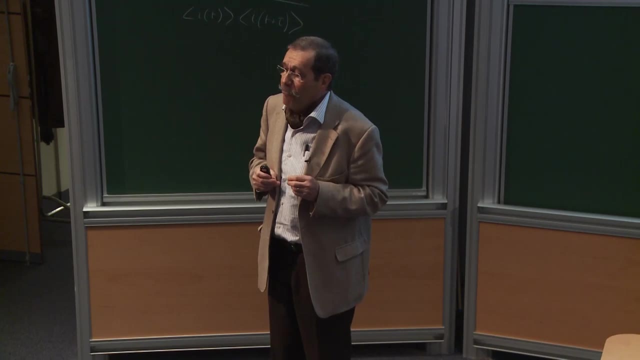 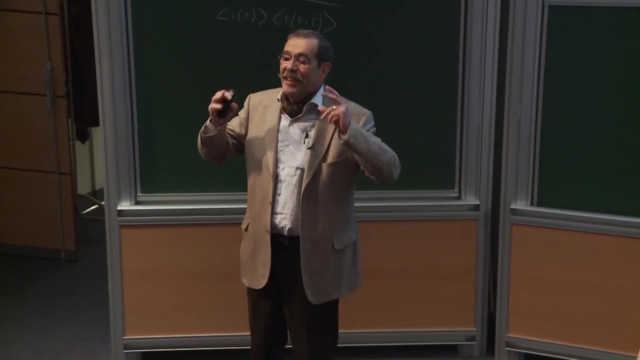 Okay, let me explain better. They indeed arrive with the same velocity, but because they have different masses, the de Broglie wavelength are different And the size of the hole can be related to the de Broglie wavelength. So, in the quantum sense, 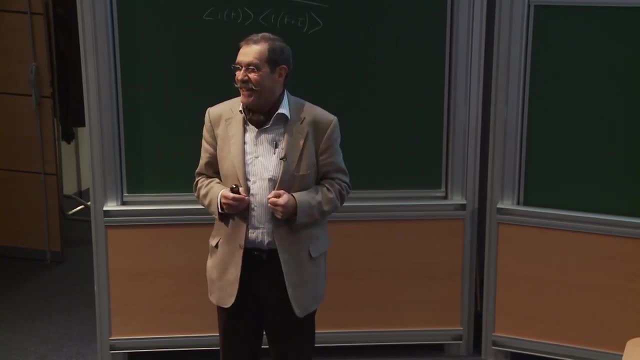 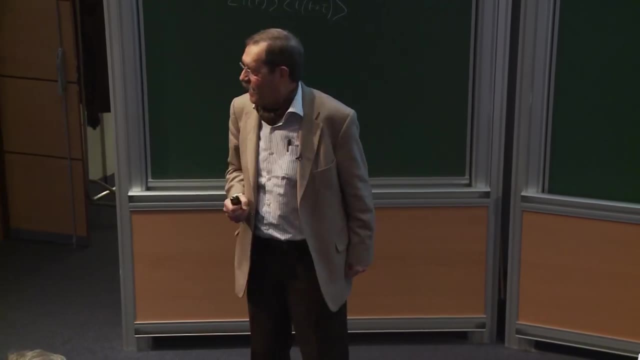 they don't fall the same. They have the same velocity, but the de Broglie wavelengths are not the same. Well, I like to provoke people When there are Italian people, usually they defend Galileo And I defend Du Bois because I'm French. 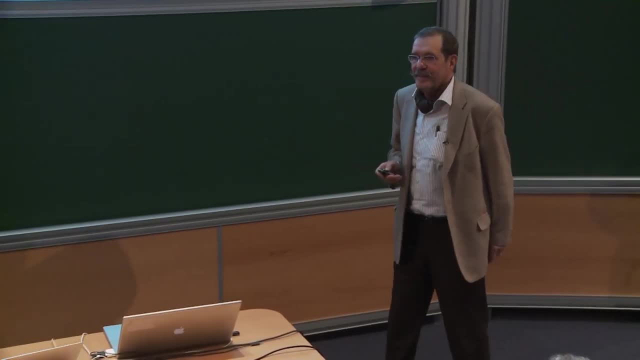 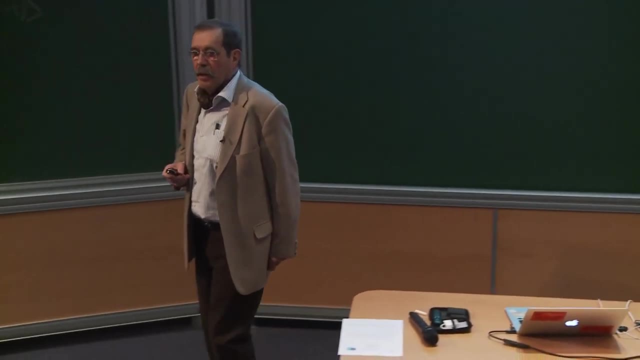 Good, I thought something you said was ratio is 4 over 3.. It's not related to helium-4 and helium-3.. Yes, the ratio is 4 over 3.. And helium-4 and helium-3, it's the same 4 over 3, yeah. 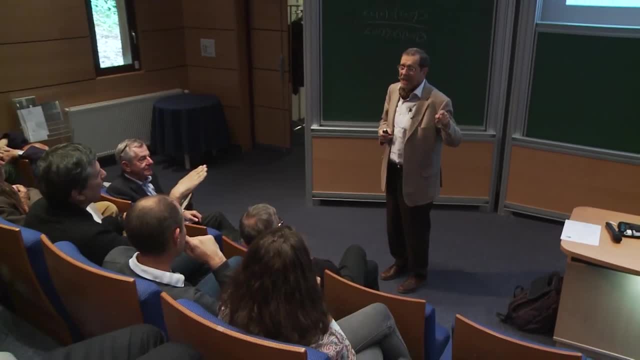 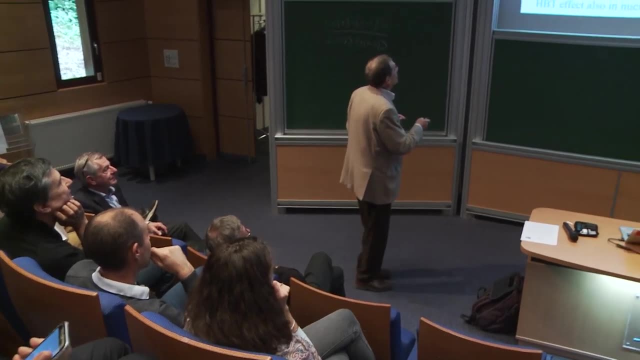 Yes, because the de Broglie wavelength is inversely proportional to the mass. for the same, The curve goes up and down because it depends on fermions and bosons. No, okay, Up and down because fermions and bosons. But now the width. 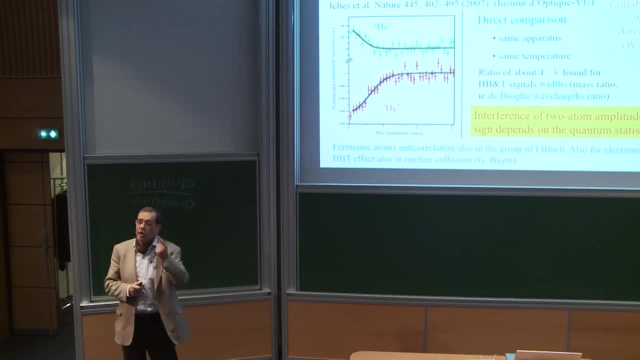 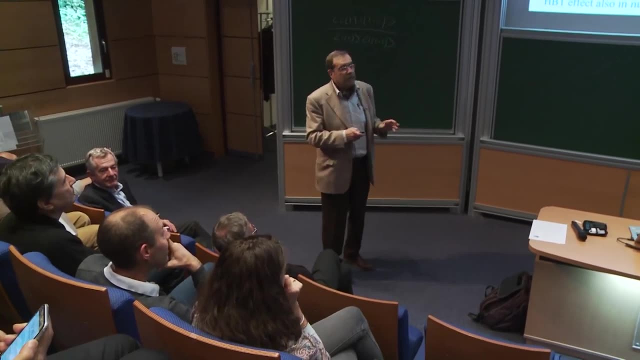 look at the width: here The width is bigger and the width is bigger because the de Broglie wavelength is bigger by a factor 3 to 4. And I should ask that the contrast is less here as bigger here, because when you make a convolution, 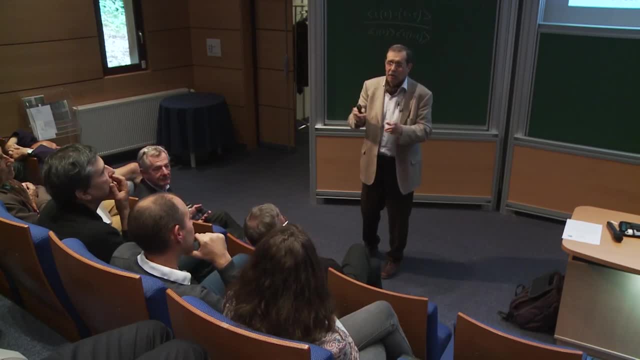 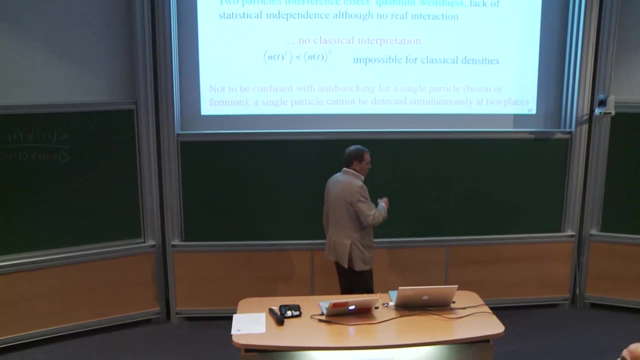 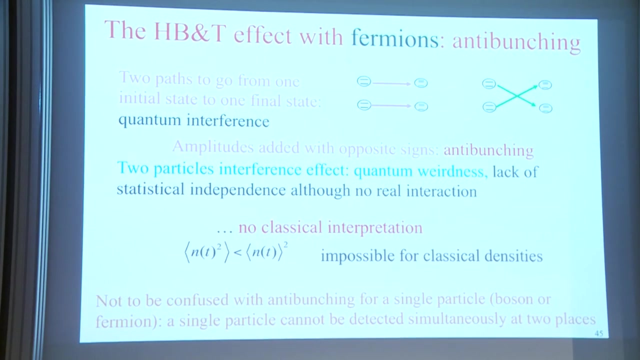 the visibility, the contrast of the convolution depends on the relative width. But this is technical So I don't know. I can talk for hours, okay, So at the end of the day, the Ambry-Brown effect with fermions. 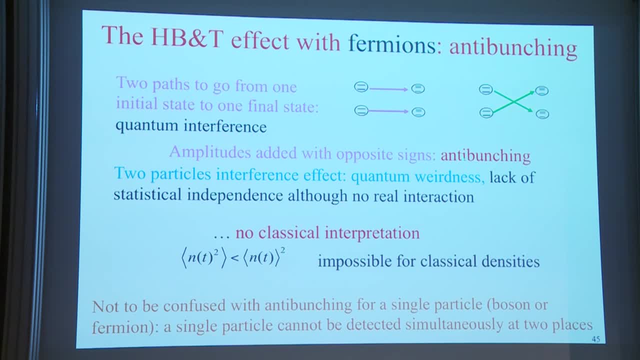 which can be interpreted by subtracting the diagram which is here, leads to the conclusion that the average of the square is less than the square of the average, And this is not classical at all. okay, There is this, of course. formula is stupid. 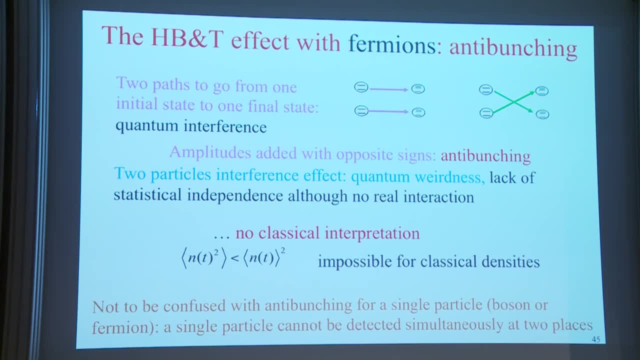 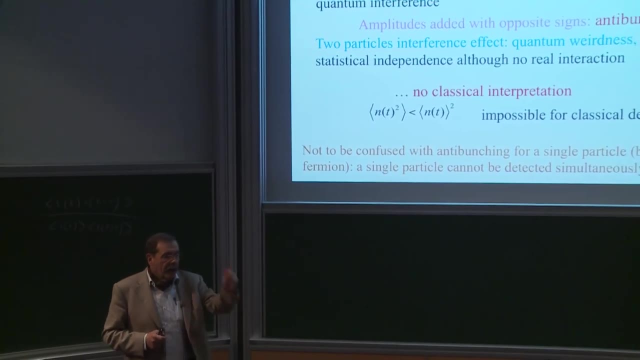 if it is classical numbers. But in fact in real quantum physics here I must use second quantization. So I must use operator of creation and annihilation. And if I replace n by creation annihilation operator, then because of the commutation relation of fermions. 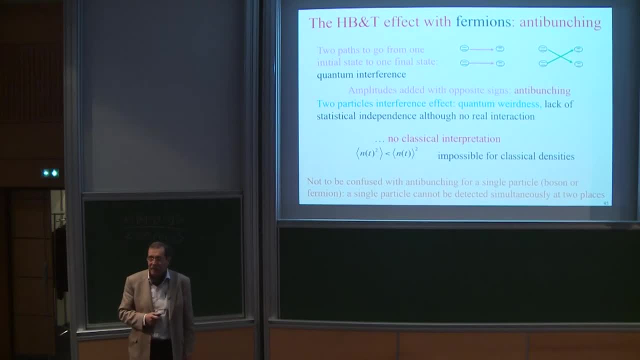 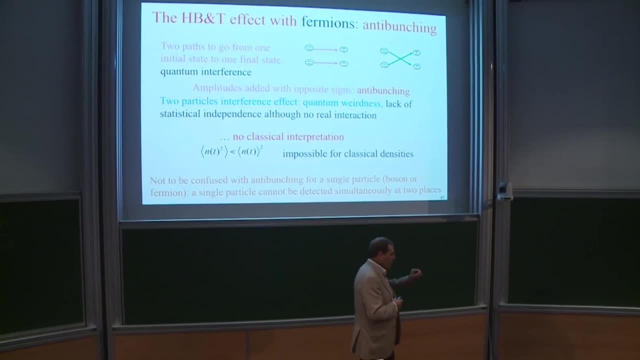 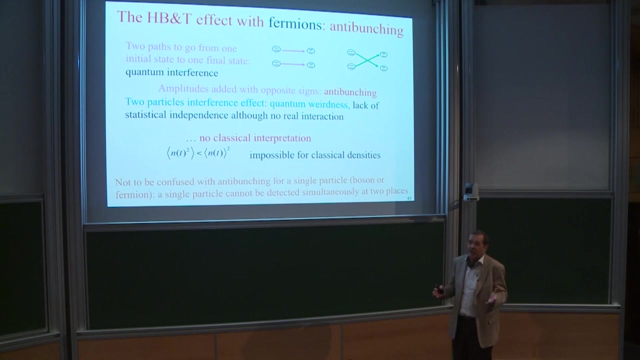 this becomes possible. So, from this point of view, if you compare for photons and for fermionic atoms, for photons, of course I can describe it with quantum physics, but, if I insist, I can describe it with classical physics, While here, 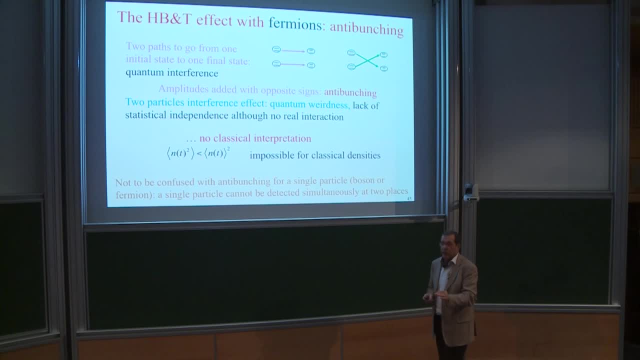 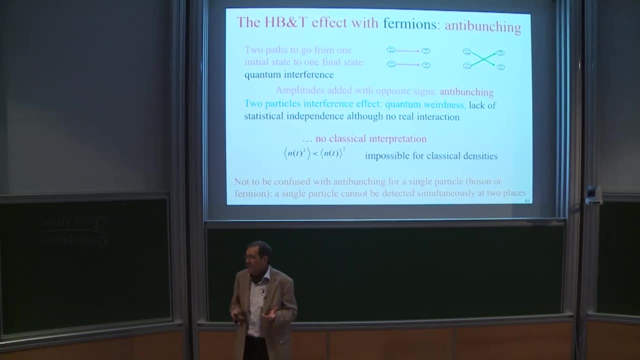 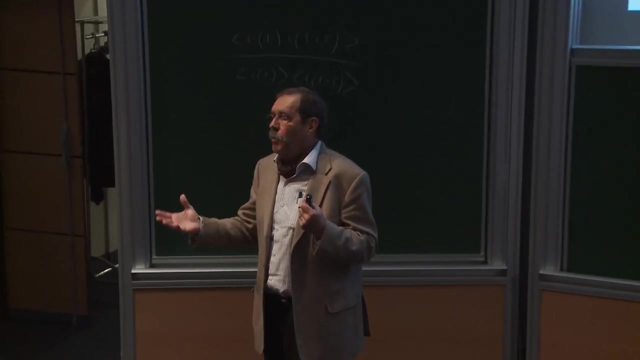 there is absolutely no classical explanation. So in this sense, fermions are more quantum than bosons. I think that it is true because, in fact, all classical waves, as we know them, get their properties from the fact that you can make many bosons. 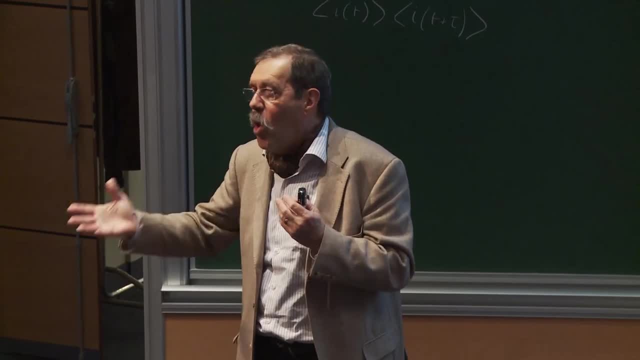 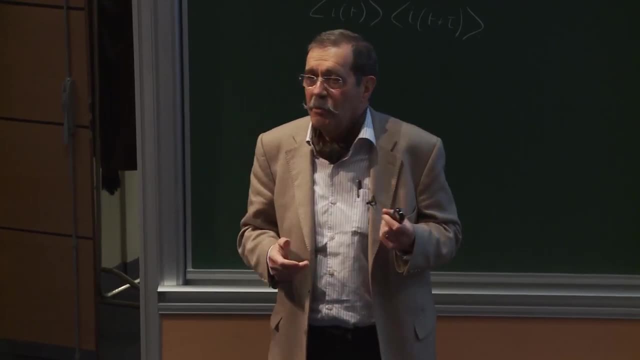 in the same wave, in the same mode, elementary mode of the electromagnetic field, And at this point you get a macroscopic wave. You cannot do that with fermions, With fermions when you have put one in an elementary mode. 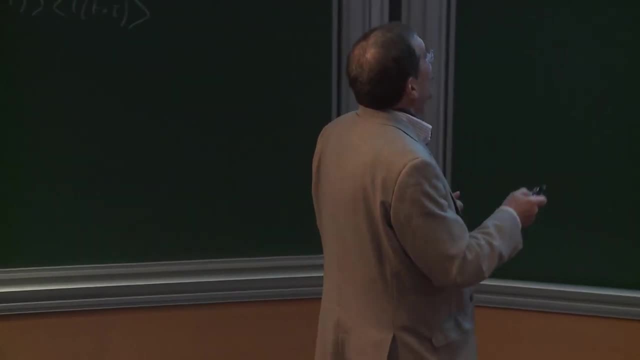 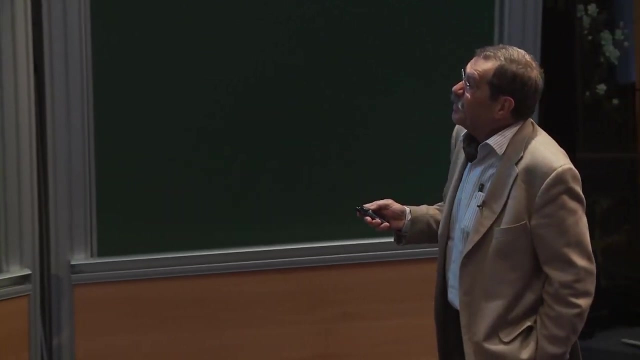 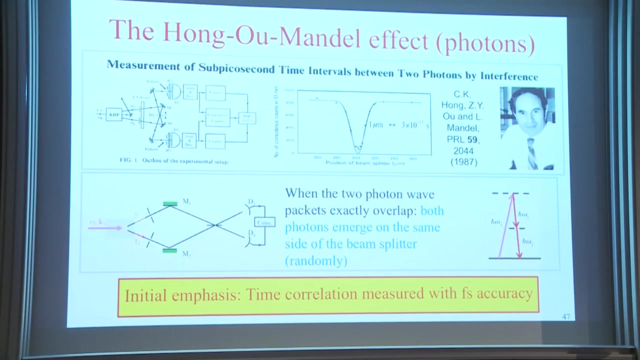 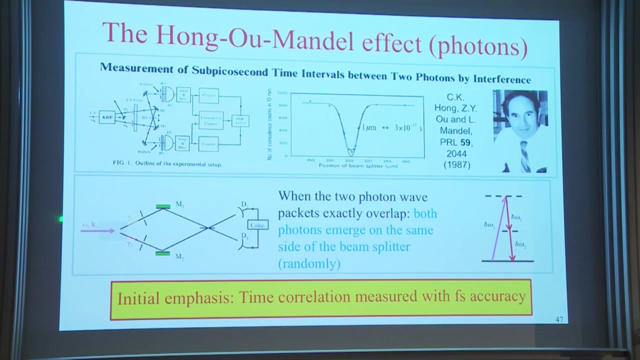 that's the end of it. Okay, I will describe the Ongo-Mendel effect and I think it will be enough. The Ongo-Mendel effect was discovered in 1987.. And you have a complicated experiment, but you can simplify the script. 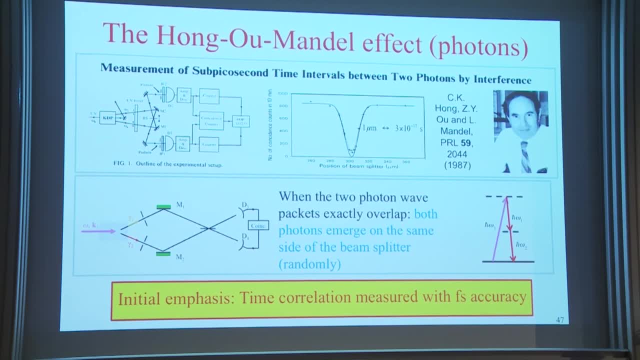 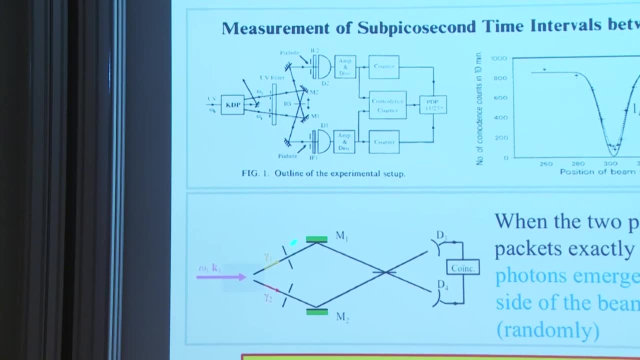 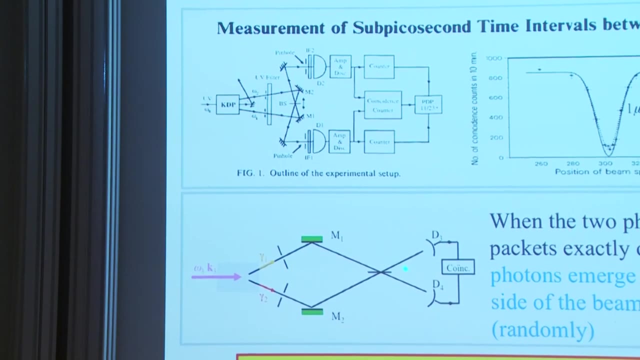 to understand better. And the idea is the following: Here you create pairs of photons- And the two photons are well isolated, here with diaphragm, et cetera- And you join them, you combine them on a beam splitter. here: 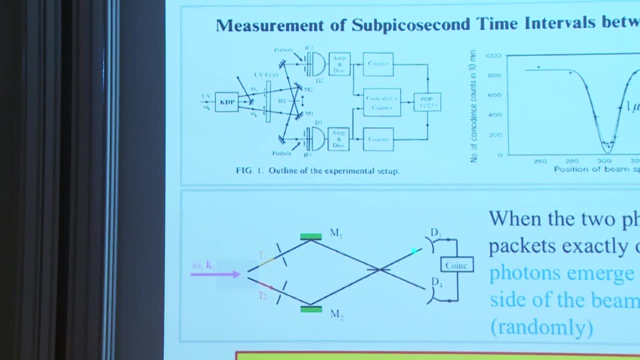 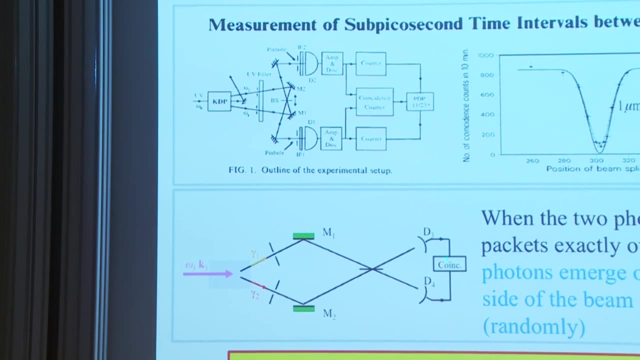 So you have a pair of photons and you combine them on a beam splitter And now you have a single photon detector and you look for correlation. So you look for coincidences And you look at the probability to detect one photon here and one photon there. 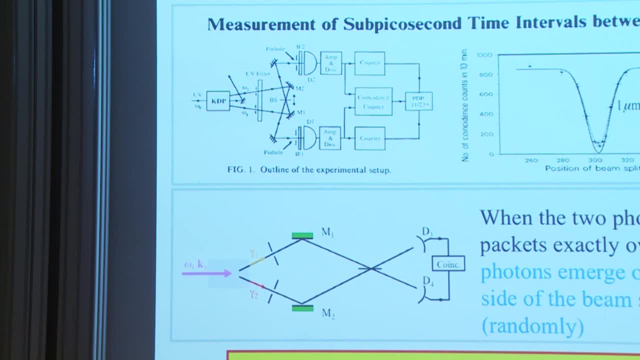 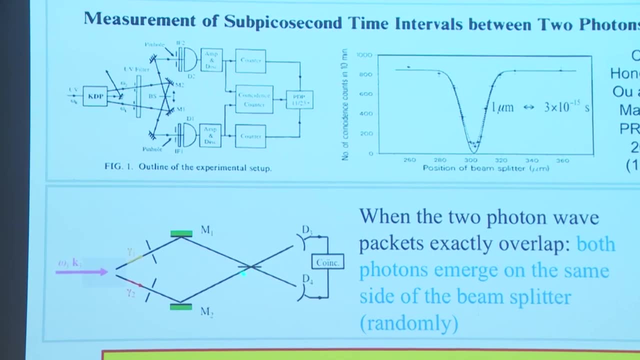 And the fantastic result which was observed by Ongo-Mendel is the following: If the beam splitter is at a position such that the two trajectories here are exactly equal, so that the two photons arrive exactly at the same time of the beam splitter, 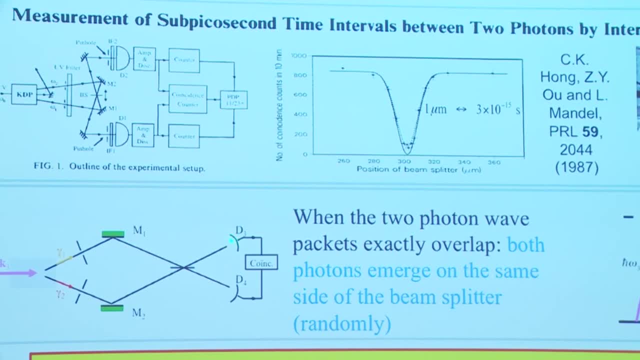 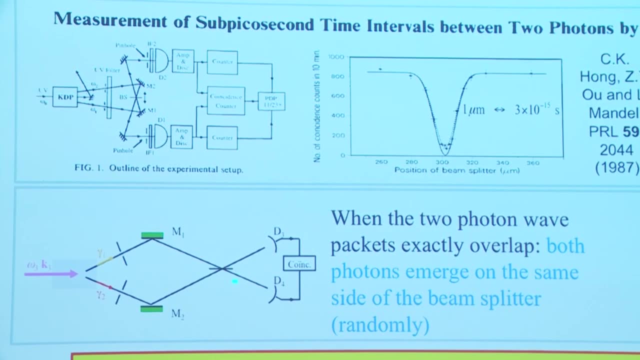 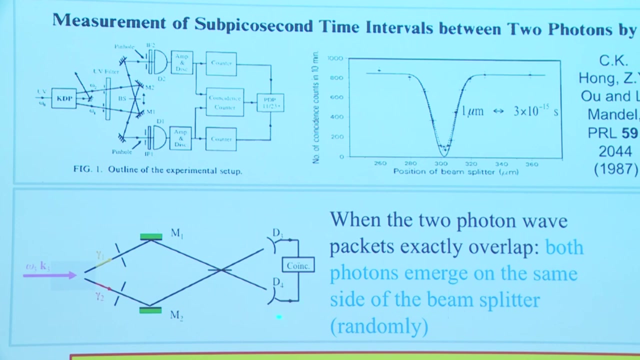 then the probability of joint detection here and there drops to zero, Which means that in this situation, when the two photons arrive here at exactly the same time, either the two photons will be detected here or the two photons will be detected there, But you will never observe. 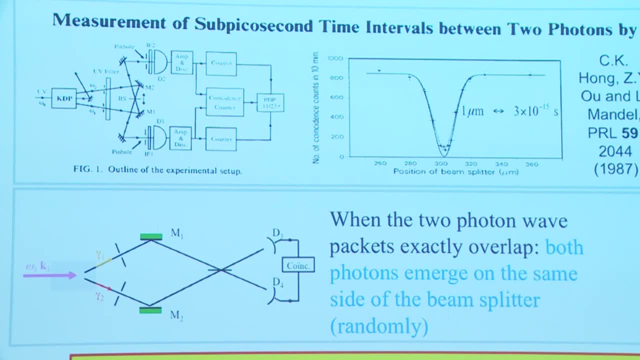 one photon here and one photon there. This really missed the point. If there were classical particles, of course you would have one for probability to have two here, one for probability to have two here and one half to have one on one side and one on the other side. 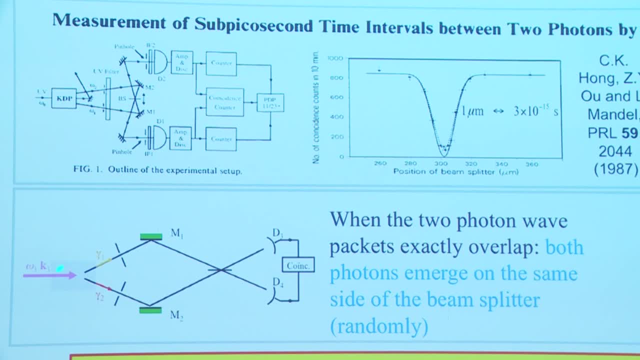 And if now you displace the beam splitter so that the time are not exactly equal, then the probability becomes large. So when the two photons arrive exactly at the same moment, then the probability drops to zero. This is a fantastic quantity of quantum effect. 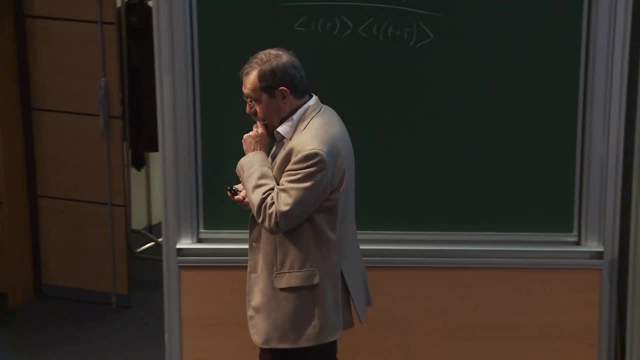 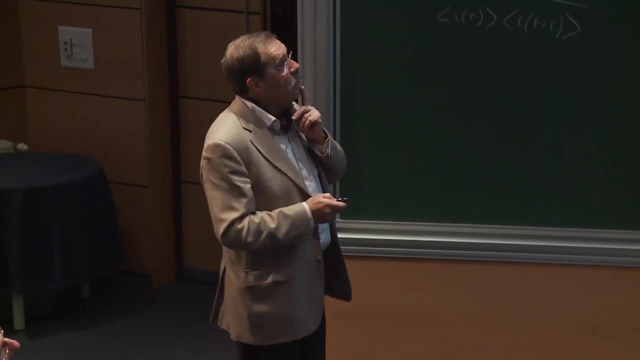 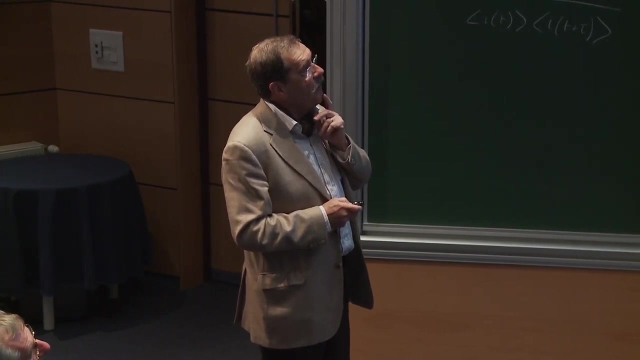 And when you read the paper of Mr Hong Hu and Mandel, they don't even mention the fact that it is a subtle quantum effect. They are extremely proud because they can measure the width of this dip with an accuracy in the femtosecond range. 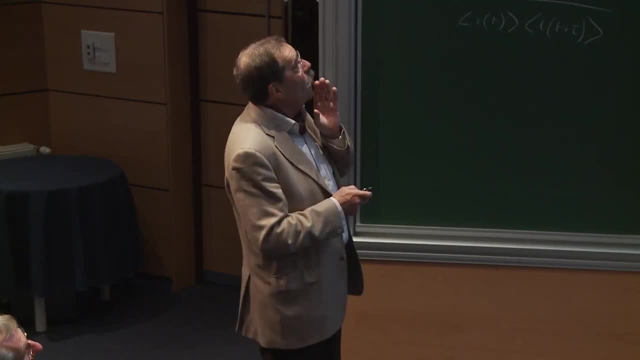 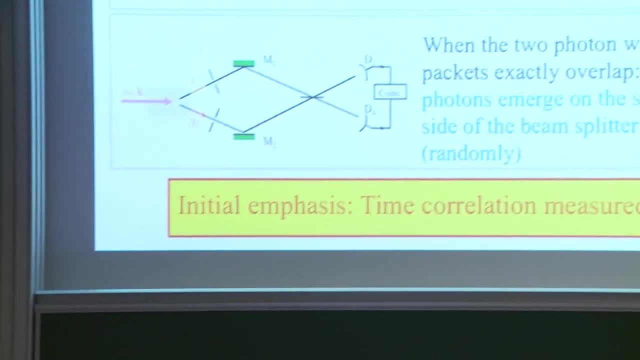 And there is no detector able to see that. And the way they find femtosecond is just that they push or pull the beam splitter with a transducer and with this transducer you can control a fraction of micrometer. so you can control a femtosecond. 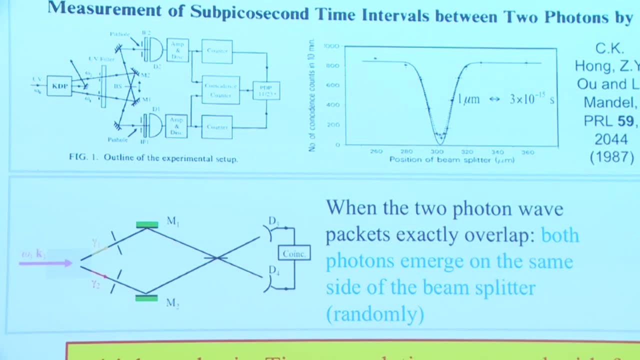 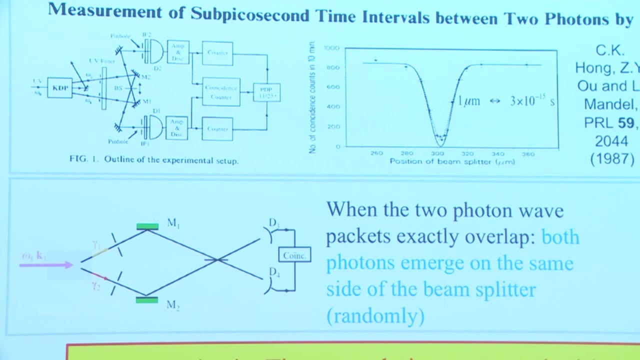 And they are extremely happy because they have a resolution of femtosecond And one year later they publish a paper and say: oh, by the way, this phenomenon that we observed is a very nice quantum effect. It's amusing, huh. 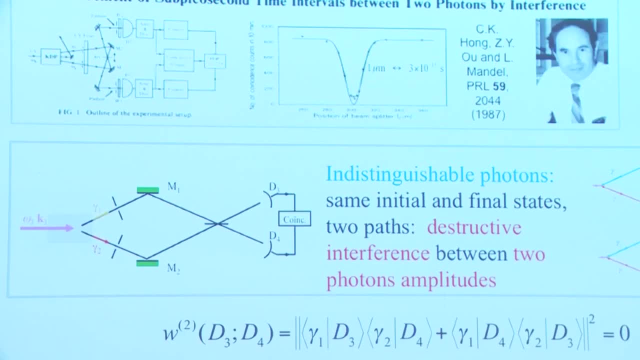 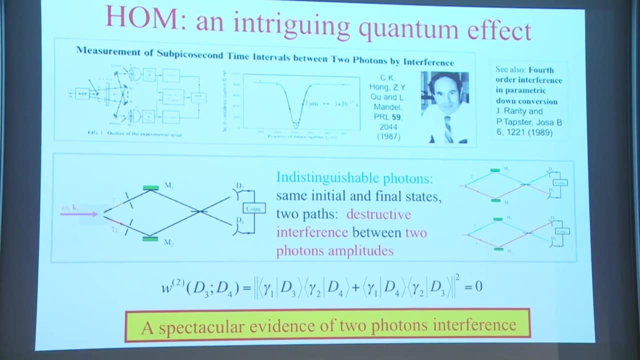 OK, So why is it a nice quantum effect? Because the only possible. there is no classical explanation of this effect. The only explanation is again to say I have two photons and at the end of the day, I want to look for the correlation and I must look at. 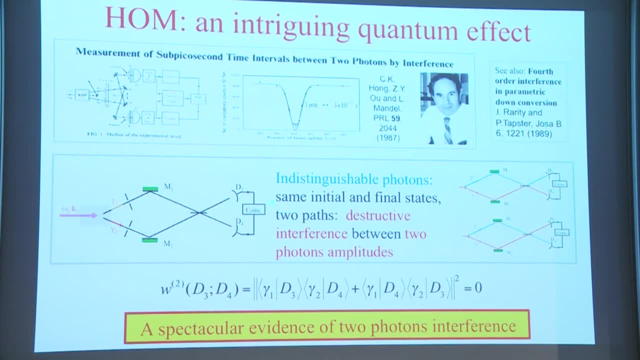 all the amplitudes for going from an initial state to a final state. And here are the two processes. The first, the photon going up, will be detected up and the photon going down will be detected down. But of course there is another possibility. 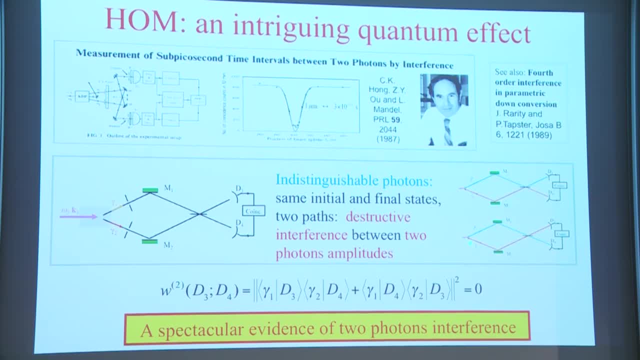 The photon starting up will be detected down and the photon starting down will be detected up. I must add the two amplitudes. Now it turns out that the two amplitudes have an opposite sign, And the reason why they have an opposite sign. 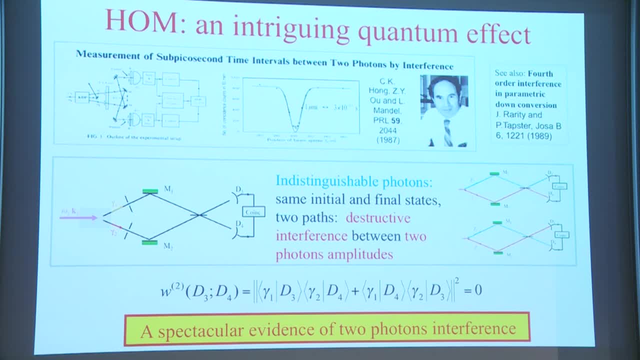 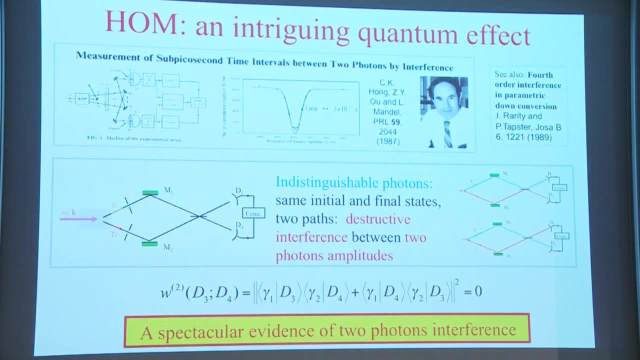 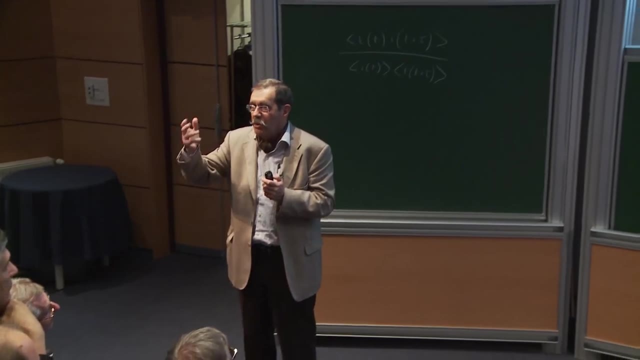 is a property of the beam splitter which is not a technological property. It's the fact that if you have an ideal beam splitter, the- maybe you call it the S matrix, but the matrix expressing the output as a function of the input must be unitary. 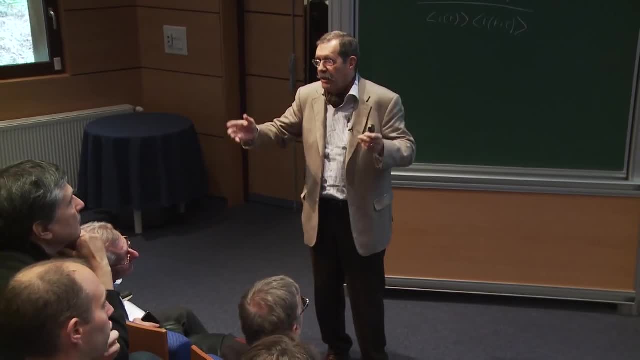 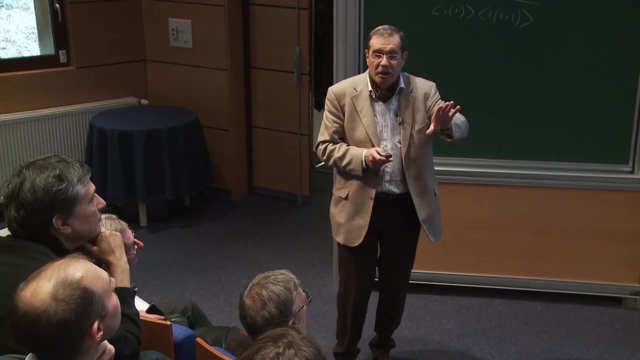 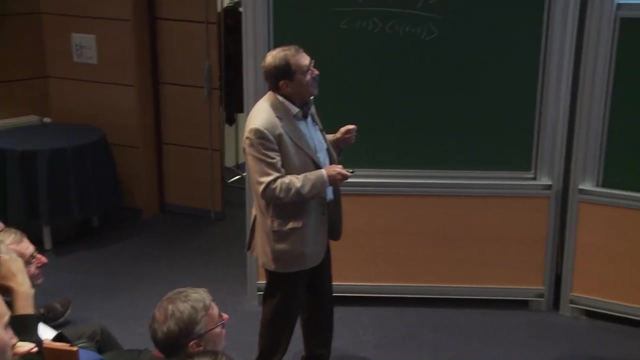 in order to provide energy conservation, of probability conservation or whatever conservation, the fundamental conservation. And because of this property, which is very fundamental, there is a minus sign between the coefficients that you have here and the coefficients that you have here. So the two amplitudes 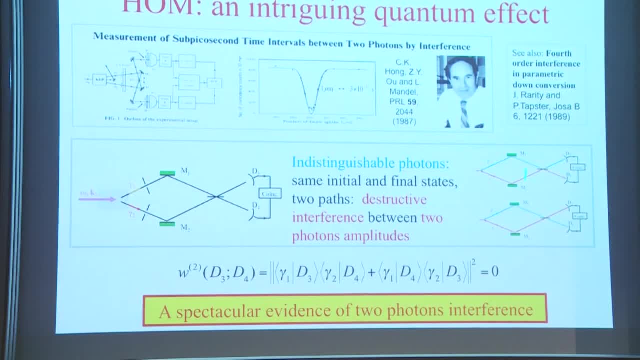 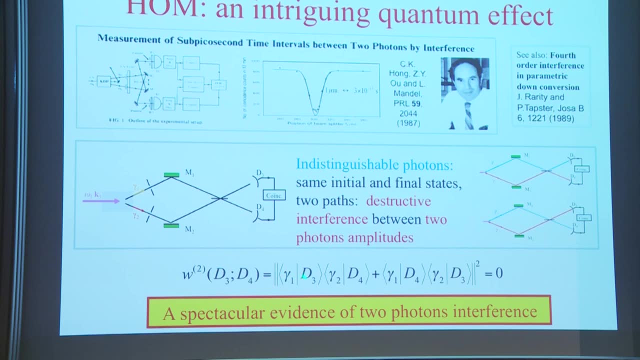 that you have here have opposite signs, which means that they cancel and lead to zero, And so the probability of detection, which is the sum of these two amplitudes squared, the sum is zero. So this is spectacular evidence of two photon interference. And again, 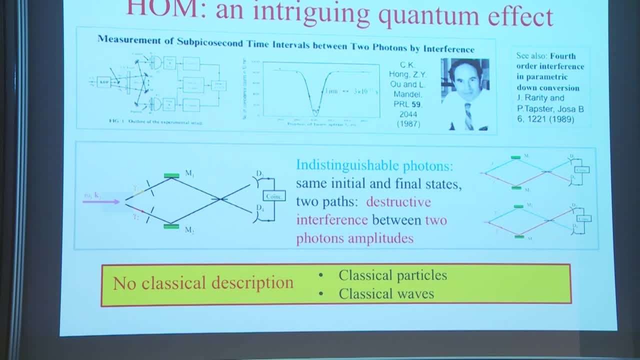 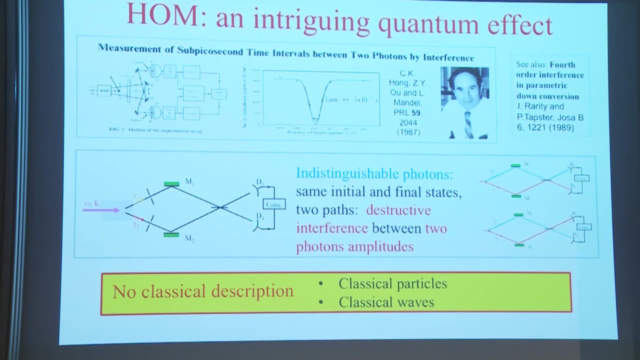 there is absolutely no classical model for that, because, of course, if it was classical particles, they would be split between the. okay, you have a model when you say: I have a particle which has 50% chance to be reflected and 50% chance to be transmitted. 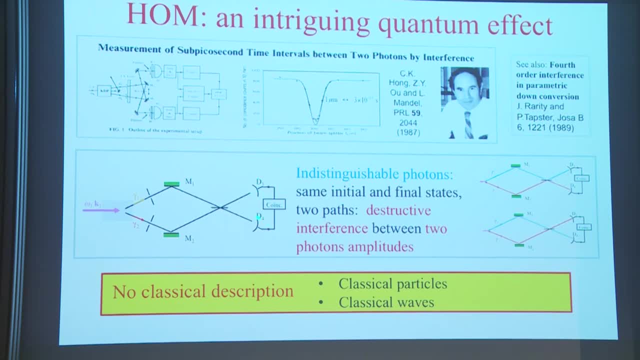 Of course, what you get is one quarter for both here, one quarter for both here and one half for one on each side. Okay, But with classical wave it's a little more subtle. You can think of a classical wave arriving here and a classical wave. 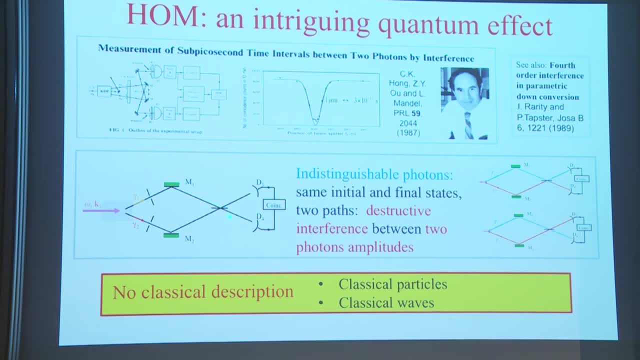 arriving here and then by tuning the phase, you can convince the two waves to go out here or the two waves to go out here. But the point is the following: you have also a randomness in the effect, So you must add a fluctuation in the phases. 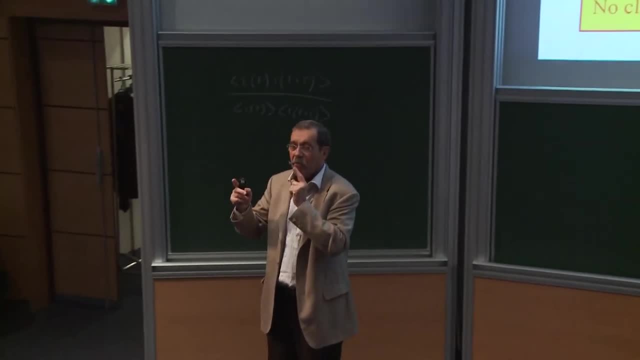 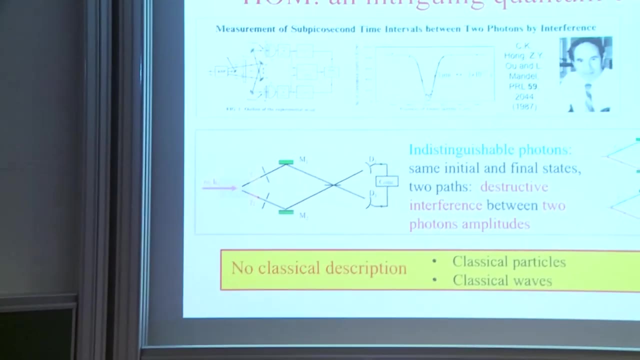 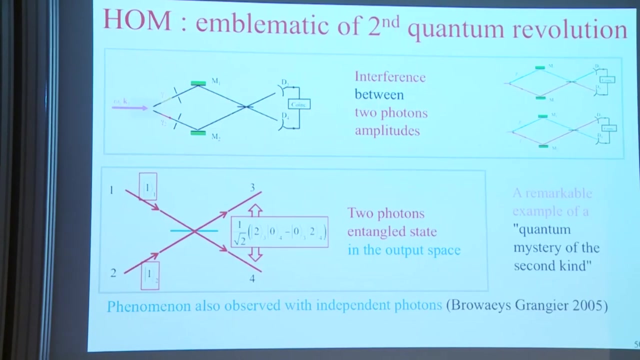 Okay. And when you have, when you add fluctuation between the phases, you find that with classical wave you can indeed have a dip, but the dip can never go below one half. So there is no classical model for rendering an account of something going like that. 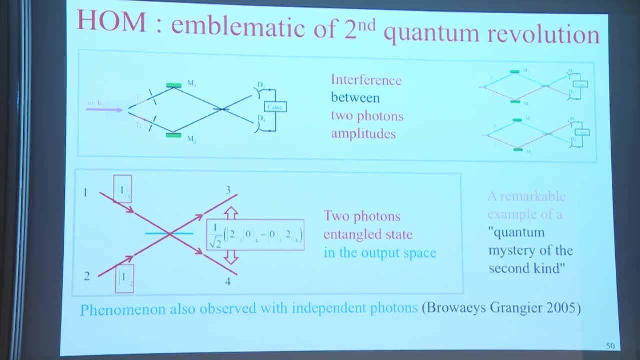 I would like to add something which is extremely subtle from a theoretical point of view. This phenomenon can also be observed with independent photon, because in the experiment of Ongo and Mandel, the two photons are produced from the same source, They are produced simultaneously. 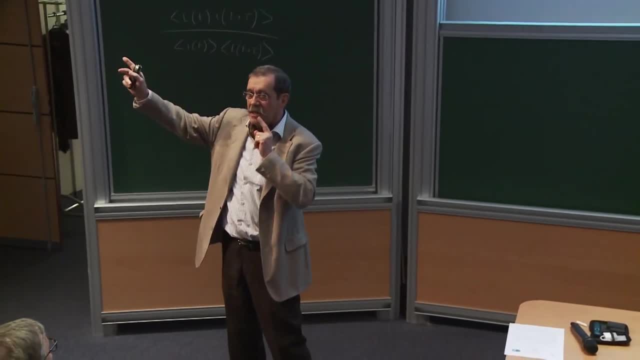 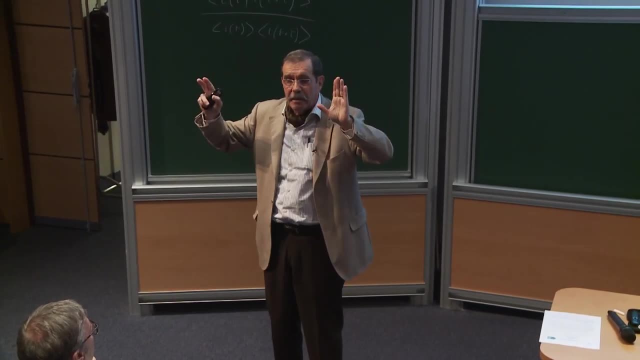 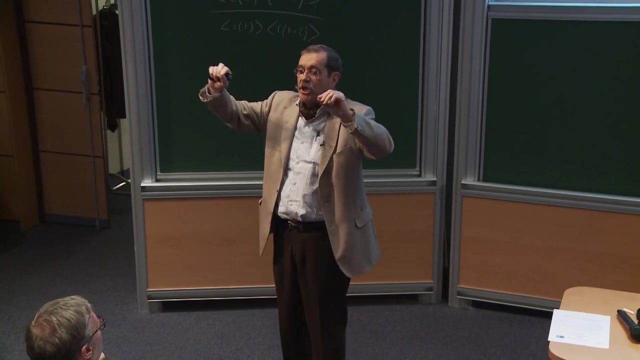 But if you take two photons coming from two distant galaxies, provided that they arrive at the same time, by chance- but it may happen- provided that they arrive at the same time on the same spatial mode, with the same frequency, etc. then you will have the same effect. 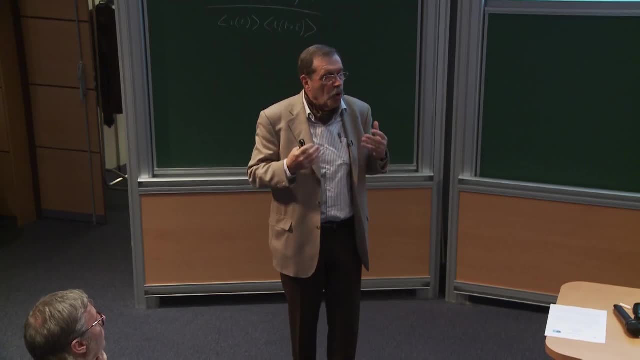 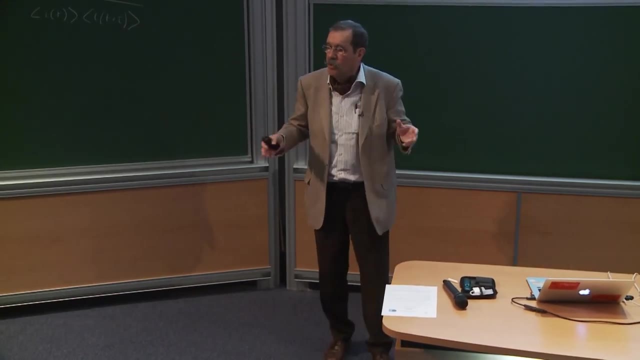 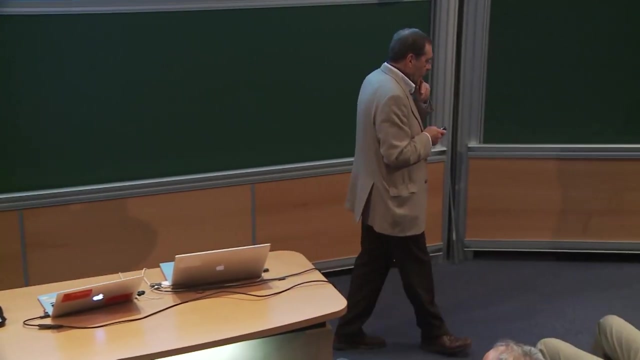 So it's really due to a quantum statistical effect, Again, the fact that it is boson and you have to symmetrize the wave function, the quantum, the quantum state, etc. So the experiment has been done not with distant stars but with two atoms. by Grangier and Brouwers. It has been done with two atoms held in optical tweezers, that is to say, you hold one atom here, you hold one atom there, you excite them so that they emit randomly spontaneous photons. then they recombine it. 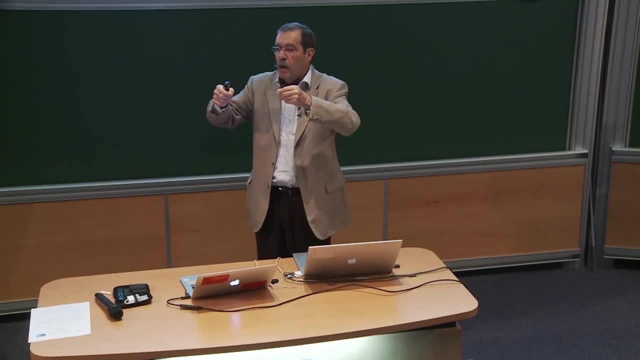 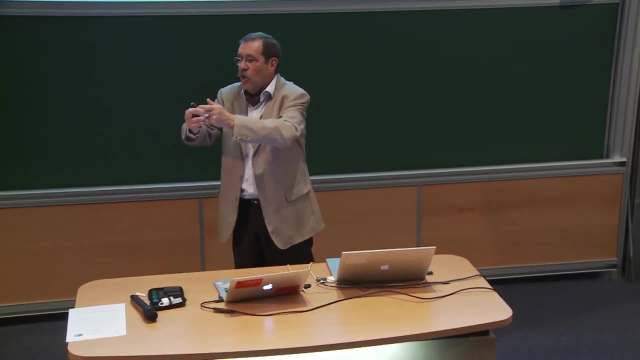 on a beam splitter, selecting the mode, etc. and by chance, from time to time the two photons arrive exactly at the same moment. and then they observe indeed that either both go on one side or both go on the other side, and never on both sides. So this effect. 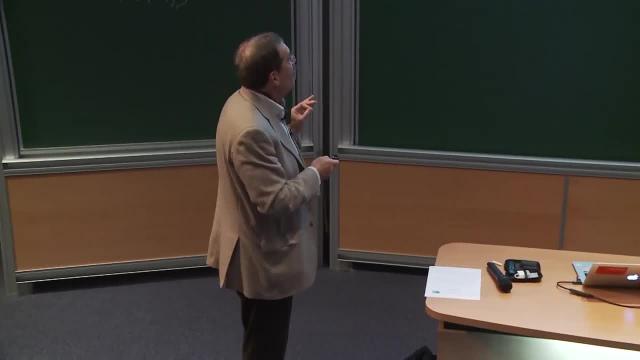 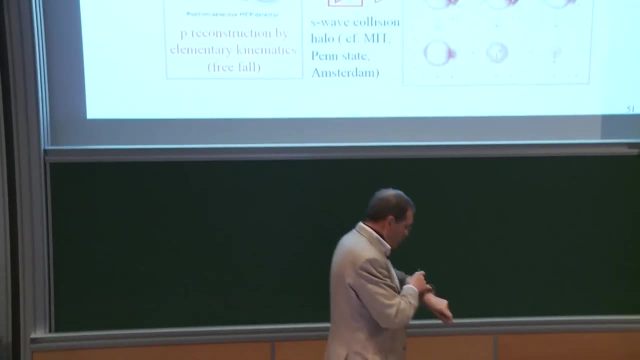 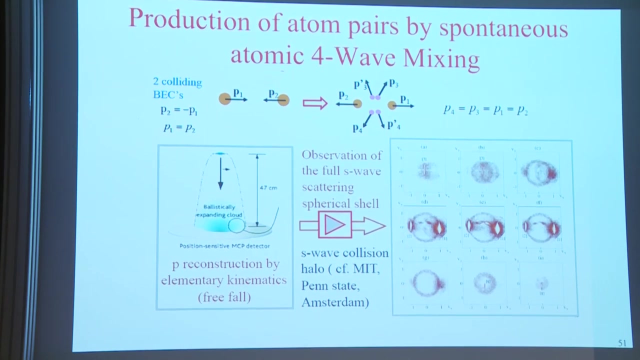 is really purely quantum effect. So can we observe the Hong-Wen-Mandel effect with atoms? The answer is yes. we succeeded a few years ago. I will give you a little information about how we do the experiment. First, we want to create pairs of atoms. 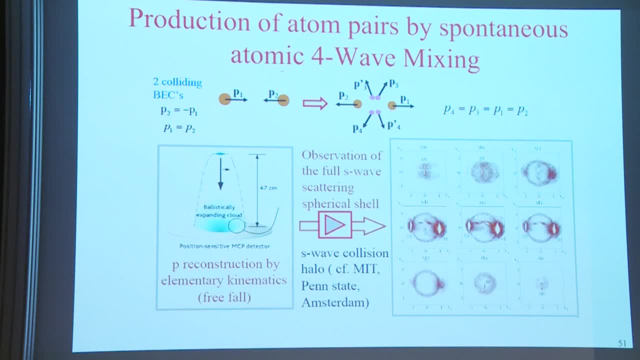 in order to test the effect, starting from pairs. Why is it better to start from pairs? Because if you rely on random arrival, it takes forever to by chance have particles arriving at the same moment, While if they are emitted at the same time, it's very easy. 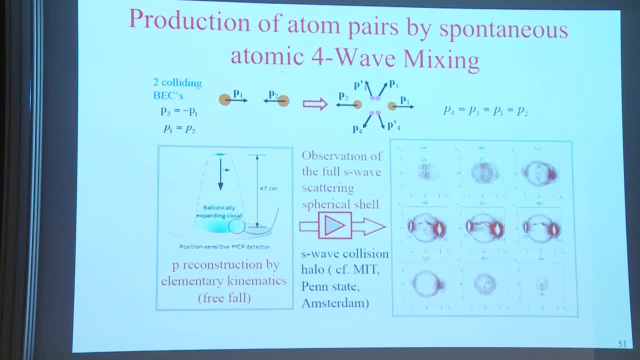 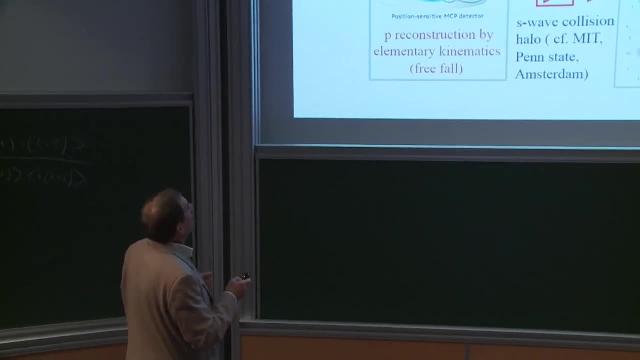 to recombine them at the same time, Right? So this is why Hong-Wen-Mandel did it with a pair of photons emitted by a source, and we want to do the same with atoms. So we want to create pairs of atoms, So to create. 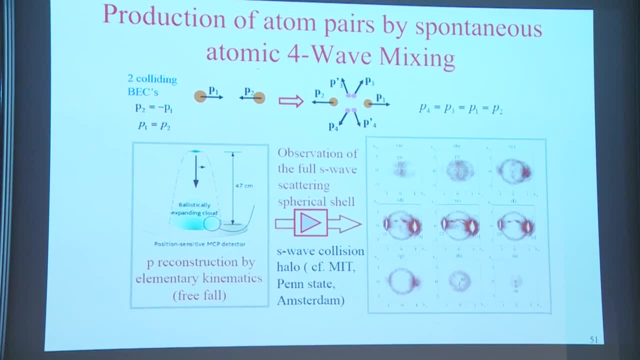 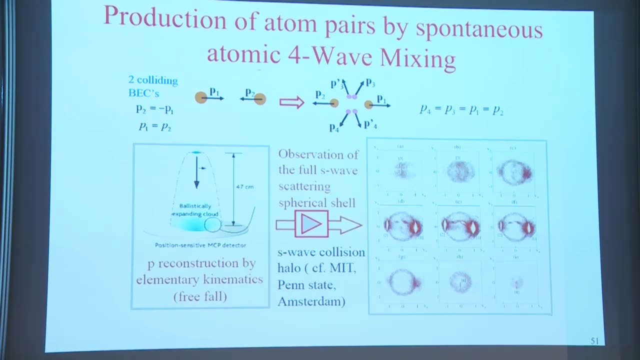 pairs of atoms. we collide two Bose-Einstein condensates and because of conservation of energy and momentum, if we work well, because of conservation of energy and momentum, when we collide the two Bose-Einstein condensates, they cross each other. then we create pairs like. 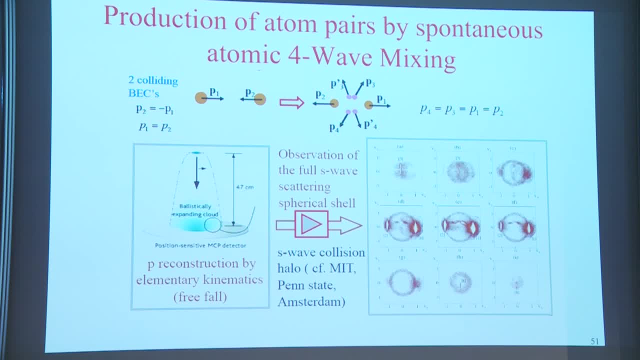 P3, P4, with P4 equal minus P3, or P prime 3, P prime 4, etc. Okay, And in order to observe it, what we do is, again, we use our wonderful detector, which is in fact a three-dimensional detector, So we make. 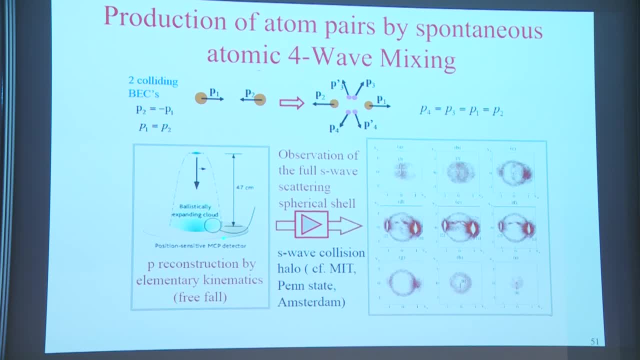 the collision and we observe the ballistically expanding cloud. and because we are far from the source, what we do is we create a sphere with a shell, and this sphere with a shell is all these atoms which are due to the collision. here I can probably show it. 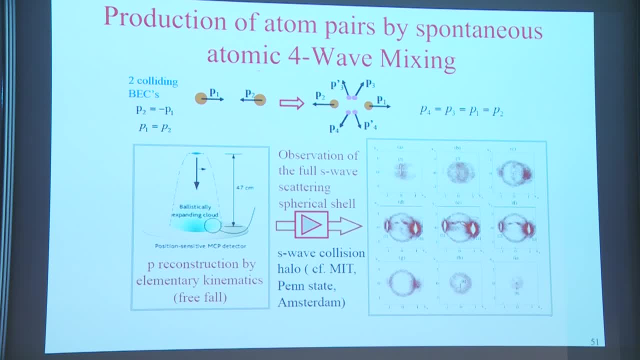 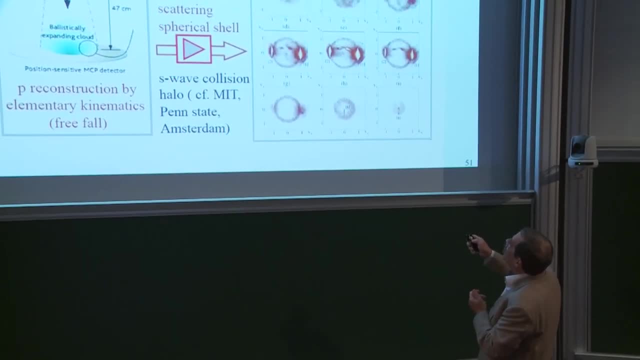 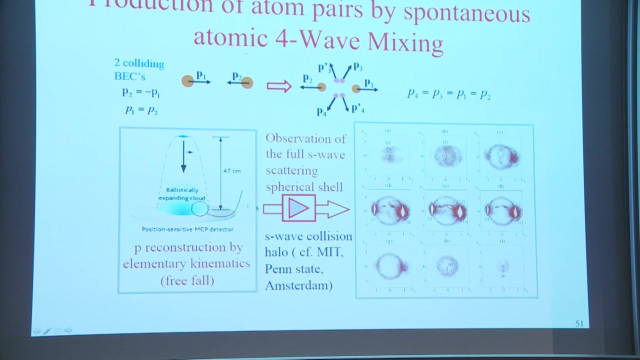 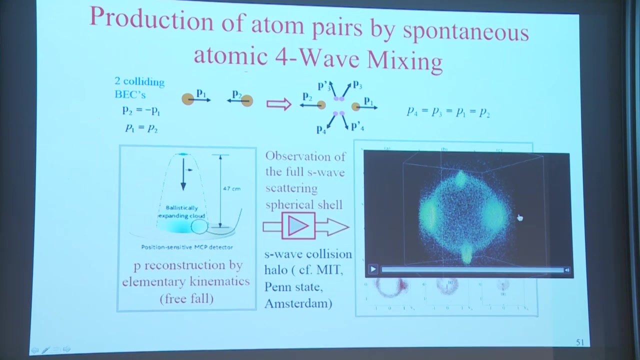 yes, I can show it here, my scale. and this sphere with a shell is all these atoms which are due to the collision, and I show it here. my students have prepared a beautiful image, just like in CERN. okay, so what you observe here is the remaining boson-chan condensate. 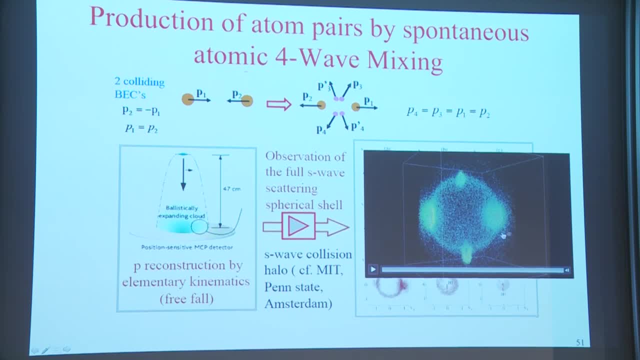 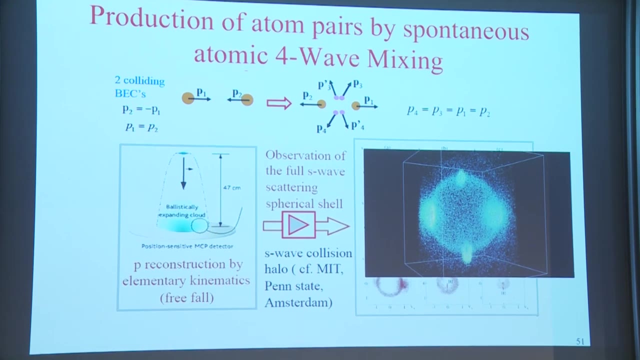 this is not an artifact, but a supplementary thing that we have, and I don't want to comment it. and you see, we can have everything rotating. so it's clear that we have atoms on the shell which correspond to atoms produced by this collision. now, this does not. 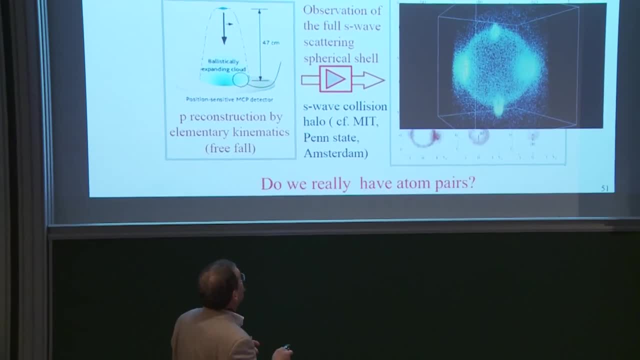 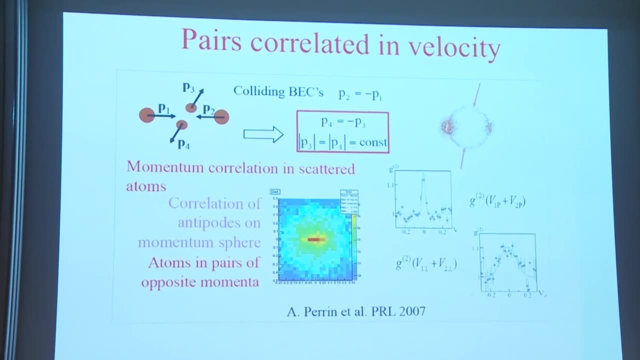 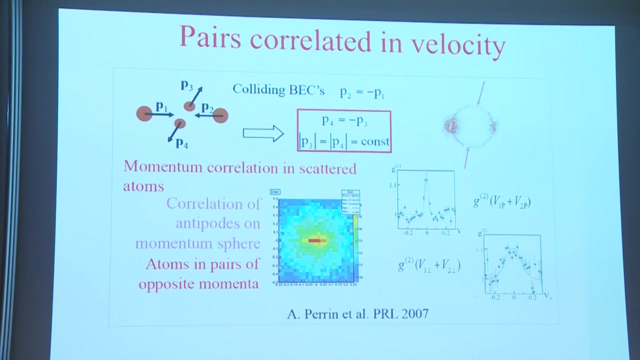 mean that they are emitted by pairs. so to show that they are emitted by pairs, what we do is we look for correlation in antipodes, and when we do that, indeed, we find peaks. so now we know that we produce the atom by pairs, like that anyway. 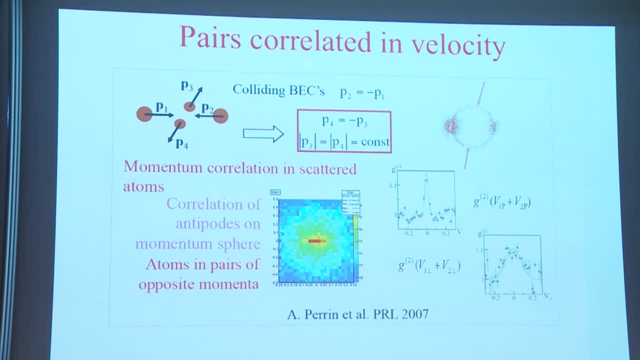 it's not ideal for doing the next experiments because, the atom being emitted in all directions, we want to convince them to go in a well-defined direction in optics. we know how to do it in non-linear optics by the so-called phase matching condition, so we looked 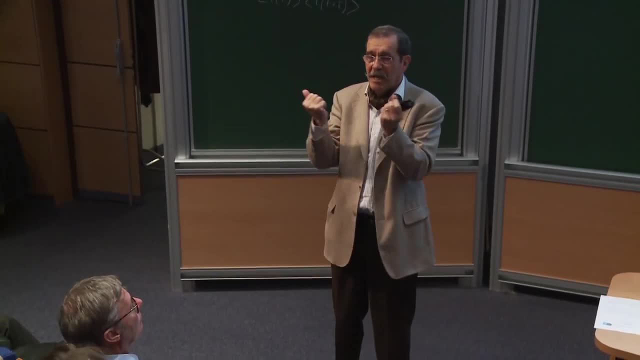 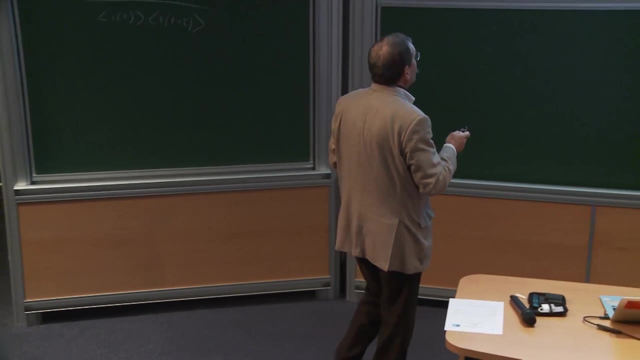 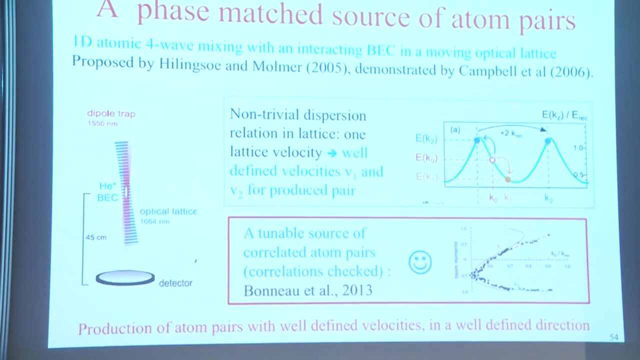 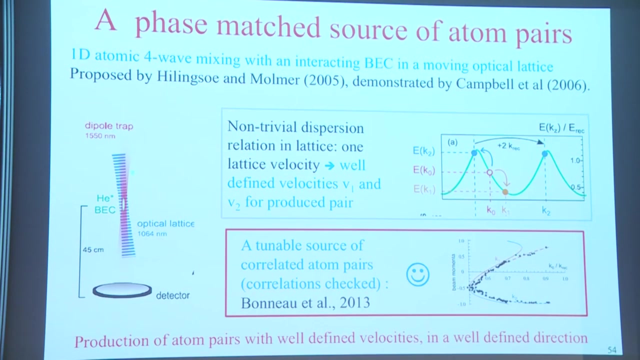 for a condition equivalent in our collision. we would like to have a process forcing the pairs to be emitted along well-defined direction with well-defined velocity, and we succeeded using a process by a nice Danish and a smart Danish theorist, Klaus Mulver. the idea is the following: 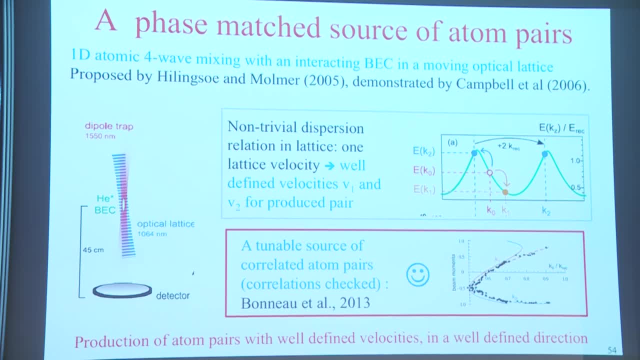 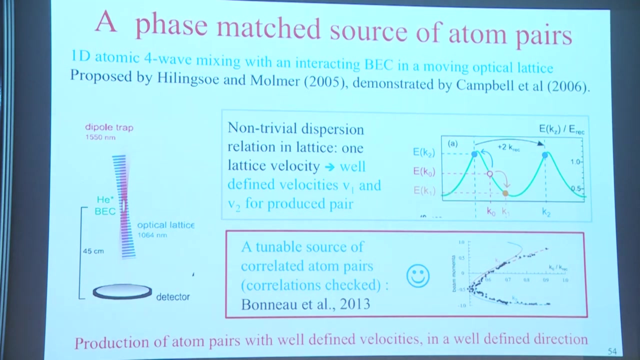 if we force the atom to circulate. so this gives you an idea of the subtlety of the experimental technique we use. first we force the atom to circulate in a de Broglie wave guide. this is a compass word but it has a truth. 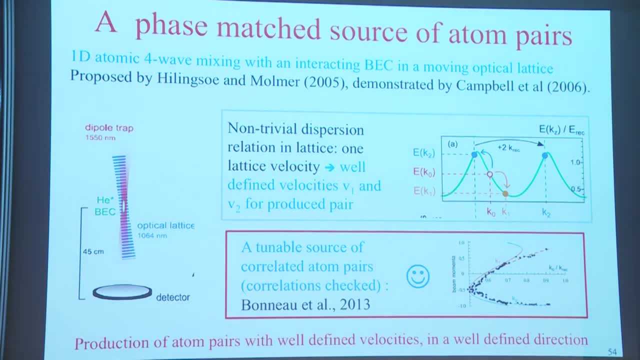 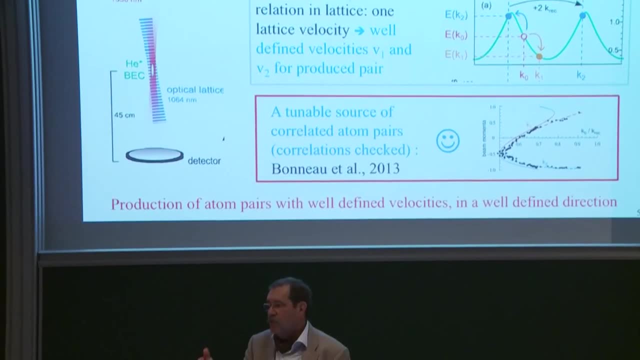 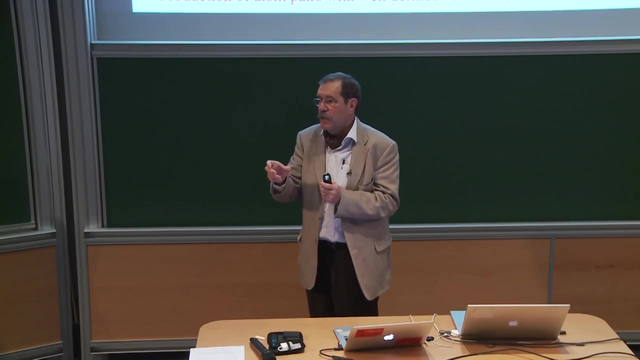 in it. to say that we have a laser beam which attracts atoms towards the center of the beam, so transversely, is just like a harmonic oscillator, and in fact the transverse velocities are so small that the atoms are in the ground state of the transverse. 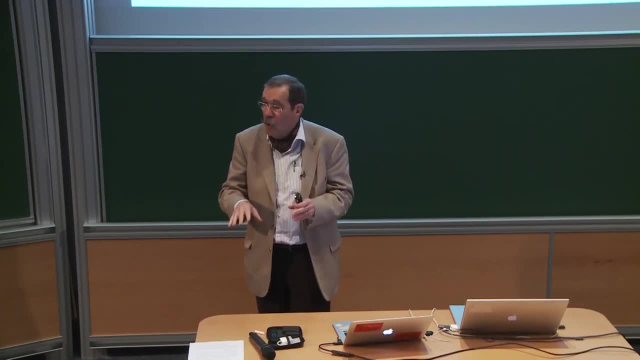 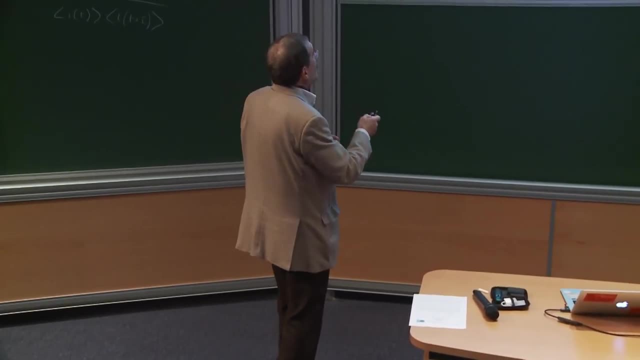 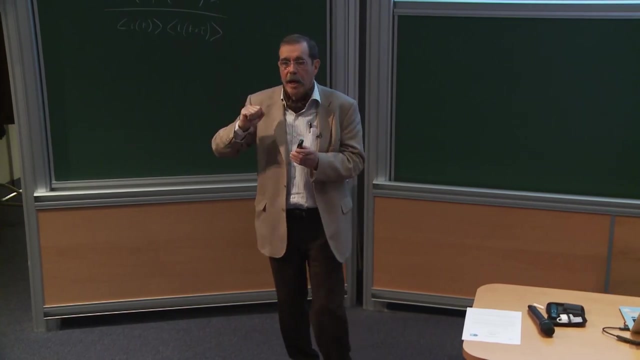 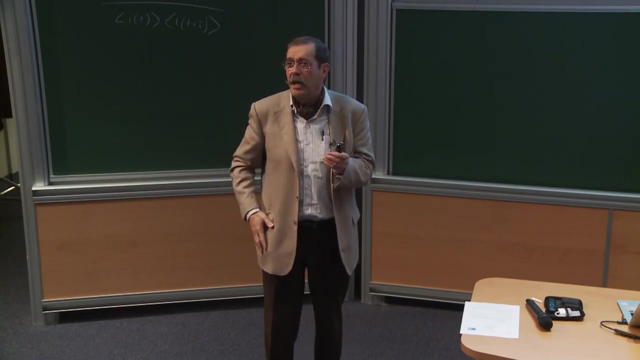 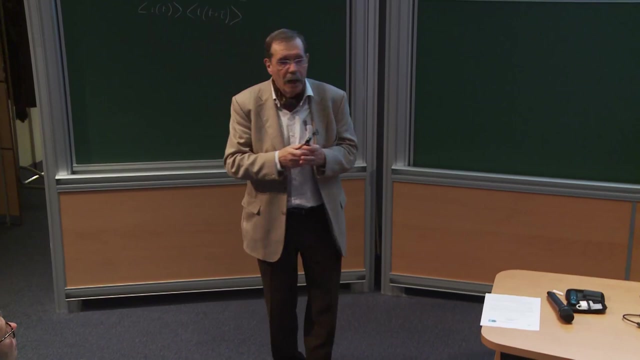 harmonic oscillator. we are in the lowest state of the harmonic oscillator, so the atoms are forced to circulate along this direction. along this direction we impose, with a standing wave, a periodic potential. so now we have something like electrons circulating in a periodic potential, and what you have? 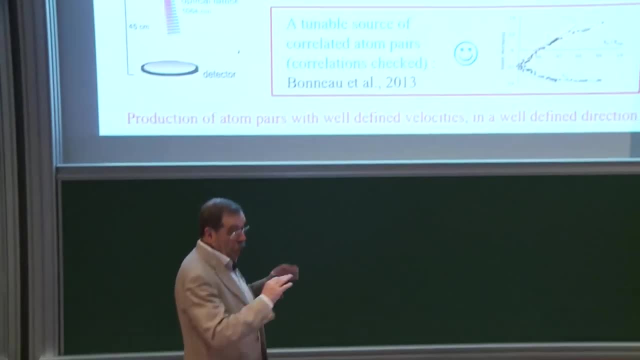 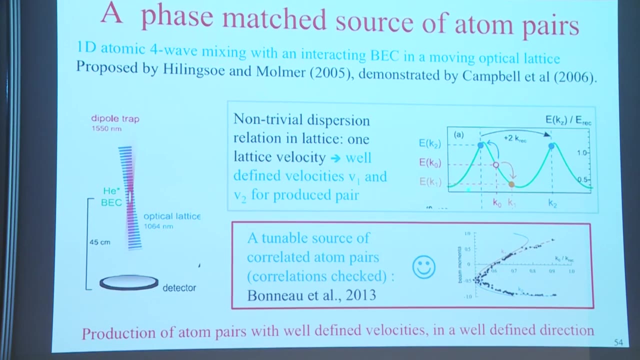 is. it's a fully quantum problem and the solution is dispersion relation, that is to say energy as a function of the momentum which has a shape like that, so which is far from trivial now if we have a collision between two atoms and we impose conservation of energy. 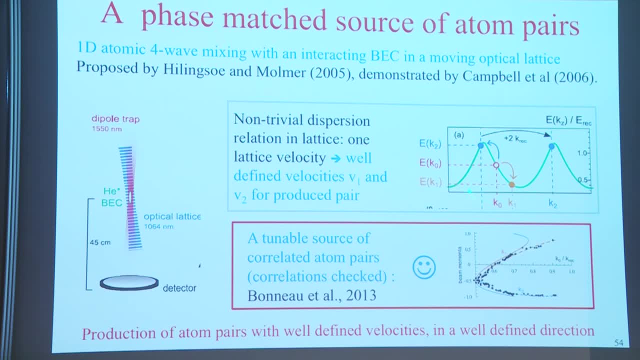 and we impose conservation of momentum for a given initial pair of atoms which collide between each other. there is only one solution, which means that now, if i have a given velocity of my atom- it's a dynamical instability- and produce two atoms with a given energy, which is 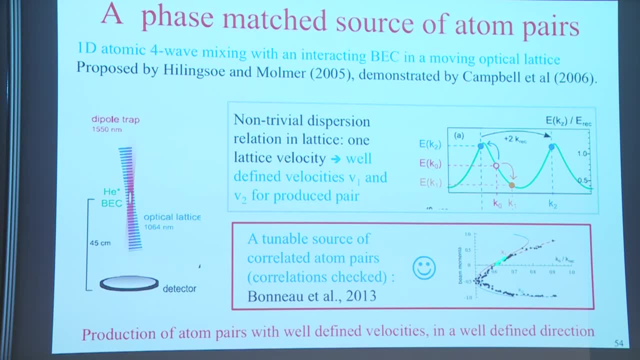 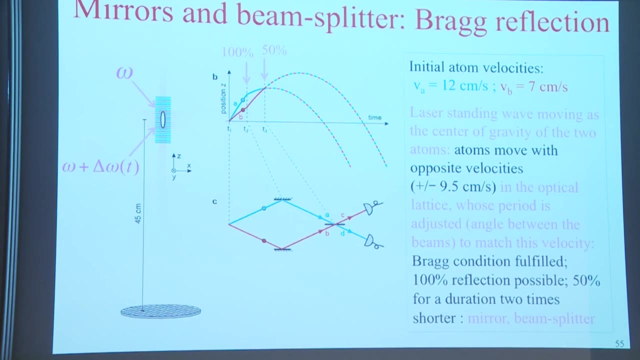 fixed by this condition. so i know now this is what is plotted here. it's a paper that was published. we know how to choose a parameter to produce two atoms with a well-defined velocity. so now this is how it looks, with a well-defined velocity and rather 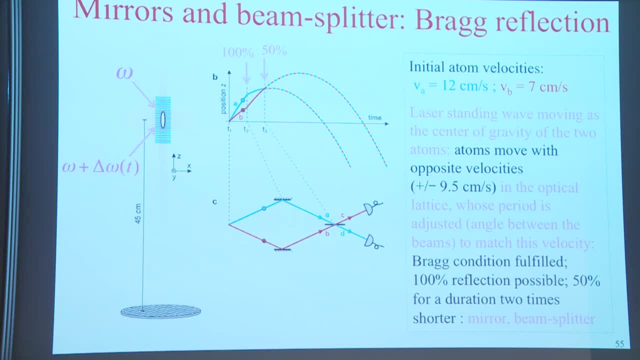 than describing it in the usual space with parabola, etc. etc. it's annoying. i will put myself in a frame of reference which is, following the param, the parabola of the center of gravity, of the barycenter, of the two atoms. so the scheme. 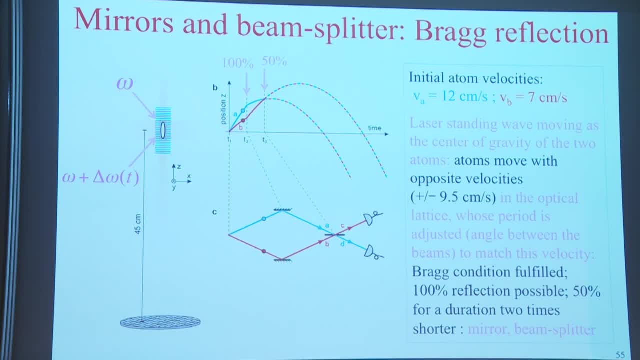 will be this one, and at this time i will recombine the two things. it would be a little long to explain you how we reflect atoms and how we make a beam splitter. in fact, for people who have an idea, we use a light standing wave which imposes. 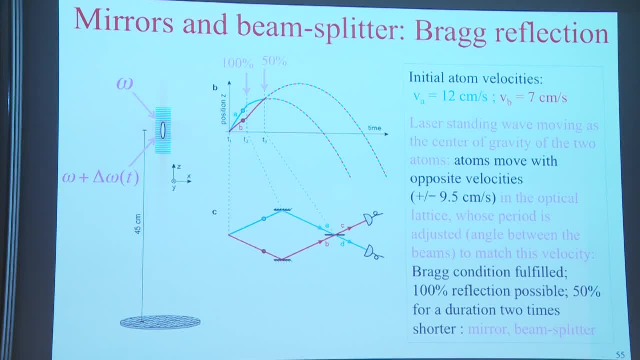 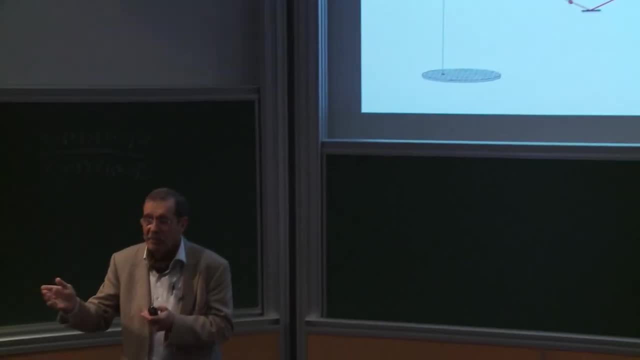 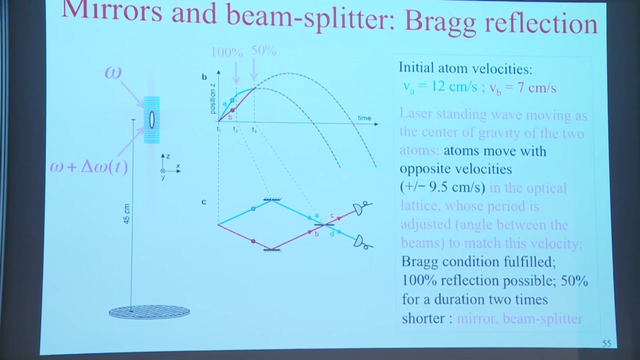 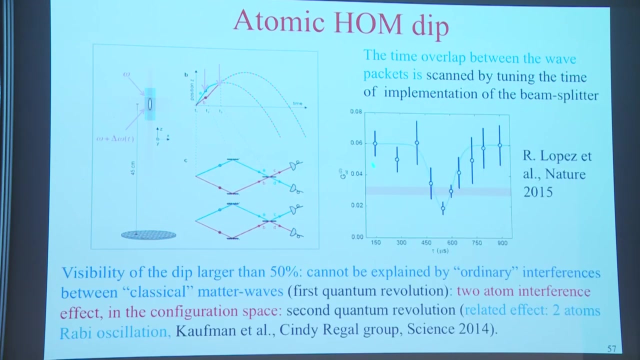 periodic potential, and the beam splitter will reflect only partially and transmit only partially. so here we can totally repeat the scheme of amber brown, of hongo and nandol, and so this is the usual explanation, okay, and what we observe is indeed the hongo and nandol. 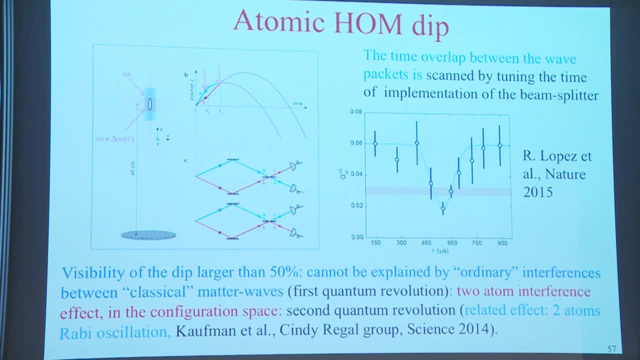 dip with a 30%. so there is no way to explain it by any classical image. and here i am really exaggerating, because what i call a classical image would be two de Broglie waves and deferring, but two de Broglie waves in our 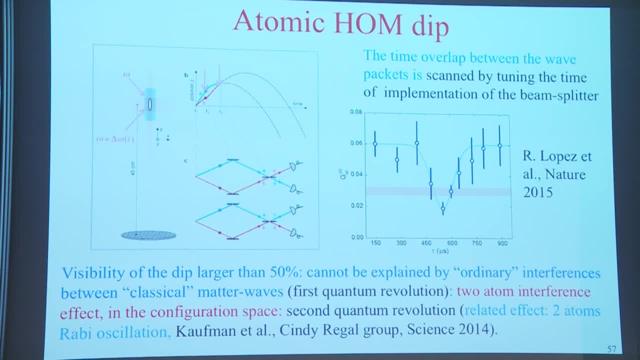 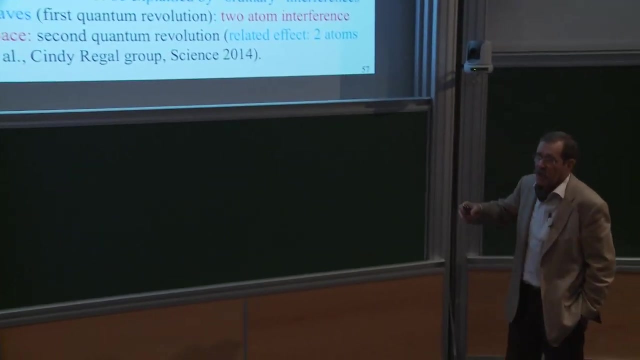 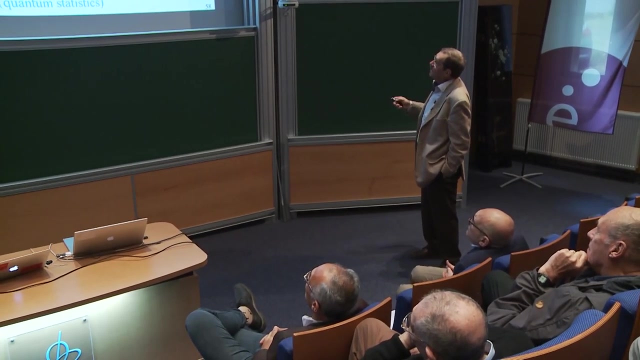 ordinary space. it can not be two ordinary de Broglie waves in our space. okay, so maybe it will be time to stop and to let you ask some questions, because i have another subject, but i'm afraid it's a little too long. so what we have, 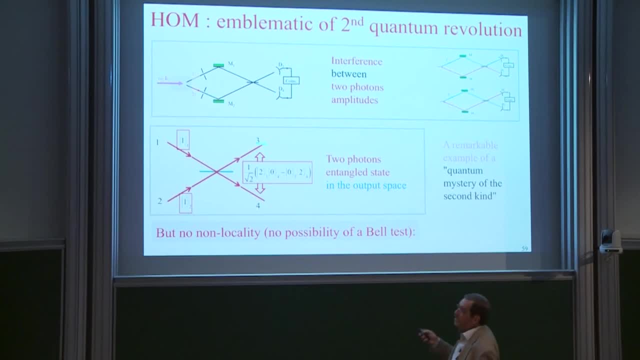 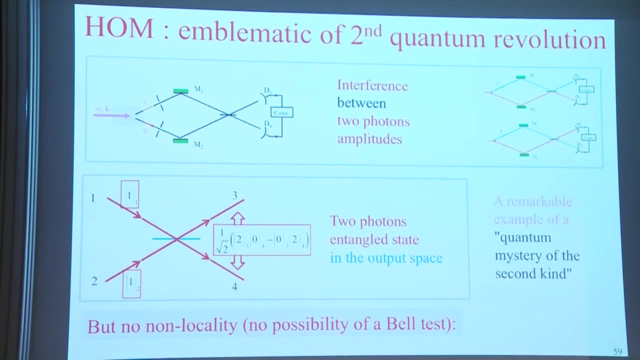 shown here is again a remarkable example of quantum evolution. so you can ask yourself the question: if i have an entangled state like that of two particles, could i test bells inequality with it? and of course, this is what we want to do and the answer is we. 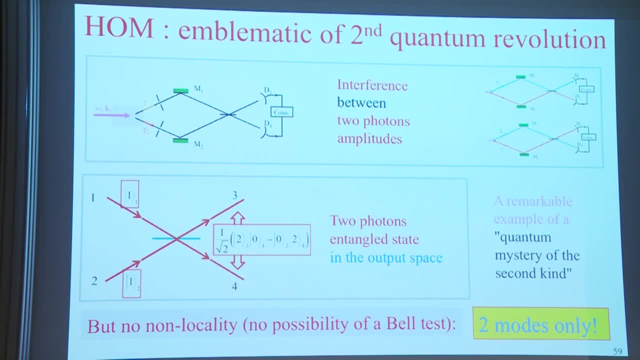 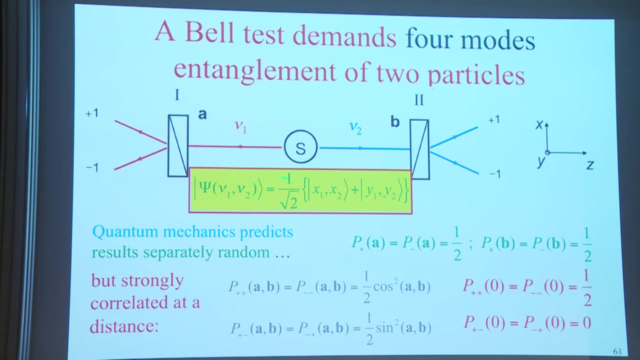 don't have enough here. to test bells inequality. for people who know about bells inequality, you need four modes and i will explain you why. if you take the standard experiment of test of bells inequality with photons, okay, what do you mean by polarisation? horizontal and same here? 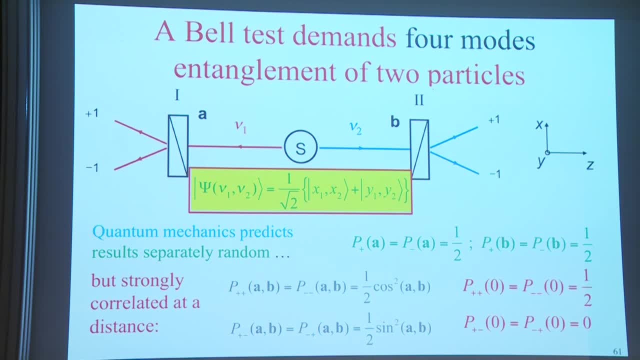 polarisation vertical, polarisation horizontal. so this entangled state is an entanglement between four modes and you need these four modes in order to have something here which is a of x1 and x2, there is no way to assess Bell's inequality. 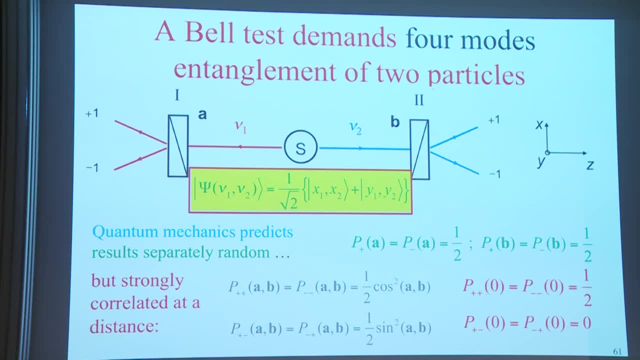 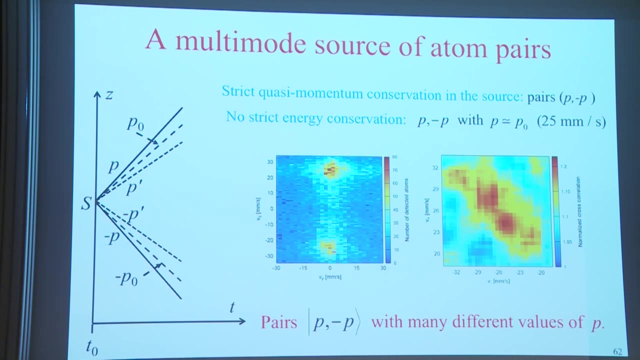 Bell's inequality is not just one measurement. You must compare several measurements And for that again you need two modes on one side and two modes on the other side. So in the experiment that we have done we look for interference between this and between that. 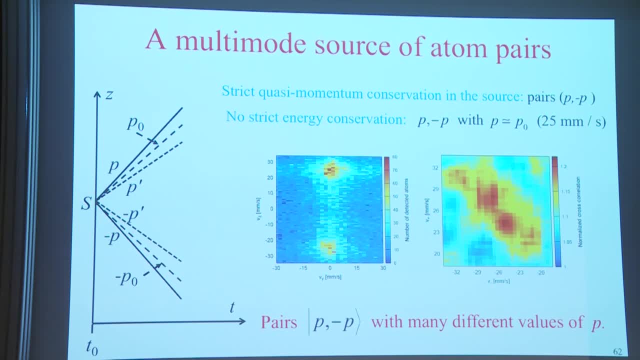 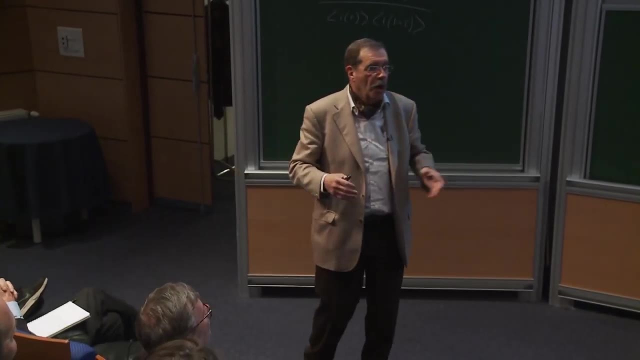 It's only two modes. But something fantastic happened in our experiment. It turns out that with our beautiful detector we record everything, just like in CERN. In CERN they record everything and then they look for events We record. well, we are not as big as CERN. 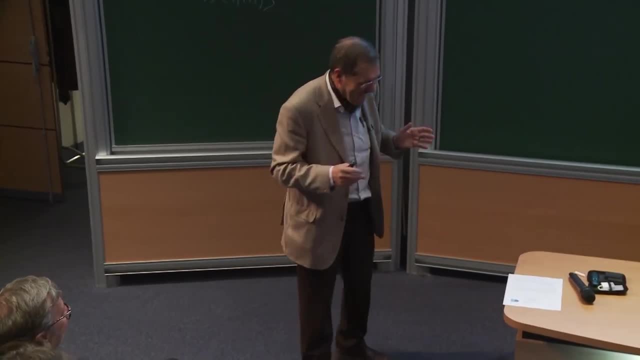 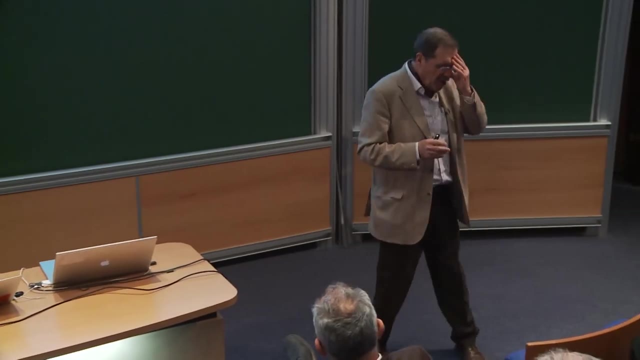 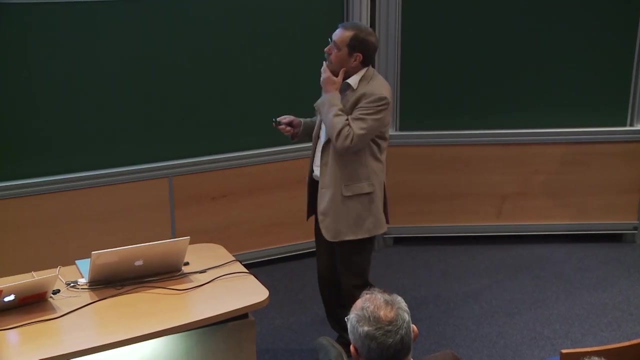 We don't cost as much And we are less people, But anyway, we record everything. And then we had a PhD student who had the version Very good idea. He looked into the recorded data and said: but in addition to pairs like that, 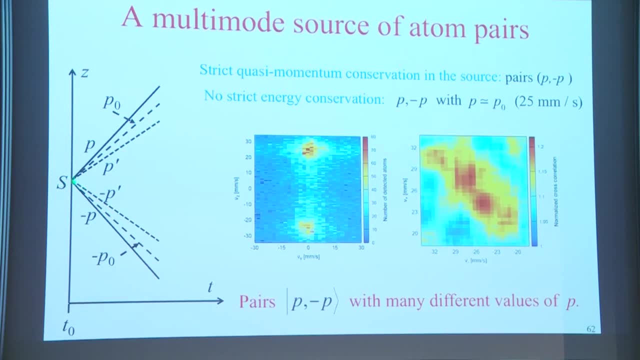 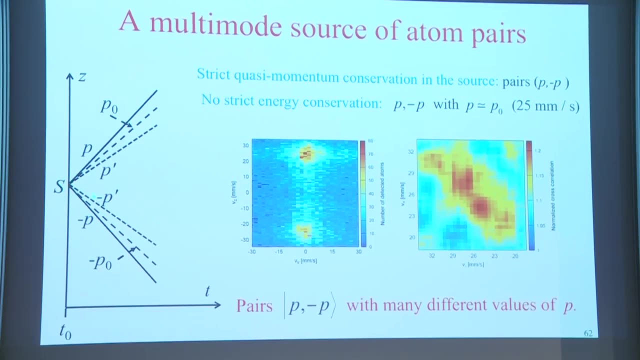 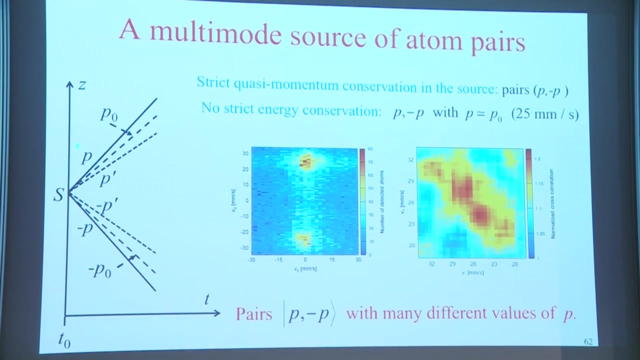 there should also be pairs like this one. So you see, this is position as a function of time, So it's different velocity, And there should also be pairs like that. Couldn't it be that we have simultaneously emission of this amplitude and that amplitude? 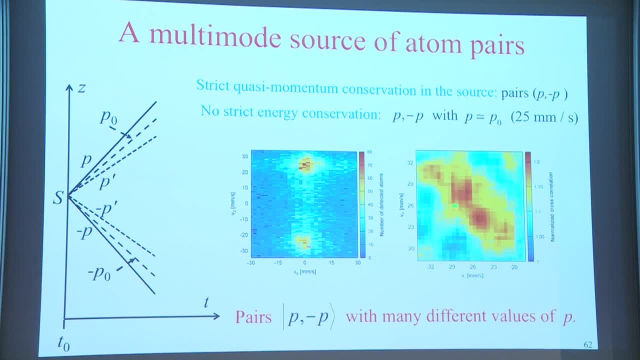 And by processing the data- I don't go into the details- we found that, yes, there are certainly pairs- p minus p- with many different values of p. So can't we have a superposition of two things like that? These would be really entanglement in four modes. 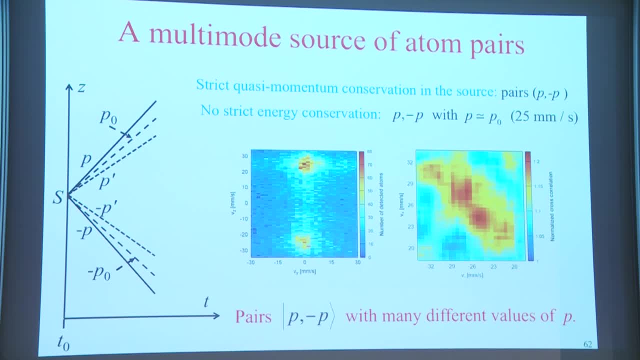 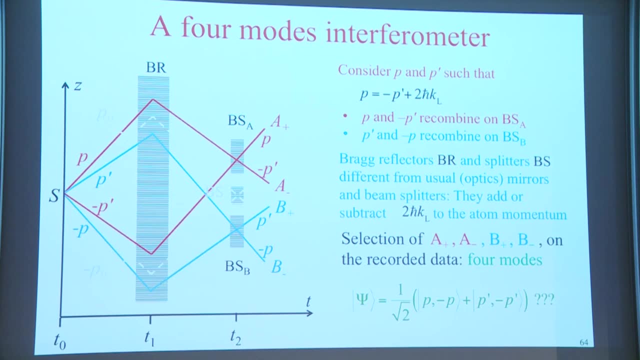 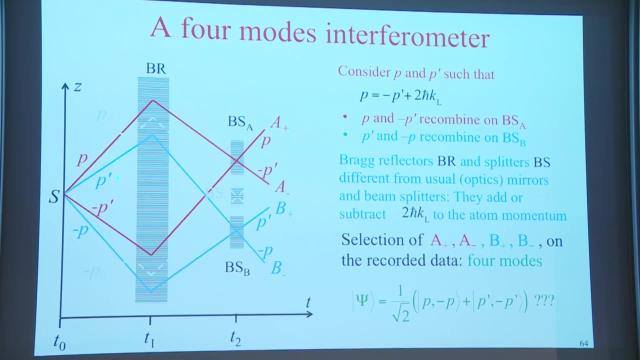 because I would have p minus p, p prime minus p prime. So we discovered by full chance- we have not anticipated it in the scheme that we had- if there was a pair p minus p and a pair p prime minus prime respecting some condition which 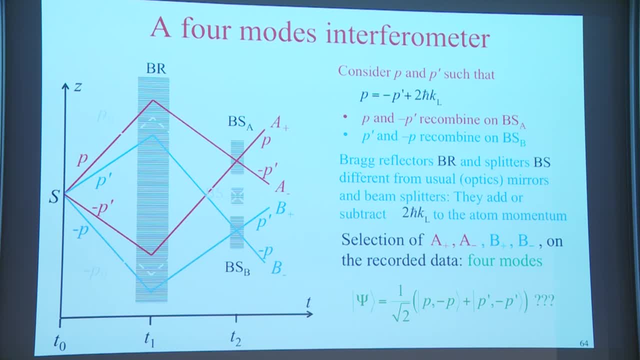 is here, which is related to the Bragg condition. I don't go into details. it turned out that the experiment which had been done for Ongo and Mandel, that is to say applying a first standing wave and a second standing wave, would recombine this and that. 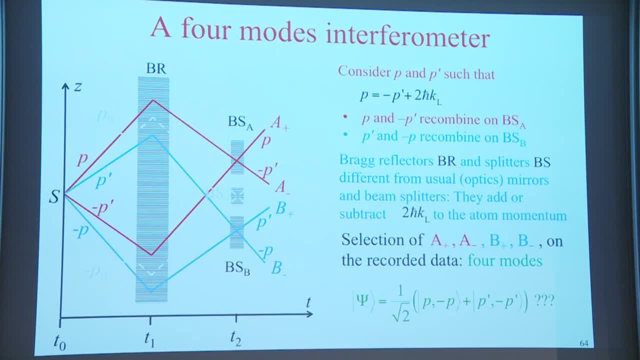 And this is exactly the scheme for testing Bell's inequality. But we miss something. The relative phases between the two things are fixed by the experiment. We don't have a knob to change this because we did not plan it. it was there. So anyway, we have looked into the correlation associated. 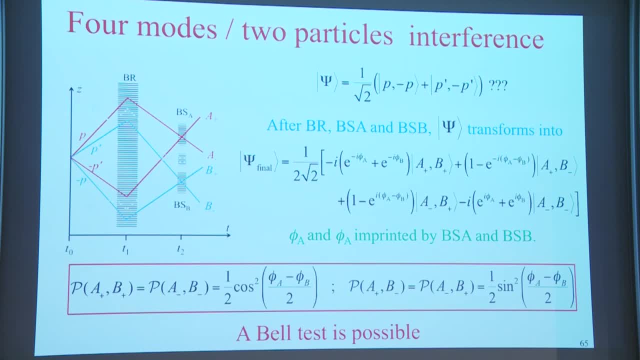 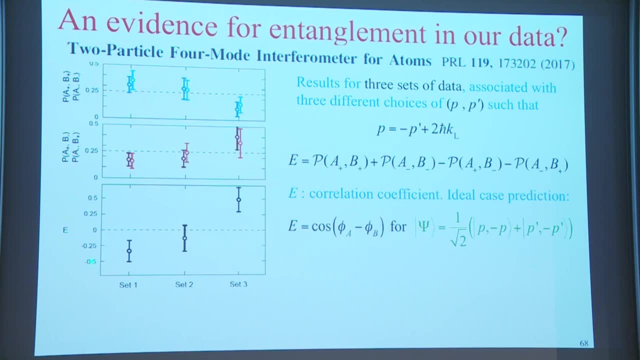 between various diagram like that And what we have found whoops, whoops, okay, And what we have found whoops, whoops, okay, And what we have found whoops okay Is the correlation coefficient, which for a first set is different from zero. 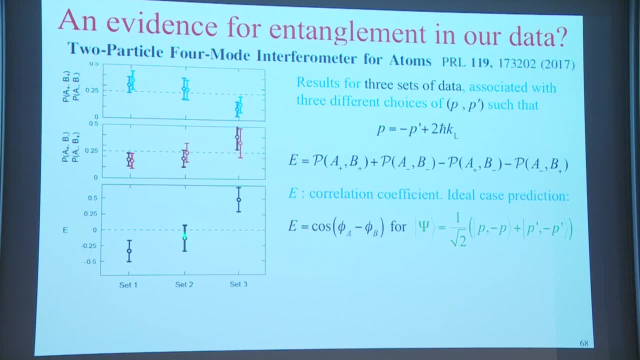 from another set is different from zero and for that set is equal to zero. The fact that we have this and that shows that we have entanglement for four modes. But I am a serious experimentalist, I don't claim much when I have something. 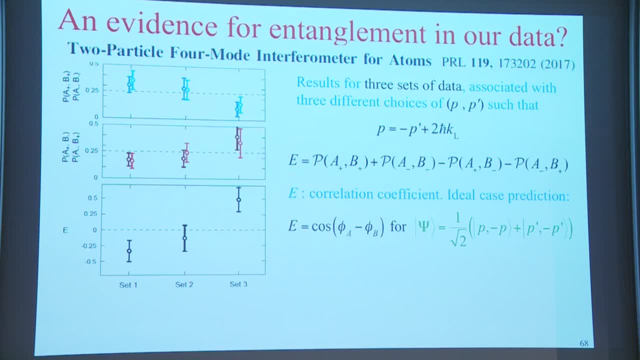 with one standard input, One standard deviation. okay, So we publish this and we say that the results that we observe are compatible with existence of entanglement. but we must improve the experiment in order to prove it, And this is what we are doing now. 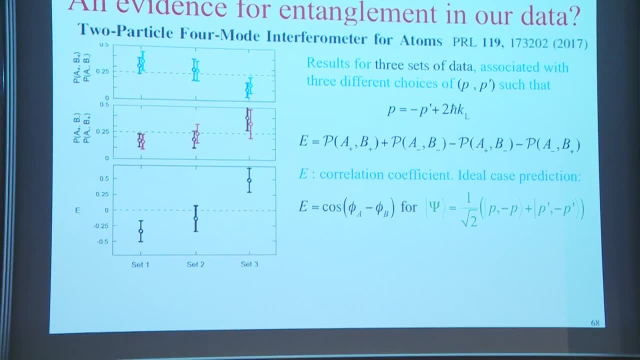 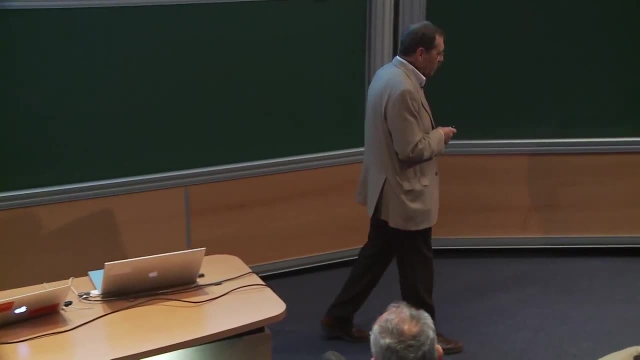 But the important thing is the following: I've been working about Bell's inequality for more than 30 years And for many, many, many years I was deeply concerned, And for many, many, many years I was deeply concerned. 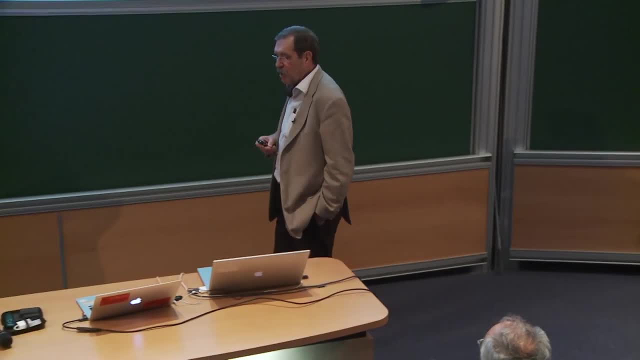 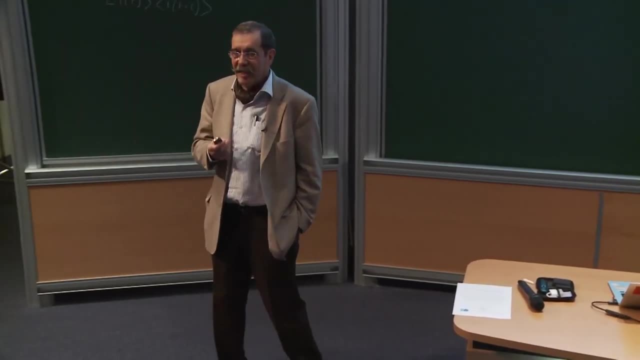 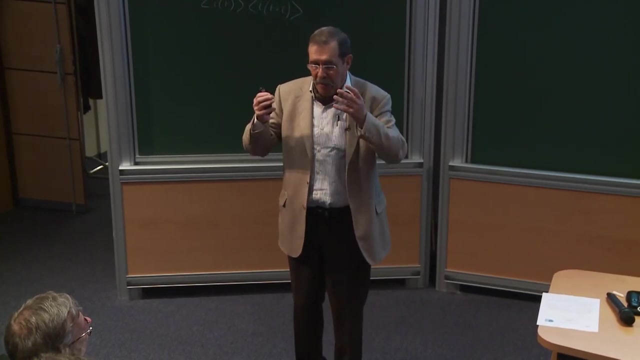 I was deeply convinced, intuitively, that violation of Bell's inequality is stronger than the Hong Wu and Mandel effect, But I could not exactly know why. Because we have done this experiment, now I know why Bell's inequality violation is entanglement. 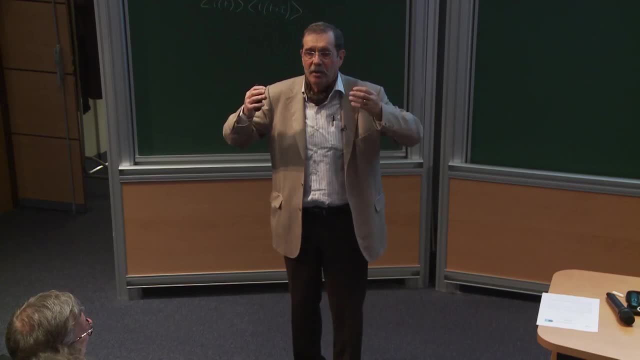 between two particles in four modes. Hong Wu and Mandel is entanglement between particles in two modes And for the Hong Wu and Mandel it's entanglement between two modes And for the Hong Wu and Mandel it's entanglement between two modes. 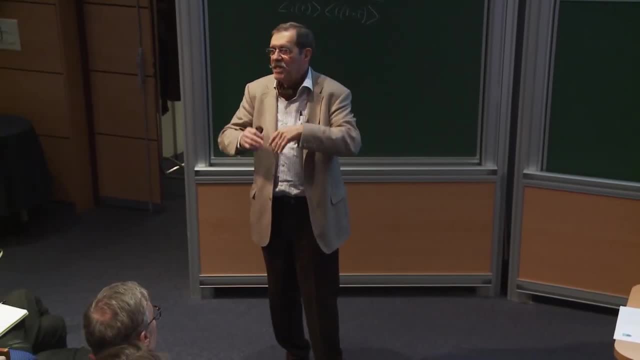 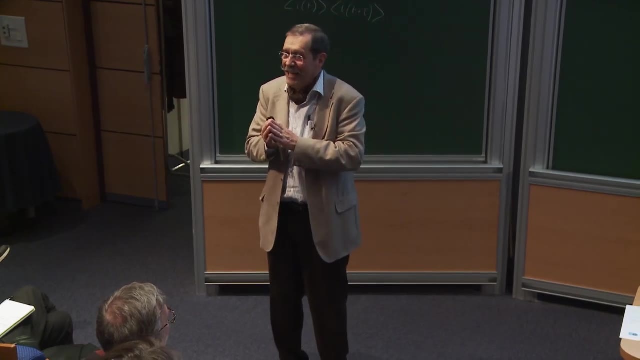 And for the Hong Wu and Mandel it's entanglement between two modes. So I can invent a classical model, that with hidden variables. but I can invent a classical model that will reproduce a result For Bell's inequality violation there. 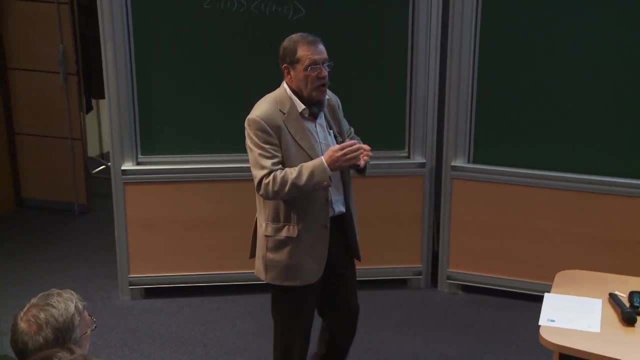 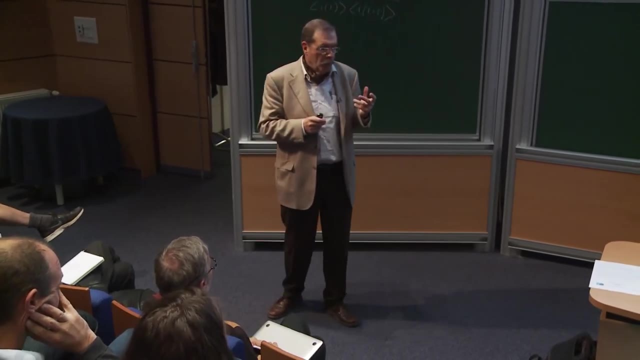 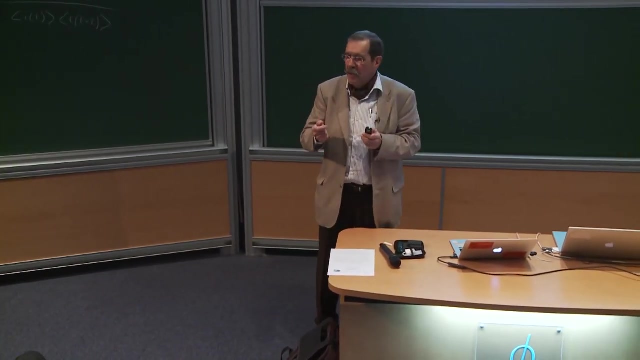 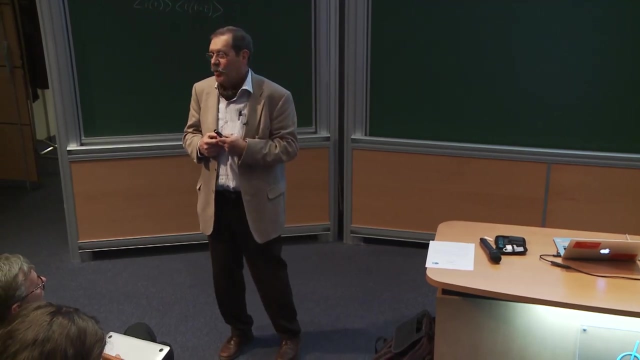 is no classical model to reproduce the result, unless you accept nonlocality, which is another story. So what I want to show you is that by doing experiments, people like me are forced to think. They are forced to think, to think deeply about impression, intuition that I had. okay, I had the feeling, but because we have 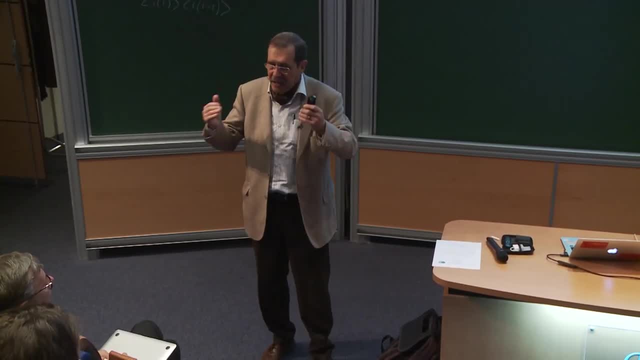 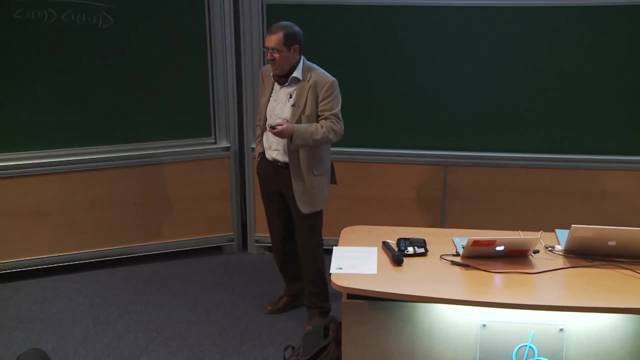 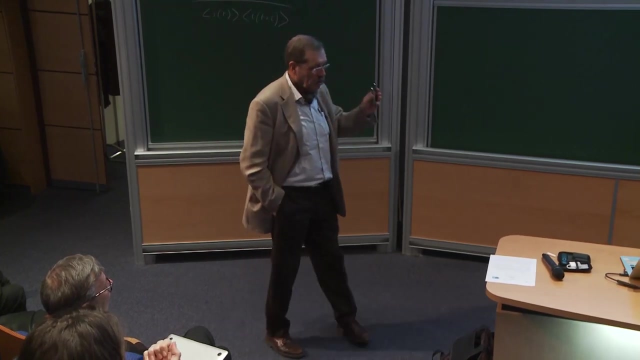 an experiment, I am forced to think deeply, And so I think it helps to better understanding quantum physics. And when you better understand quantum physics, maybe you can develop applications. And this world of quantum information of which you hear a lot. there is a lot of hype, too much. 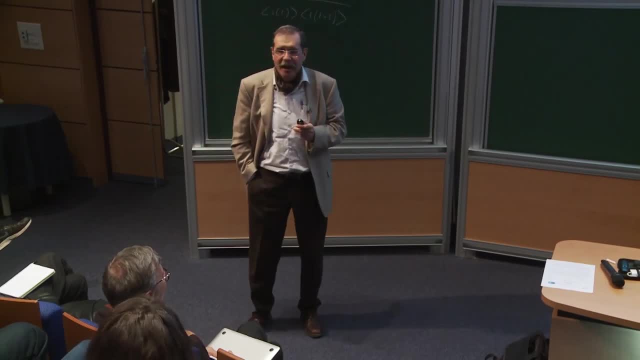 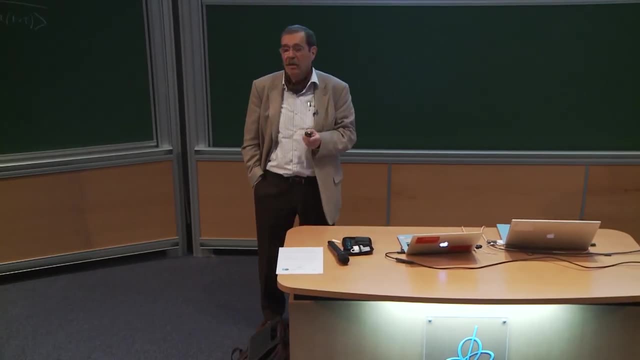 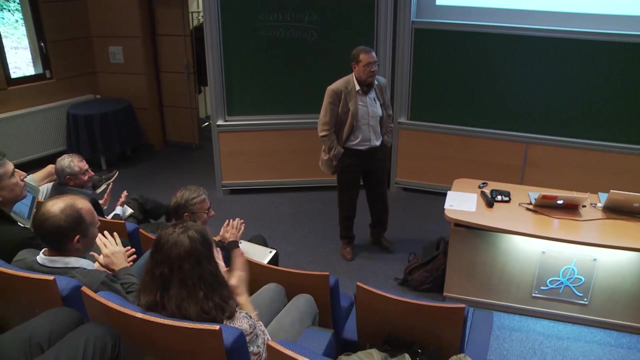 but there is also something in quantum information, And I think that quantum information really benefits a lot by this kind of reflection. So I think I will stop here because you are probably tired, but I am open to any question you want to ask. I don't know what I can show here. 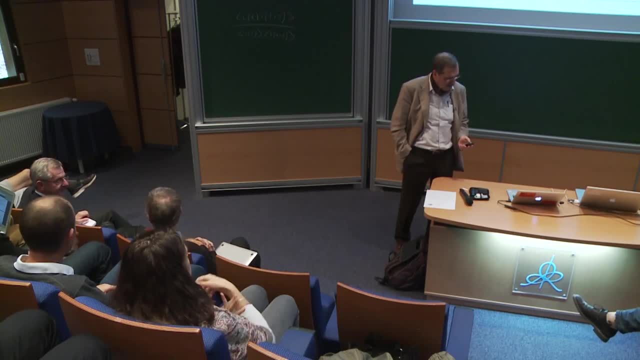 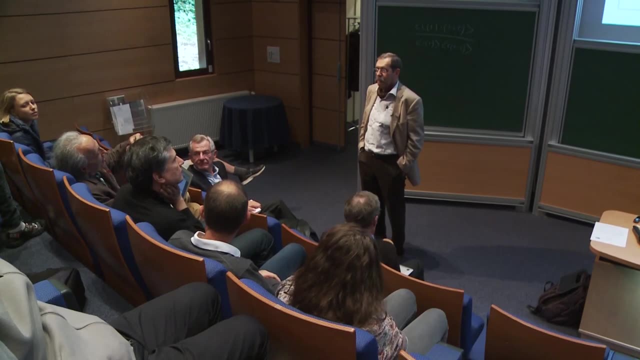 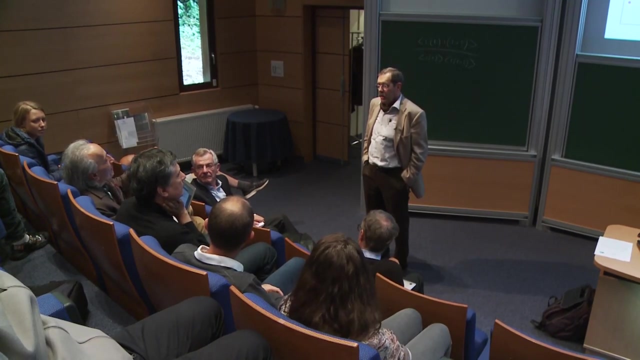 Alan. by the way, the fact that you have these P minus P, you have these states with correlated things. It's what Einstein, Podolsky, Rosen were imagining. They were using special states which were correlated with. Could you? 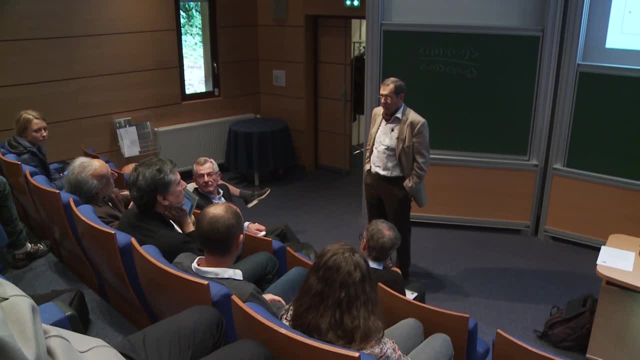 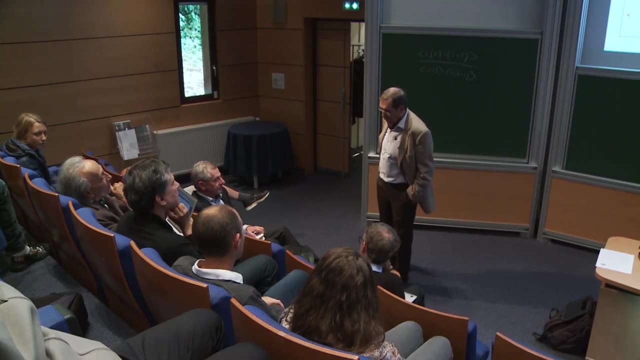 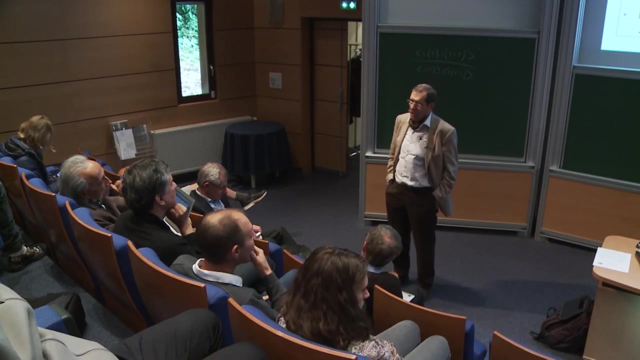 then realize what they wanted to show. you could measure positions and non-communicating things, just from the conceptual point of view. You write, of course, until a certain point, but it's not exactly the EPR wave function anyway. But the second, the most important point is: 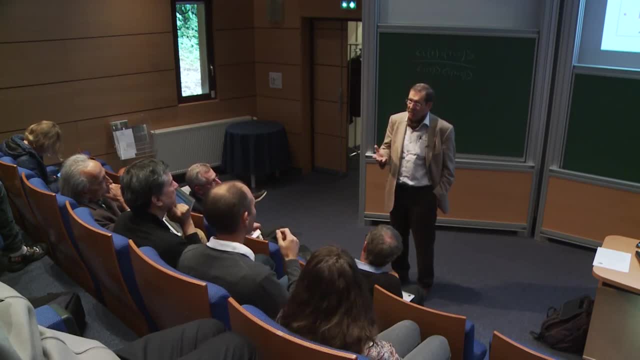 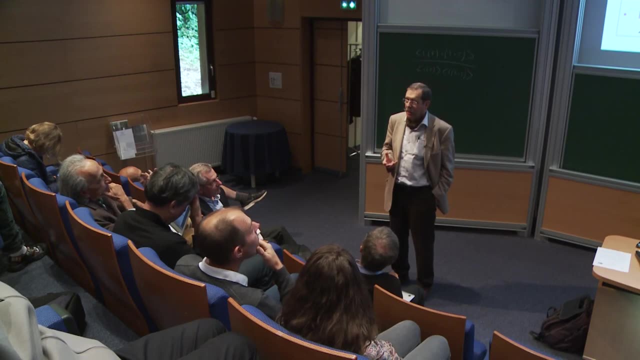 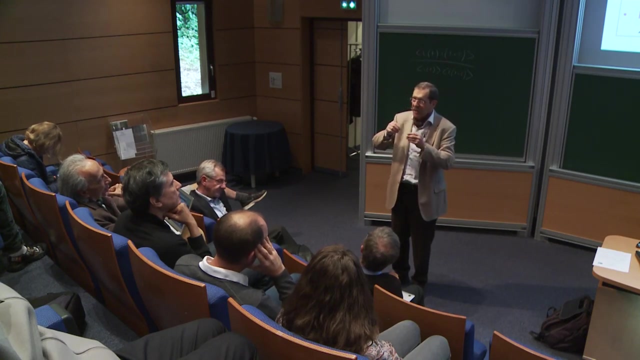 in the EPR situation you have continuous variables and its correlation between continuous variables. But as far as I know, to test Bell's inequality you must have discrete things, And our trick here is just like with the photons: We select two modes. 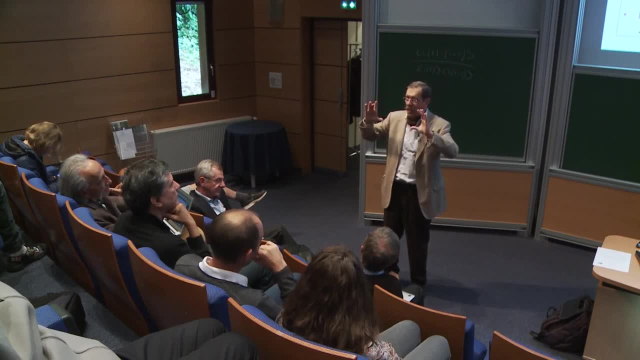 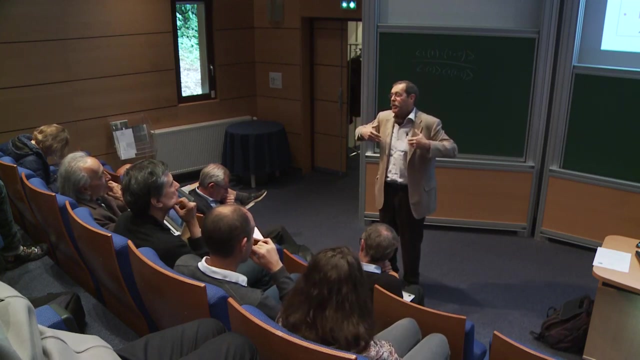 And then other the two modes and now we have four modes And I think that until the moment when you have four and only four modes, you cannot test Bell's inequalities. So it would be amusing to do that, but of course because of my personal history I think 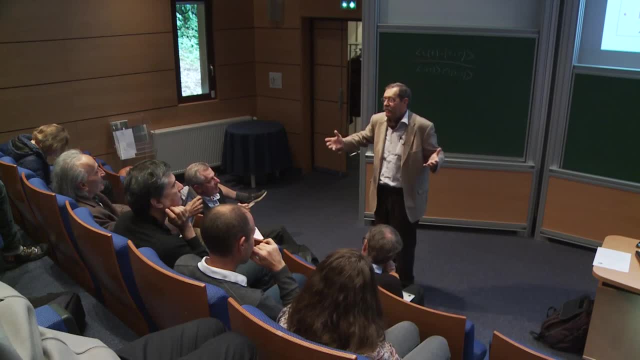 But I think that Bell's inequality, a Bell's inequality violation, is really the most quantum thing we can cure. 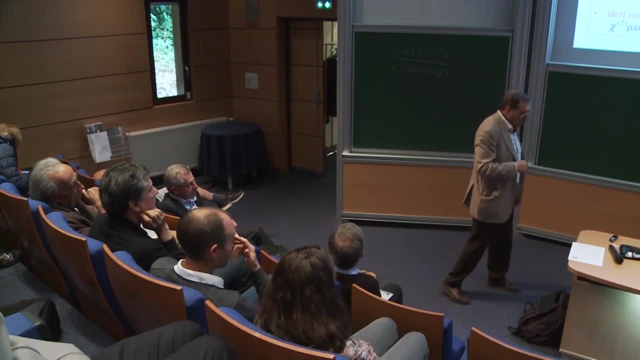 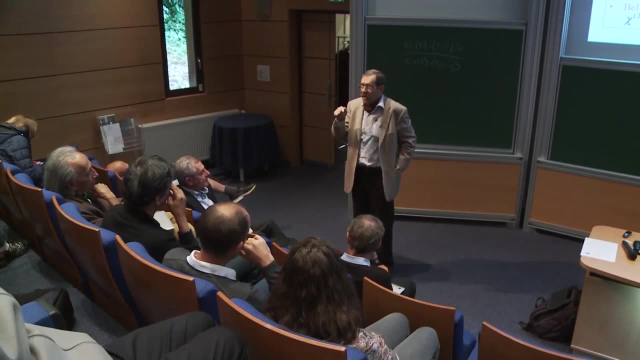 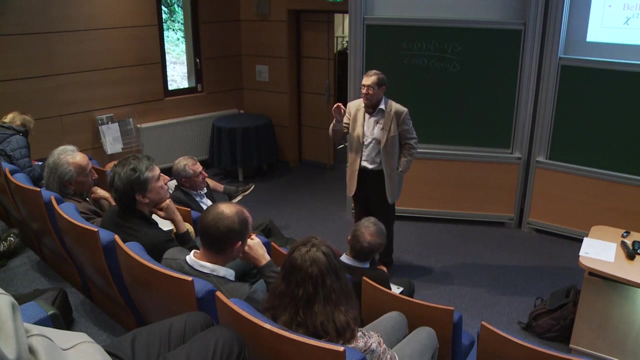 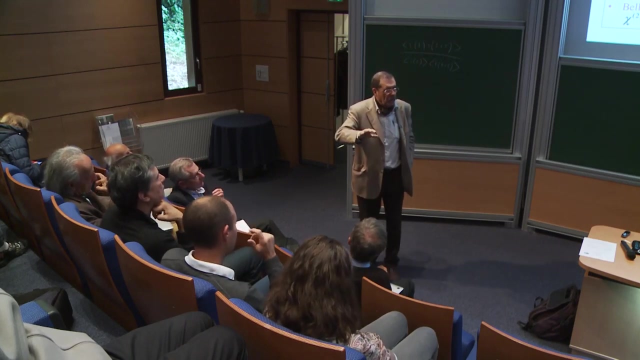 can think of. I think that the real value of the EPR rezoning paper, whatever, is to draw the attention on the fact that two-particle quantum effect is dramatically different from single. And if we think of the history we all know, of the Solvay conference of 1927, when Einstein was 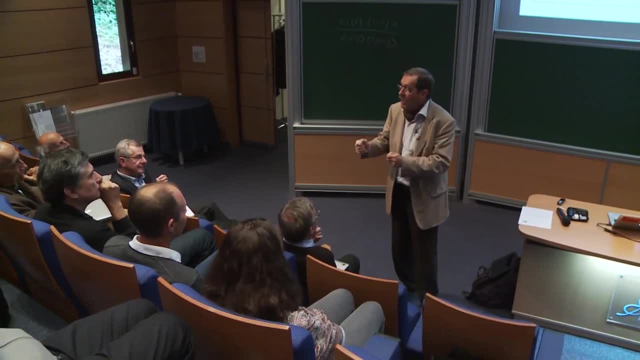 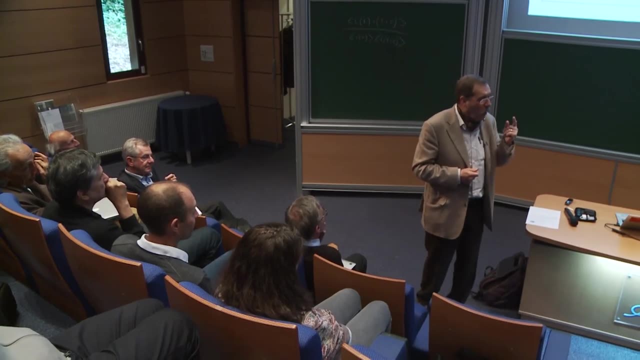 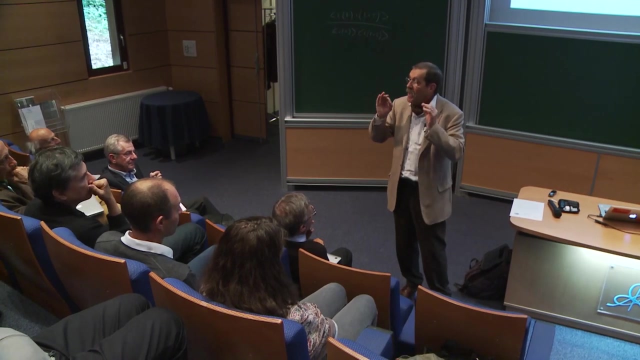 coming with an objection to Bohr and Bohr would reply, And the replies of Bohr were fully convincing in that case. And all these attacks of Einstein were based on quantum effect of a single particle. He was dealing with Heisenberg. It was always a single particle And he always failed. 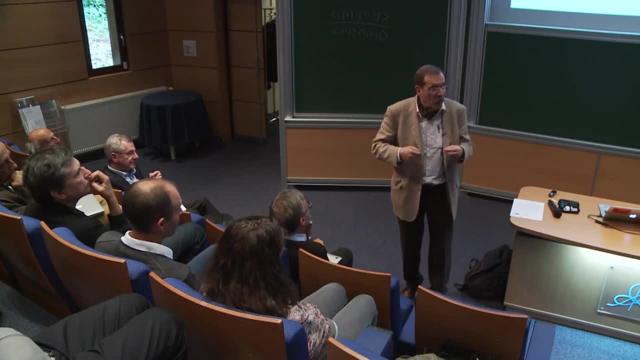 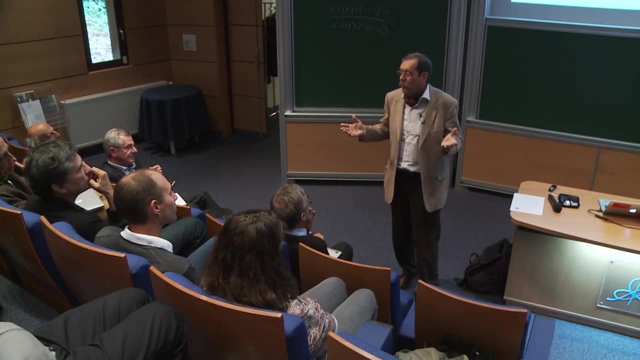 in his attacks with single particles. But when he came in 1935 with two particles and with entanglement, then he was able to do it, And he was able to do it, And he was able to do it. And then we must say honestly, the reply of Bohr to Einstein is not very convincing. 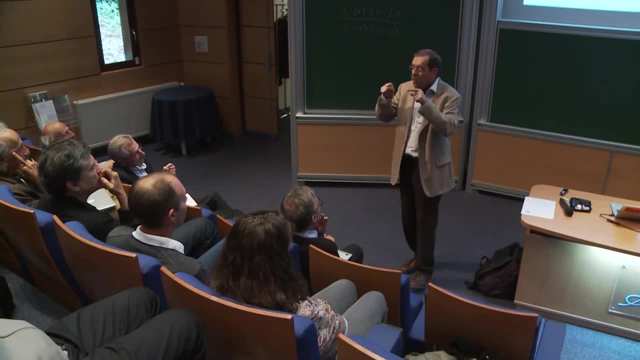 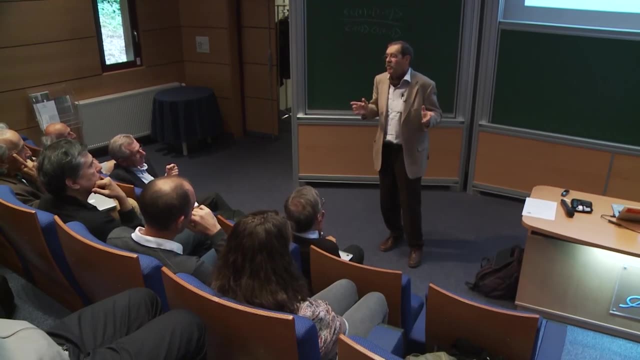 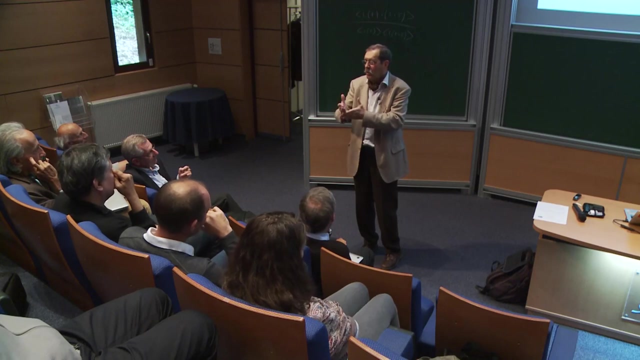 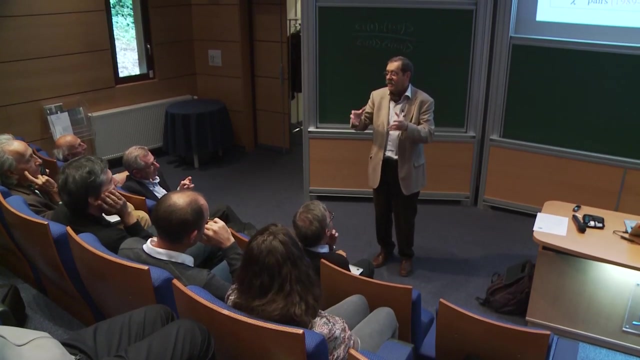 So the beauty of the EPR paper is to have shown that when you start with two particles then you have a different problem, totally different problem. But then we must give credit to Bell for coming with a really quantitative distinction between the classical world and the quantum world, And even Feynman, in 1982, when he realizes that 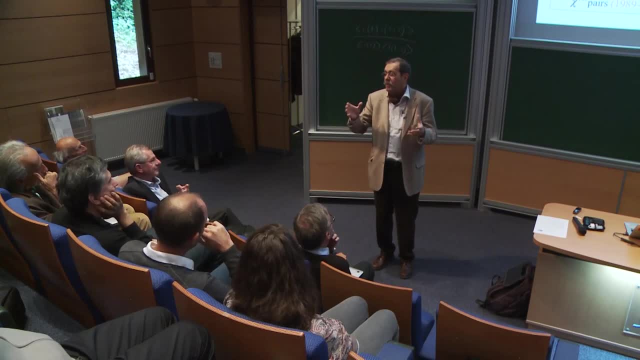 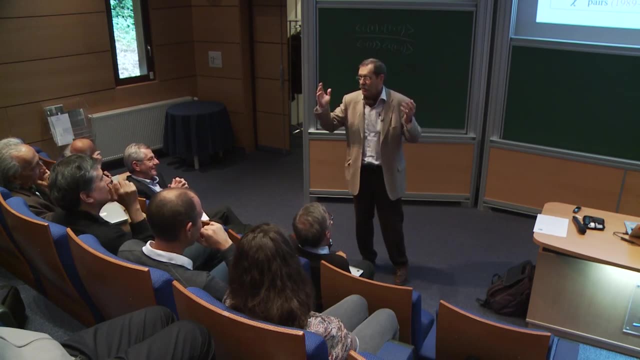 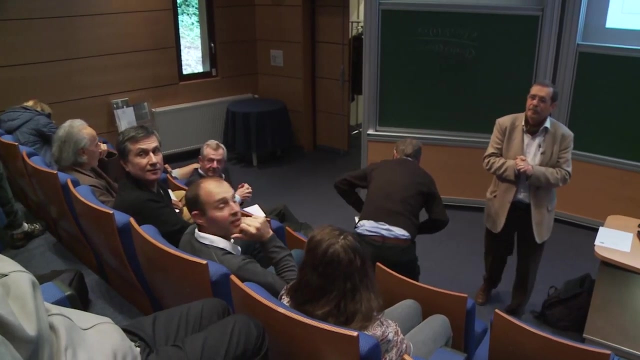 entanglement is different. he writes something which is like Bell's inequality, And of course Feynman does not cite Bell, because Feynman re-events everything, so he does not cite anybody. But we can forgive him. So why are you so reluctant to this last experiment? 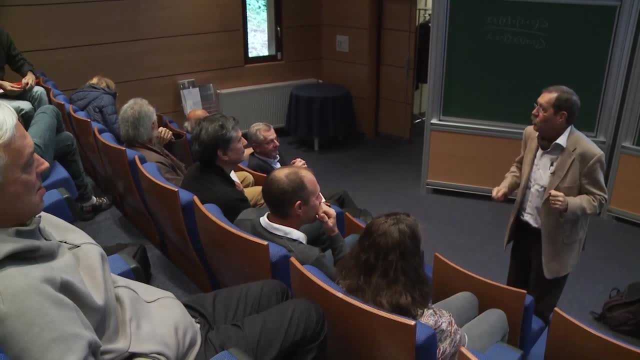 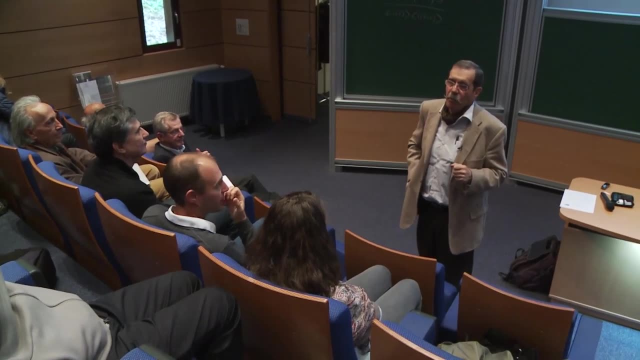 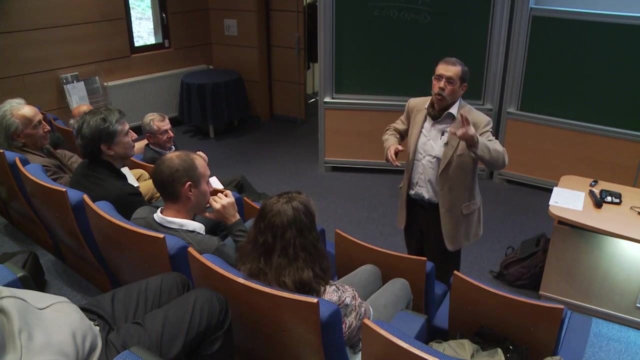 I'm not reluctant. Why I'm reluctant? I'm going to tell you, but don't repeat it. In 2015,, there were three experiments which made a lot of noise about so-called loophole-free tests of Bell's inequality. Two of them gave a violation of Bell's inequality by 10 standard deviation or 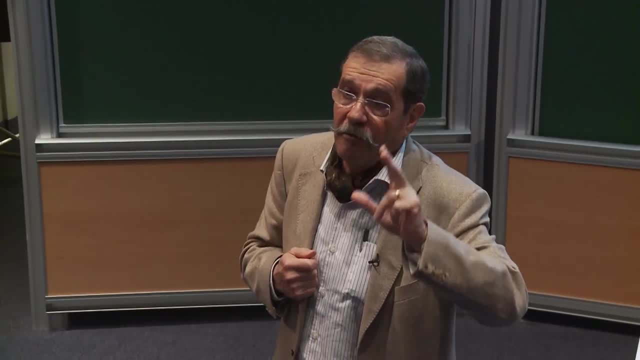 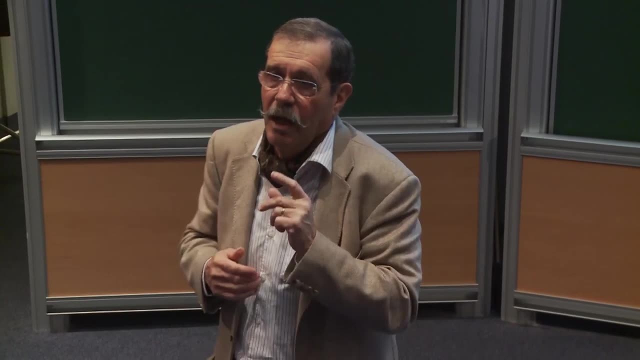 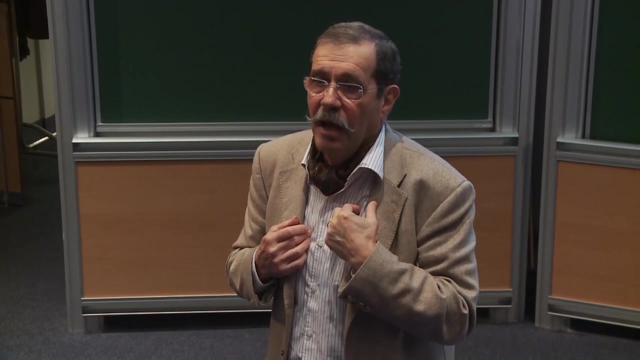 something like that. But the third one, which made a lot of noise because it was published as the first one by Nature and Nature made a lot of noise about it, etc. violated Bell's inequality by two standard deviations. But that's not a big deal. I think it's a big deal. 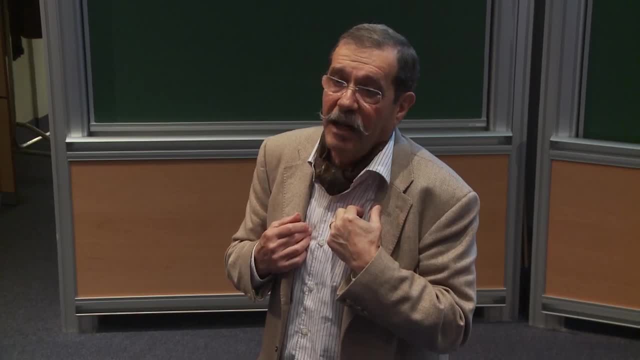 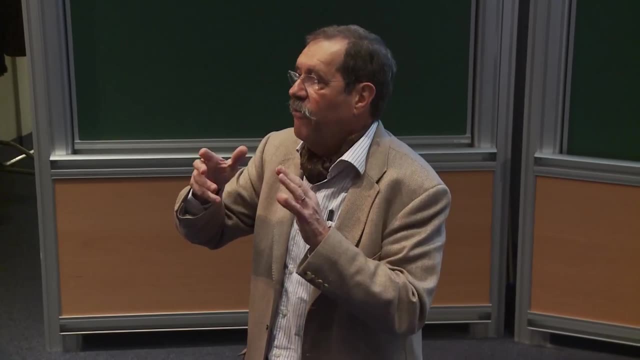 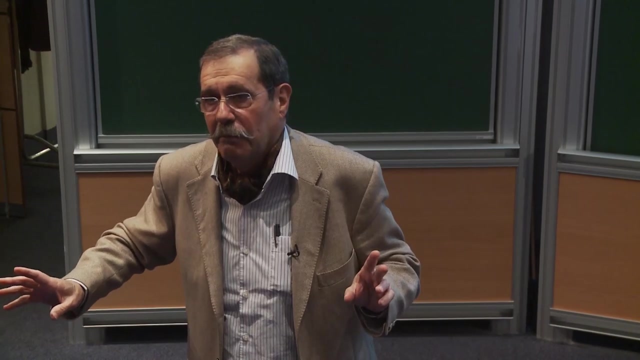 If I were to pass a reasonable experimentalist, I would never claim something seriously if I don't have five standard deviations In CERN. when they have a bump, when they have two to three standard deviations, they leak the information that maybe they have something When there is. 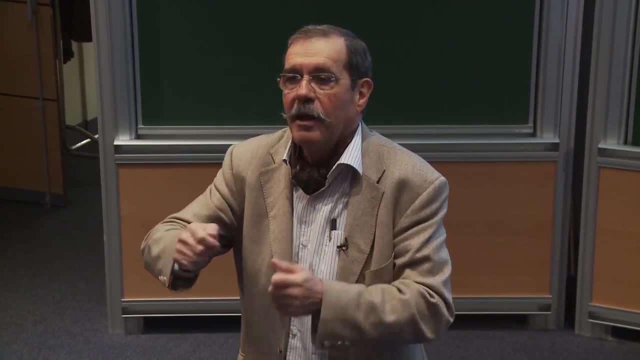 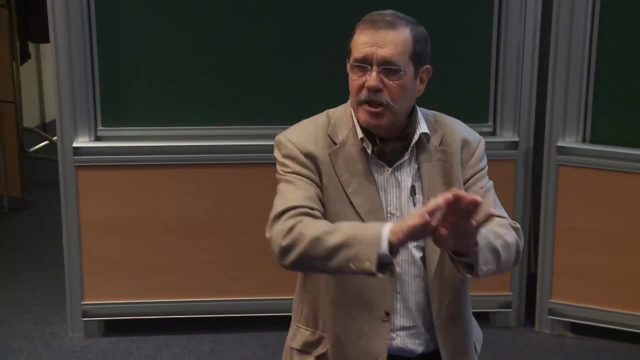 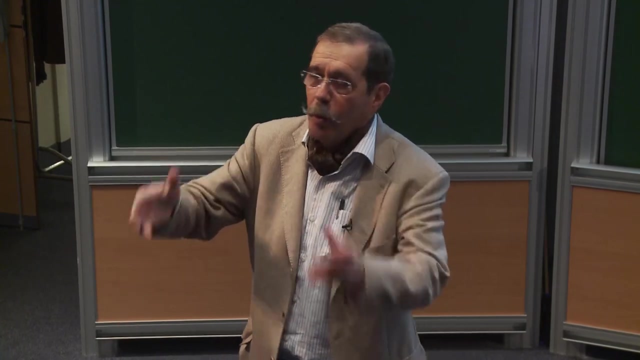 a bump with a signal-to-noise ratio corresponding to five standard deviations. So because I show only one standard deviation, I say my result is compatible with, but I don't claim anything more like that. I'm deeply convinced that in a few months we will. 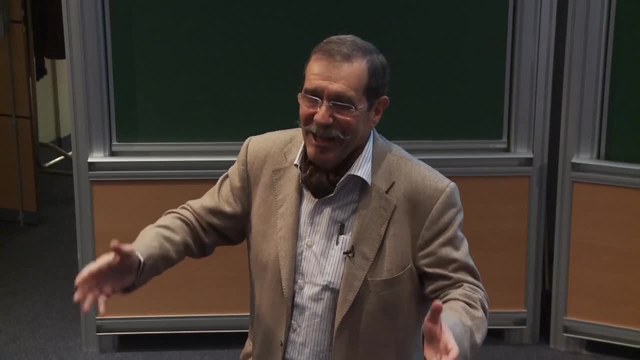 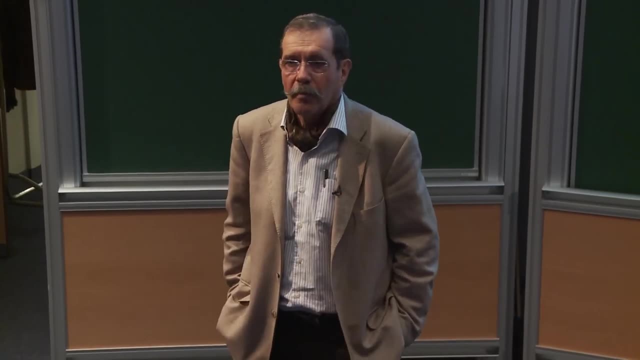 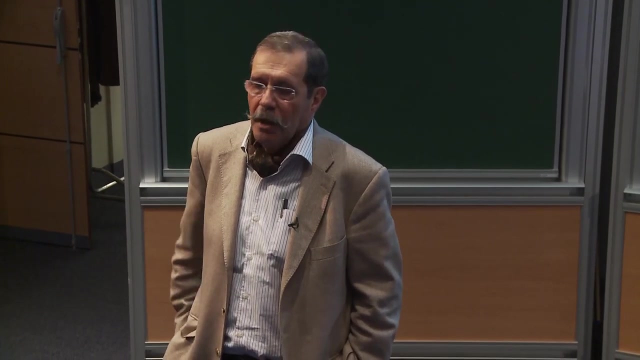 have a result with a large enough number of standard deviation and, in addition, we will have a control of the relative phases. So thank you to ask the question And I was asked to write. you know now it's a trend to have comments about the paper. 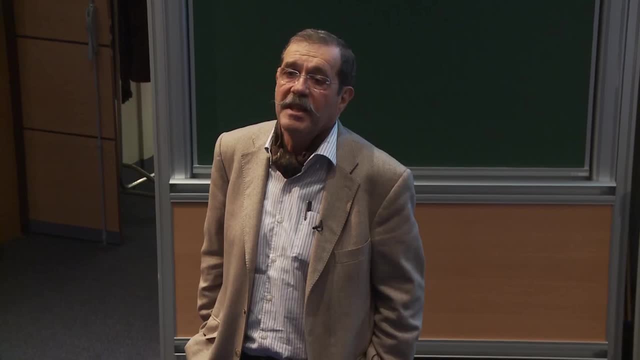 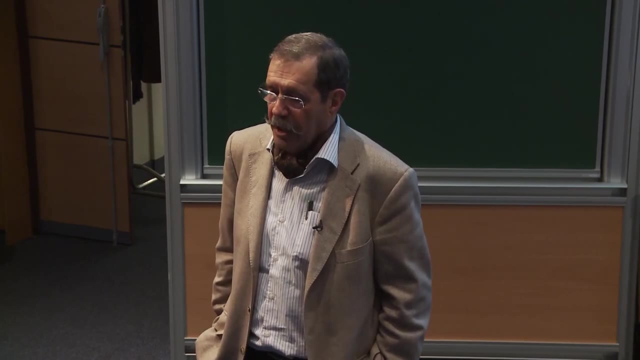 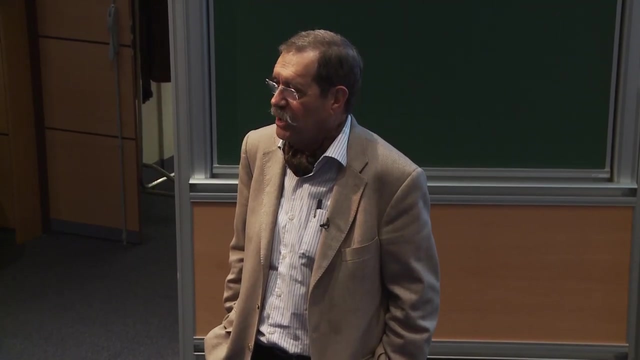 So I was asked to ask comments about this re-experiment in 2015.. And I wrote a comment in the not in Nature because I was not happy with the way Nature processed all that. I cannot say details because I am a referee, an anonymous referee, so I should not give. 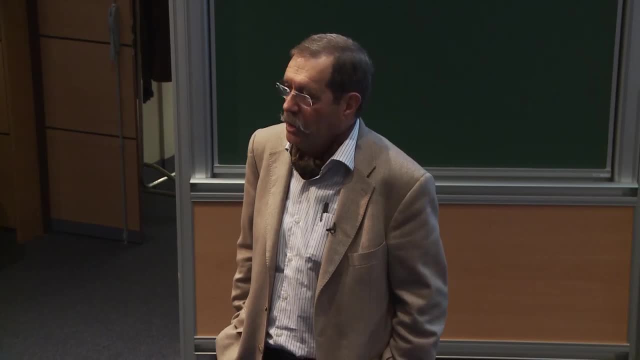 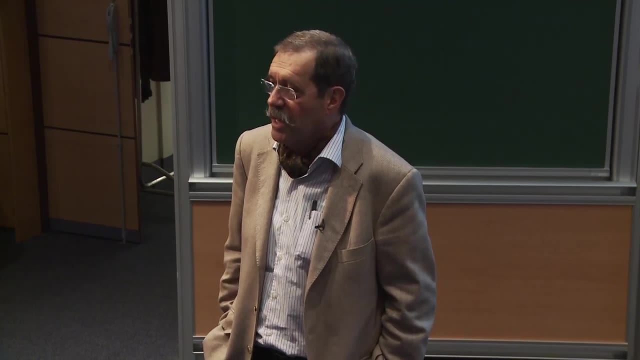 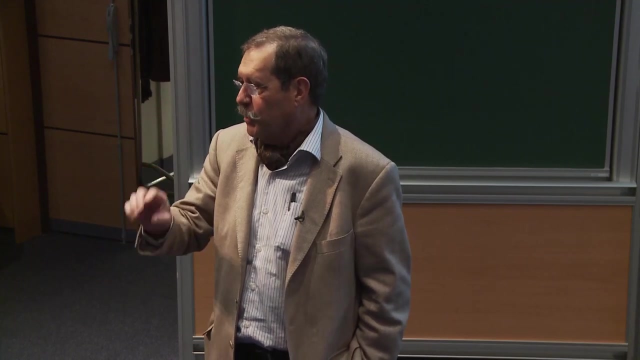 details. But I was not happy about the way Nature processed all that. So I wrote a comment in an American Physical Society journal which is named Physics, where my position is very clear. I put exactly: what are the standard deviations in each experiment, et cetera, et cetera. 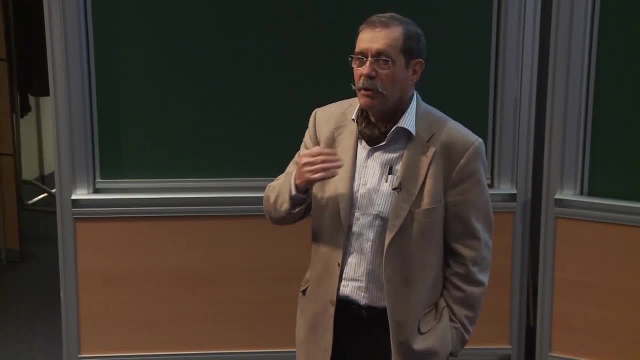 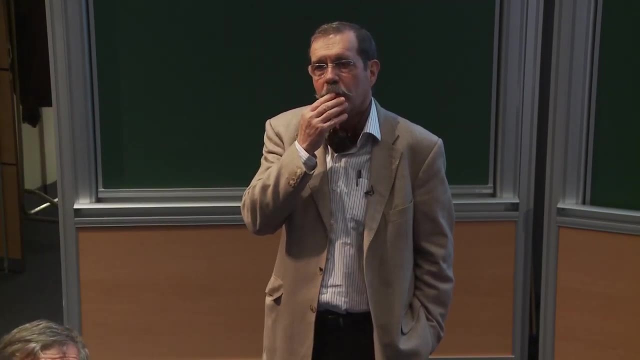 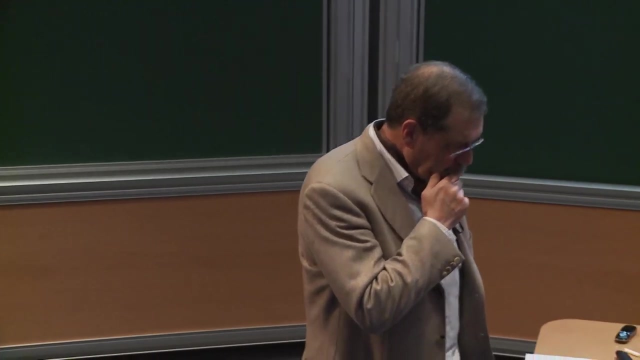 If you read me between the lines, you understand that the three experiments are not at all of the same quality. Okay, On the second hand, I would be really interested to see real applications of all these different Oh. So the first application is quantum simulation. 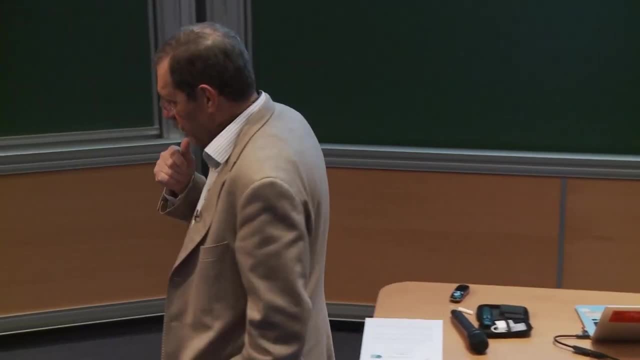 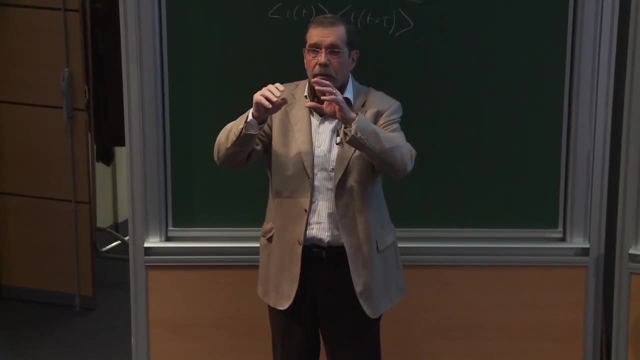 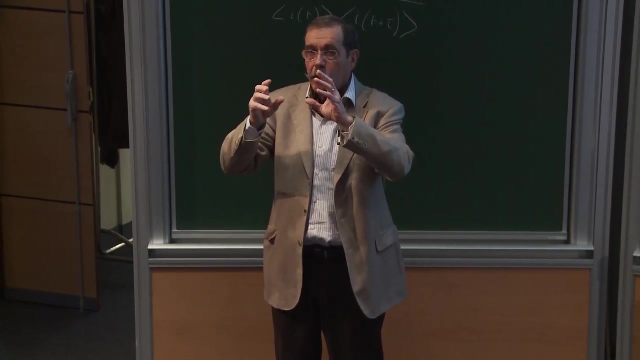 For instance, my colleague Antoine Boes, which, by the way, is a former PhD student. he has now a network or, I don't know, a lattice of 50 atoms, And for these 50 atoms it can create entanglement at will. 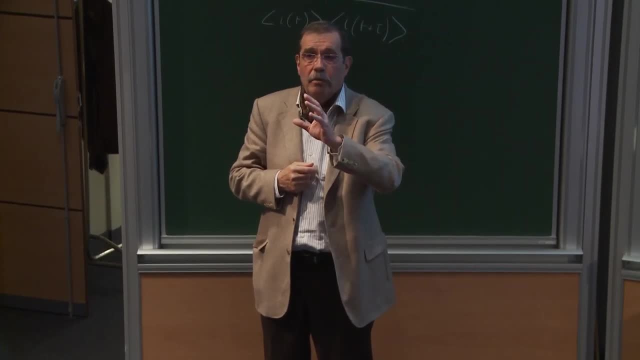 So it is a problem which is a many-body problem. He can get into a plausible workshop, no matter what he does. He can't get into one of everybody's lives, but he can't get inside anybody else's harbours. Where there is oneerders' world, there's oneerder's world. 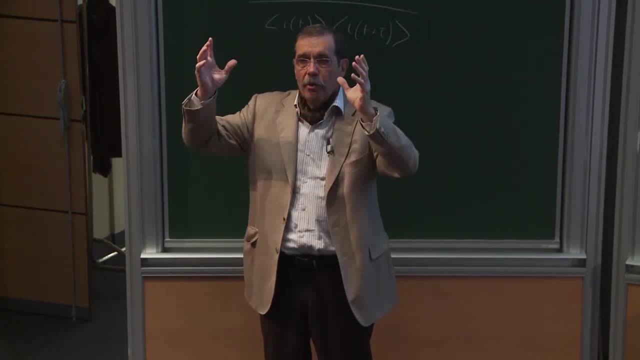 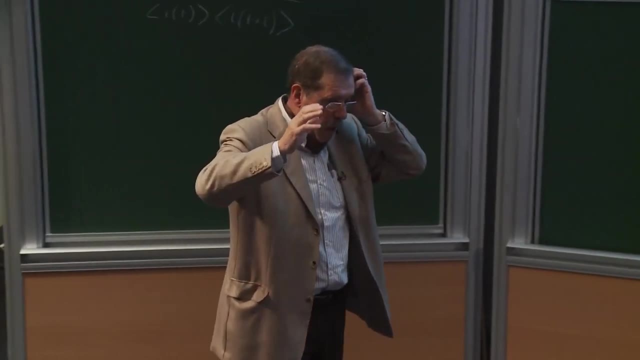 About the destrohymes you just saw in the documentary, which I know is the police brain right now. In the end this could be written again, of course, by sound, But that's still another problem for which you cannot do any calculation with a computer, because the size of the Hilbert. 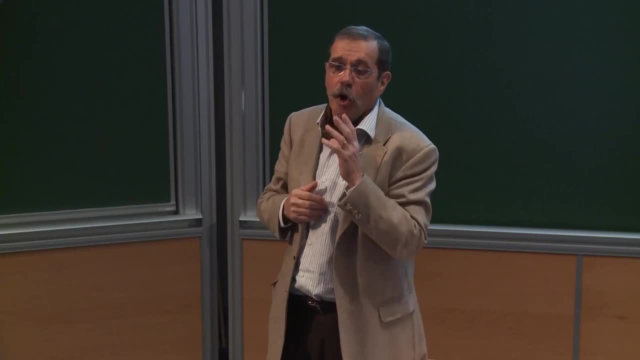 space, the many-body space described in that is, as you know, there is exponential explosion, et cetera. Curiously – I have not looked into details, but I trust Antoine Boes and the people who worked about that- It seems that this kind of thing cannot only help to understand the problem of condensed 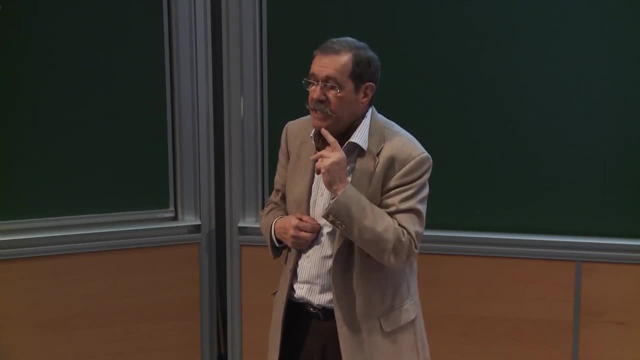 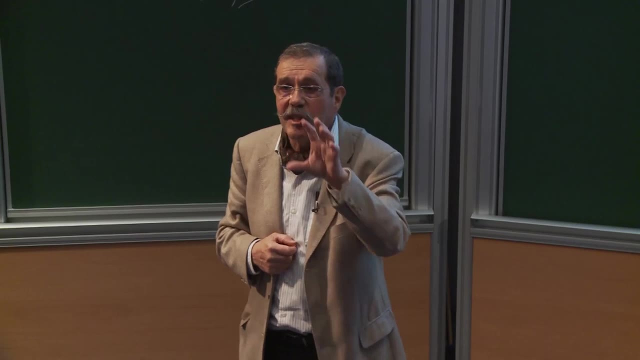 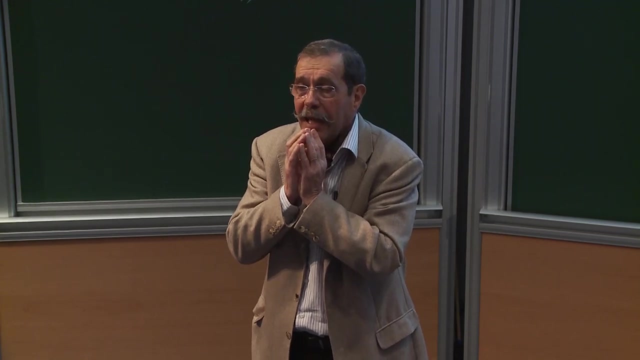 matter better than that. It seems that there are optimization problems, like the traveling salesman problem or stuff like that, which could be solved with this kind of quantum simulator And, for instance, I understand that EDF or the electric company are subsidizing this kind of. 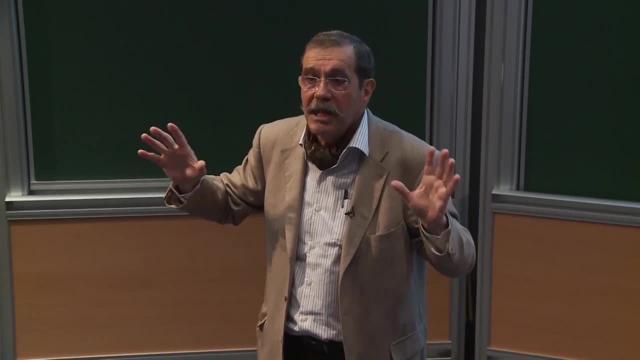 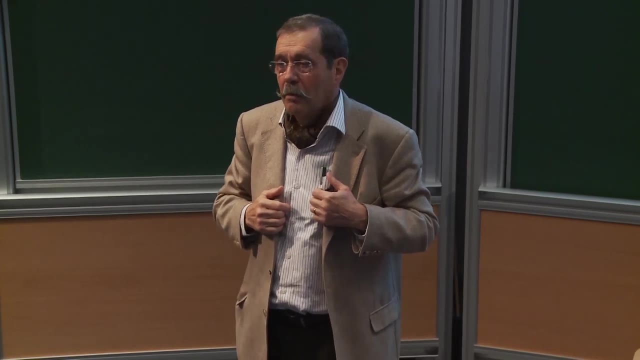 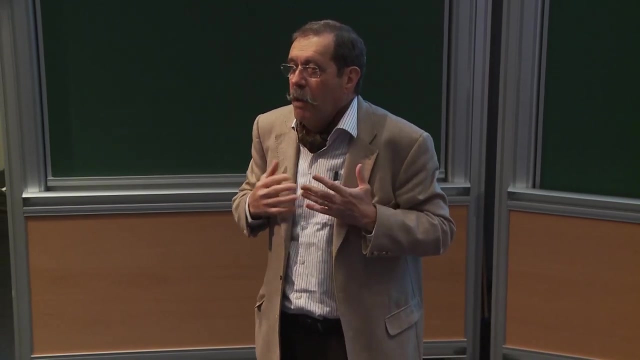 research, because the optimization of the grid is a big problem for them. So I don't say that it works, But these are the kind of ideas that people have And big, complete problems. Yes, exactly, Yeah, exactly. Don't ask me details, But serious theorists claim this kind of thing. 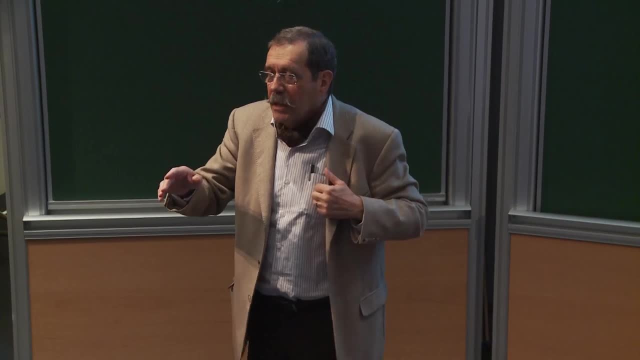 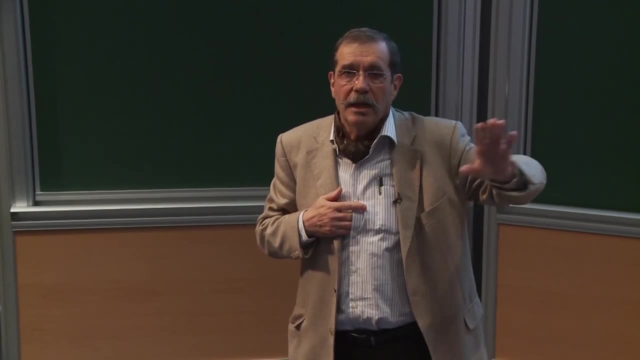 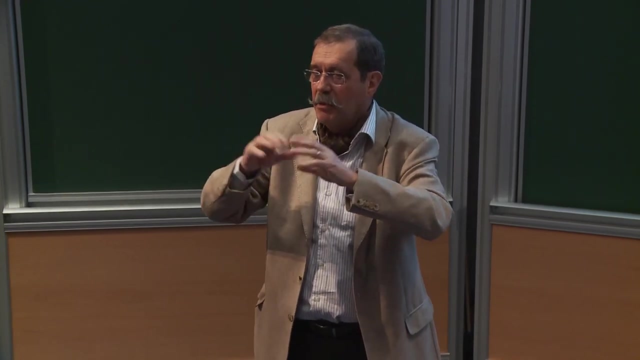 And you know, the most obvious thing is to say: I can treat – this is what I do. for instance, I do Anderson localization. Anderson localization is a problem of condensed matter, physics: As soon as you pass a certain degree of complexity, three-dimension, etc. there is no exact. 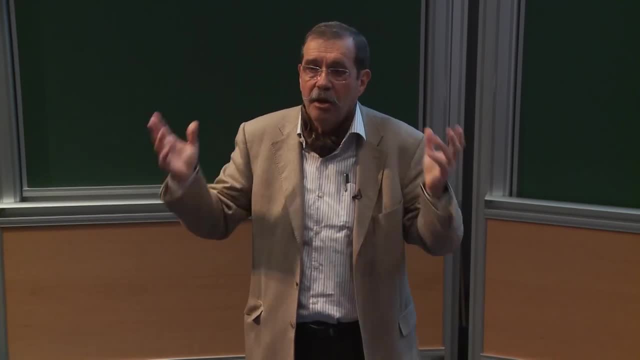 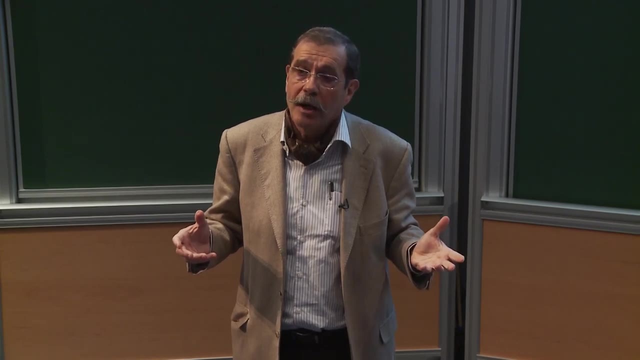 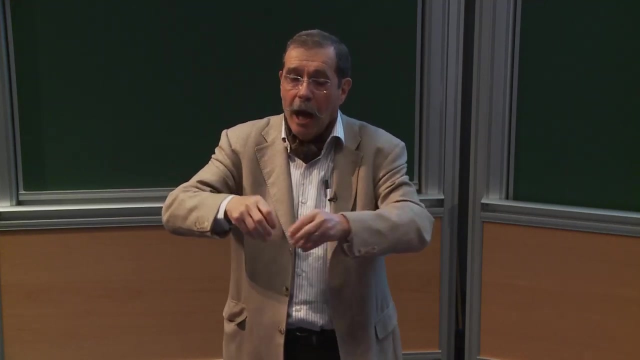 theory for treating it And there is no computer big enough, with a big enough memory to make a numerical calculation. We do the experiment with ultracold atoms replacing electrons. So I simulate a lattice with standing waves of laser. I put ultracold. 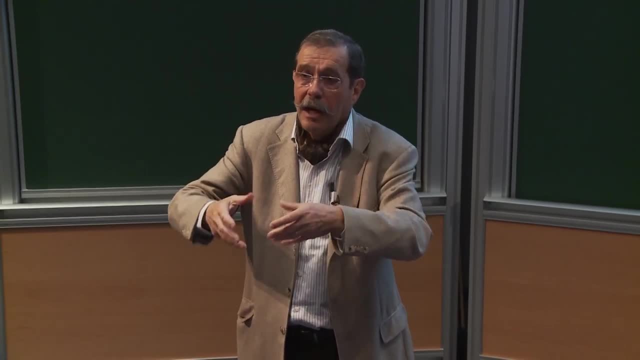 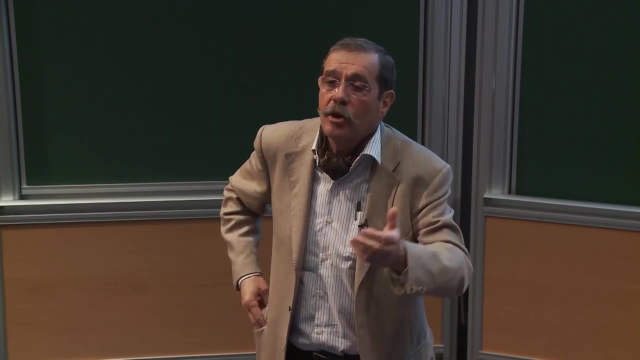 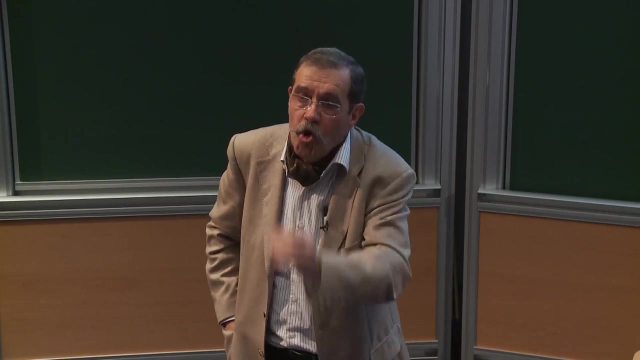 atoms, which simulate the behavior of electrons, And I look at what happens. So it's a – I don't – wait – simulator. It's analogous calculation, But it's analogous calculation in a situation where we know that no computer ever will be able to do it, because it would demand. 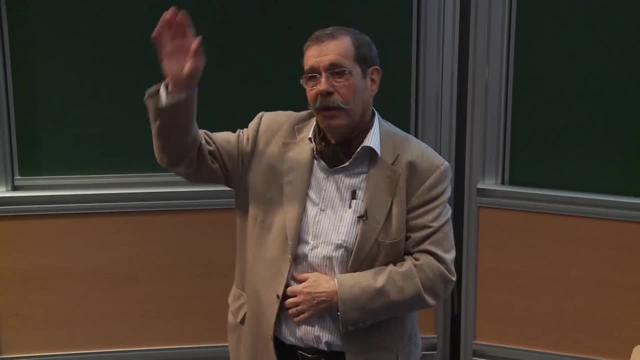 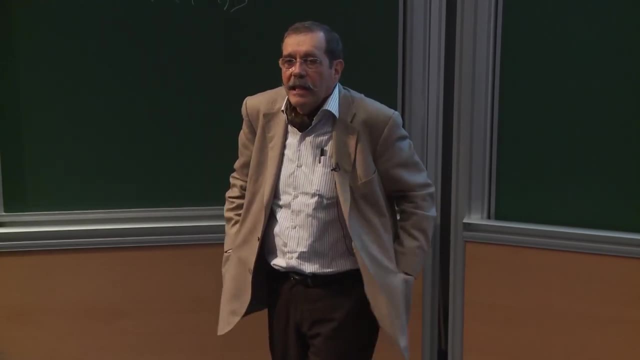 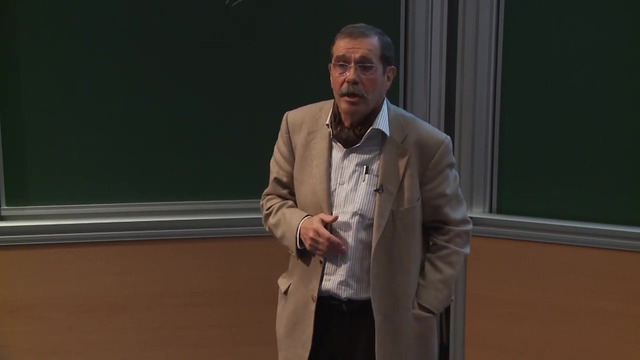 the number of bits, as large as the number of – I don't know – atoms in the universe, or something I know. people write big numbers, etc. So the idea is to try to do something, But the question of the of optimization of the grid seems to be serious enough that there is money invested on that. 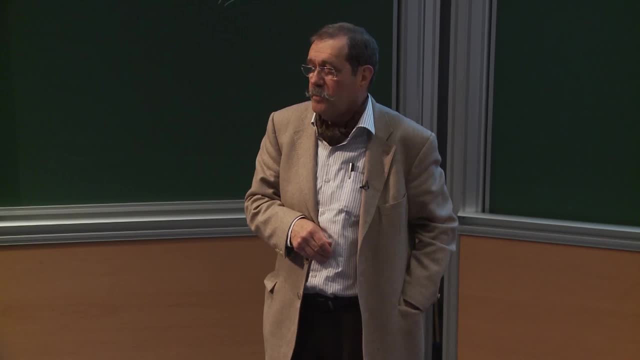 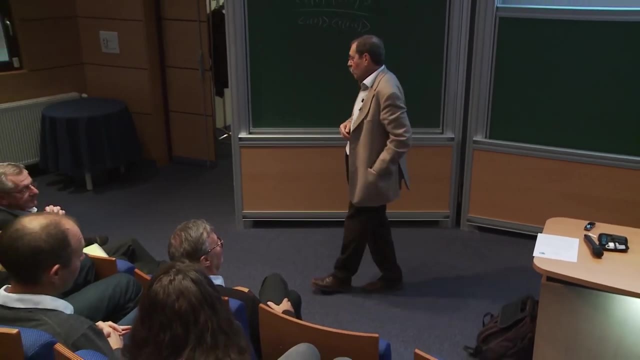 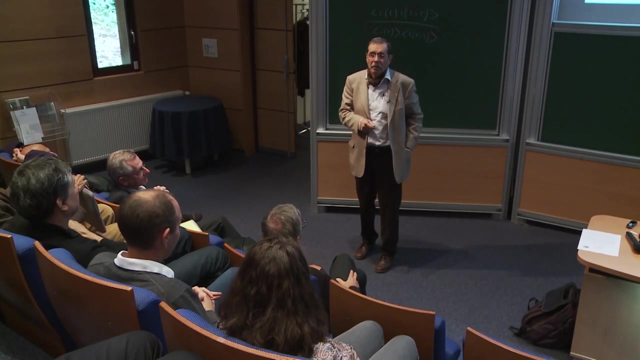 Don't ask me more. There is, of course, quantum cryptography which is based on- Well, the safest method of quantum cryptography is based on entanglement. There are methods which are not based on entanglement, but they are not as safe. 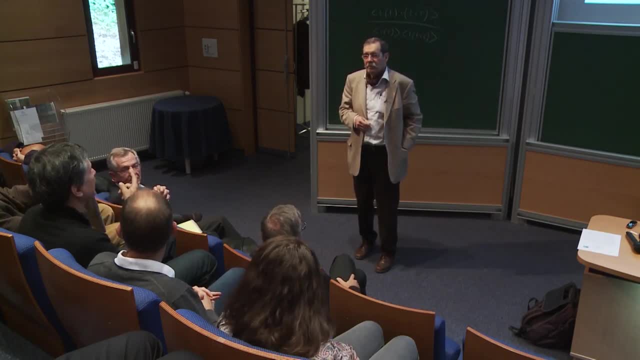 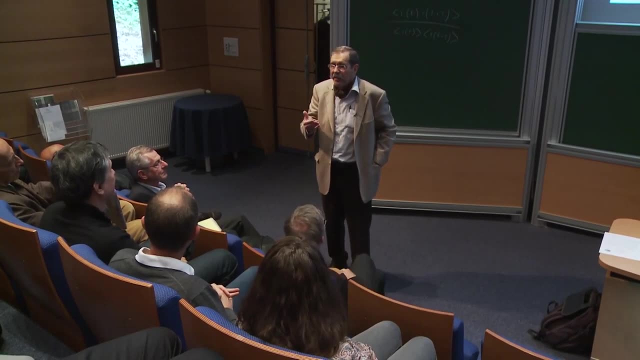 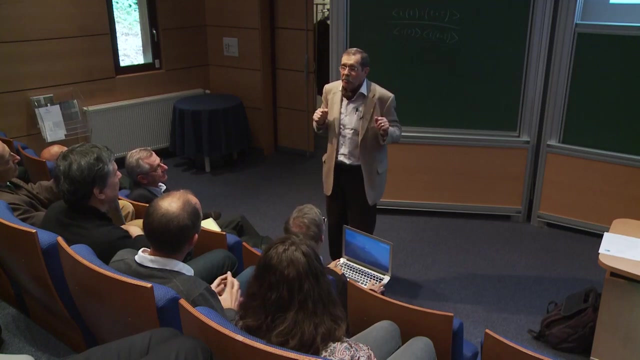 This is our Chinese writers. Yes, this is hype. From the text that they publish, you cannot guess what it is. They speak of subatomic particles. My best guess is that it is just light, and so a photon is a subatomic particle. 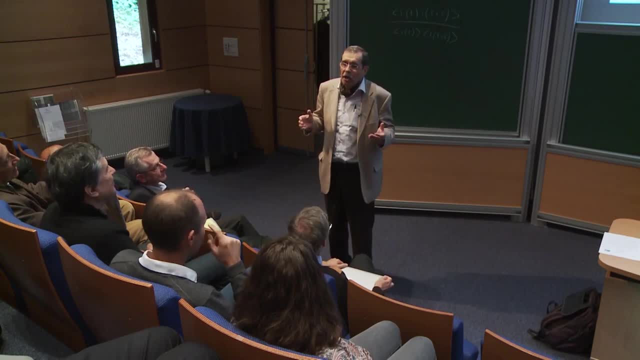 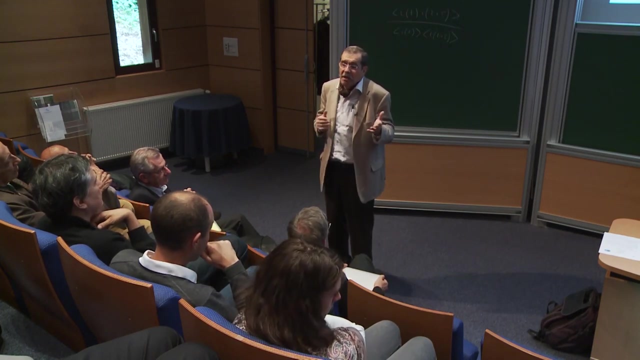 And then they don't say what they do. But look in classical logic, in standard optics. well, in usual optics, let's say, we already know how to go to the standard quantum limit, and we even know how to pass the standard quantum limit. 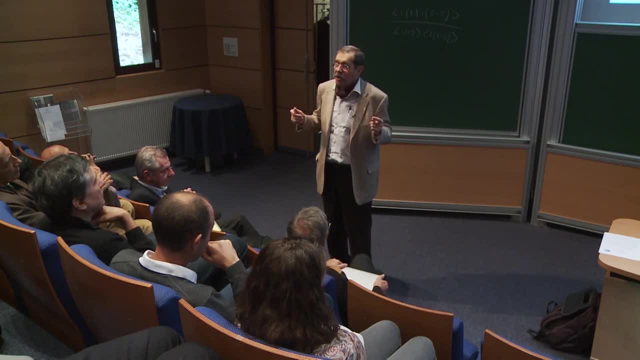 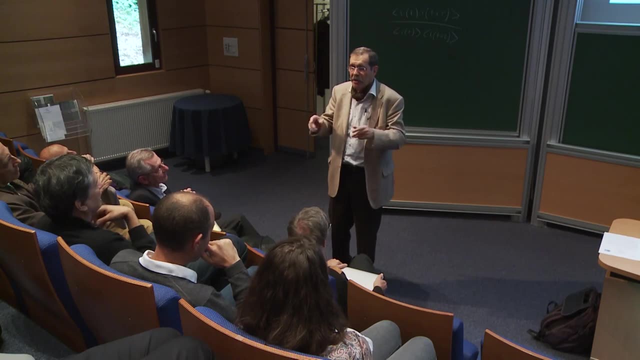 So it may be an experiment of that kind. We have the exchange with colleagues and we have decided that we don't waste our time until they publish a preprint. When they publish a preprint, it's not a preprint. Let me specify it for you. 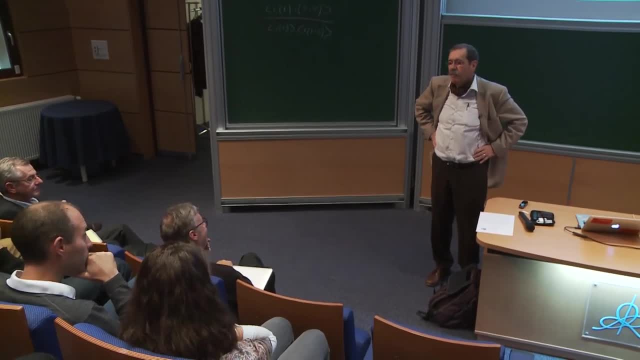 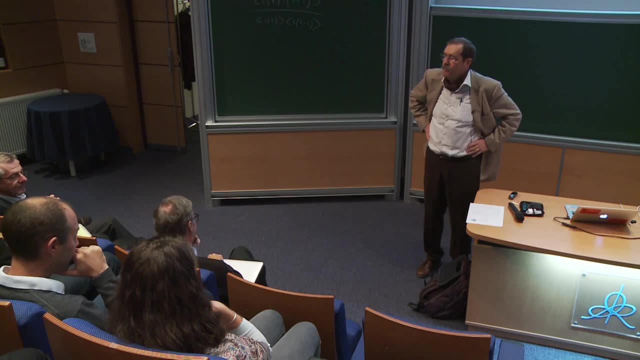 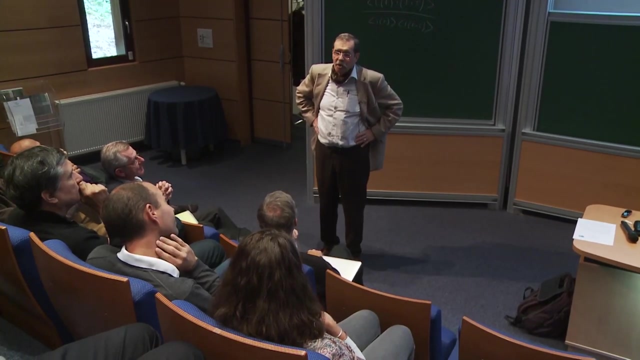 Okay, we'll see. I think it's part of the hype about quantum information. It's too much. I don't like this way of doing physics. but okay, You know, I have been one of the people who have advocated the emergence of the famous quantum flagship at the European level. 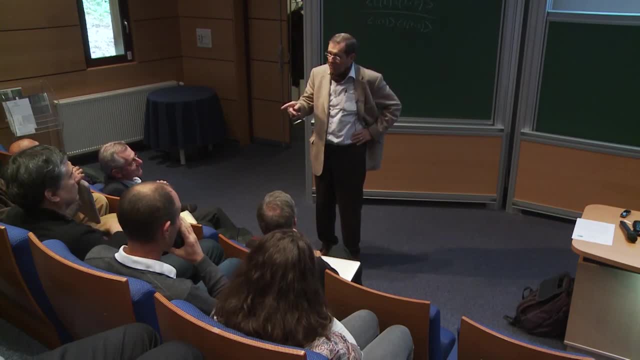 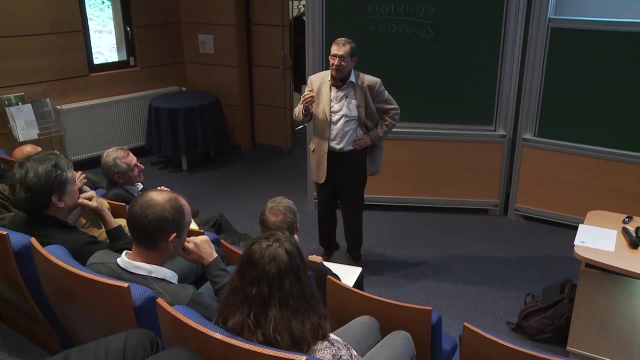 I have presented my ideas several times- He knows he was there once- in front of the commissioners. I always told them the following: I feel, regarding the universal quantum computer, as I felt 30 years ago regarding the detection of gravitational waves: Okay, 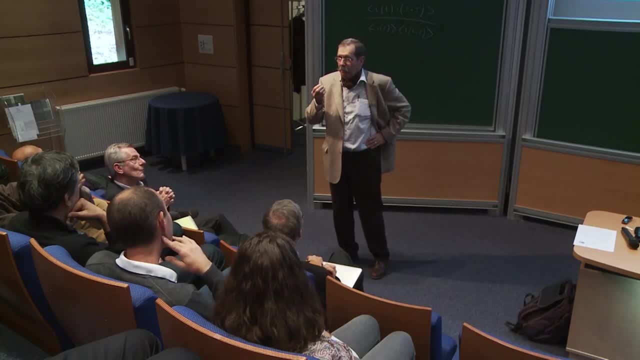 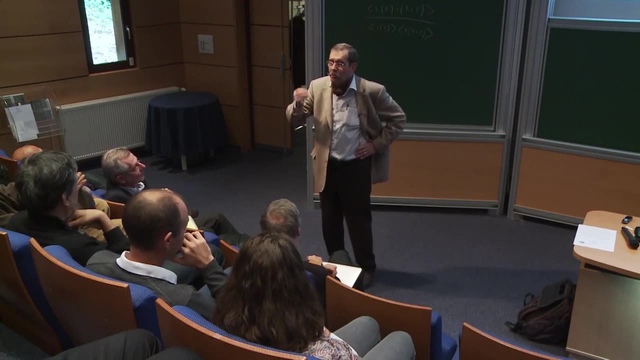 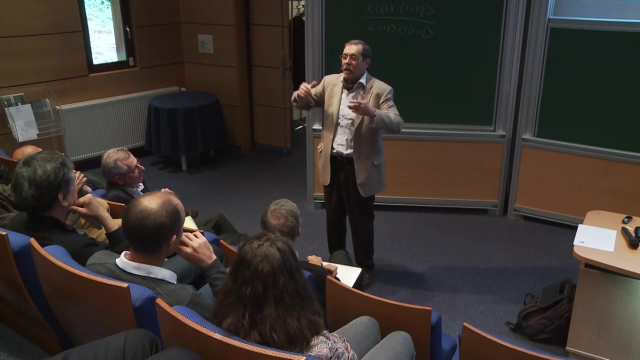 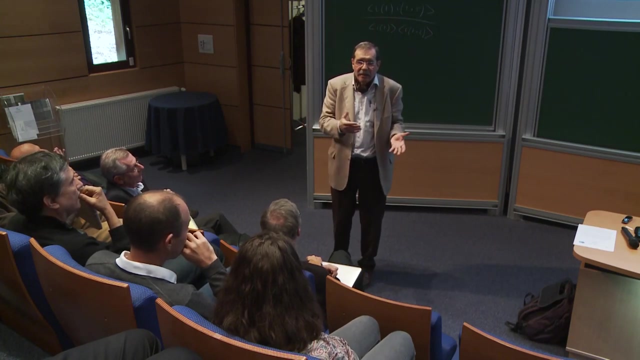 No fundamental theory, or property or theorem- whatever property- tells you principle. No fundamental principle tells you that it is impossible, but the technological gap looks immense. I feel the same regarding the universal quantum computer. I don't know any fundamental law of physics saying that it is impossible. 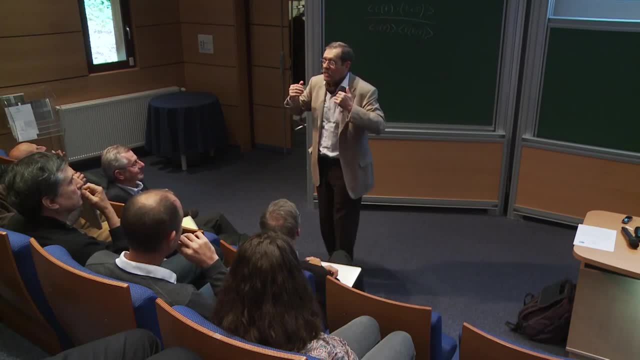 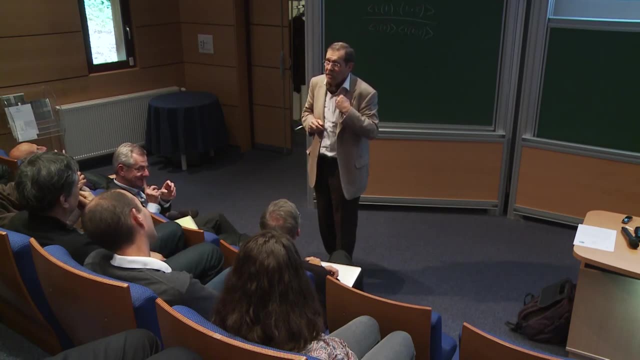 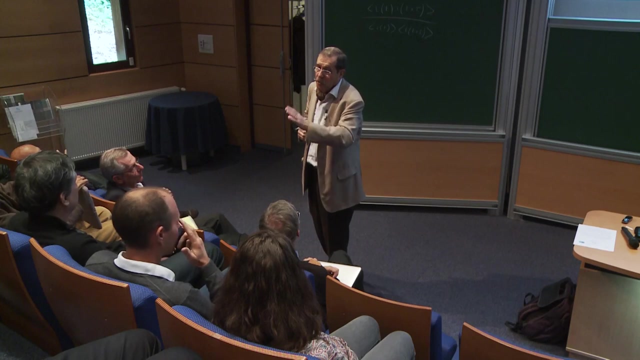 but I have no idea as we can succeed. Okay, I said that several times in front of the commissioners, but some of my colleagues were promising to deliver a universal quantum computer within five years. I can tell you there will be no universal quantum computer in five years. 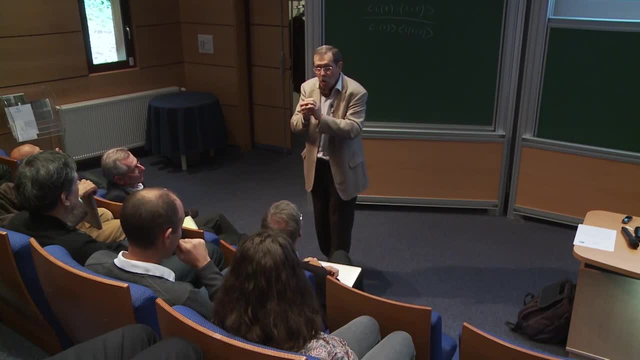 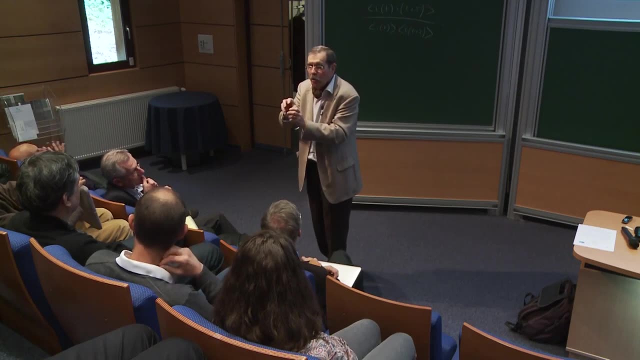 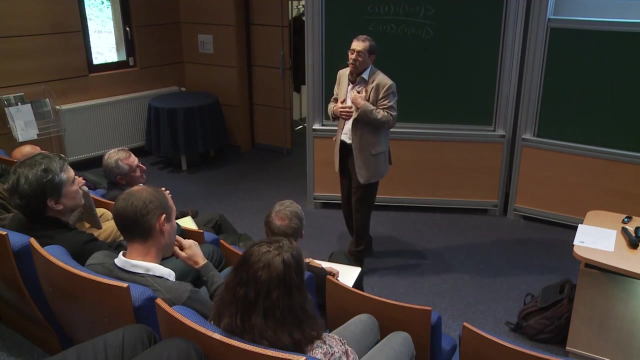 What we will have is small local applications microprocessor with a well-defined task doing a well-defined task here. This, yes, but universal quantum computer? I have no idea. So my personal position is that we have to be very careful about this hype. 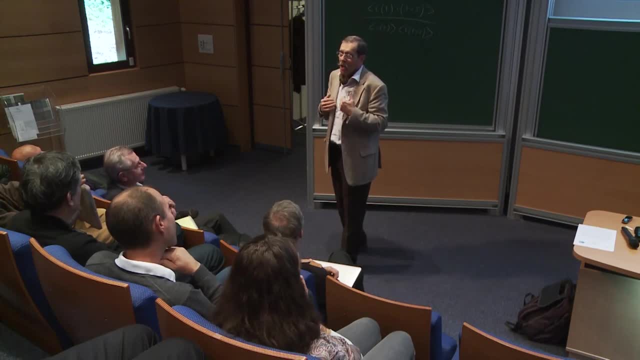 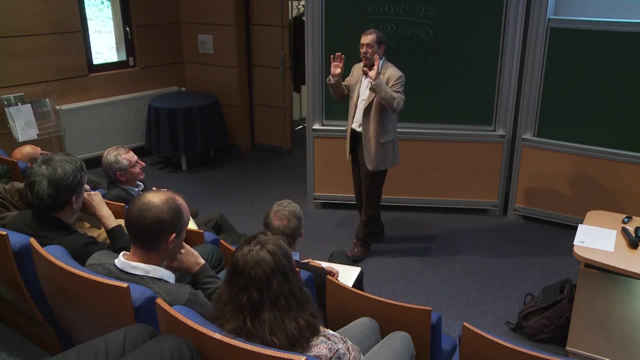 because at one point there will be backlash. So I'm old enough that I will not be hurted by the backlash, but my young colleagues could be hurted. At least they cannot say that I promised too much. I never promised too much. 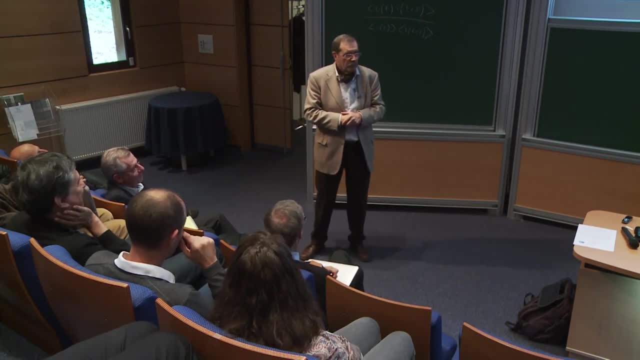 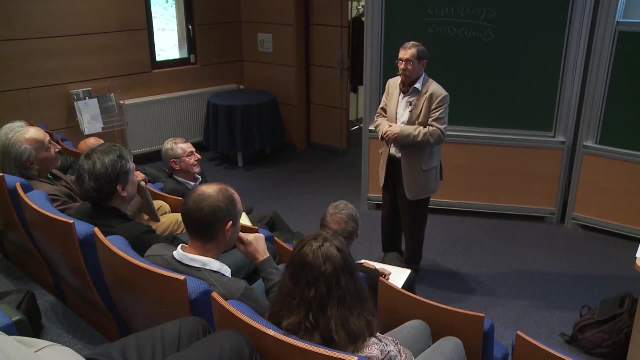 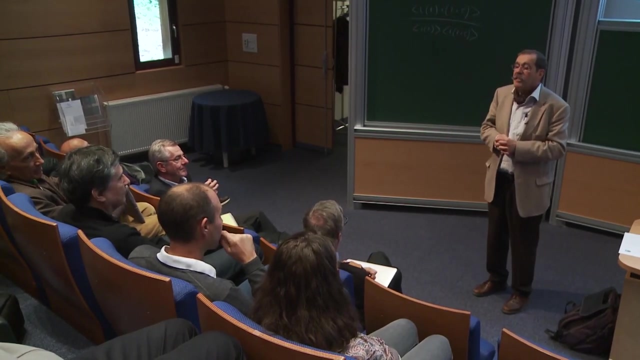 You were there, right, Yeah, Still, China invests $10 billion, I know, And they are good, And they are good the technology, Sure, No, no, they are good. You know, we'll see. It's a very interesting. 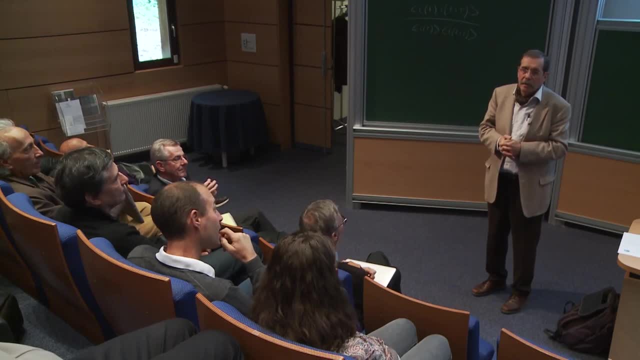 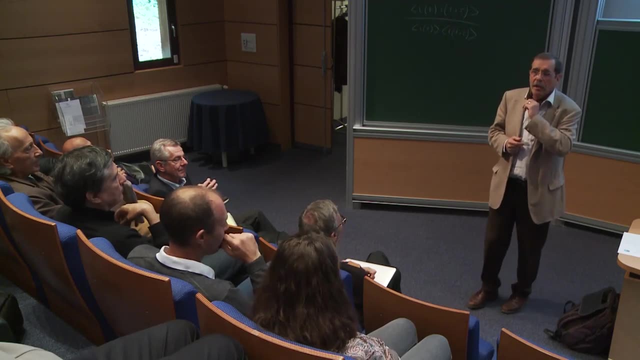 IBM claims. Yes but No. but it's a claim. It's not a universal quantum computer. It's a universal quantum computer. You know, a good news is that there is a European, French, but let's say European company. 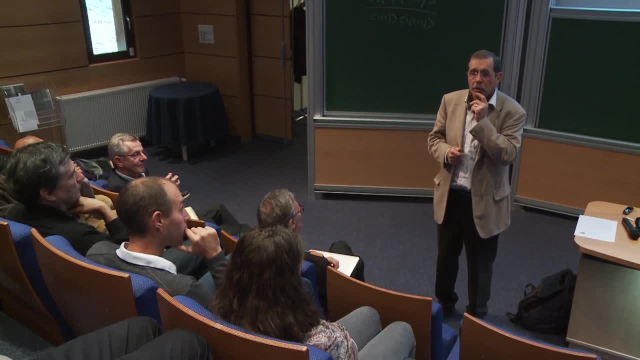 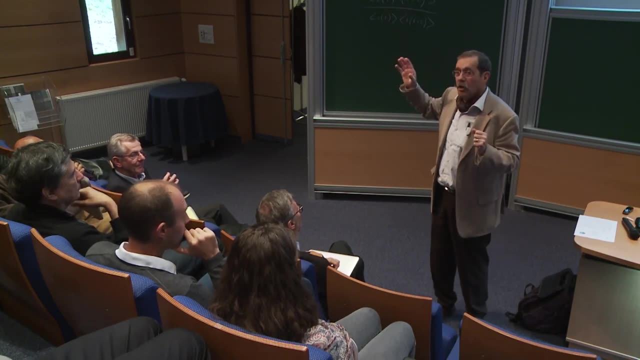 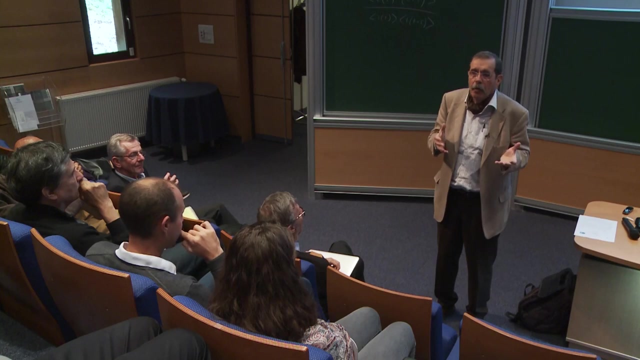 which has taken the challenge. It's Atos, Thierry Breton. Thierry Breton says there is no reason to leave only the Chinese and the American. So there is a quantum computing program with Atos And because Atos is not doing anything in hardware. 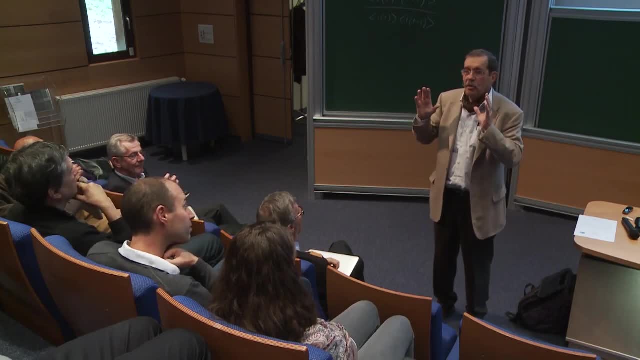 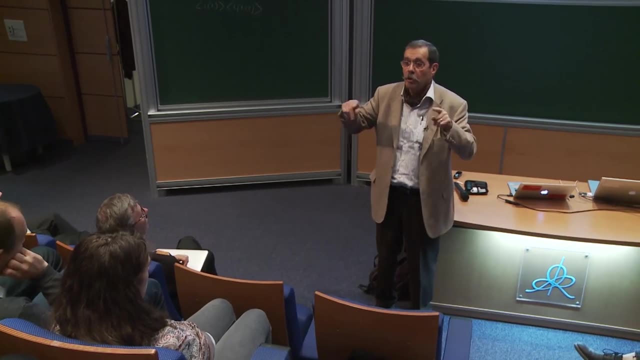 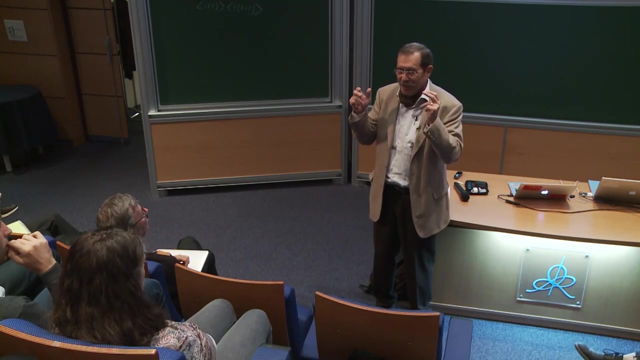 in fact he has attacked the problem of software. What he is doing is the following: Because Atos has now the most powerful European computer- Bull computer, Not in the world but in Europe, that's the most powerful computer They can with an ordinary between quotes, but powerful computer. 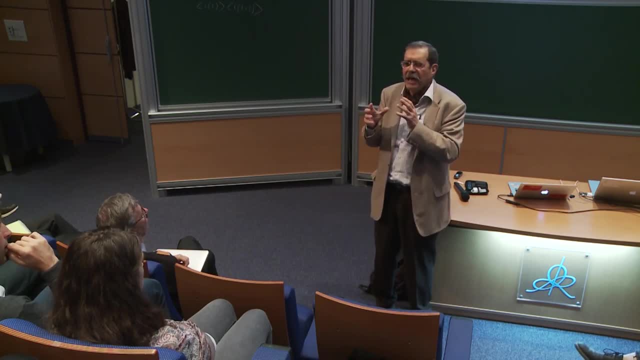 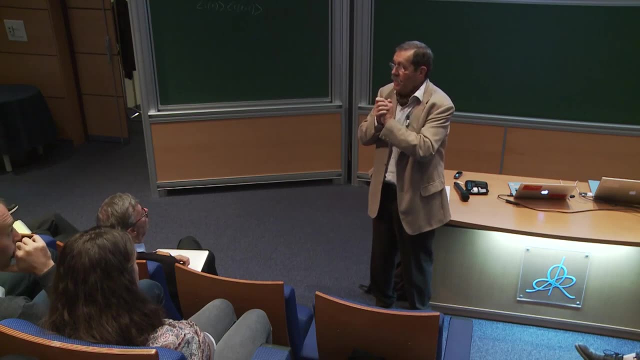 they can mimic something like 30 entangled qubits, And so they say: now if we had 30 entangled qubits, what could we do with it? And what they come to try to develop is a good interface with a high level language, to say: 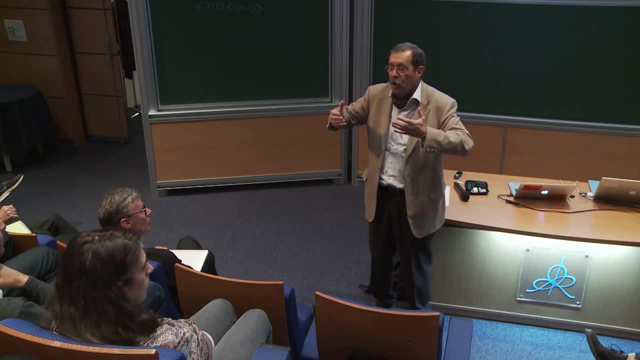 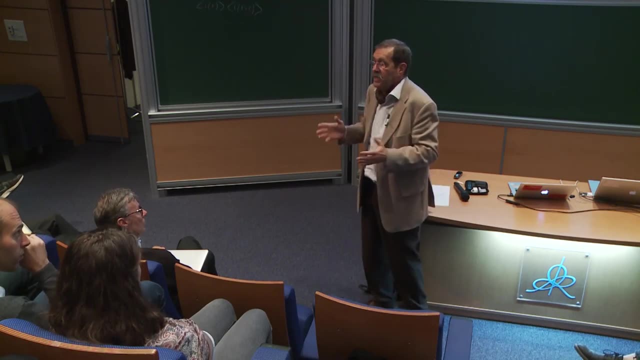 what kind of algorithm can we develop if we have a quantum computer? How should we have a convenient language of programmation, et cetera. I think it's an interesting, because it is what they know to do, And so I'm happy. 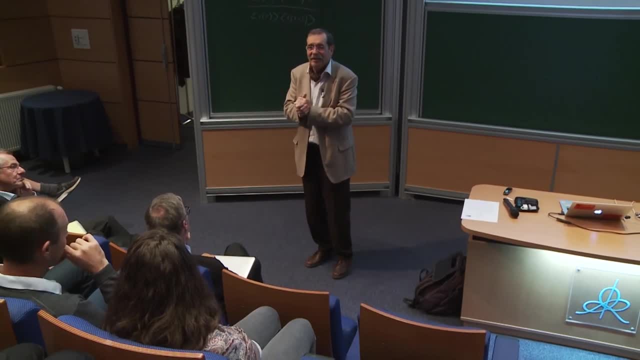 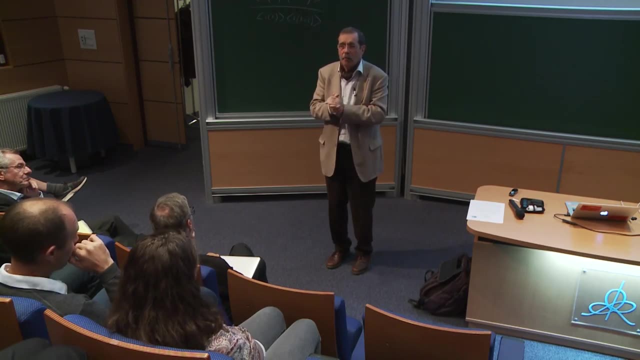 I must say I belong to the scientific advisory board, but I think it's great. It's very nice to see a European company taking the challenge to say we are not absent, We are in the game, But of course they are not putting billions.